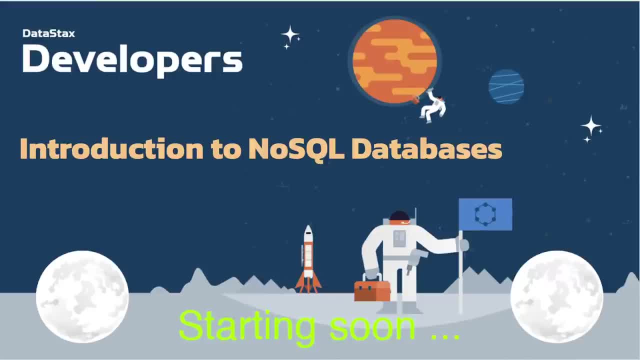 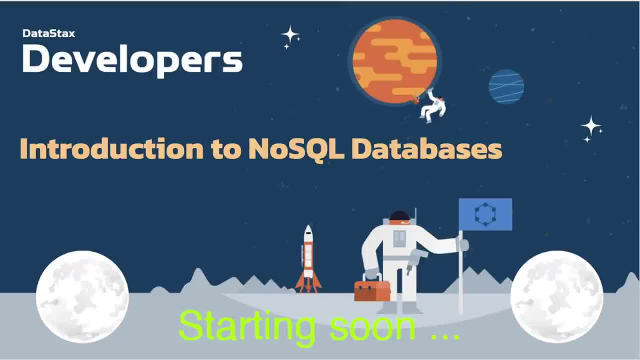 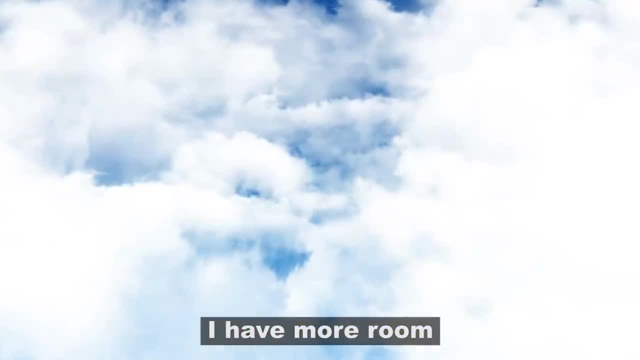 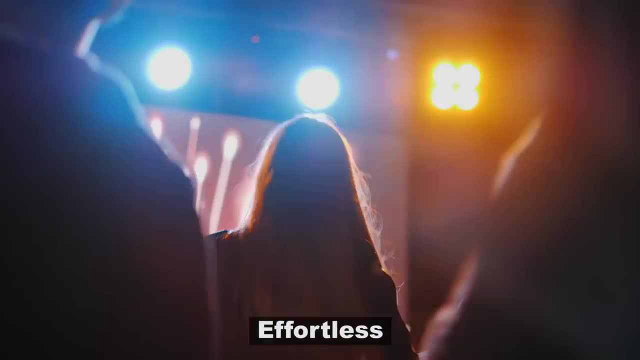 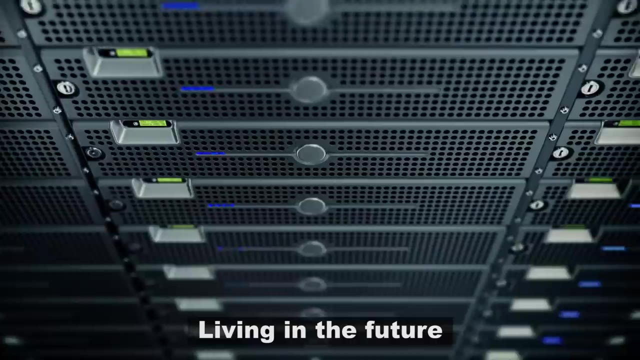 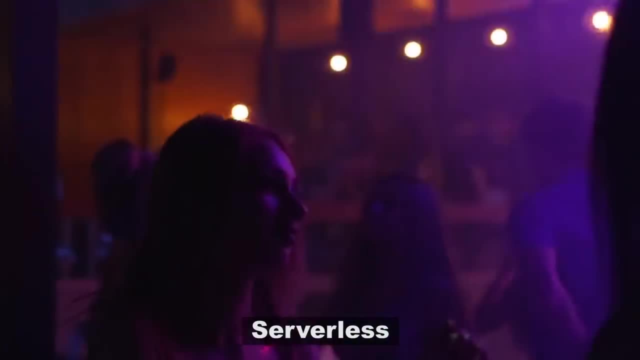 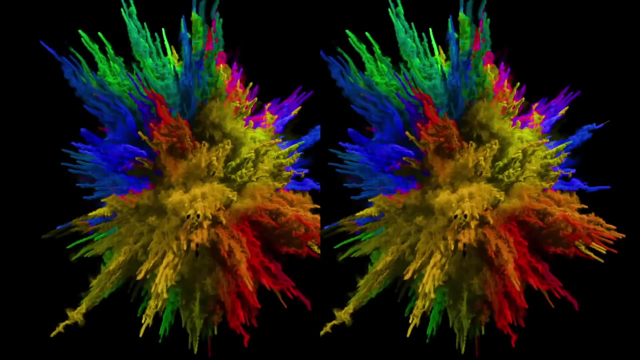 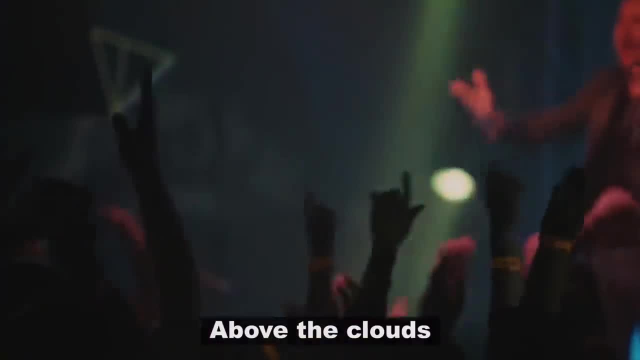 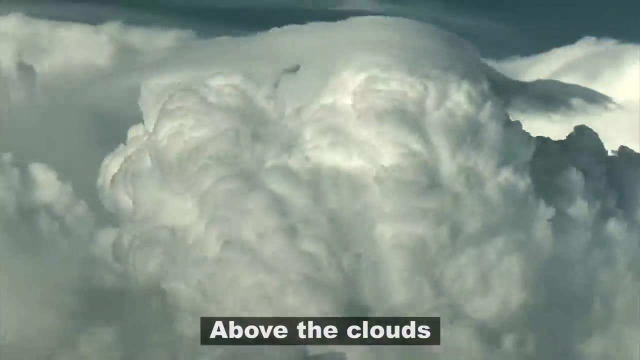 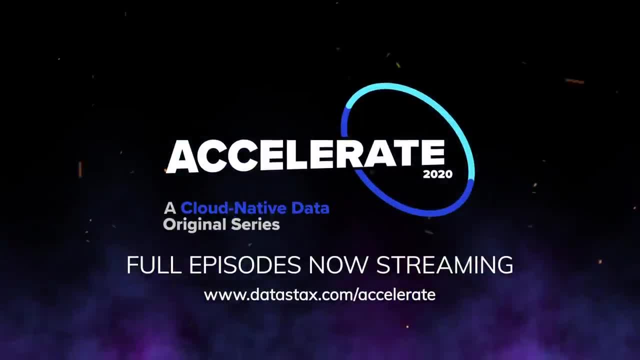 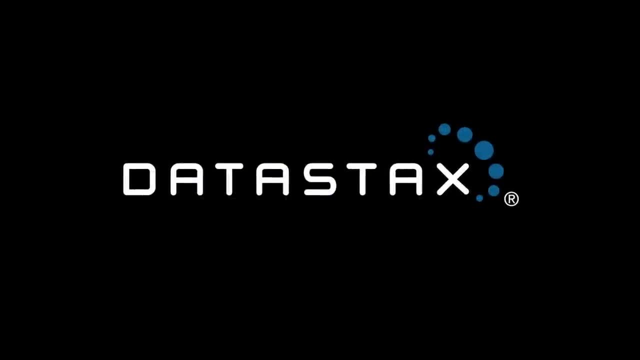 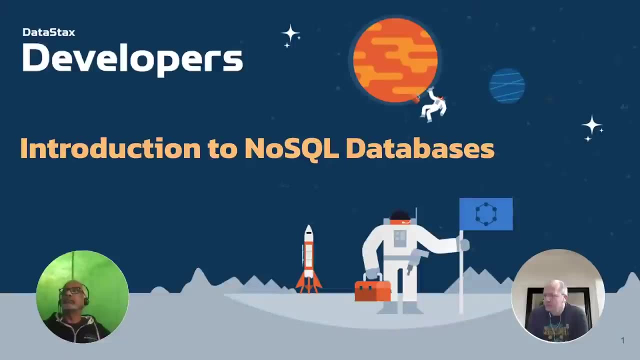 Thank you, Thank you, Thank you, Hello, good morning, good afternoon or good evening, whichever part of the world you're from, you know glad to be part of this really international community. I know I see people chatting, you know, checking weather at different. 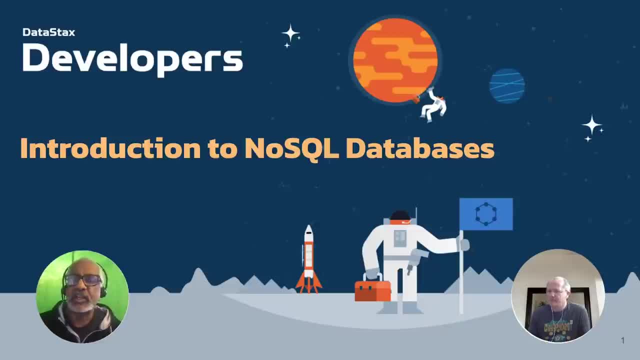 parts of the world, you know. but welcome to this edition of the workshop on introduction to NoSQL databases. As many of you who have been on our workshops together, the first thing we do is make a sound check. So I myself Rags. I will introduce myself in a little bit. 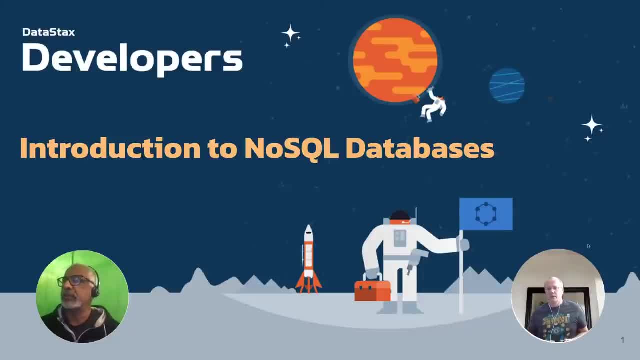 but, Artem, can you say hello and make sure that the sound is good? Yes, hello everyone. Hello everyone, glad to be here and talk about NoSQL databases to you, Perfect, All right. So let me see if I can share my presentation and then we can go from there. 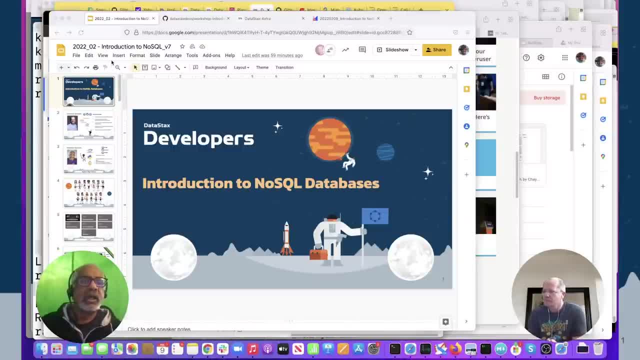 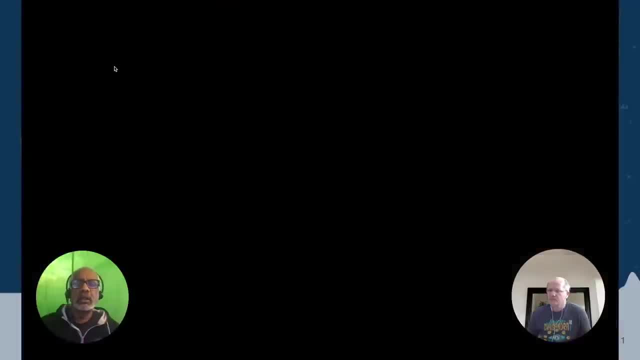 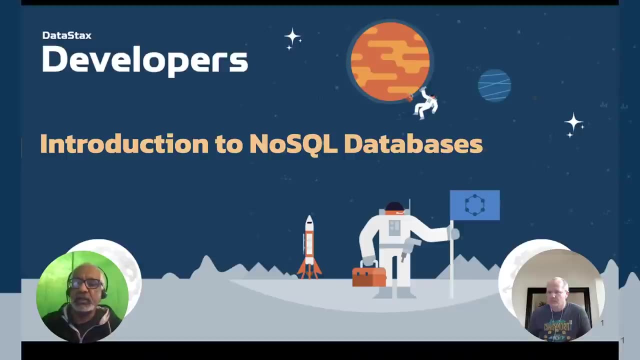 Okay, so I'm good And let me go ahead and present. Okay, So again, my name is Raghavan Srinivas and we are here to talk about introduction to NoSQL databases. Welcome again. Can you go to presentation mode? 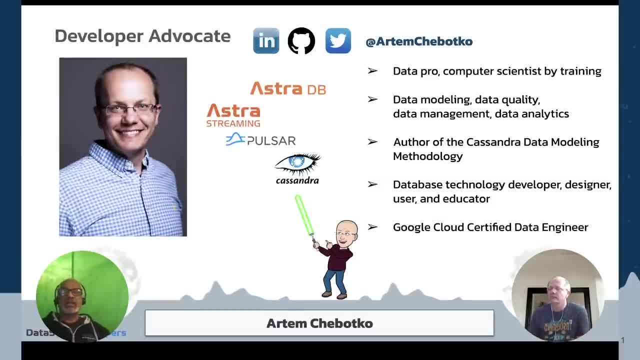 And what we have here is the famous Artem Chabotko- Now hopefully I'm saying that right, but you know he can geek out for hours about data modeling, But he's here today. So, Artem, why don't you introduce yourself? 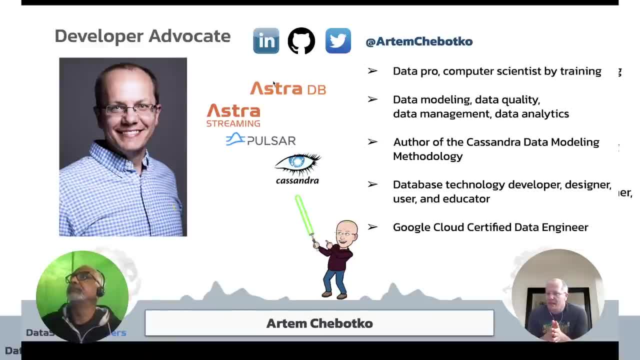 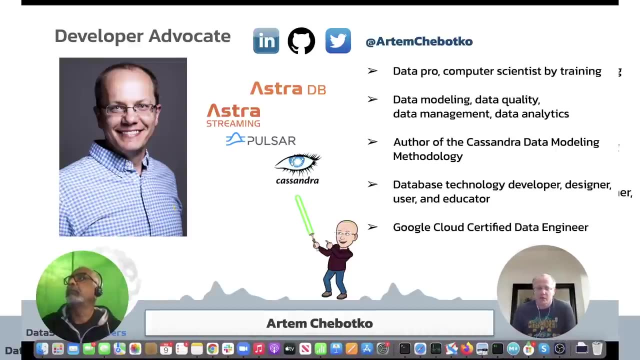 Yes, thank you, Rags. indeed, I love data modeling and data management in general: data quality, data analytics, all those kinds of things about data. I did also the Cassandra data modeling methodology. Maybe you use it, maybe you've heard about it. 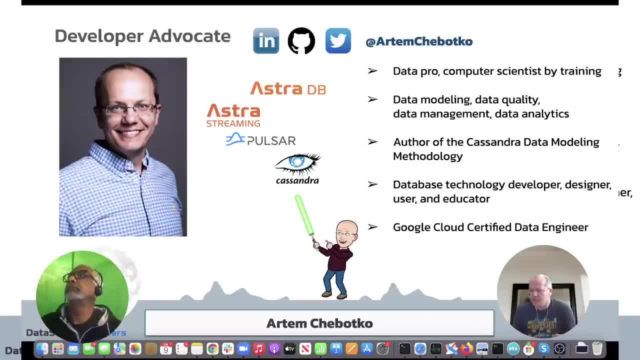 But I'm also a user of databases. I use dozens of different databases and I'm using different types of databases these days, whether it's NoSQL, relational or modern data warehouses like Snowflake and BigQuery. So today I'll be happy to share some of my experience, some of my knowledge about those. 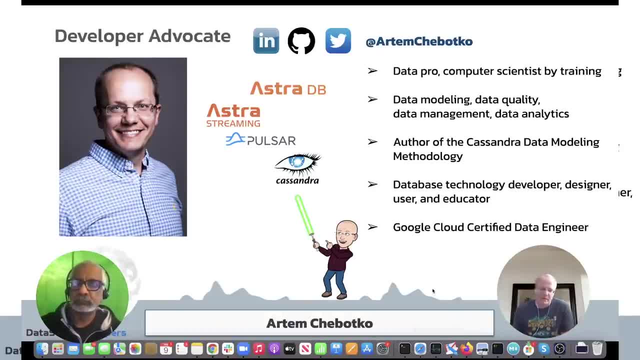 databases- about NoSQL databases specifically, and we're going to talk about several of them. I'm also a Google Cloud certified data engineer and I'm proud to work with Cassandra, AstroDB, AstroSteam and Pulsar. We're going to discuss those technologies as well. 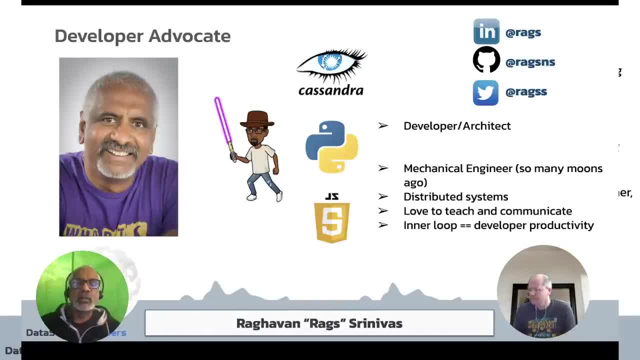 Rags back to you. Perfect, So my name is Raghavan Srinivas and, for whatever reason, people in the world have a tough time pronouncing my name. I have no idea why, but I just go by Rags. 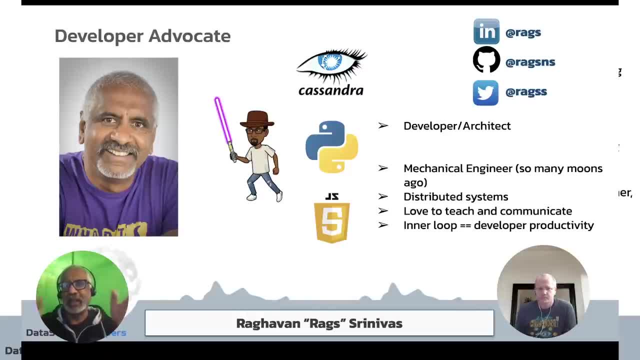 You know Rags on LinkedIn, I'm RagsNS on GitHub and I'm RagsS on Twitter. I just can't make up my mind, right, But I basically I'm a mechanical engineer- Cut the mentee music. I thought I did. Let me try that. Just give me a second. 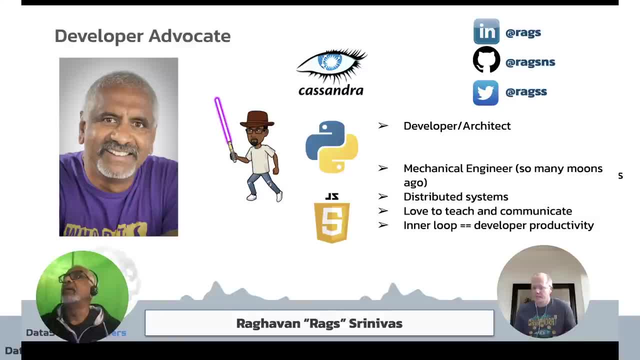 And I'll cut the mentee music. If it's still on, let me know, Is the music bothering? But if not, let me keep going. Let me know if it's still on. But really, welcome to everyone, and I think Artem and I were talking about this. 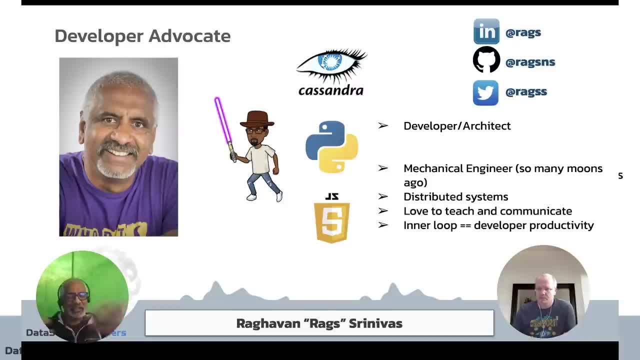 It's so much easier when you're live and you don't have to worry about, you know, these kind of virtual tools. but I think we have created a great community and you guys are part of the community and really you know I want to welcome you back for those of you. 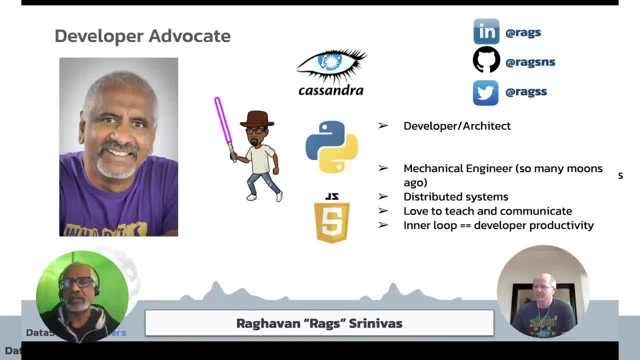 who have been here before. But again to go through my introduction, I'm a mechanical engineering engineer. I've done a lot of distributed systems. you know typically, mostly you know middleware, So you know, as long as things are working, nobody notices me right. 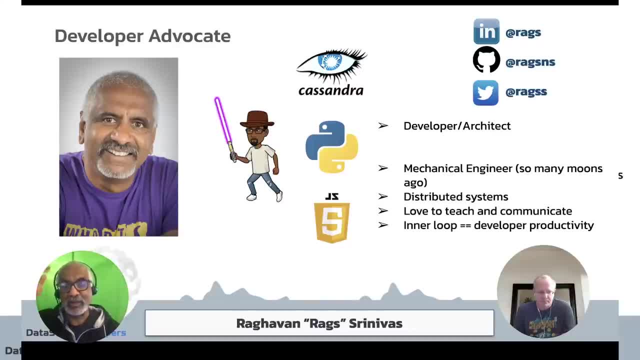 And the moment things don't work, you know they will. they will, you know, find me right. I love to teach, I love to communicate. I live in Boston, where I've taught a number of undergrad and undergrad courses. Actually, Artem also has taught, So so you know, the idea of our group is 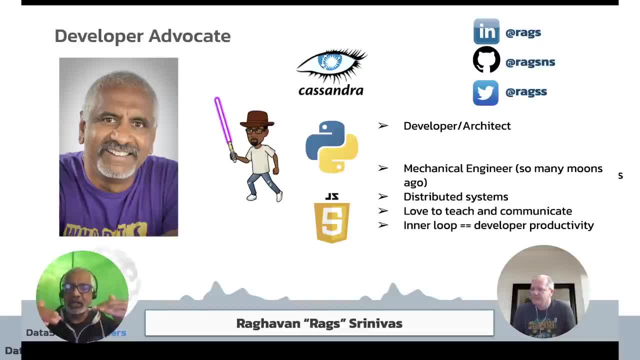 to level up developer skills, no matter where you are, whether you're starting or whether you are an advanced developer, and we'll talk about you know all that in a second. I'm a big fan of what is referred to as the inner loop, which is really about developer. 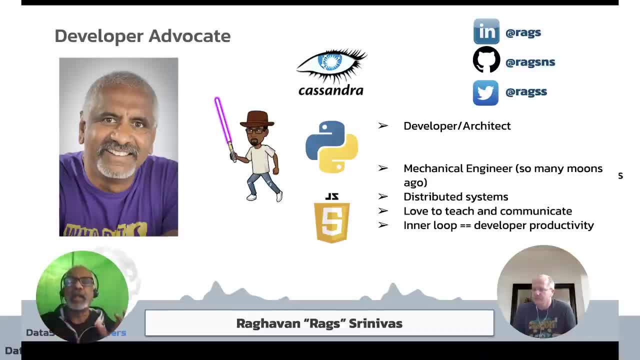 productivity, where you do these things, you know multiple times during the day and you want it to be as quick, as easy, as seamless as possible, and you know. with Kubernetes, with you know, with some of the newer platforms it's a lot easier, but it's still not there. 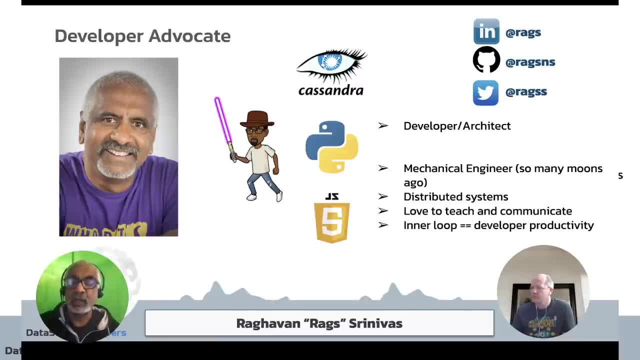 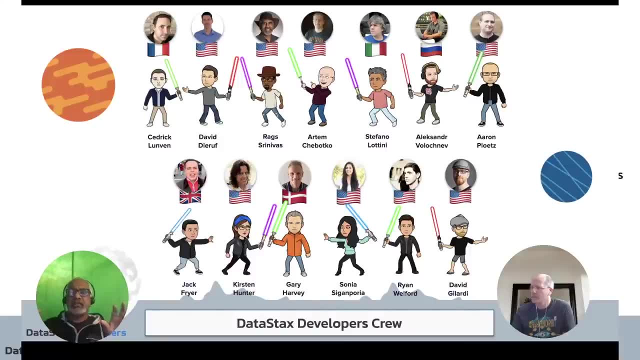 yet, I mean, this is what we've been striving to do for almost three decades. Okay, So, although you see Artem and me on the screen, there are plenty of other people who are helping put this together. You know, in fact, there are some people who are not even on this screen. 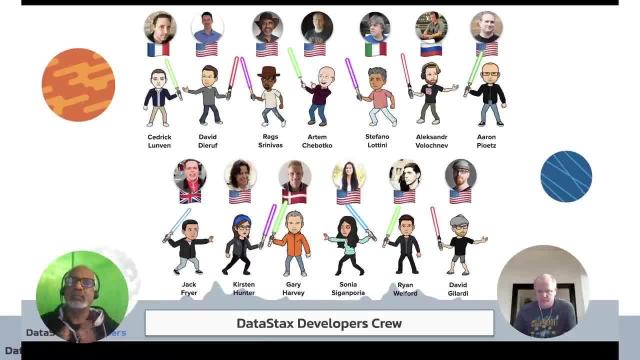 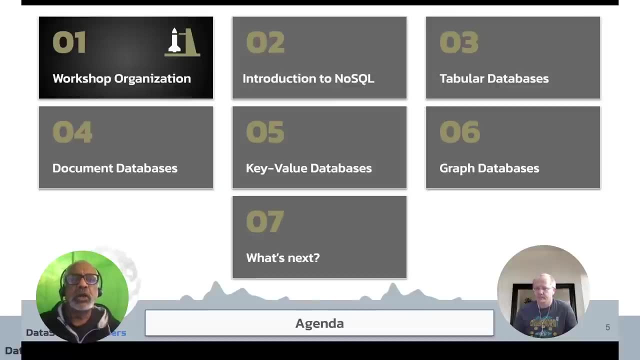 all around the world. you know, all trying to help. you know, basically, make sure that you guys have a good time during the workshop. You have some fun, but, more importantly, you also learn. Okay, So we will. this is kind of the agenda for today. We will. you know, this is going to be about two hours, so we will. it will be pretty fast, you know, but at the same time you will have instructions just in case you're falling behind a little bit. no worries. 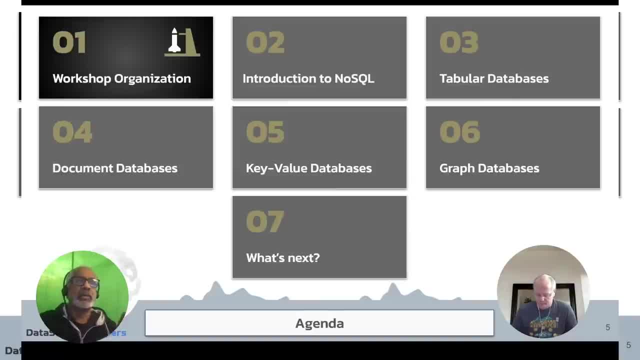 You know I have fallen behind plenty of times and all that I do is go back to my instructions and kind of look at it right. If you want to, you know you can just hit exclamation- GitHub, You know, and Nightbot will respond to you about where the instructions are and you can. you can start following that, Okay. 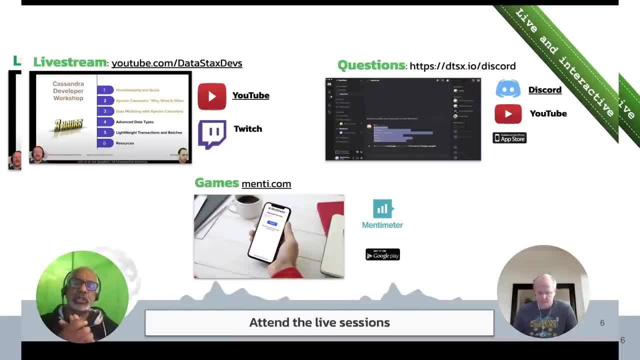 We are live streaming on both YouTube and Twitch, you know, just in case YouTube goes down and we've had some issues before you can, you can go to Twitch, but we respond only to YouTube chat. Okay, So there are two things to be aware of If you want to chat. 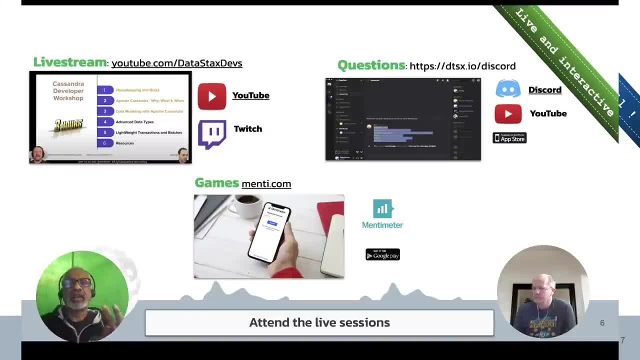 you can either go to YouTube or you can go to Discord. We recommend Discord for more. you know, detailed discussions, something that are, you know, probably going to last beyond this workshop, right? And then, of course, there is Menti. So when we get to the Menti part of it, don't do anything in chat, you know, do everything on Menti. 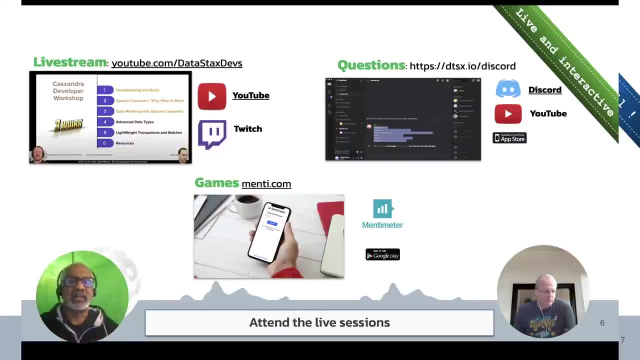 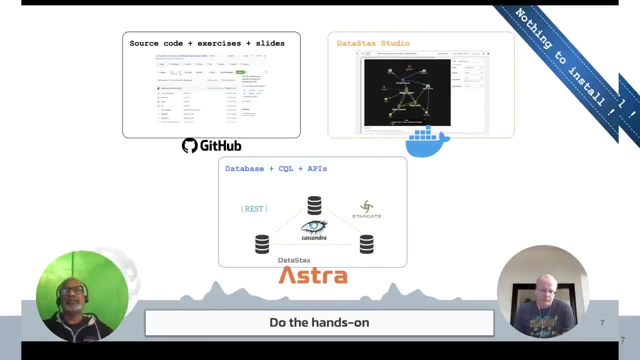 And for some of you who attended this, you know the drill. it's pretty straightforward. I think that's good enough for that slide, but there are plenty of resources, And I keep talking about this: This is a golden age for developers. 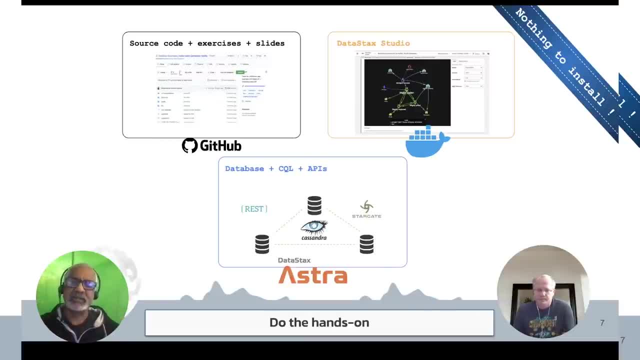 There are so many resources and the best part of that is it's free right. Most of it is free. you know, and I think you can, you can really, you know, experience a lot of this. One of the first things you know: I come from the Cunningham and Ritchie side of the world, you know, remember the hello world right. 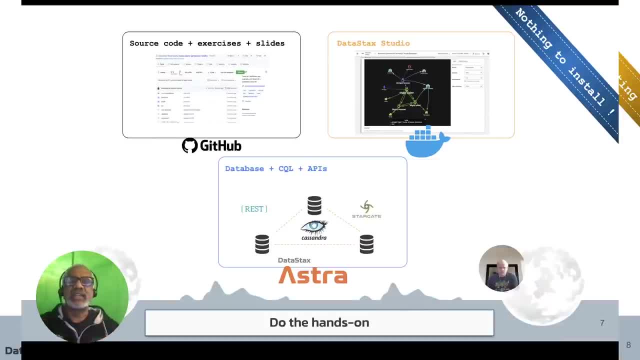 So time to first. hello. world is so quick these days because you know you can do a lot of things. You know you can get started pretty quickly today. okay, So some of these are GitHub- We use what is referred to as Gitpod. 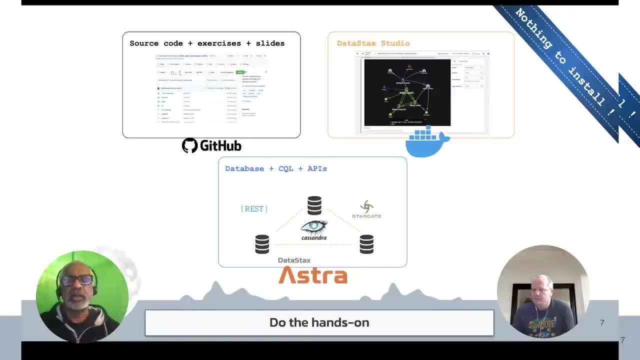 Today we are not going to use Gitpod, but you know, typically our workshops use Gitpod. And then of course there is Astra, which is what we call the serverless database. And the nice thing about all our workshops: nothing to install. 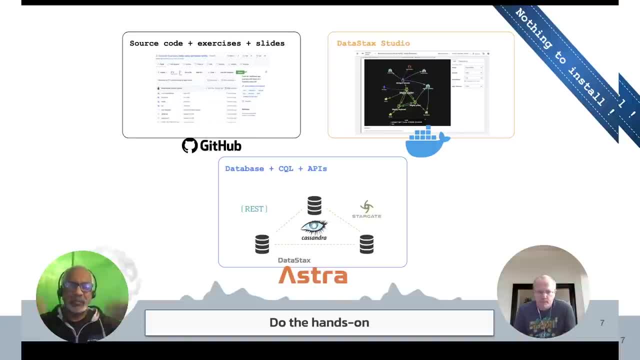 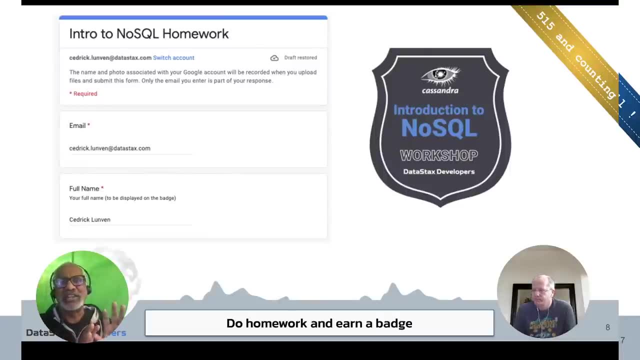 Just come, you know, do stuff with us, practice, practice, practice and then have some fun. okay, So I've said enough, but you know we're not going to let you easy, right, You know we'll make you do some homework. 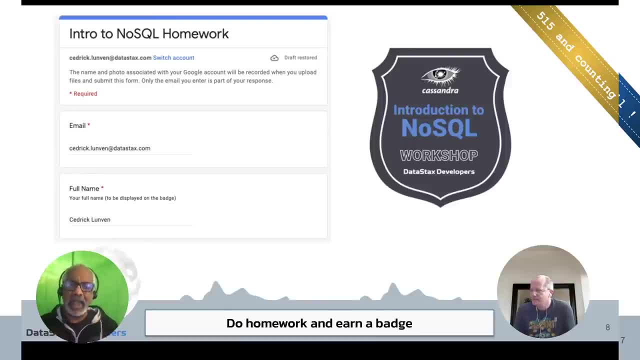 So you know, if you're serious about kind of earning a badge, if you want to earn a badge, bragging rights, you know, as some people would say, you know maybe your salaries will go up depending on the badge. 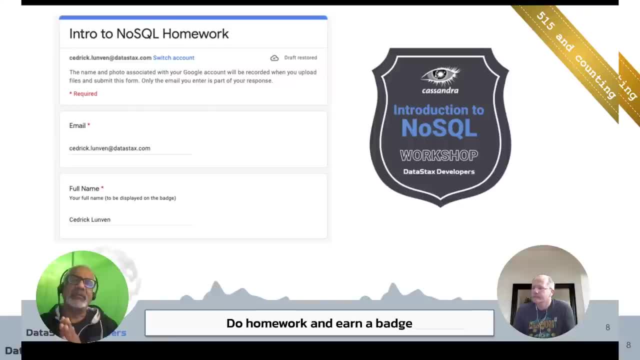 You know, no guarantees there, But you know, I think the important part is that you learn a lot by the homework as well, So you do practice, Then go back and try it out. We typically don't have a time frame for submitting the homework. 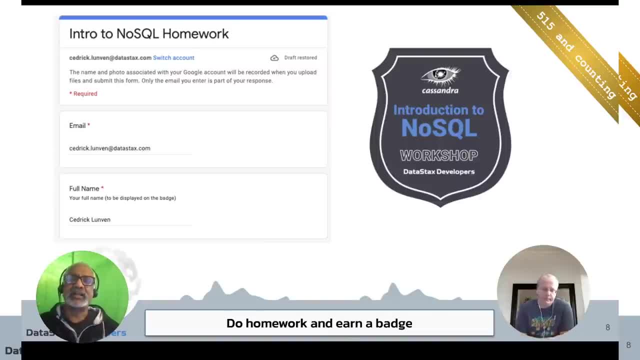 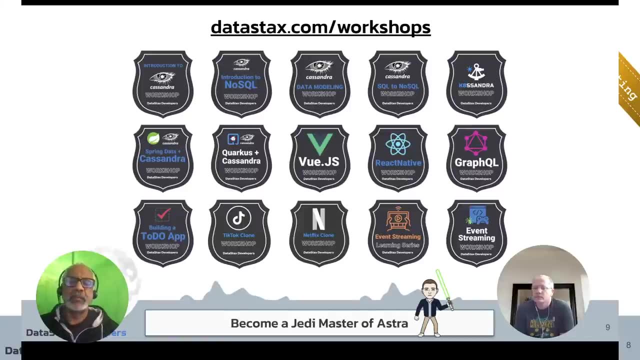 You know we are not, you know, a very tough grader. Typically we recommend like two weeks after the workshop. There are plenty of other badges as well. I don't know if we have. you know who has, you know how many badges, and leaderboard on badges and things like that. 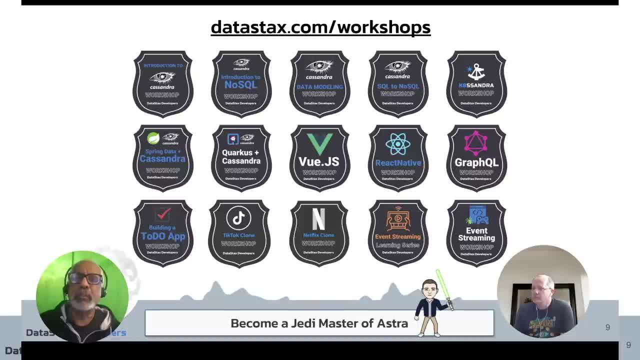 Maybe we should start something like that, But I know that many of our attendees they lose. So if you like this part and you know, just earning the badges- a variety of different ones, you know, like intro to NoSQL, Cassandra, data modeling- you know, maybe Artem will be back for that. 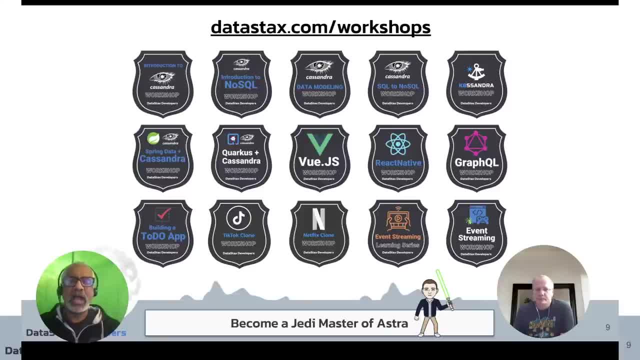 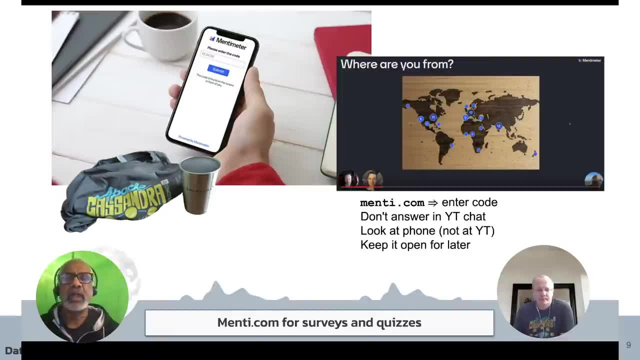 You know, even streaming, building a to-do app. you know a very simple to-do app: Quarkus Spring Data. you name it. Okay, So I'm not going to spend too much time on that, All right. 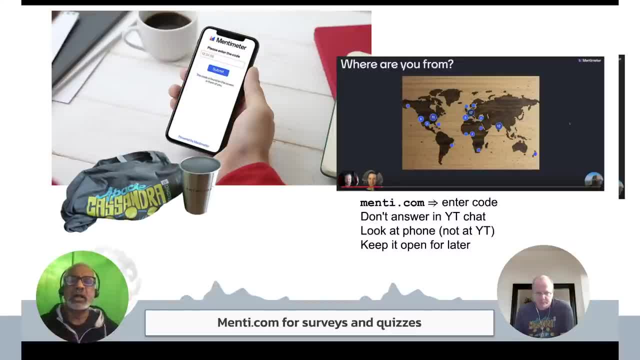 So again, you know, some of you have seen this Before- what we do here is we're going to go into Menti. Okay, And to go to Menti, what I have to do is I have to do a couple of things. 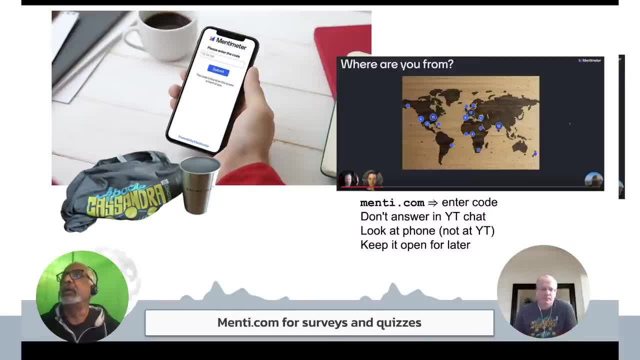 So you know you may also want to subscribe to our workshops. You know you subscribe to our link and we'll put that out at the end as well, But just in case you don't stay till the very end, you know, just wanted to inform you right now. 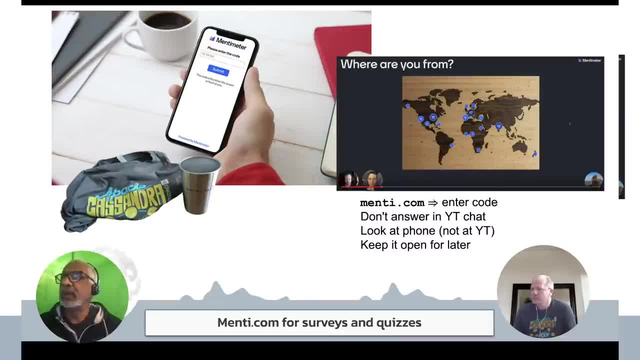 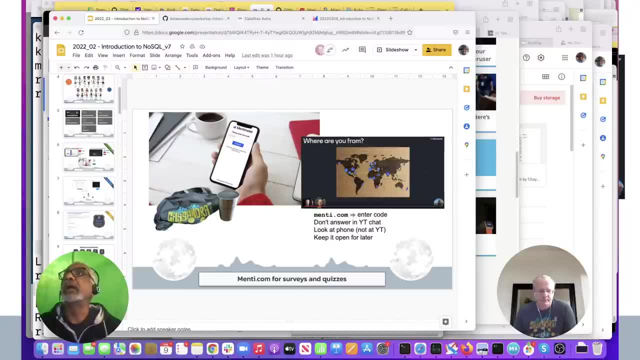 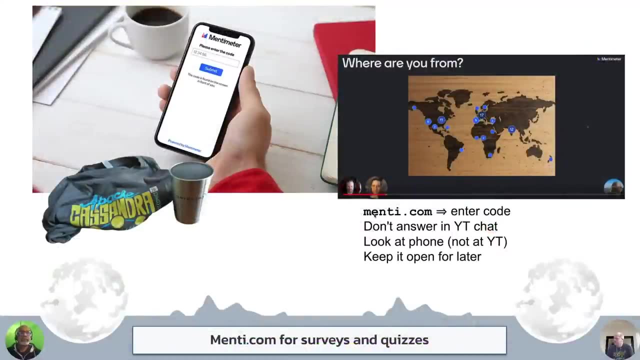 With that said, let's go to Menti. Okay, And for those of you who have done Menti, you know the drill, But let me make sure I go back to something All right. Okay, So let me present Menti. 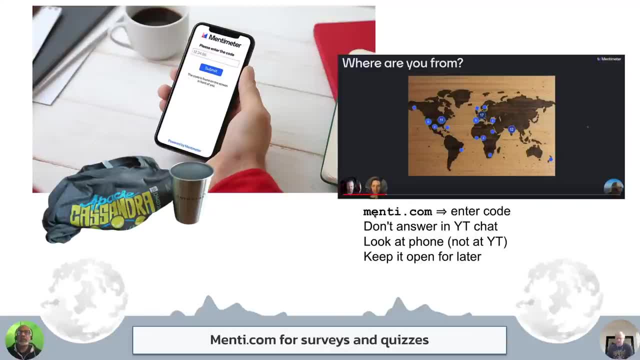 All right, Give me a second here. All right, Let me go into presentation mode. All right, All right. So here's the link For those of you who know how to do this pretty straightforward right. Basically, go to Menticom and enter the code 48153410 and it'll be available throughout. 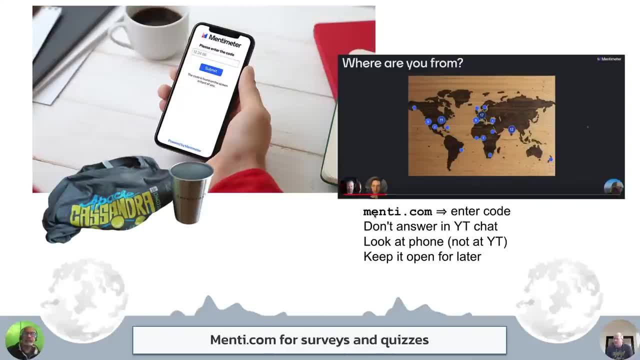 Or, if you want to just hit bang Menti, you will get the code as well. Okay, We have a few questions just to warm you up, But the idea is that you know, towards the end. you know, basically, Artem has created a quiz. 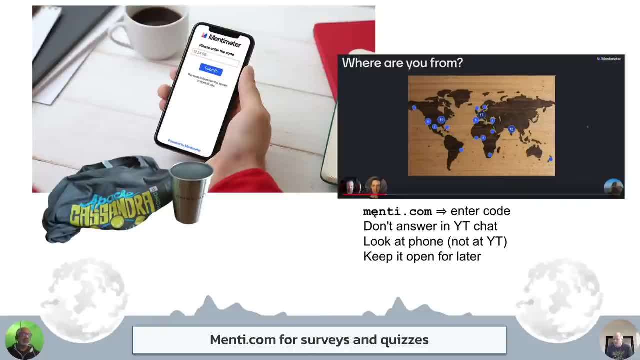 And you know it's not trivial but it's not, you know, terribly difficult. You know you'll see that if you answer those in time and you answer them correctly, you'll have a chance to win swag. So, with that said, let me get into the Menti. 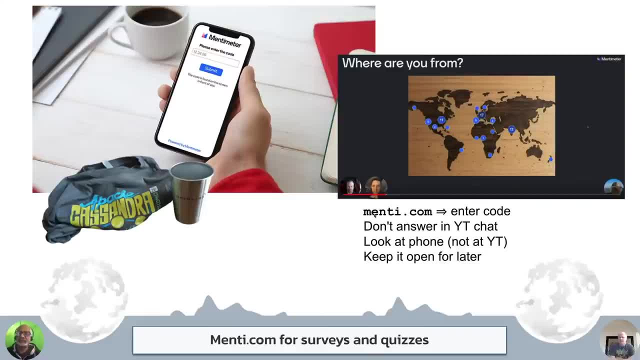 First question: This Menti quiz is pretty short. We're going to in a few minutes we'll start talking about databases and doing our hands-on Perfect. Yeah, Exactly, Yeah, Yeah, We don't want to spend too much time on Menti, but we know that people love Menti. 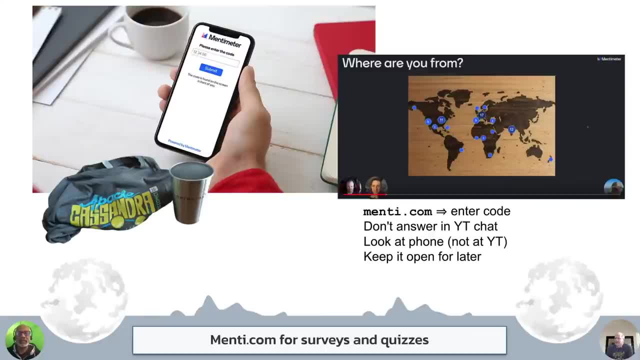 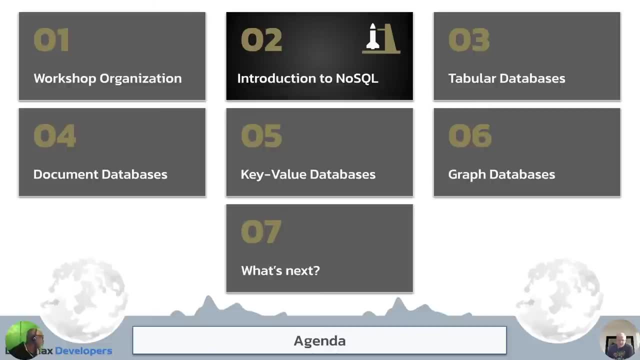 So let's see where you're from. Perfect, We see only 22,, but hopefully we can see a little bit more. I know that we have about 500 people who are out there And for those of you, you know, who are joining the stream for the first time, we were able to get some special permission to do more. 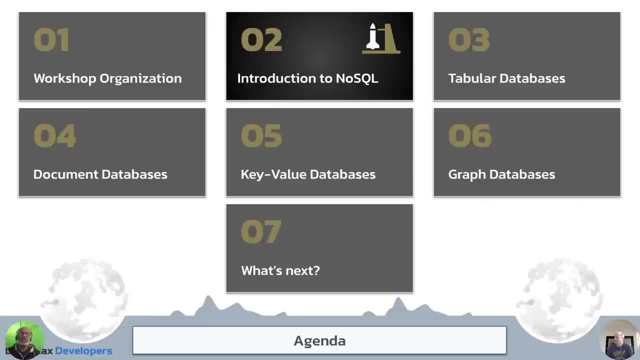 So if you stick till the very end, it's not just going to be the top three, We are probably going to have a little bit more, depending on how many people are at the end of the show. Okay, So you have more chances to win swag. 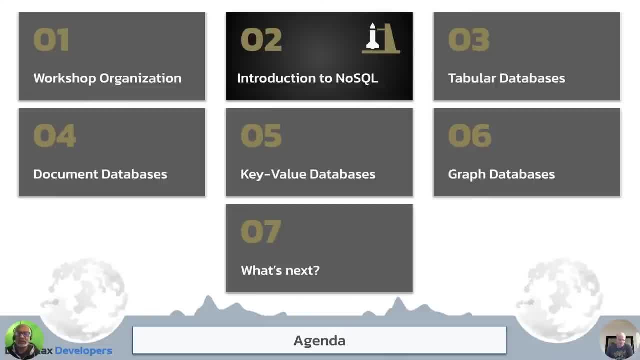 All right. Any comments on this? Anybody from, oh, somebody from, Brazil? That's right, Obrigado, All right, So let's go next, Right? So I myself, I'm from Boston And at this time I keep wondering if this is the place where I want to live the rest of my life. 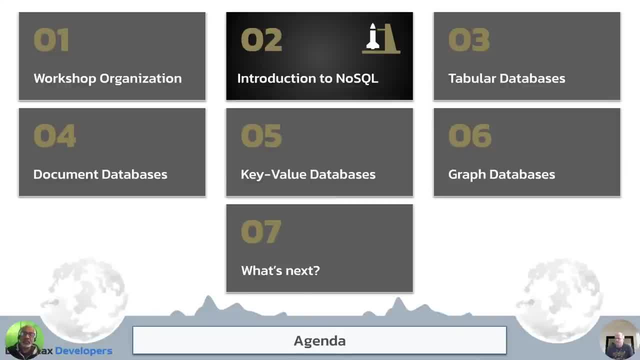 You know, it's pretty cold Today. it's not bad, It's 40s, But I always dream, dream of being in another place. So which continent would you rather move to? If you're happy where you are, that's fine. Love to see that movement. A lot of people want to move to Asia. Wow, I'm happy where I am- Fantastic. A lot of people want to move to North America. That is pretty cool. Move within the continent. Yeah, I would love to go to Australia and New Zealand too. 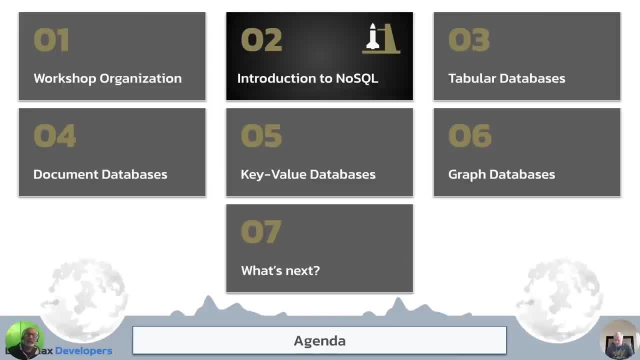 You know I've been to Australia and New Zealand a few times, But any comments on this, Artem. I know you're from Russia as well, right, You know originally I'm not. I'm from Ukraine. Okay, Ukraine. 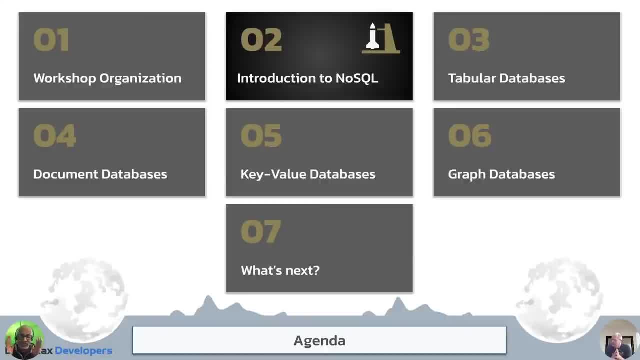 Sorry, Yeah, yeah, Okay, yeah, Big difference, Big difference, Agreed, Agreed. I wanted to comment. I wanted to say that I don't see the Menti on YouTube. The Menti is not showing anything, essentially on YouTube. 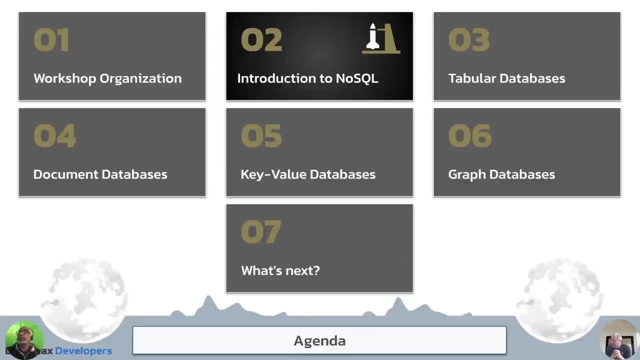 There is no screen, so maybe you can share it or something Sounds good, Okay, Thank you so much. Yeah, but speaking of countries, I did live in Russia for three years, So that's a big question. I'm not able to figure this out. 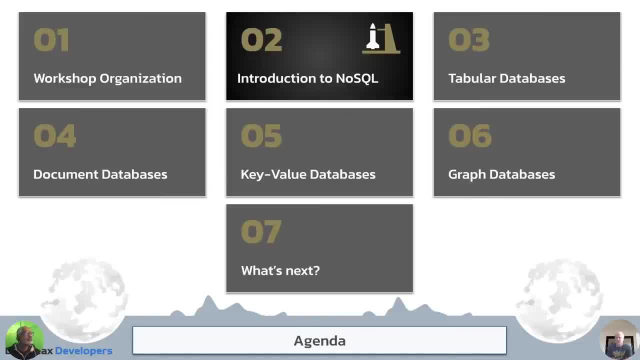 Just give me a second, I'll figure this out. You know what I'm saying. I'll figure this out. Let's see, I'm not able to figure out what those two things are. Let's try to look at it one by one. 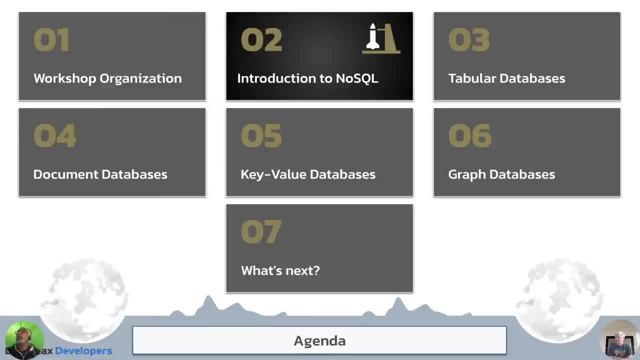 Okay, Okay, All right, All right. So let's go back to our features. Let's go back to our features and we're going to go back to challenges. I think I lost the Okay. There I am Okay. 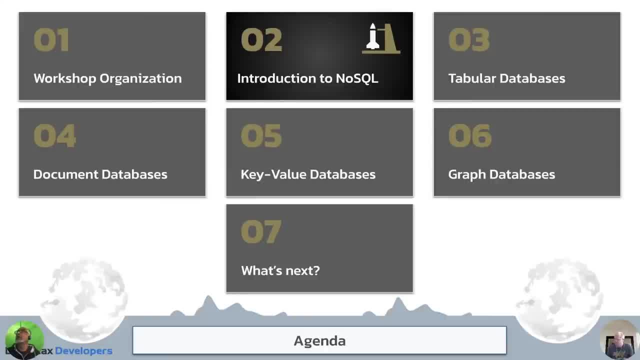 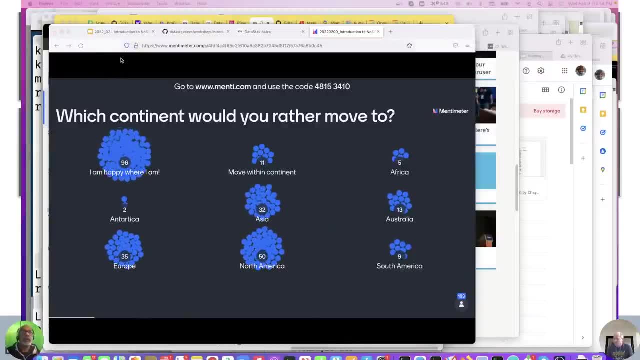 So, yeah, So you should be able to see the main monitor. Thanks for bringing that up. That's great. Okay, Let me go back to Presentation mode. Now you should be able to see Menti, Okay, and you can see here a lot of people happy where you are, and that's great. but 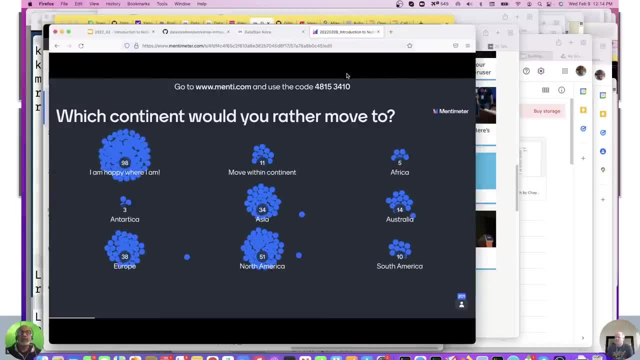 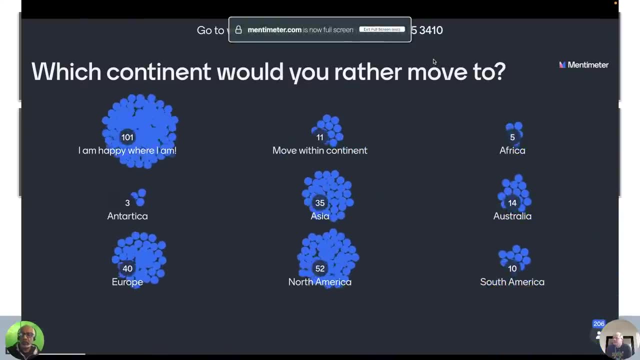 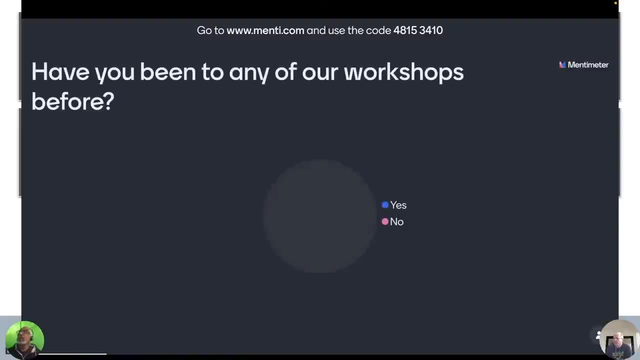 like I said, you know I would. I would like to. at least I feel like I want to move. okay, so let me go back to present. all right, cool. moving on, a few more questions. have you been to any of our workshops before? this will give us an. 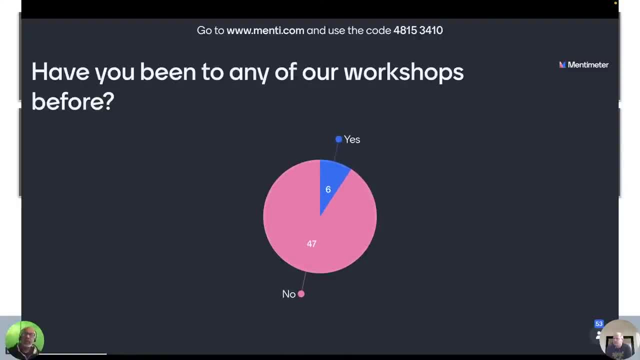 idea of who we were talking to. okay, so that's cool, this kind of what we expect, right? you know a lot. large part of our audience haven't come to the workshop before. hopefully you'll come again, but you know quite a few who have attended workshop before. so welcome back. all right. any other comments? Artem? 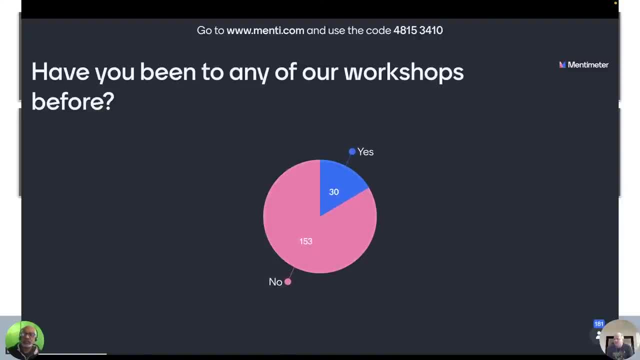 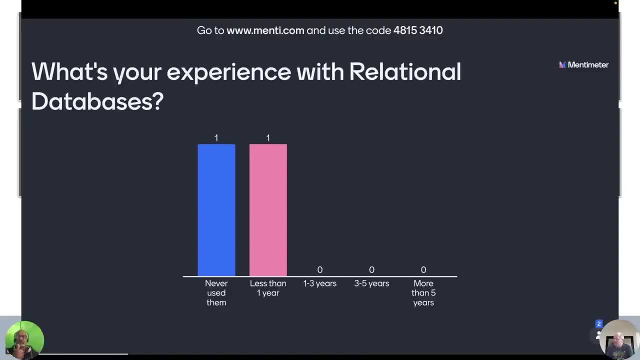 any other comments? Artem. any other comments? Artem? all right, let's get started on the workshop. all right, let's get started on the workshop. all right, let's get started on the workshop right. yeah, we have many new right. yeah, we have many new right. yeah, we have many new people that are over 500 live viewers, I think. 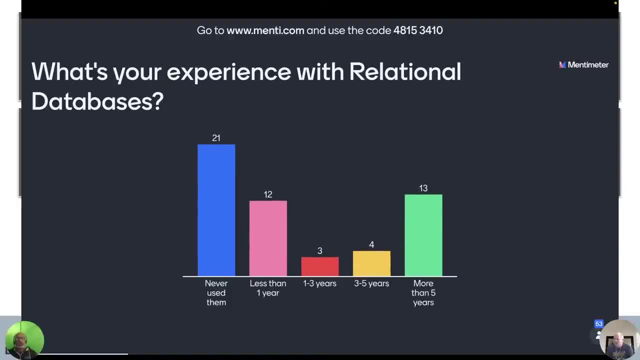 people that are over 500 live viewers. I think, people that are over 500 live viewers. I think these are important for us to know. these are important for us to know. these are important for us to know. you know what's your experience with. you know what's your experience with. 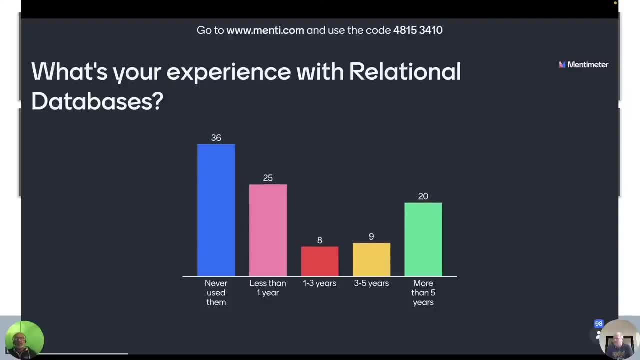 you know what's your experience with relational databases? fantastic, we have a relational databases- fantastic. we have a relational databases- fantastic. we have a lot of people who are more than five, lot of people who are more than five, lot of people who are more than five years of experience and, as you know, we 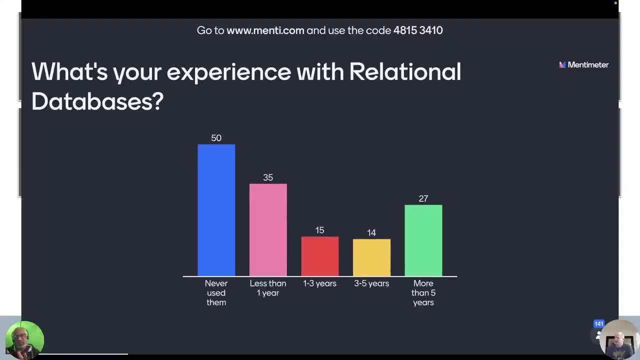 years of experience and, as you know, we years of experience and, as you know, we are not going to be talking about, are not going to be talking about, are not going to be talking about relational, although your knowledge relational, although your knowledge relational, although your knowledge definitely helps and, and you know, I'm 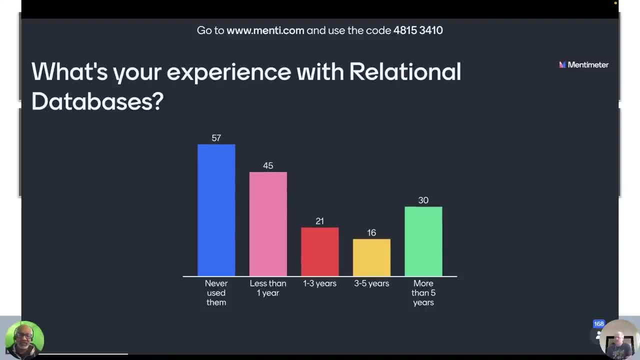 definitely helps, and- and you know I'm definitely helps and and you know I'm- for those of you have never used it, or for those of you have never used it, or for those of you have never used it, or less than a year, or one to three years. 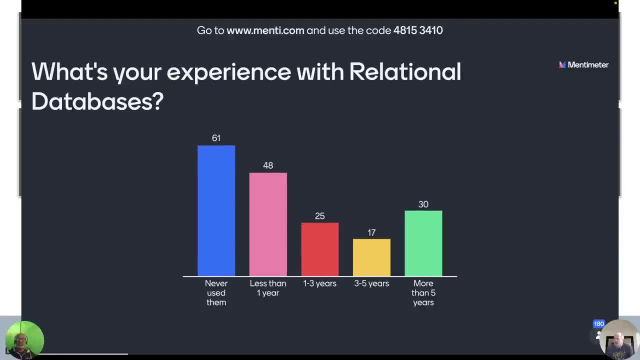 less than a year, or one to three years. less than a year or one to three years, are you still gonna learn a lot here? are you still gonna learn a lot here? are you still gonna learn a lot here? okay, so, yeah, well, that those who never. okay, so, yeah, well, that those who never. 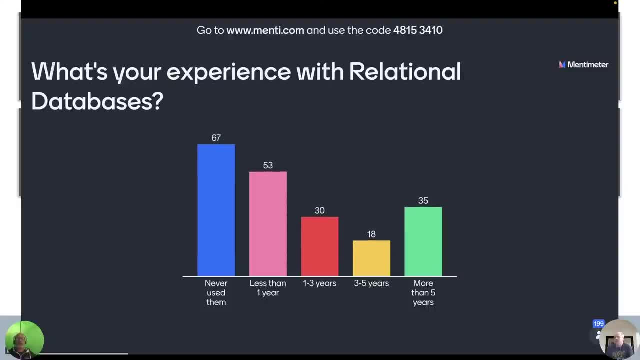 okay, so yeah, well, that those who never use it probably didn't use any database use it. probably didn't use any database use it. probably didn't use any database before. exactly exactly, yeah, more than before. exactly exactly yeah, more than before. exactly exactly yeah, more than likely correct. yeah, very unlikely right. 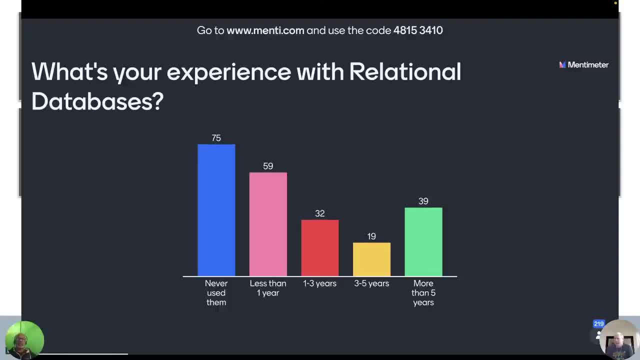 likely correct. yeah, very unlikely, right. likely correct. yeah, very unlikely, right. you know you would have used a no sequel. you know you would have used a no sequel. you know you would have used a no sequel database but never used a relational database. but never used a relational. 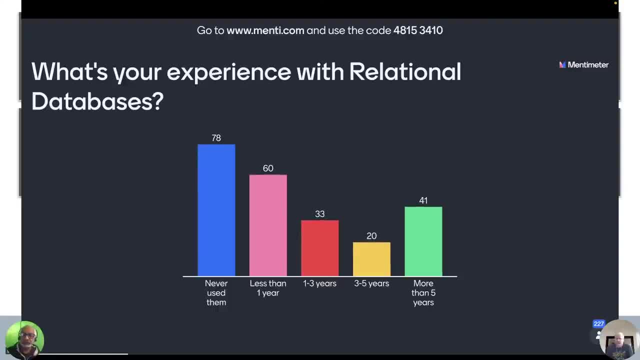 database but never used a relational database. right, yeah, yeah, and my queen database right, yeah, yeah, and my queen database right, yeah, yeah, and my queen all right moving on. what's your all right moving on? what's your all right moving on. what's your experience in no sequel databases? right? 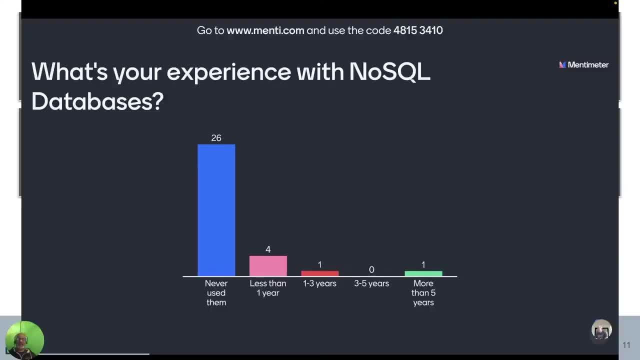 experience in no sequel databases: right, experience in no sequel databases: right, right, thank you, okay. okay, this is kind right, thank you, okay. okay, this is kind right, thank you, okay. okay, this is kind of what we expected, right, so I think I of what we expected right, so I think I. 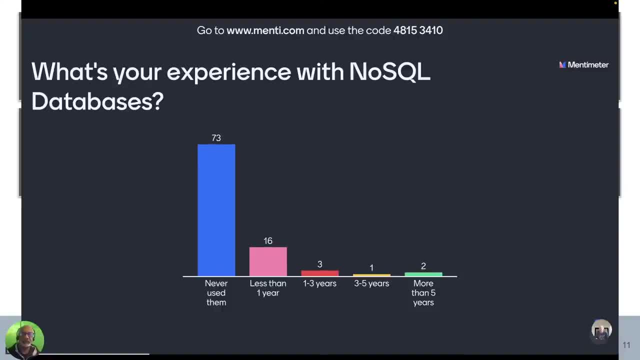 of what we expected right. so I think I think we have the right audience. what do think we have the right audience? what do think we have the right audience? what do you think right indeed, yes, this kind of you think right indeed. yes, this kind of you think right indeed, yes, this kind of what we expected. so let's not dwell too. 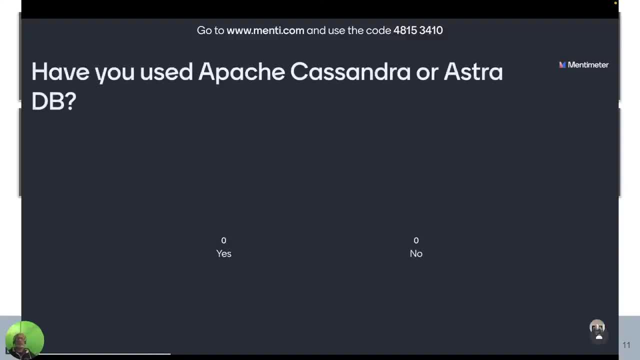 what we expected. so let's not dwell too what we expected. so let's not dwell too much on this, because I don't think it's much on this, because I don't think it's much on this, because I don't think it's gonna be a total surprised. have you used? 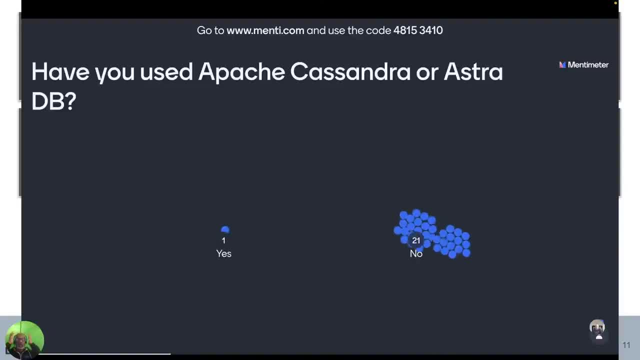 gonna be a total surprised. have you used? gonna be a total surprised. have you used Apache, Cassandra or Astro DB? if you're Apache Cassandra or Astro DB. if you're Apache, Cassandra or Astro DB, if you're like I have never heard of this, that's like I have never heard of this, that's. 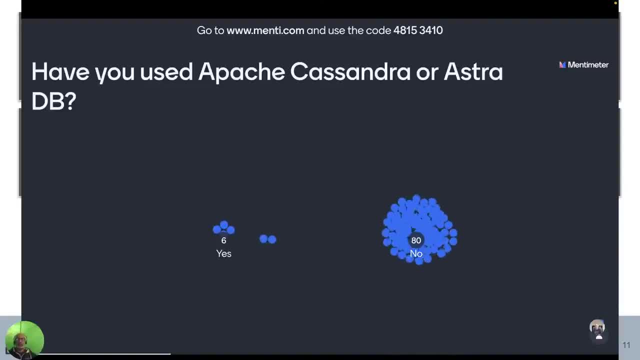 like I have never heard of this. that's fine, you know. so again, kind of expected, right, okay, that is cool, okay, so we have like: okay, that is cool, okay, so we have like. okay, that is cool, okay, so we have like what? maybe like 10% of the people who 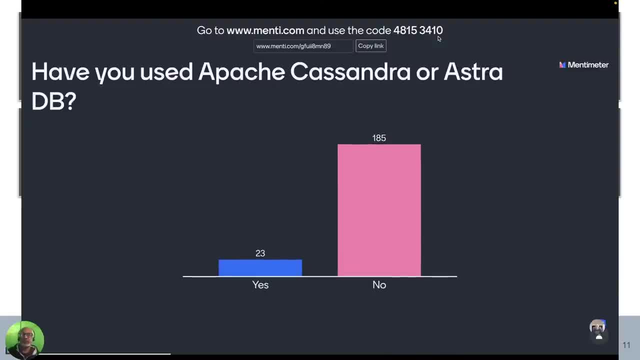 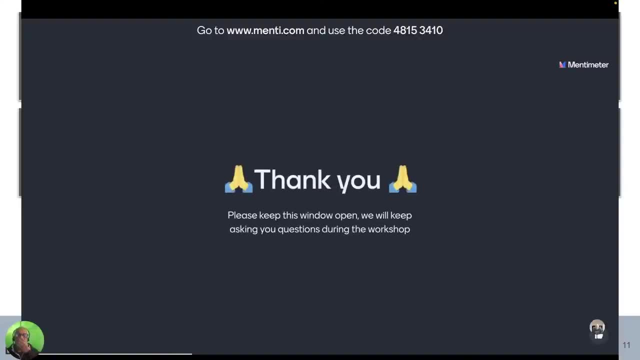 what? maybe like 10% of the people who? what? maybe like 10% of the people who have used Apache Cassandra. so so that's have used Apache Cassandra. so so that's have used Apache Cassandra. so so that's all right, moving on, we will you keep? 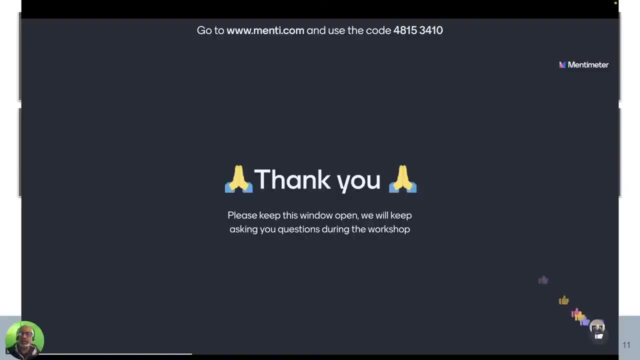 all right, moving on. we will you keep all right, moving on. we will you keep this window open. we will keep asking you this window open. we will keep asking you this window open. we will keep asking you questions during the workshop. okay, so, questions during the workshop, okay, so. 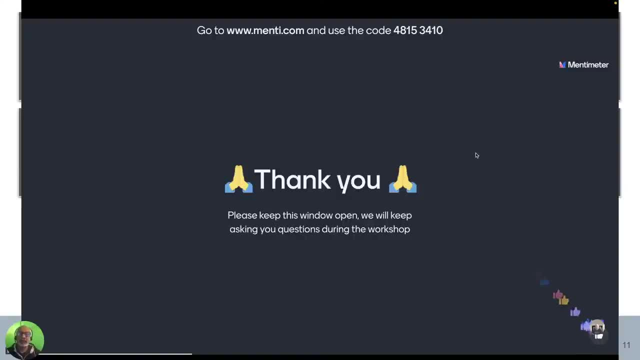 questions during the workshop. okay, so, just just keep it open, right, and we'll just just keep it open, right, and we'll just just keep it open, right, and we'll come back here again with that said: let come back here again. with that said: let come back here again with that said: let me move to. you're ready, Artem, to go? I'm. 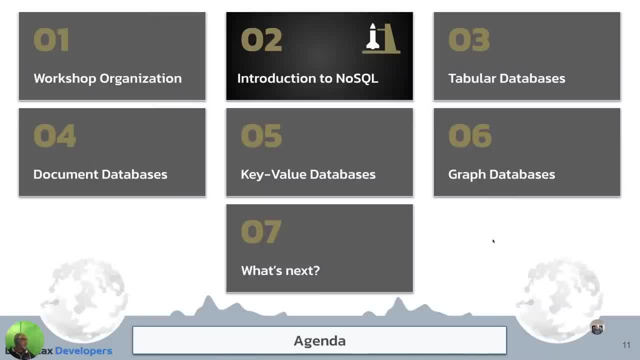 me move to. you're ready, Artem, to go? I'm me move to you're ready, Artem, to go? I'm, yes, I'm ready to go right. here's an yes, I'm ready to go right. here's an yes, I'm ready to go right. here's an original slide. you're good to go. 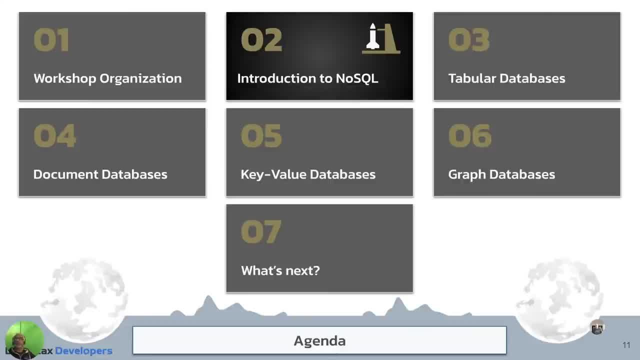 just let me know you're good to go. just let me know you're good to go. just let me know you're good to go. yeah, sure question. yes, so let's start. yeah, sure question. yes, so let's start. yeah, sure question. yes, so let's start talking about databases, right? no, SQL is. 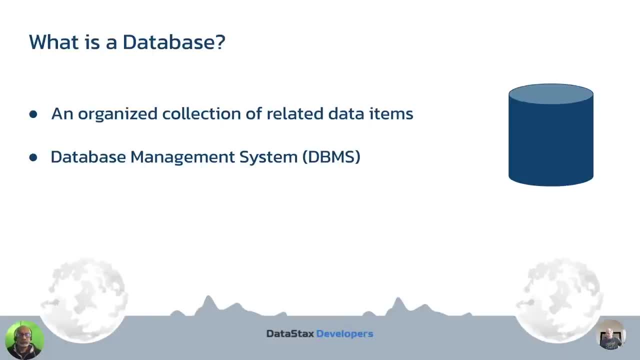 talking about databases, right? no, SQL is talking about databases, right? no, SQL is one type of database and it's good to one type of database and it's good to one type of database and it's good to have a well-defined, have a well-defined, have a well-defined notion of. 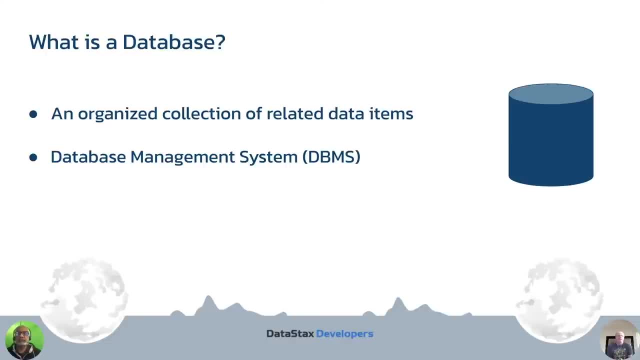 notion of notion of what database is right. because we're what database is right, because we're what database is right, because we're gonna talk about different types of, gonna talk about different types of gonna talk about different types of databases. so when we say database, we databases. so when we say database, we 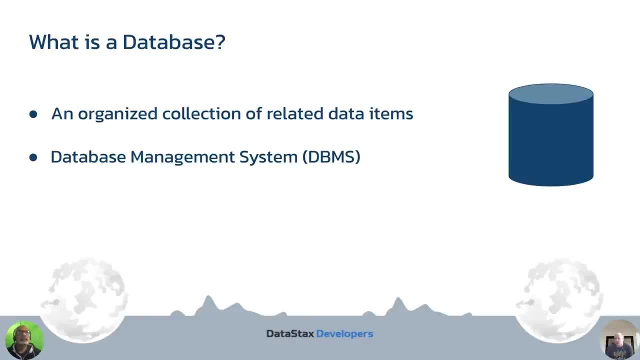 databases. so when we say database, we usually mean one of the two things. we usually mean one of the two things. we usually mean one of the two things. we mean organized collection of related data, mean organized collection of related data, mean organized collection of related data items, and it's important to understand. 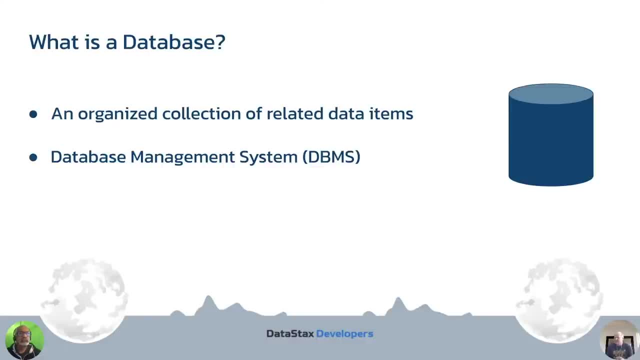 items and it's important to understand items and it's important to understand its organized collection. so there is its organized collection, so there is its organized collection. so there is some data modeling involved. you, you have some data modeling involved. you, you have some data modeling involved. you, you have to organize your data into tables, into 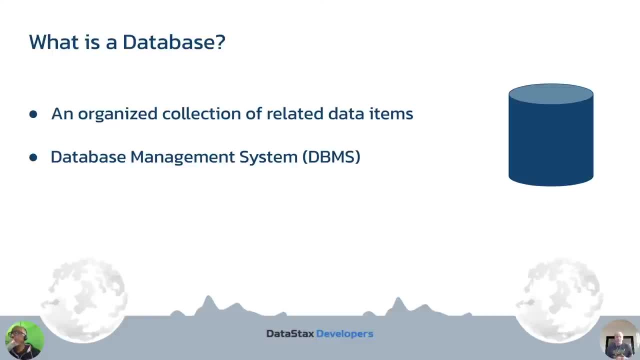 to organize your data into tables into. to organize your data into tables, into json documents, into a graph into key json documents, into a graph into key json documents, into a graph into key value pairs, something like that. but it's value pairs, something like that, but it's. 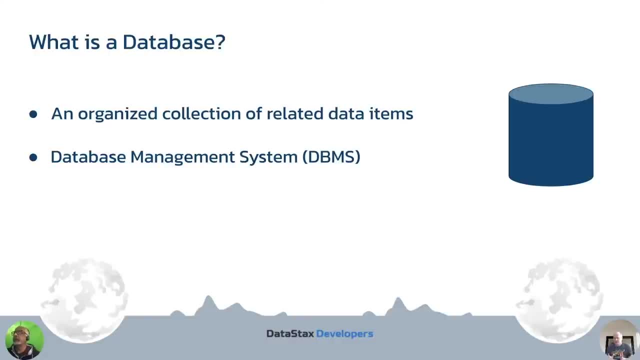 value pairs, something like that. but it's also the data is also related to some. also the data is also related to some. also the data is also related to some enterprise or some application and we enterprise or some application and we enterprise or some application, and we will actually talk about the difference. 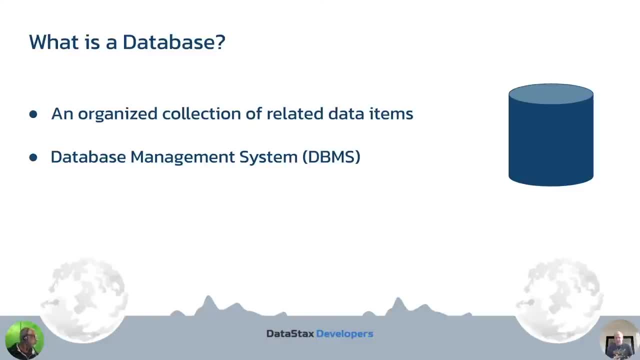 will actually talk about the difference, will actually talk about the difference between enterprise and application. I the between enterprise and application. I the between enterprise and application. I the why. what kind of databases? what's the why? what kind of databases? what's the why? what kind of databases? what's the difference between them? the other notion: 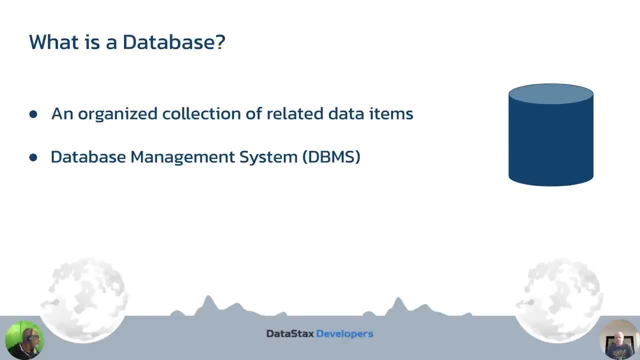 difference between them, the other notion, difference between them, the other notion of a database is when we refer to of a database, is when we refer to of a database, is when we refer to database management system and which is database management system and which is database management system and which is basically software that is able to. 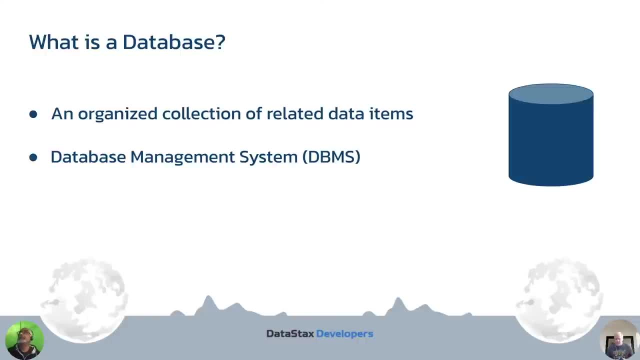 basically software that is able to, basically software that is able to create database, create that collection of create database, create that collection of create database. create that collection of data, manage it, store data, retrieve data data. manage it, store data, retrieve data data. manage it, store data, retrieve data. okay, so we will be using these terms. 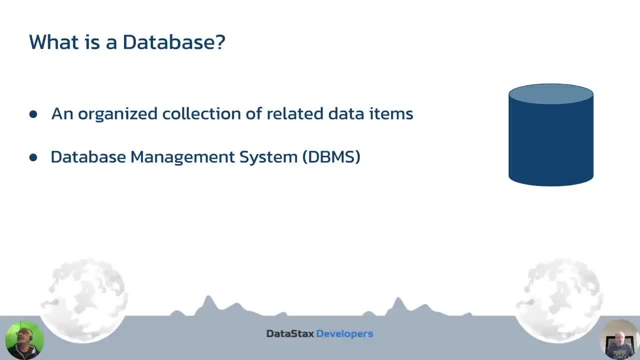 okay, so we will be using these terms. okay, so we will be using these terms kind of interchangeably, by hopefully from kind of interchangeably, by hopefully, from kind of interchangeably, by hopefully from the context will be easy to understand. the context will be easy to understand. 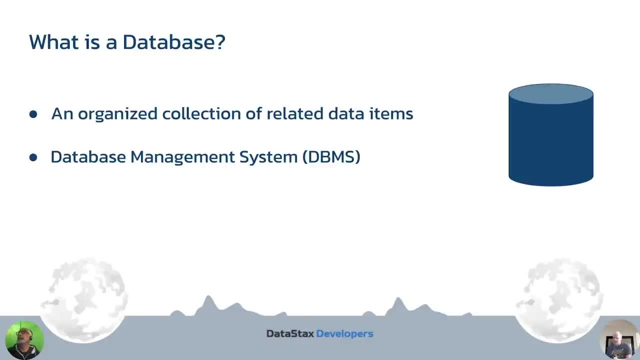 the context will be easy to understand. we'll be using Astra DB as which is no. we'll be using Astra DB as which is no. we'll be using Astra DB as which is no SQL database, but we will also create a SQL database, but we will also create a. 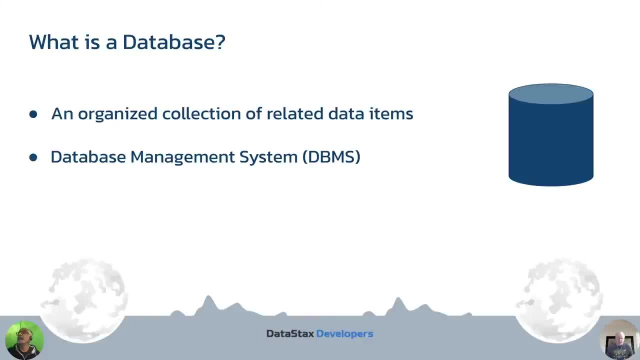 SQL database, but we will also create a database inside of Astra DB, which will be database inside of Astra DB, which will be database inside of Astra DB, which will be a collection of data. so give me a, a collection of data. so give me a. 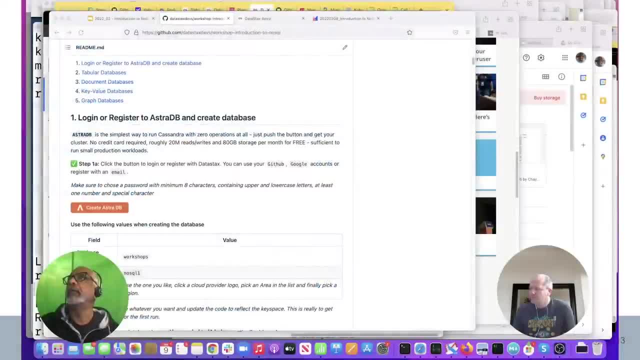 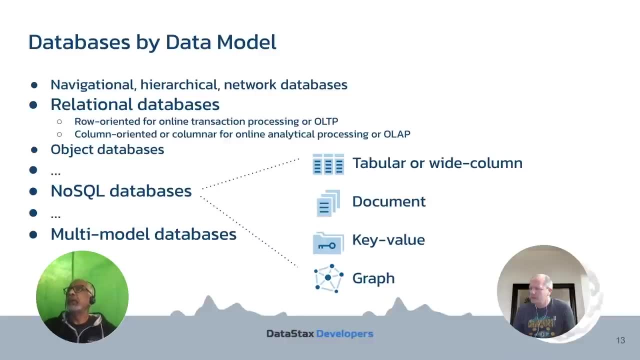 a collection of data. so give me a second. okay, so I will switch to full second. okay, so I will switch to full second. okay, so I will switch to full head. give me a second and make sure you head. give me a second and make sure you head. give me a second and make sure you have control. good to go, good, so when we 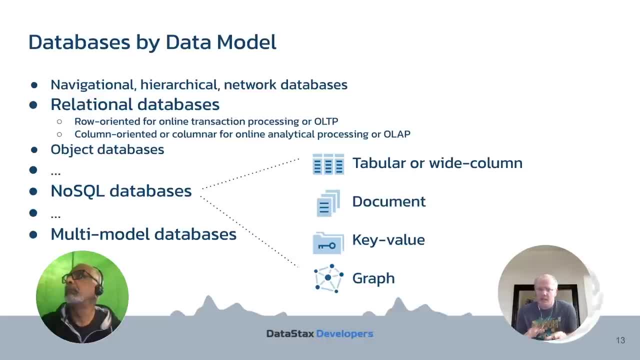 have control: good to go good. so when we have control, good to go good. so when we talk about databases, we usually classify, talk about databases. we usually classify, talk about databases. we usually classify them based on data model that they them based on data model, that they them based on data model that they support: okay, based on data model that. 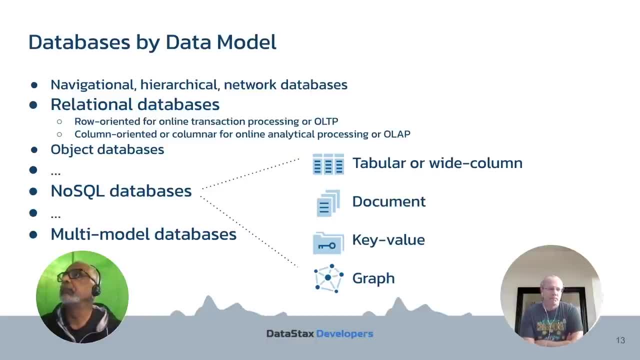 support: okay, based on data model that support- okay, based on data model that they support. and historically we have they support and historically we have they support and historically we have quite a few different data models. but I quite a few different data models, but I quite a few different data models, but I just listed here the main ones. so some 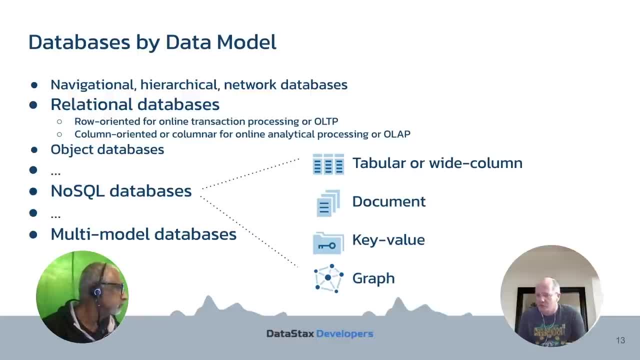 just listed here the main ones. so some just listed here the main ones. so some of the legacy systems were navigational of the legacy systems were navigational. of the legacy systems were navigational systems. they use hierarchical on network systems. they use hierarchical on network systems. they use hierarchical on network model and essentially a tree or graph. 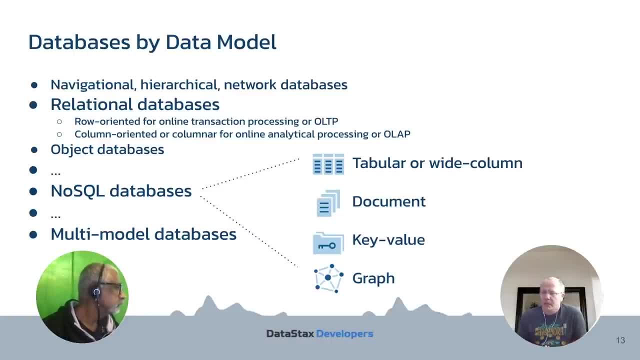 model and essentially a tree or graph model and essentially a tree or graph. but they were just the beginning of the but. they were just the beginning of the but. they were just the beginning of the of databases. they didn't have a good of databases, they didn't have a good. 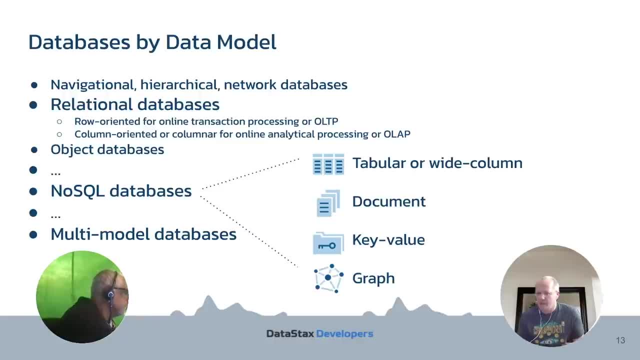 of databases. they didn't have a good query language. each time you have to query language, each time you have to query language, each time you have to retrieve data, you have to navigate that retrieve data. you have to navigate that retrieve data. you have to navigate that graph, literally write in code to: 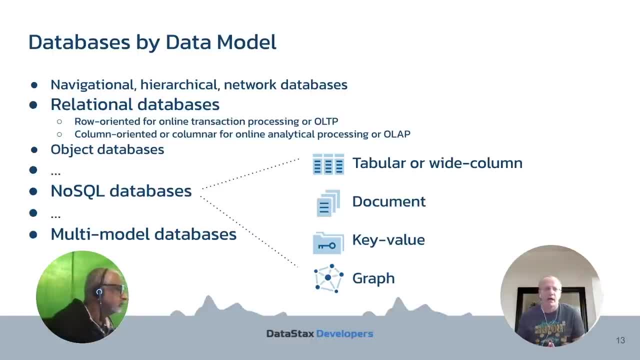 graph: literally write in code to graph: literally write in code to traverse the pointers, to find your traverse the pointers, to find your traverse, the pointers, to find your information. so they were not easy to use information, so they were not easy to use information, so they were not easy to use. then in 70s we had relational databases. 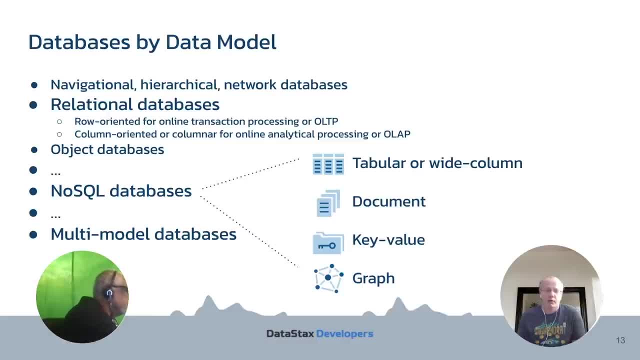 then in 70s we had relational databases. then in 70s we had relational databases, and they're still very useful now and and they're still very useful now and and they're still very useful now. and there are many, many different. there are many, many different. 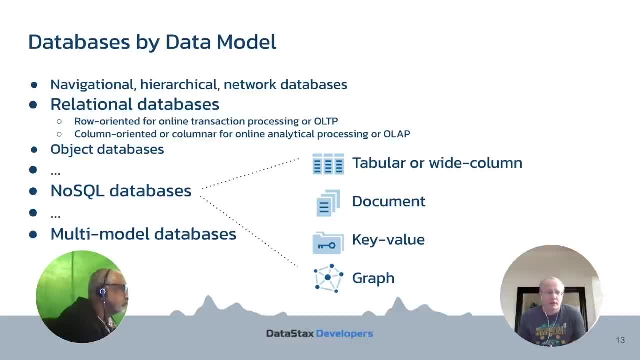 there are many, many different organizations and applications. that organizations and applications, that organizations and applications that that rely on relational databases, we that rely on relational databases, we that rely on relational databases, we will talk about, will talk about, will talk about many good advantages of relational, many good advantages of relational. 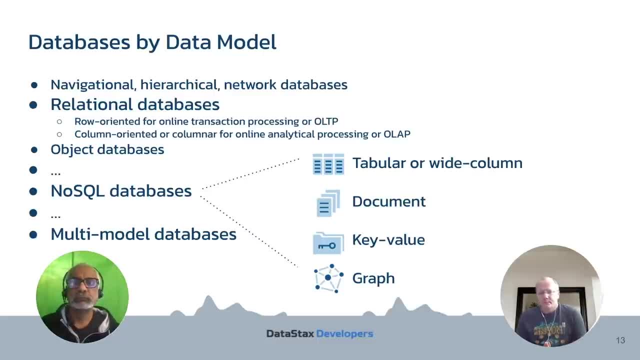 many good advantages of relational databases. then there was a movement for object databases. why movement for object databases? why movement for object databases? why object databases is basically to object databases, is basically to object databases, is basically to make it easier for an app for an. make it easier for an app for an. 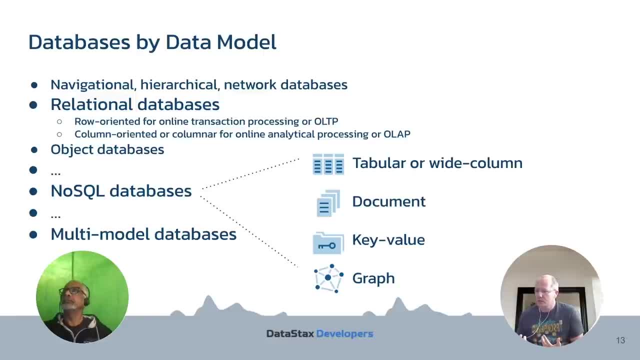 make it easier for an app for an application to application to application to application that manipulates data using application that manipulates data. using application that manipulates data using objects in memory to store those object objects in memory. to store those object objects in memory, to store those object right into database. unfortunately, the 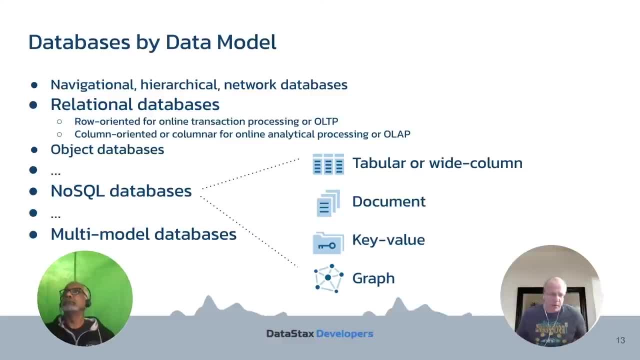 right into database. unfortunately, the right into database, unfortunately the object databases didn't become very object databases didn't become very object. databases didn't become very popular, but then there were a bunch of popular. but then there were a bunch of popular, but then there were a bunch of other types of databases like XML. 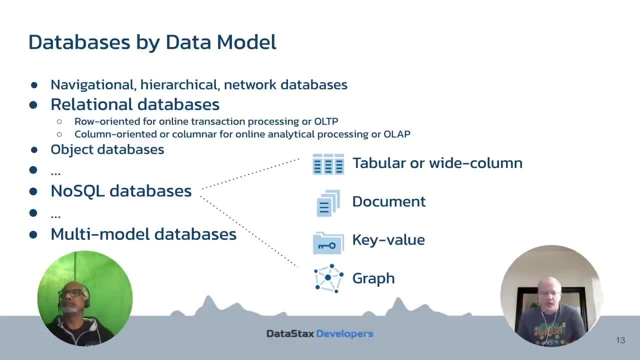 other types of databases like XML, other types of databases like XML. databases are the of databases, and then databases are the of databases, and then databases are the of databases. and then we had the movement of no SQL, no sequel. we had the movement of no SQL, no SQL. 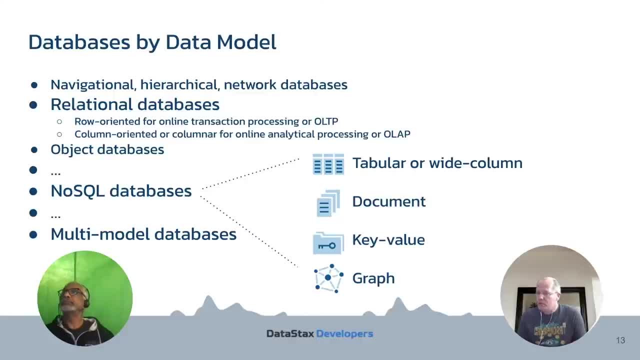 we had the movement of no SQL. no SQL databases: we will mostly focus on them. databases: we will mostly focus on them. databases: we will mostly focus on them and compare them with relational databases: we will mostly focus on them and compare them with relational databases. and we will focus on the four. 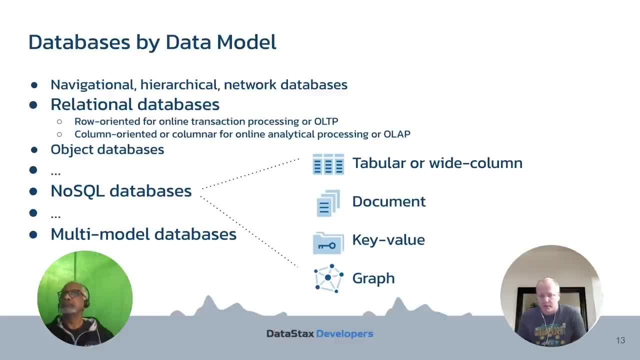 databases and we will focus on the four databases. and we will focus on the four different types of no SQL databases, which different types of no SQL databases, which different types of no SQL databases which include tabular which store data in. include tabular which store data in. 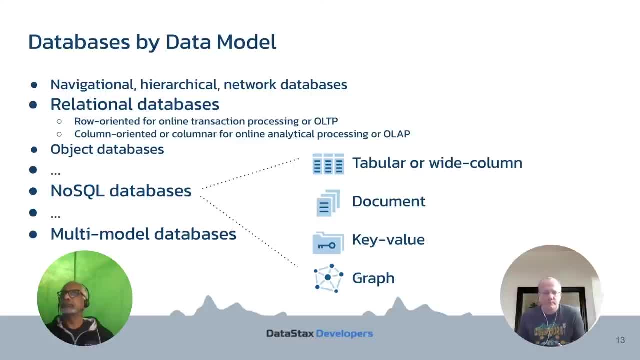 include tabular, which store data in tables just like relational. so if you tables just like relational, so if you tables just like relational, so if you familiar with relational, you will like familiar with relational. you will like familiar with relational, you will like tabular. no, no sequel databases there. 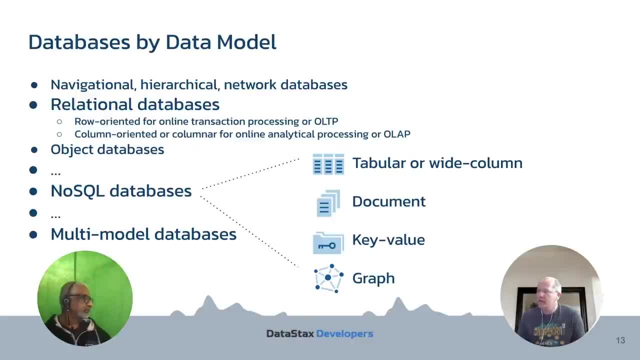 tabular: no, no sequel databases there. tabular- no, no, sequel databases there will be. we'll talk about document key will be. we'll talk about document key will be. we'll talk about document key. valor and grab as well, okay, and of valor and grab as well, okay, and of. 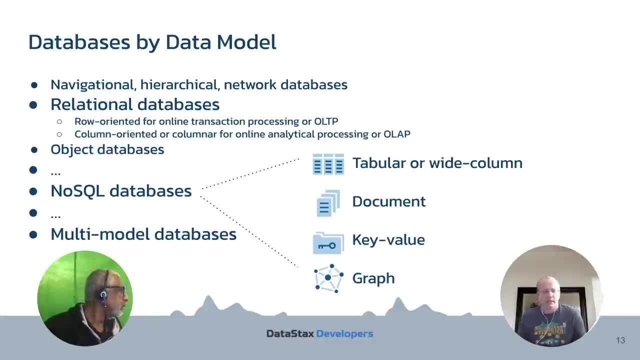 valor and grab as well. okay, and of course, nowadays, many databases support course. nowadays, many databases support course. nowadays, many databases support multiple data models, and that's true for multiple data models and that's true for multiple data models and that's true for no sequel, true for relational databases. 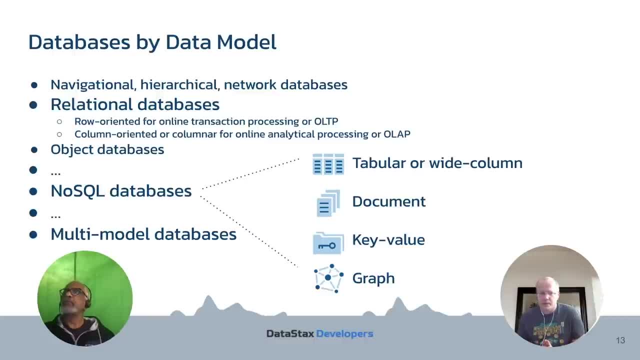 no sequel true for relational databases, no sequel true for relational databases as well. so the relational database may as well. so the relational database may as well. so the relational database may support a relational model, but also may support a relational model, but also may support a relational model, but also may support graph or XML or JSON. and 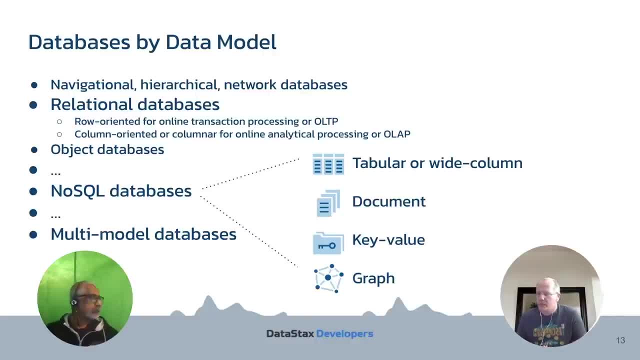 support graph or XML or JSON. and support graph or XML or JSON and similarly for no sequel databases. they similarly for no sequel databases. they similarly for no sequel databases. they more and add more and more features and more and add more and more features and more and add more and more features and they support all kinds of different. 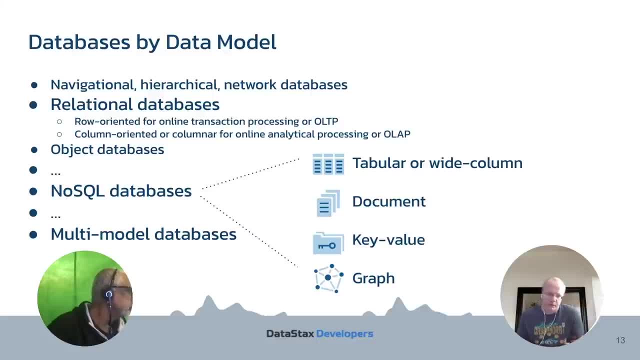 they support all kinds of different. they support all kinds of different capabilities that allow you to work with capabilities that allow you to work with capabilities that allow you to work with different models. so we are gonna use different models. so we are gonna use different models. so we are gonna use multi-model database today. so there is a. 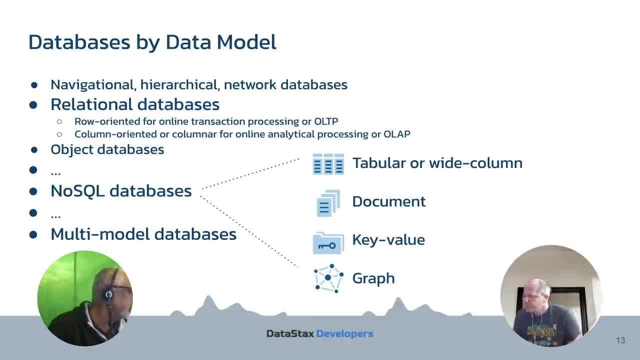 multi-model database today. so there is a multi-model database today, so there is a. so another is a question from Shri. so another is a question from Shri. so another is a question from Shri Kant, which is probably you know pretty Kant, which is probably you know pretty. 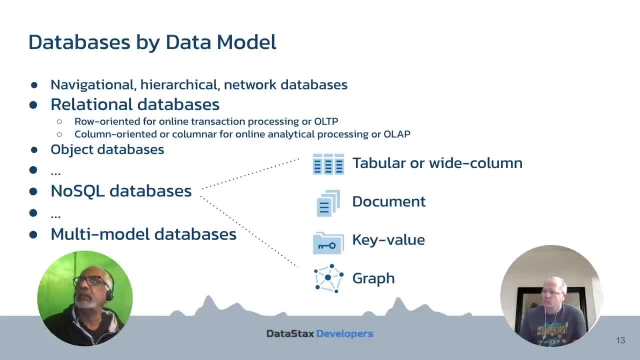 Kant, which is probably, you know, pretty appropriate, is object databases, like appropriate is object databases, like appropriate is object databases. like AWS s3. no, s3 is is basically object, AWS s3 is is basically object, AWS s3 is is basically object storage. so it's it's not really really a. 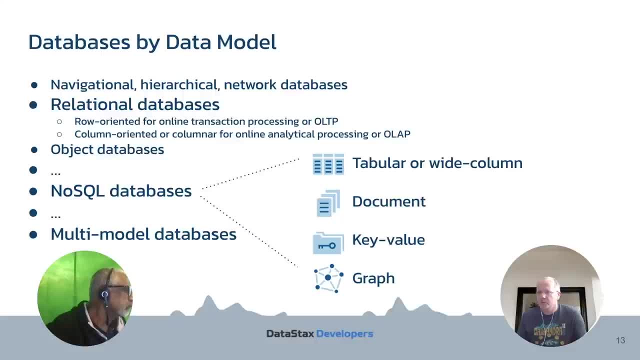 storage, so it's. it's not really really a storage so it's. it's not really really a database in in the sense that we think database in, in the sense that we think database in in the sense that we think about transactions, we think about query, about transactions, we think about query. 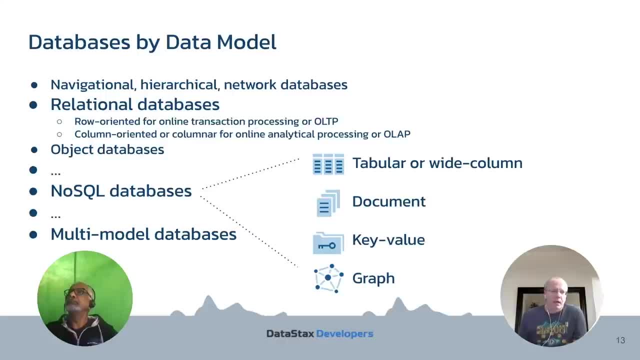 about transactions. we think about query language and things like that, so one language and things like that, so one language and things like that. so one more point here I wanted to make is for more point here I wanted to make is for more point here I wanted to make is for relational databases. I also have these. 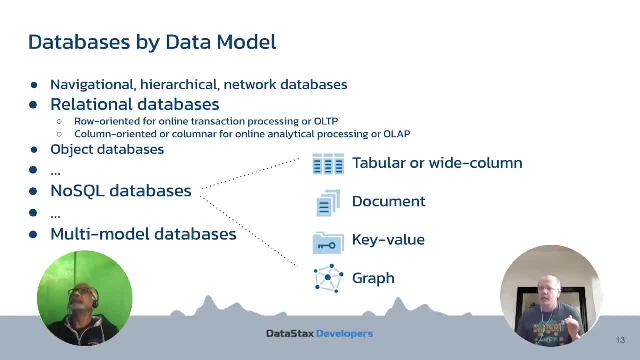 relational databases. I also have these relational databases. I also have these two bullets for row, oriented and column, two bullets for row, oriented and column. two bullets for row, oriented and column, oriented or columnar. so essentially, this oriented or columnar, so essentially this oriented or columnar. so essentially this will be. this will be true for any. 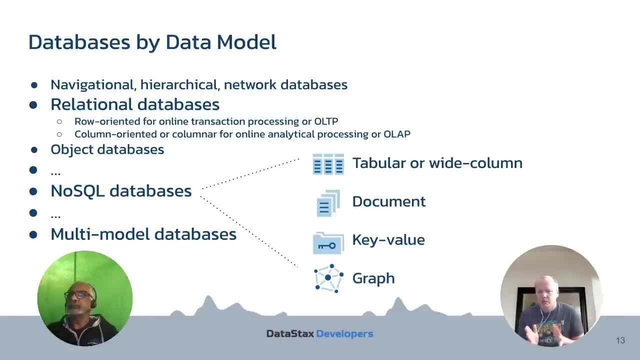 will be. this will be true for any will be. this will be true for any tabular databases. so, for example, most tabular databases. so, for example, most tabular databases. so, for example, most equal tabular databases. they also have equal tabular databases. they also have. 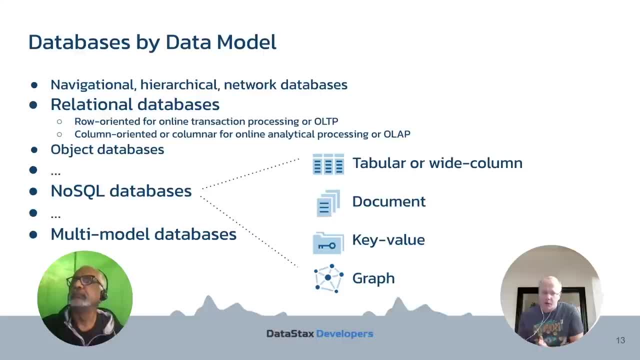 equal tabular databases. they also have rows and columns and they can be row, rows and columns, and they can be row, rows and columns, and they can be row, oriented or column, and essentially this oriented or column and essentially this oriented or column, and essentially this is a storage model, how database stores. 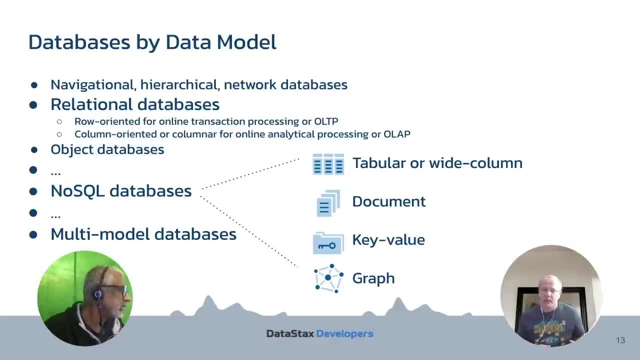 is a storage model how database stores is a storage model how database stores those rows and columns. you can. if it those rows and columns you can. if it those rows and columns you can. if it stores all the data in a row together. stores all the data in a row together. 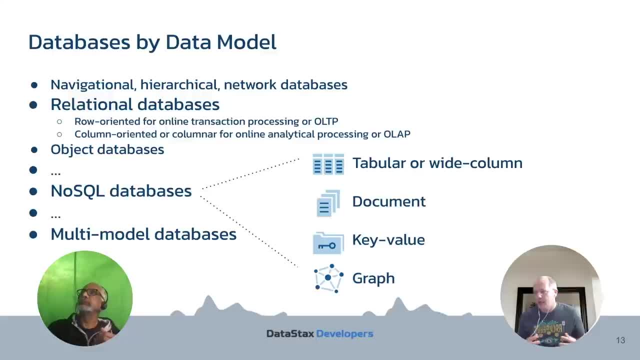 stores all the data in a row together, then it's that, then it is row oriented, then it's that, then it is row oriented, then it's that, then it is row oriented database, and it's great for real-time database and it's great for real-time. 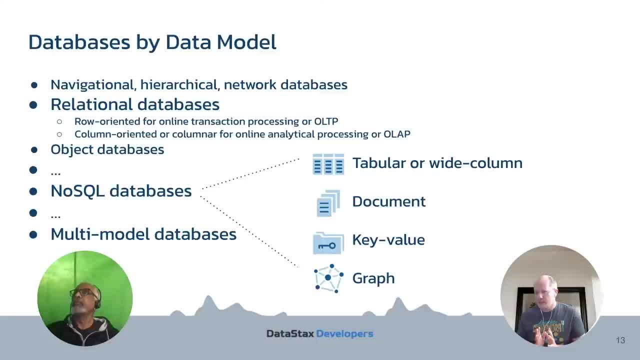 database and it's great for real-time uh transaction processing. so it's it's uh transaction processing. so it's it's uh transaction processing. so it's it's it's uh called OLTP type of system and uh called OLTP type of system and uh called OLTP type of system and we're going to use OLTP. 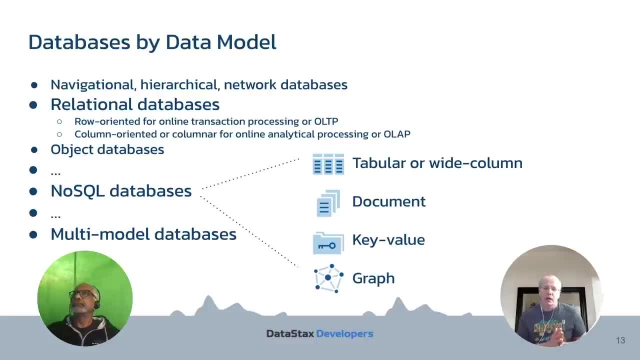 we're going to use OLTP. we're going to use OLTP database today, but also column oriented database today, but also column oriented database today, but also column oriented or columnar, they or columnar, they or columnar. they basically store all, basically store all, basically store all failures in a column from different rows. 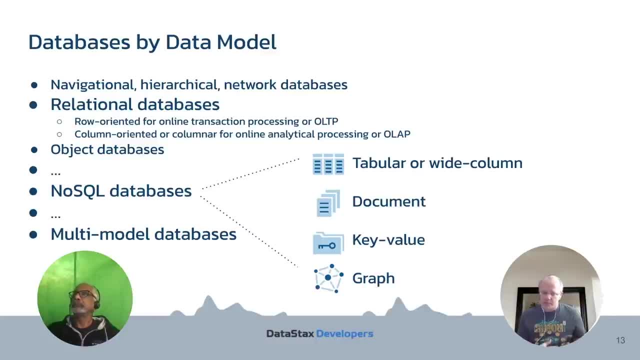 failures in a column from different rows, failures in a column from different rows together, together, together, so that they can be retrieved together, so that they can be retrieved together, and um analyzed quickly, and these are and um analyzed quickly, and these are and um analyzed quickly, and these are all app systems usually. 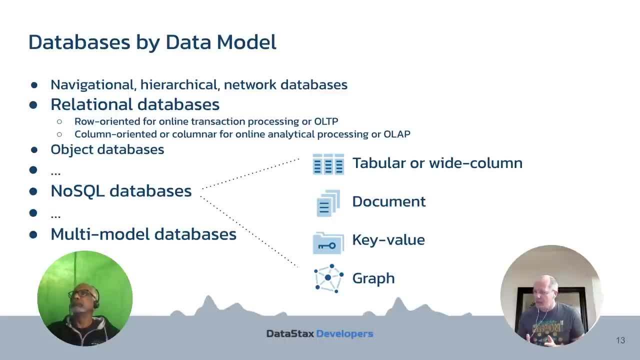 all app systems, usually all app systems usually. so they are for analytical processing. so they are for analytical processing, so they are for analytical processing. they, they, they, they, they, they, they have slow response, but they usually have slow response, but they usually have slow response, but they usually process more. 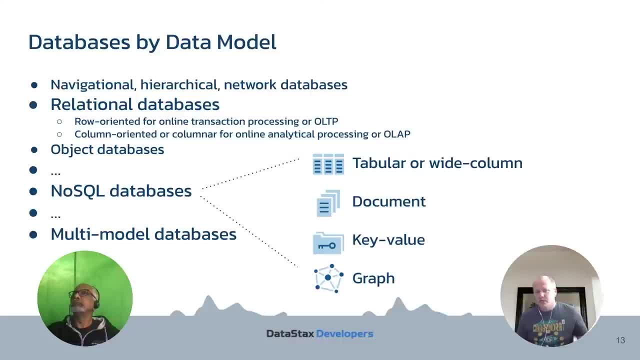 process, more process, more data. and besides relational databases, data and besides relational databases, data and besides relational databases, there are some more sql databases, that there are some more sql databases, that there are some more sql databases that are that are column oriented. there are. are that are column oriented, there are. 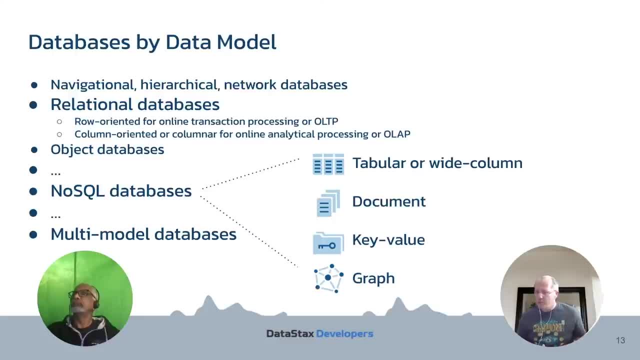 are that are column oriented. there are also also also um data: where how modern data, um data, where how modern data, um data, where how modern data warehouses? they are column oriented like warehouses. they are column oriented like warehouses. they are column oriented like big video and slow. big video and slow. 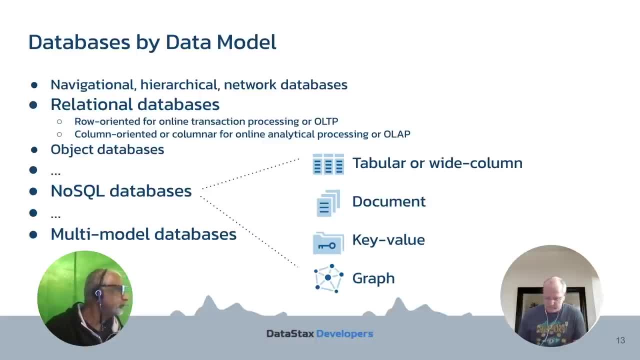 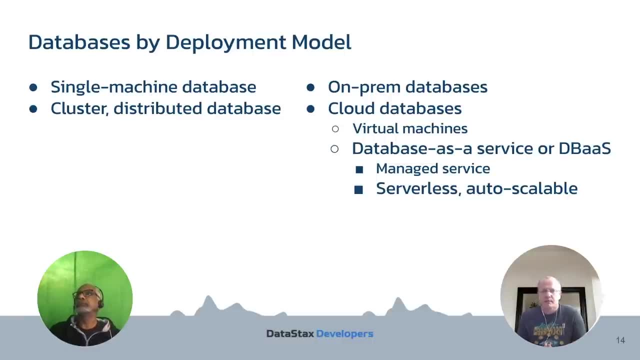 big video and slow snowflake, okay. snowflake okay, snowflake, okay. so by deployment model, we can. so by deployment model, we can. so by deployment model, we can differentiate, differentiate, differentiate uh these types of databases, uh single. uh these types of databases, uh single. uh these types of databases, uh, single machine databases. 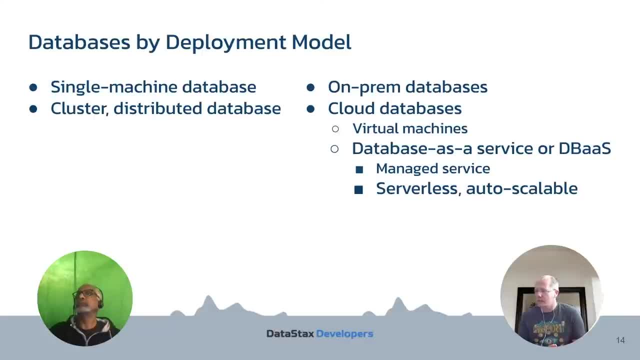 machine databases, machine databases and databases that works on clusters and databases that works on clusters and databases that works on clusters. and these are distributed and these are distributed and these are distributed databases, databases, databases, so they uh partition data, so they uh partition data. so they uh partition data and and store on different nodes with 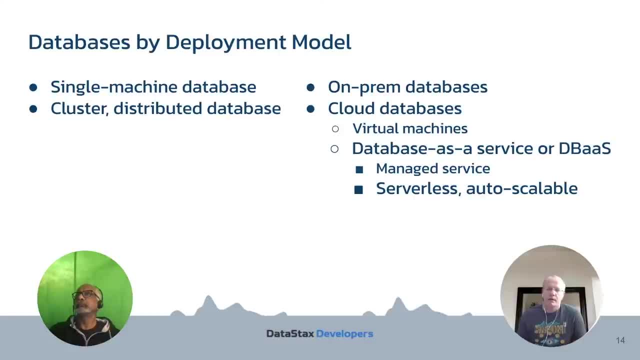 and and. store on different nodes with and and. store on different nodes with replication, replication, replication, and. and uh, uh, they. there can be multiple and and uh, uh, they. there can be multiple and and uh, uh, they. there can be multiple. data centers that are data centers that are. 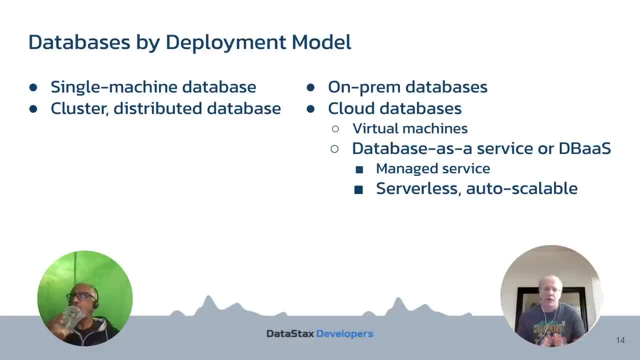 data centers that are distributed uh geographically. they can distributed uh geographically. they can distributed uh geographically. they can live in different, live in different, live in different locations. so which is good for locations, so which is good for locations, so which is good for reliability and availability. 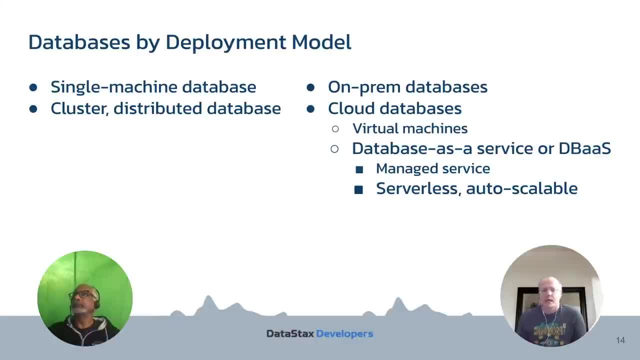 reliability and availability. reliability and availability: also. databases can be run on premises also. databases can be run on premises also. databases can be run on premises and they can be in cloud. so nowadays, we and they can be in cloud. so nowadays, we and they can be in cloud. so nowadays we have. 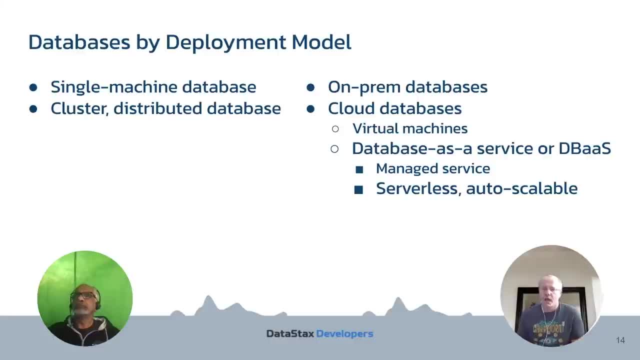 have have more and more push towards cloud, more and more push towards cloud, more and more push towards cloud. a lot of migration and in the cloud you a lot of migration and in the cloud you a lot of migration. and in the cloud you can use either just virtual machine, you. 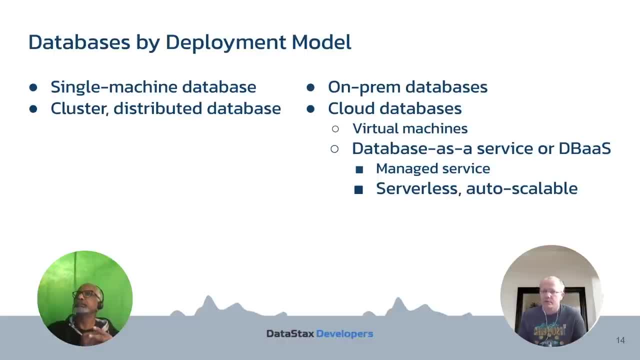 can use either just virtual machine. you can use either just virtual machine. you install your database software, install your database software, install your database software and you, you're responsible for managing, and you, you're responsible for managing, and you, you're responsible for managing that, that, that or 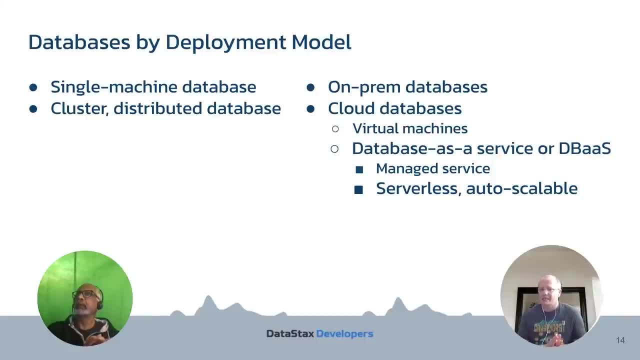 or or another another. another kind of deployment is database as a kind of deployment. is database as a kind of deployment is database as a service, service, service, where, where, where the database is already pre-installed for, the database is already pre-installed for, the database is already pre-installed for you, it already runs, already configured. 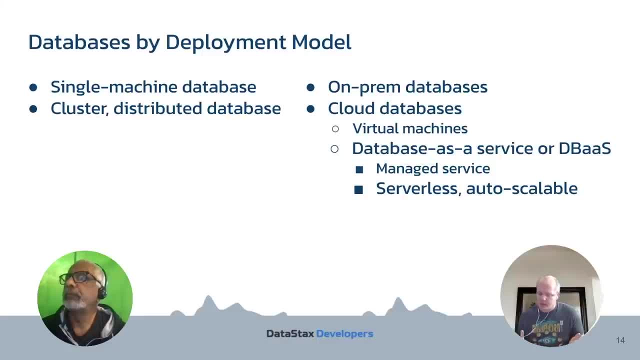 you it already runs, already configured. you, it already runs, already configured, and and you just and, and you just and and you just. there are two types of those services. there are two types of those services. there are two types of those services: managed service, where you. managed service where you. 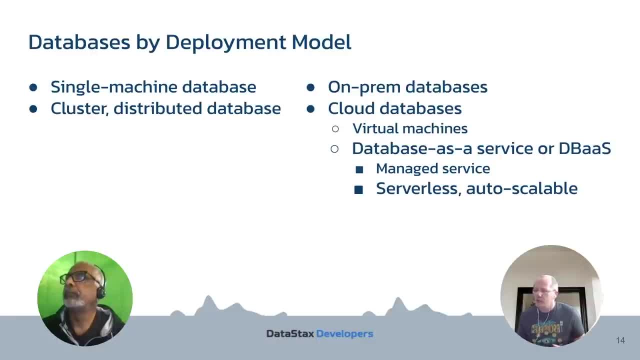 managed service where you basically specify how many nodes, basically specify how many nodes, basically specify how many nodes you you want to have, you, you want to have, you, you want to have in in that database cluster, in in that database cluster, in in that database cluster, and and basically 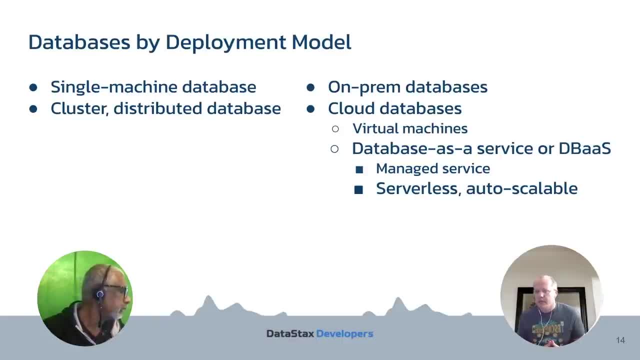 and, and, basically, and, and basically, you, you go with that number and you can, you, you go with that number and you can, you, you go with that number and you can later maybe increase it manually or later, maybe increase it manually or later maybe increase it manually or decrease it manually. 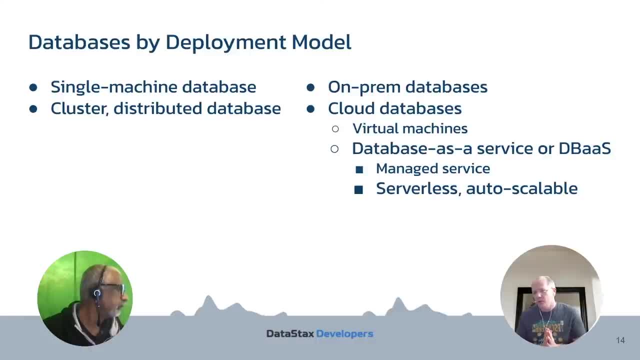 decrease it manually, decrease it manually. but the best type of those database of, but the best type of those database of, but the best type of those database of other service, that other service, that other service, that offerings are serverless and out of, offerings are serverless and out of. 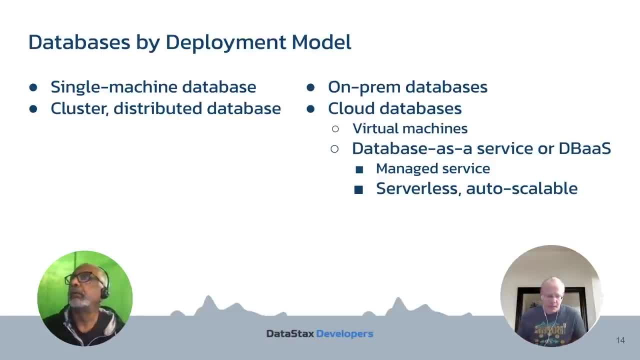 offerings are serverless and out of scalable, scalable, scalable database services. where database services, where database services where you do not really worry about how many, you do not really worry about how many, you do not really worry about how many instances you will use how many notes instances you will use how many notes. 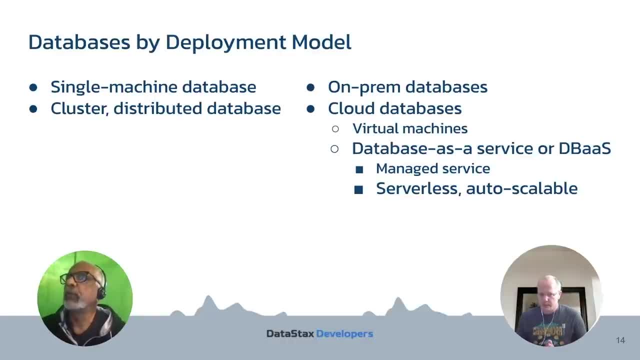 instances you will use how many notes you will need in the cluster. you will need in the cluster, you will need in the cluster. so the system, the service takes care of. so the system, the service takes care of. so the system, the service takes care of that. and if the number of transactions 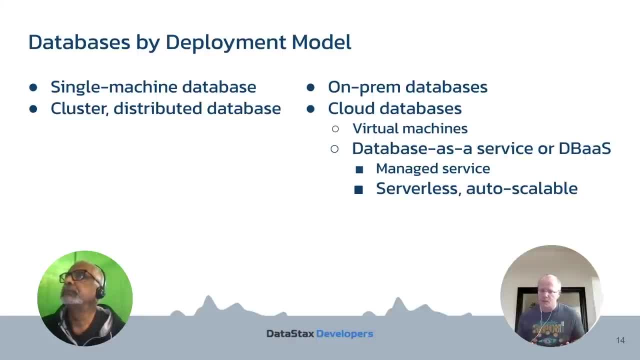 that and if the number of transactions that and if the number of transactions, the throughput, increases, the throughput increases, the throughput increases, the service will. the service will, the service will add nodes to that cluster automatically. add nodes to that cluster automatically. add nodes to that cluster automatically. when the, the, the workload decreases, then 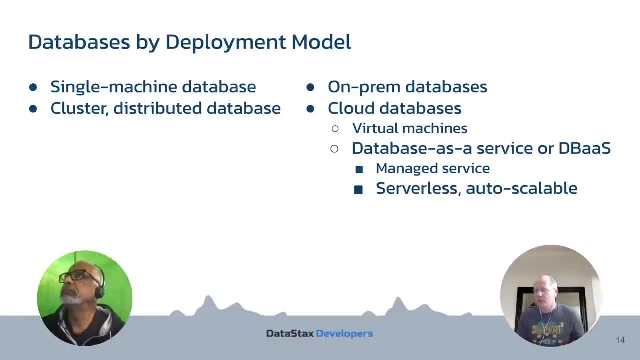 when the the the workload decreases, then when the the the workload decreases, then the the number of nodes decreases as well. the the number of nodes decreases as well, the the number of nodes decreases as well. automatically and essentially automatically and essentially automatically and essentially, you do the least amount of management. 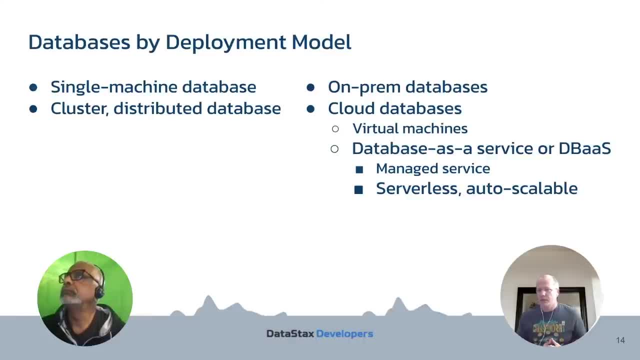 you do the least amount of management, you do the least amount of management, operations, operations, operations- with this service and you actually pay with this service and you actually pay with this service and you actually pay less, less, less for doing less, for working less because, for doing less for working less because. 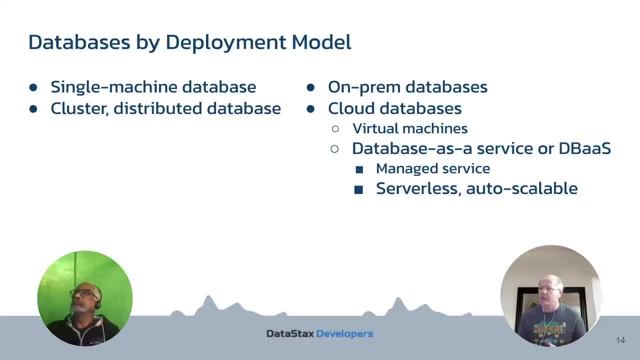 for doing less, for working less, because you're paying less, because you're paying less, because you're paying less, because it's out of scalable if, if you don't have, it's out of scalable if, if you don't have, it's out of scalable if, if you don't have a lot of 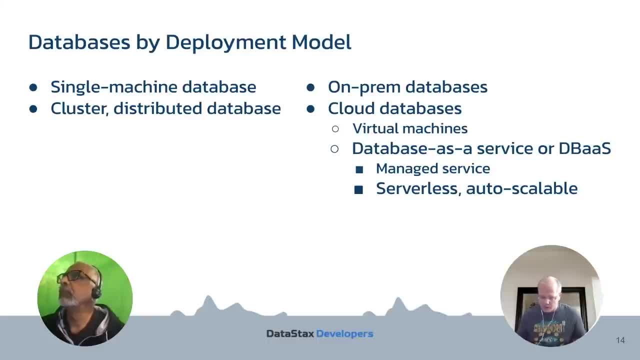 a lot of, a lot of faster it will be scaled down to 10. faster it will be scaled down to 10. faster it will be scaled down to 10 nodes, for example, nodes, for example, nodes, for example. okay, is it worth noting here that? okay, is it worth noting here that? 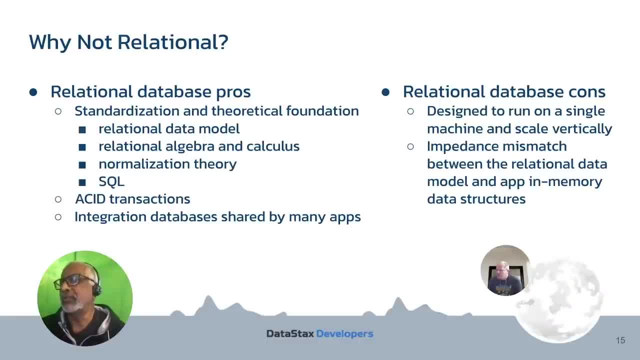 okay. is it worth noting here that you know data on the cloud is still? you know data on the cloud is still. you know data on the cloud is still relatively new. you know i'm not saying relatively new. you know i'm not saying relatively new. you know i'm not saying that, you know. 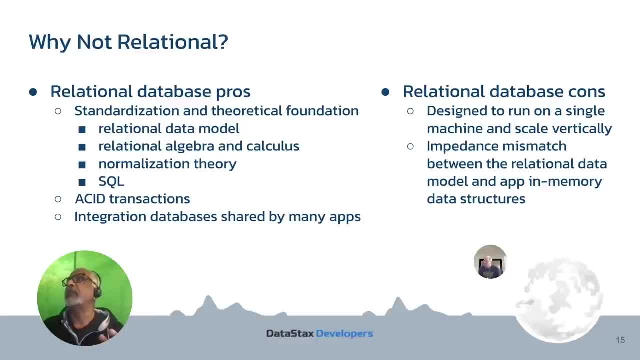 that. you know that. you know it's it's it's brand new, uh, but you it's, it's it's brand new, uh, but you it's, it's it's brand new, uh. but you know i, i come from the cloud foundry side. know i, i come from the cloud foundry side. 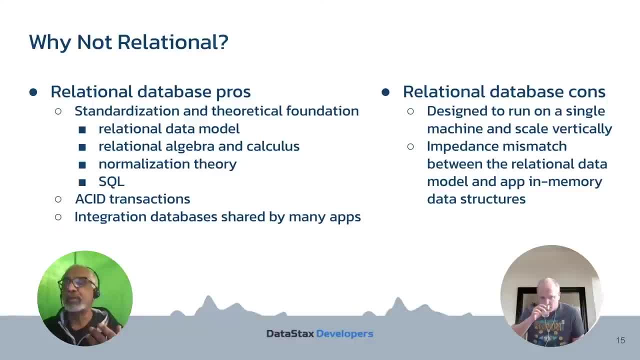 know i, i come from the cloud foundry side of the world, of the world, of the world, um, and and essentially, uh, what happens, um, and and essentially, uh, what happens um, and and essentially, uh, what happens. uh, there is, you know it's really more. uh, there is, you know, it's really more. 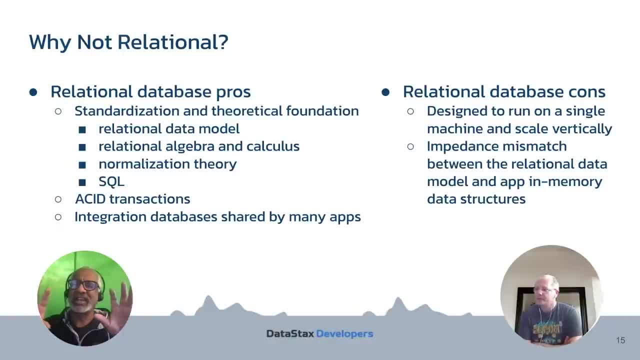 uh, there is. you know it's really more about 12-factor apps, about 12-factor apps, about 12-factor apps where you know it's more about state, where you know it's more about state, where you know it's more about state less. but stateful apps are relatively. 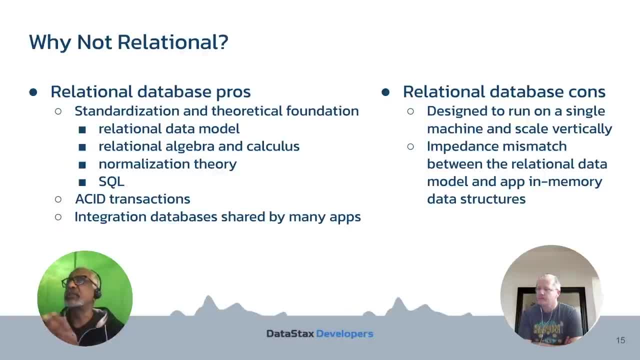 less, but stateful apps are relatively less, but stateful apps are relatively new. new, new, um you know, and in the last like uh five um you know, and in the last like uh five um you know, and in the last like uh five or six years. and 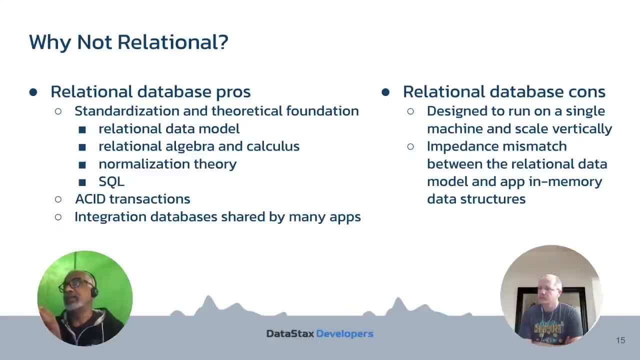 or six years and or six years and, and managing them is a little bit you and managing them is a little bit you and managing them is a little bit you. know is is a little bit different, as know is is a little bit different, as know is is a little bit different as compared to. 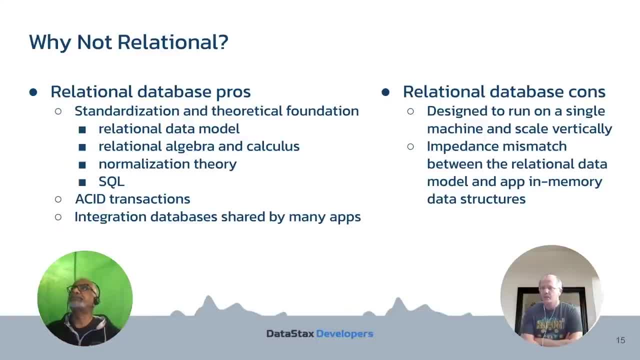 compared to, compared to. you know like uh, stateless. so you know you know like uh stateless. so you know, you know like uh, stateless. so you know, stateless, stateless, stateless. yes indeed, and and we're gonna actually, yes, indeed, and and we're gonna actually. 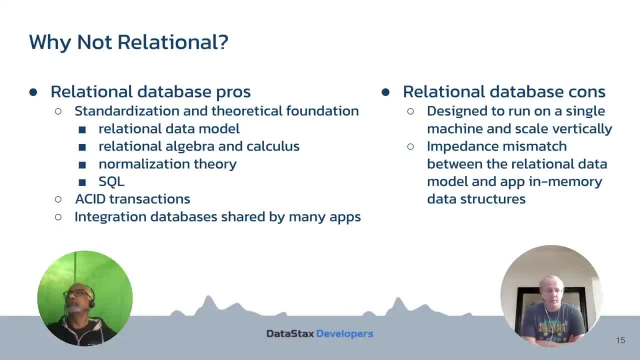 yes, indeed, and, and we're gonna actually use a cutting edge, use a cutting edge, use a cutting edge database. uh- serverless database today database. uh- serverless database today database. uh, serverless database today. uh, in many aspects it's a unique. uh, in many aspects it's a unique. 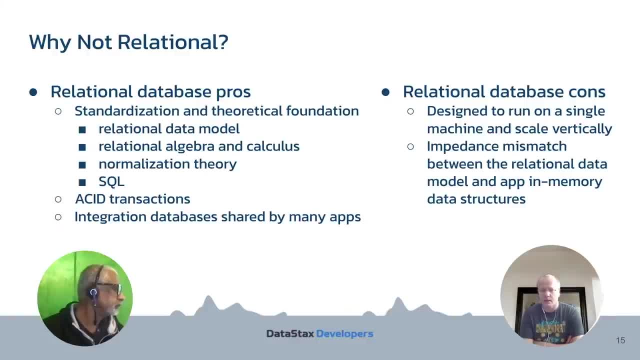 uh, in many aspects it's a unique serverless database, serverless database, serverless database. there are no other databases, that there are no other databases, that there are no other databases that have the same, have the same, have the same characteristics, characteristics, characteristics. okay, so why? okay, so why? 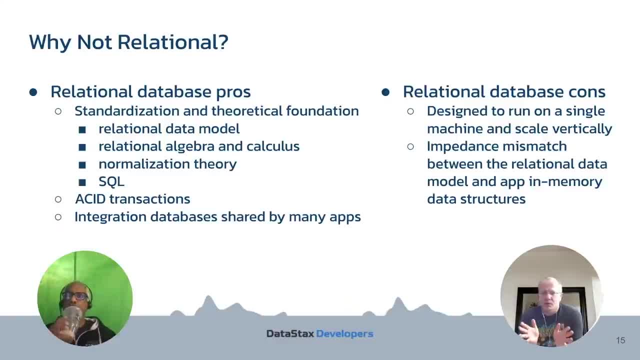 okay, so why not relate? why not? uh? so let's, let's talk, not relate. why not? uh? so, let's, let's talk, not relate. why not? uh? so let's, let's talk about just understand the benefits of, about just understand the benefits of, about just understand the benefits of relationals and and. 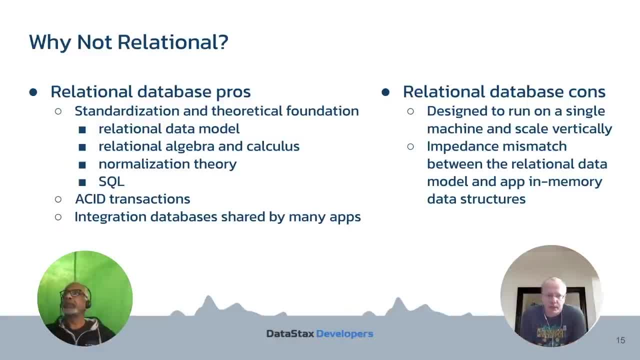 relationals and, and relationals and, and the problems that may exist with, with the problems that may exist with, with the problems that may exist with with relational databases, relational databases, relational databases: so what we like about relational, so what we like about relational, so what we like about relational databases, and that's why they became so. 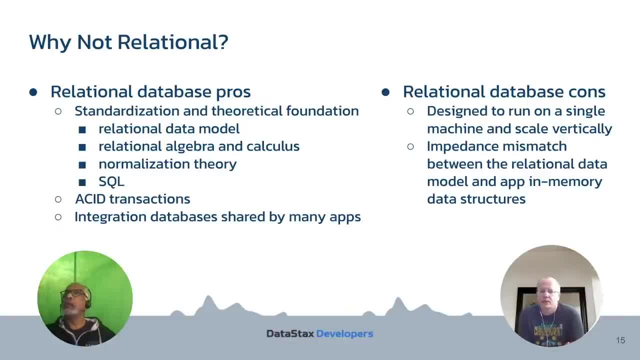 databases and that's why they became so databases and that's why they became so so popular is standard standardization. so popular is standard standardization. so popular is standard standardization. and and theoretical and and theoretical and and theoretical- very solid theoretical foundation right. very solid theoretical foundation right. 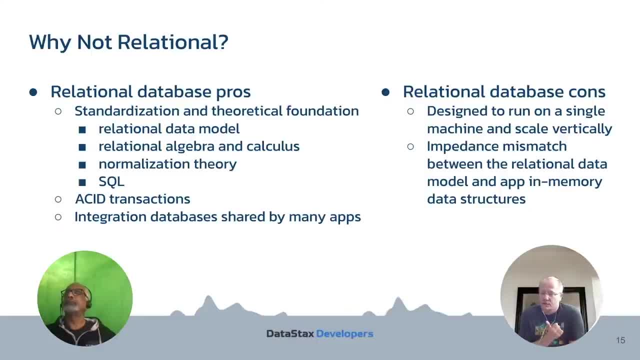 very solid theoretical foundation. right, there is a relational data model. there is a relational data model. there is a relational data model. there is relational algebra and calculus. there is relational algebra and calculus. there is relational algebra and calculus. when we usually don't care about that, when we usually don't care about that. 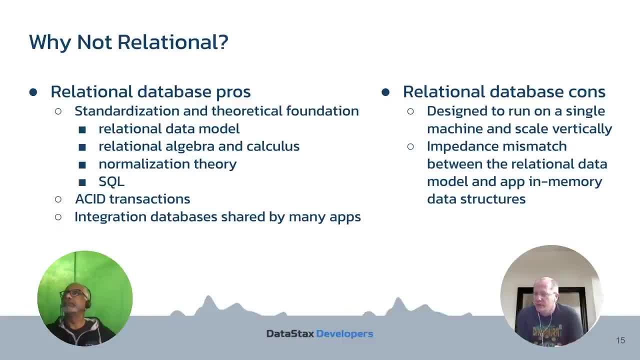 when we usually don't care about that. but people who, but people who, but people who write, uh, do do query optimizations, write, write, uh, do do query optimizations, write, write, uh, do do query optimizations, write those optimizers, they do those optimizers, they do those optimizers. they do care about those things, definitely uh. 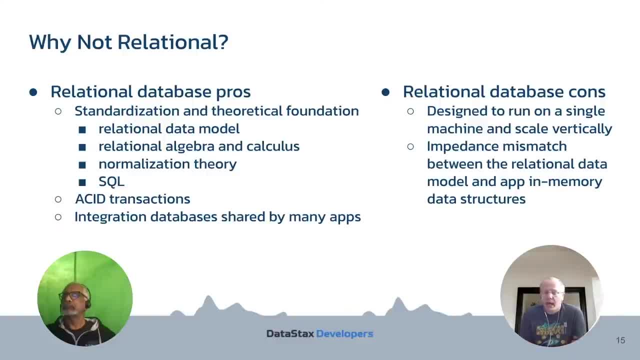 care about those things. definitely, uh, care about those things. definitely, uh, because that's because that's because that's that's what they work with, and even some that's what they work with, and even some that's what they work with, and even some. no sql databases and big data framework. 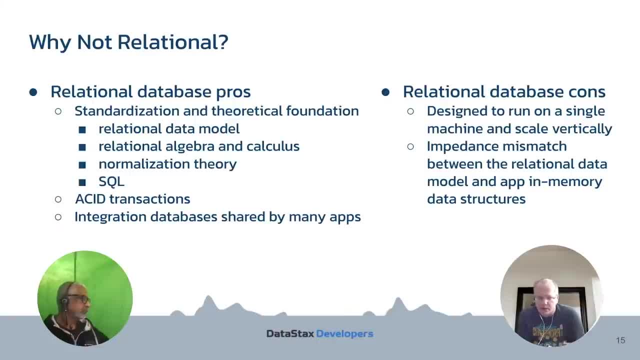 no sql databases and big data framework. no sql databases and big data framework. big data processing framework like spark. big data processing framework like spark. big data processing framework like spark. they also rely on things like relational. they also rely on things like relational. they also rely on things like relational algebra to. 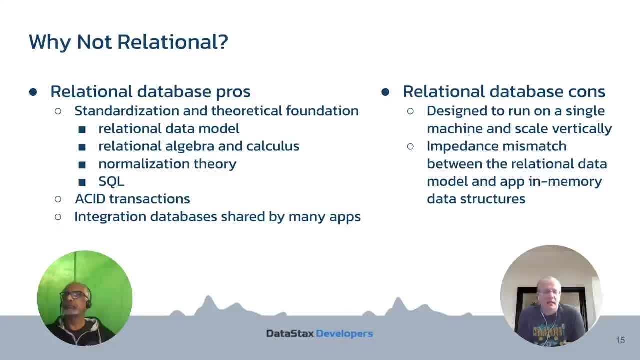 algebra to algebra, to. to optimize, to optimize, to optimize, the. the execution of those sparks, the. the execution of those sparks, the the execution of those sparks. okay, um, also there is normalization. okay, um, also there is normalization. okay, um, also there is normalization. series, we will, series, we will. 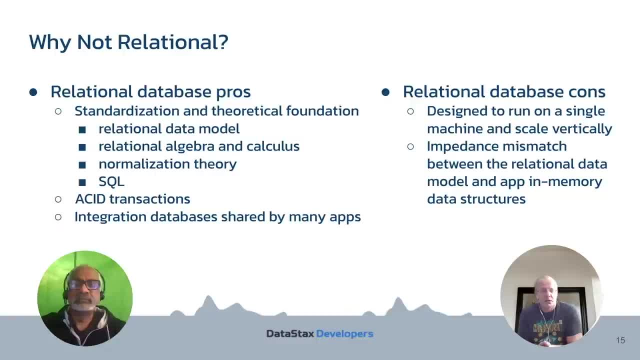 series. we will mention that normalization, mention that normalization, mention that normalization. denormalization a couple of times today. denormalization a couple of times today. denormalization a couple of times today. and there is a and there is a and there is a structured query language- sql- that we all 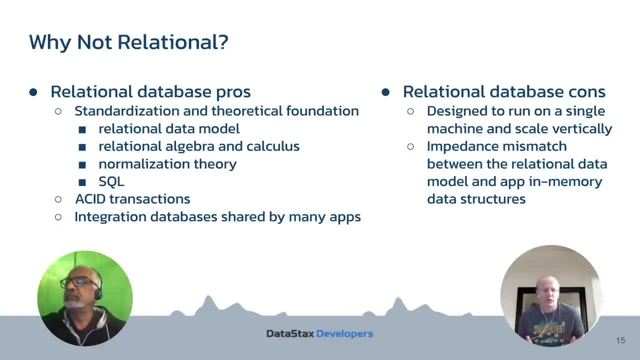 structured query language sql, that we all structured query language sql, that we all heard about it, some of us heard about it, some of us heard about it, some of us use it and know and it's and still use it and know and it's, and still use it and know and it's, and still there are many, many 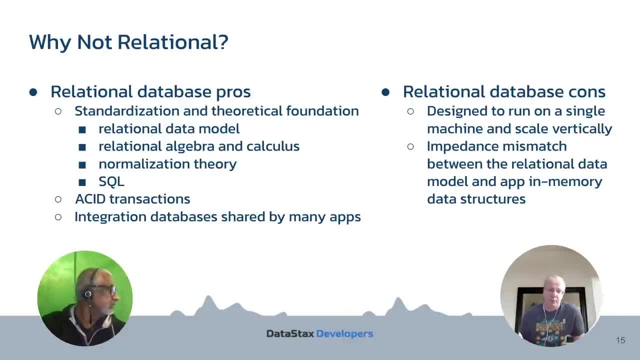 there are many, many. there are many, many applications and use cases where we will applications and use cases, where we will applications and use cases where we will prefer sql to prefer sql, to prefer sql to no sql, then there are also acid. no sql, then there are also acid. 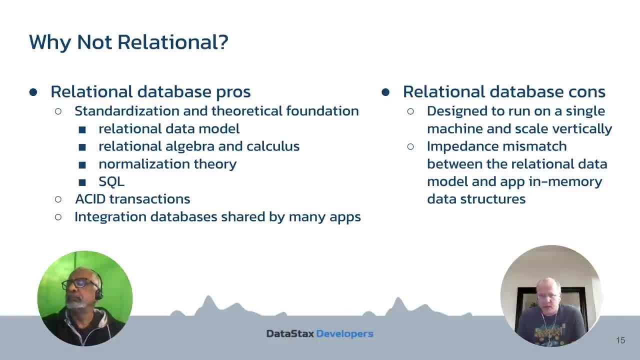 no sql. then there are also acid transactions, that transactions, that transactions that allow us to have atomic consistent allow us to have atomic consistent, allow us to have atomic consistent, isolated and durable transactions, isolated and durable transactions, isolated and durable transactions. but they kind of expensive, right, but they kind of expensive right. 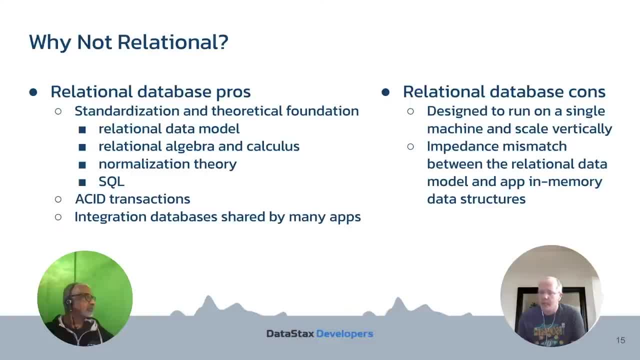 but they kind of expensive right to use, if you, especially if you have to use, if you especially if you have to use, if you, especially if you have many, many, many concurrent transactions, many, many, many concurrent transactions, many, many, many concurrent transactions, and also relational databases are, and also relational databases are. 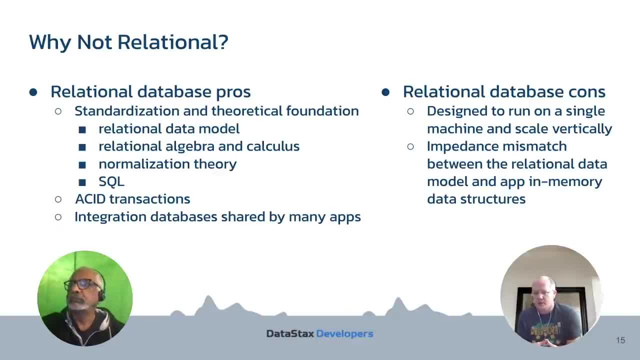 and also relational databases, are usually used as integration databases, usually used as integration databases, usually used as integration databases, shared by many, shared by many, shared by many applications. so, in other words, you have applications, so, in other words, you have applications. so, in other words, you have the single source of truth, you normalize. 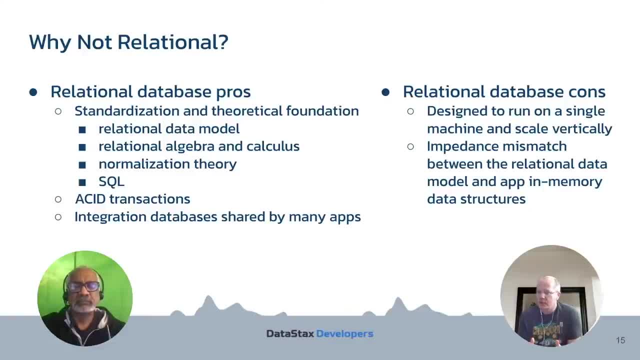 the single source of truth. you normalize the single source of truth. you normalize your tables, your tables, your tables. you store data once you do not duplicate. you store data once you do not duplicate it and many applications access use that it and many applications access use that it and many applications access use that database. 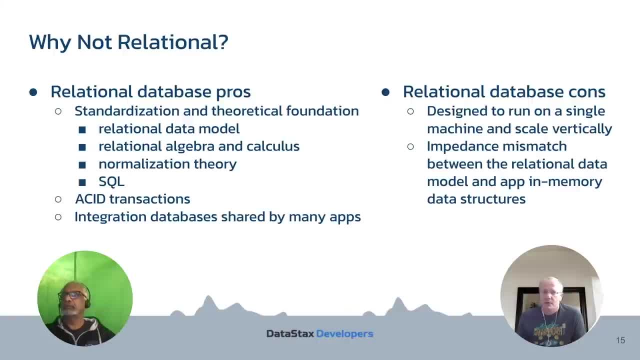 database database. okay, that's how relational are usually. okay, that's how relational are usually okay, that's how relational are usually modeled and used, modeled and used, modeled and used. then the cons would be, then the cons would be, then the cons would be that relational databases originally. 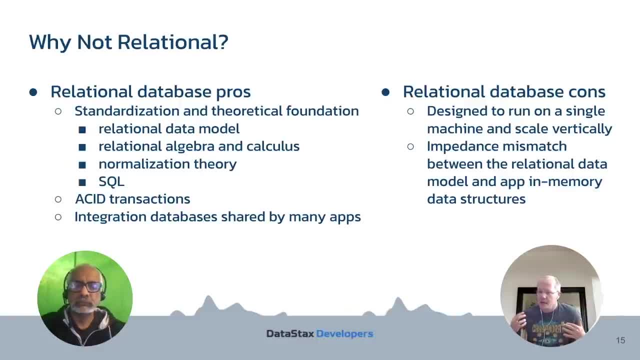 that relational databases originally, that relational databases originally designed for a single machine and they designed for a single machine and they designed for a single machine and they, they scale vertically, basically, they scale vertically, basically, they scale vertically, basically increasing the number of resources amount, increasing the number of resources amount. 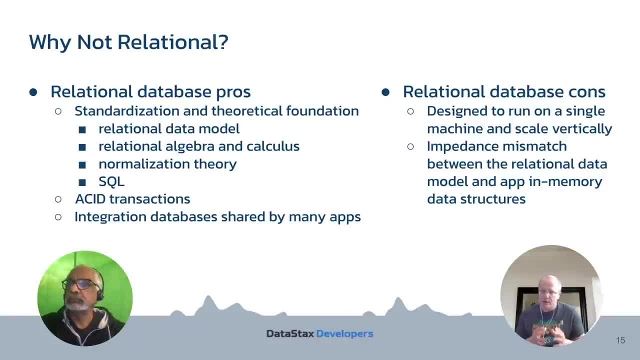 increasing the number of resources, amount of resources, of resources, of resources on one single server and on one single server and on one single server. and at that time that was at that time, that was at that time that was, uh, pretty good, but things have changed. uh, pretty good, but things have changed. 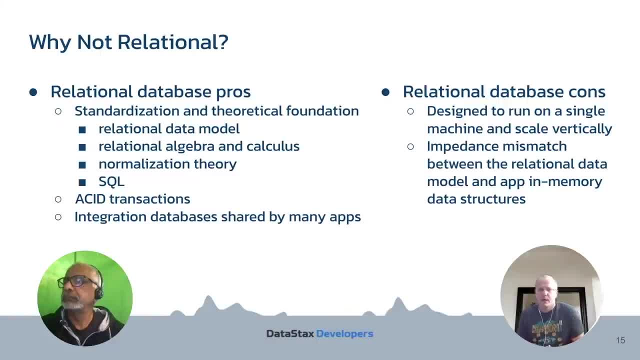 uh, pretty good, but things have changed since then, since 1970s, since then, since 1970s, since then, since 1970s, right um so. another uh disadvantage is: right um so. another uh disadvantage is right um so. another uh disadvantage is impedance: mismatch between the. 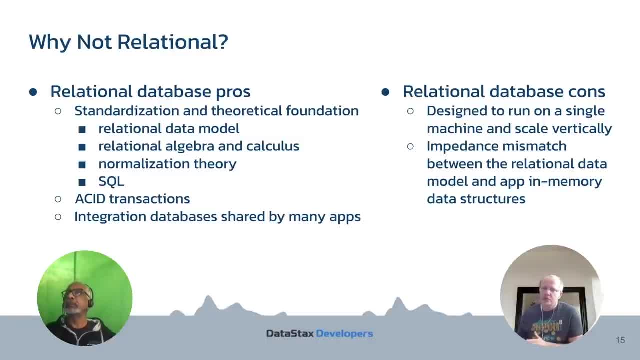 impedance mismatch between the impedance mismatch between the relational data model and app relational data model and app. relational data model and app application in everyday structure. we application in everyday structure. we application in everyday structure. we we mentioned that already. we mentioned that already. we mentioned that already. uh, um, there are, they exist relational to 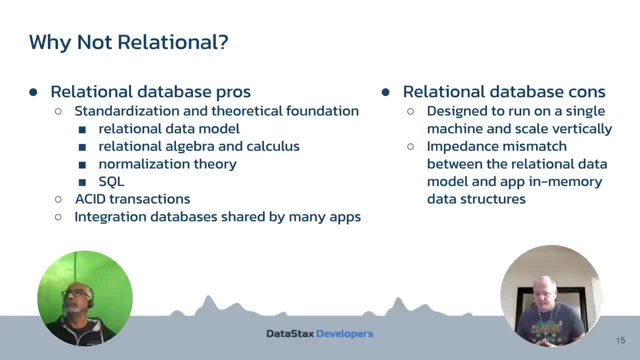 uh, um, there are they exist. relational to? uh, um, there are they exist. relational to object to relational mappings. object to relational mappings. object to relational mappings. to solve that problem, but essentially yeah, to solve that problem. but essentially yeah, to solve that problem, but essentially yeah, in your application you do not. 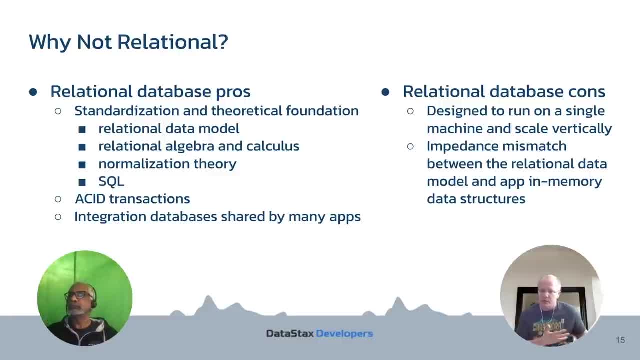 in your application you do not. in your application you do not. manipulate tables and rows in database. manipulate tables and rows in database. manipulate tables and rows in database? you do, you do, you do, but in your application you have objects. but in your application you have objects, but in your application you have objects. okay, so why no? 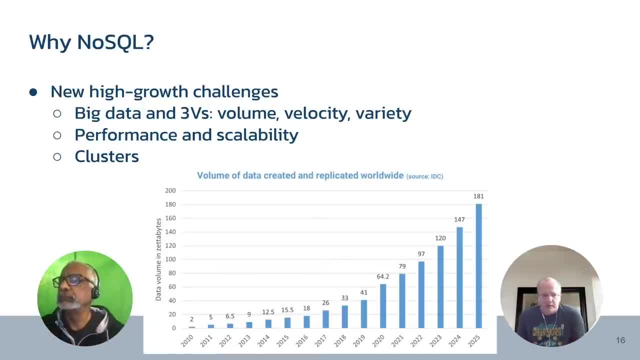 okay, so why no? okay, so why no? no sql relational databases have many no sql relational databases have many. no sql relational databases have many advantages but advantages but advantages. but at some point in uh, at some point in uh, at some point in uh in the beginning of the century, we had 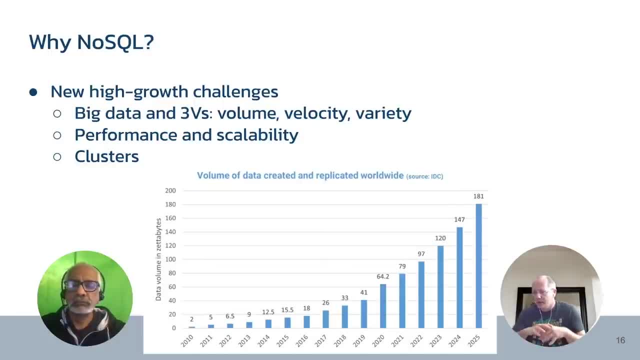 in the beginning of the century we had. in the beginning of the century we had the uh, the uh, the uh, the explosive growth of data- new high. the explosive growth of data- new high. the explosive growth of data- new high growth challenges. that growth challenges. that growth challenges. that data had to be uh processed, that had to 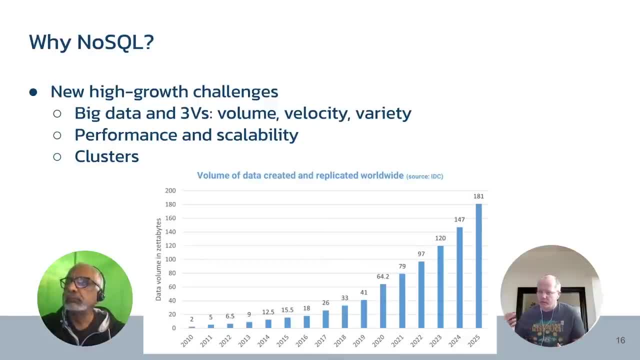 data had to be uh processed, that had to. data had to be uh processed, that had to be stored, that be stored, that be stored. that there could be uh many. there could be uh many, there could be uh many points of collection of that data and it. points of collection of that data and it. 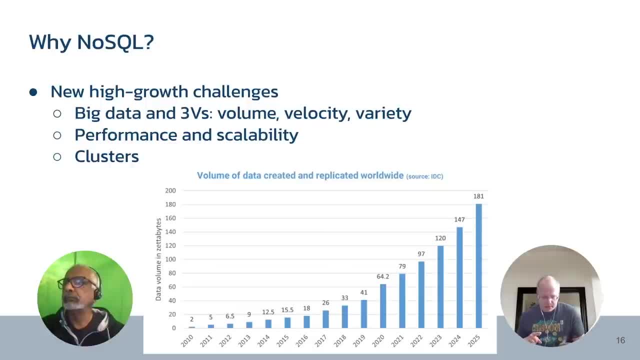 points of collection of that data, and it has to be, has to be. has to be collected fast and and collected fast and, and collected fast and. and. the data can also be in different formats. the data can also be in different formats. the data can also be in different formats, so there is a variety there. 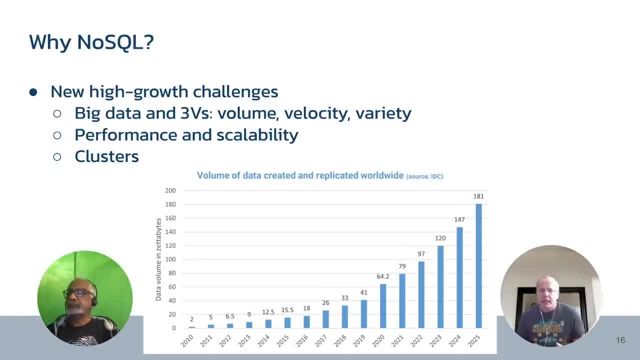 so there is a variety there. so there is a variety there. so you maybe heard about big data, and so you maybe heard about big data, and so you maybe heard about big data and cvs, which is volume, large amounts. cvs, which is volume, large amounts. cvs, which is volume, large amounts, massive amounts of data velocity. 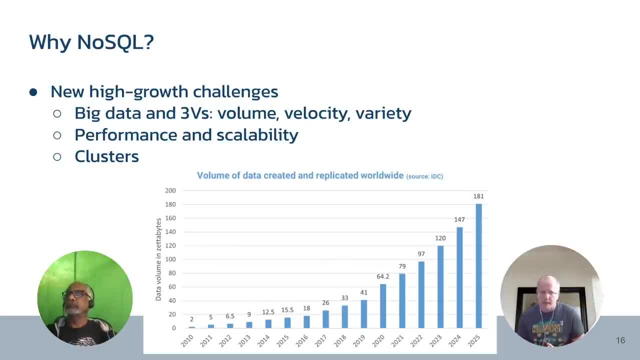 massive amounts of data velocity. massive amounts of data velocity. speed of consuming that data storing. speed of consuming that data storing. speed of consuming that data, storing it into database and variety. using it into database and variety. using it into database and variety. using different formats, but the different formats, but the 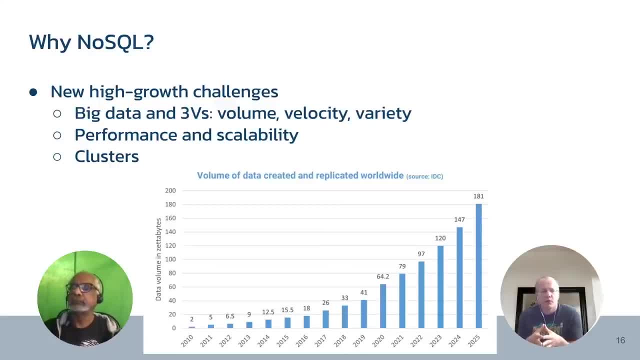 different formats, but the the main reason why no, see no sql. the main reason why no, see no sql. the main reason why no, see no sql databases into existence is because databases into existence, is because databases into existence is because, uh, relational databases lack performance. uh, relational databases lack performance. 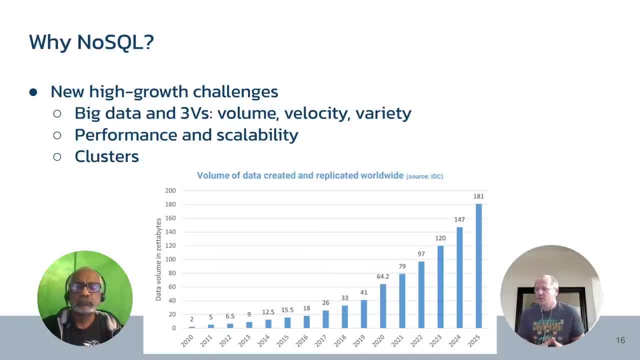 uh relational databases lack performance and scalability in this new environment. and scalability in this new environment and scalability in this new environment, where you have to store, where you have to store, where you have to store petabytes of data right peta, petabytes of data, right peta. 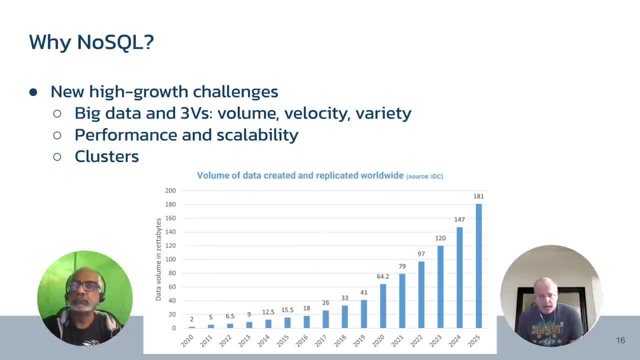 petabytes of data, right peta, bytes of data, bytes of data, bytes of data and those databases and those databases and those databases also needed to scale. no sql database also needed to scale. no sql database also needed to scale. no sql database needs to scale horizontally rather than. 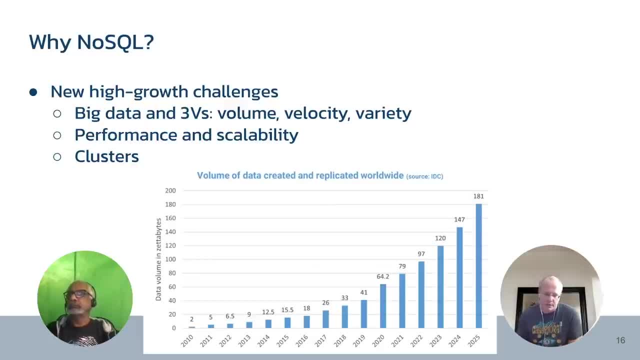 needs to scale horizontally rather than needs to scale horizontally rather than vertically, vertically on clusters. so vertically, vertically on clusters. so vertically, vertically on clusters. so here we have on this graph, we have here, we have on this graph, we have here, we have on this graph. we have this size of volume of data created and 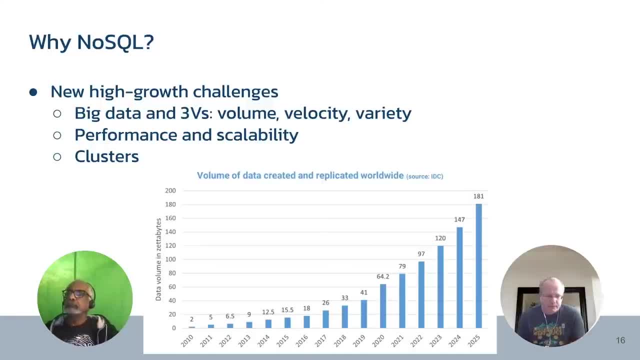 this size of volume of data created and this size of volume of data created and replicated worldwide, replicated worldwide. replicated worldwide, and it's in zettabytes- uh, one zettabytes, and it's in zettabytes- uh, one zettabytes, and it's in zettabytes- uh, one zettabytes is. 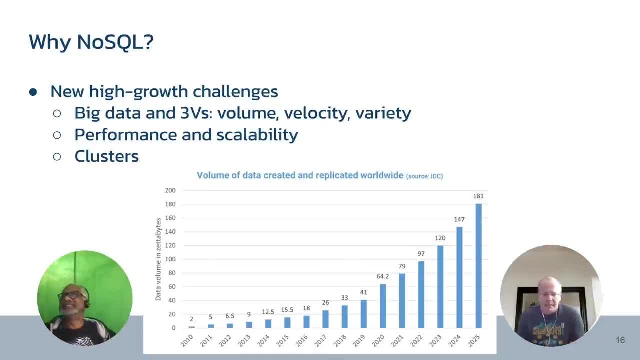 is is: um with one zettabyte is one million. um with one zettabyte is one million. um with one zettabyte is one million. petabytes, petabytes, petabytes. uh, yeah, it's, it's quite big. but uh, yeah, it's, it's quite big but. 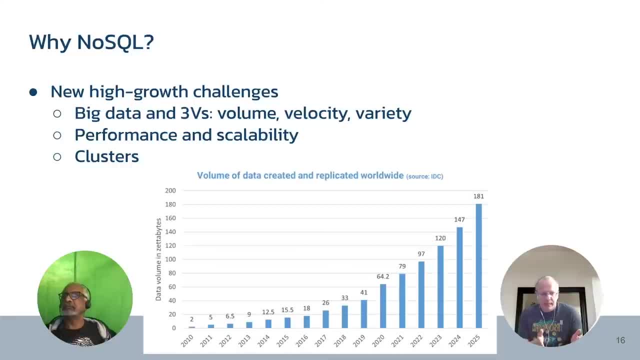 uh, yeah it's, it's quite big, but essentially you can see in. essentially, you can see in, essentially you can see in: 2010s: we have this, uh, zettabyte 2010s. we have this: uh, zettabyte 2010s. we have this, uh, zettabyte. error um started and it keeps growing. 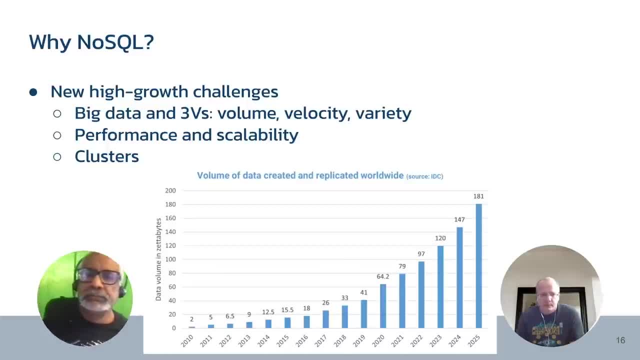 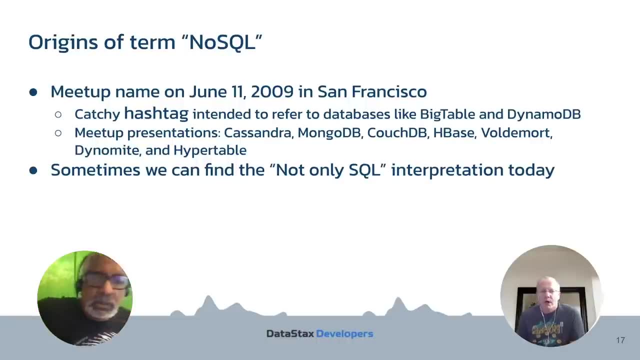 error um started and it keeps growing. error um started and it keeps growing right, right, right. so and and the relational databases so and and the relational databases so and. and the relational databases have difficulty scaling to these sizes. so origins of term: no sql, this sometimes. so origins of term: no sql, this sometimes. 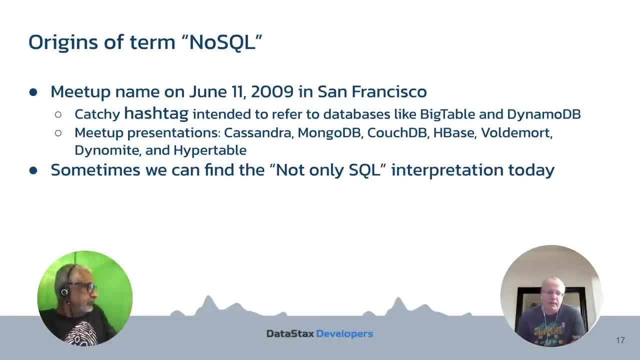 so origins of term: no sql. this sometimes can be, can be, can be controversial topic but essentially controversial topic but essentially controversial topic but essentially, uh, that was the name of the meetup and uh, that was the name of the meetup and uh, that was the name of the meetup. and also 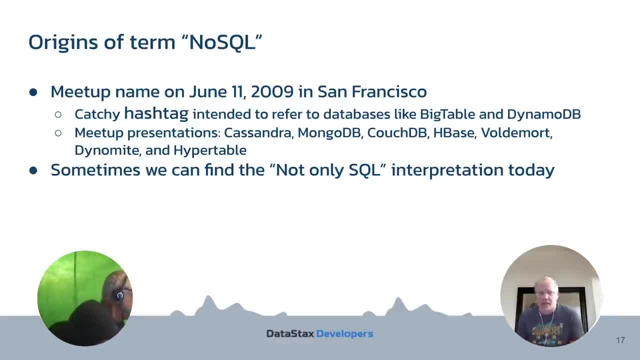 also also catchy hashtag. catchy hashtag. catchy hashtag that intended to refer to databases. that intended to refer to databases. that intended to refer to databases like big, like big, like big, big table, and and and big table and and and big table and and and. dynamo db from google and amazon. 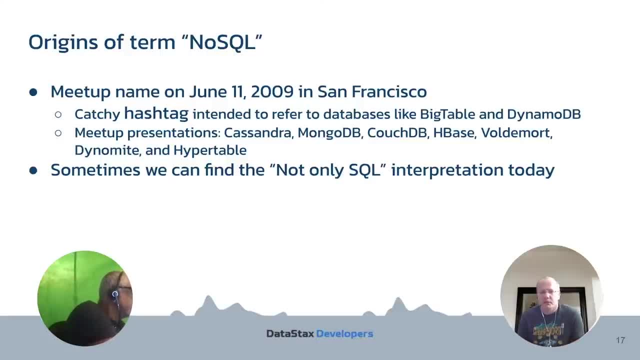 dynamo db from google and amazon. dynamo db from google and amazon, respectively. so meetup was in 2009, in respectively. so meetup was in 2009, in respectively. so meetup was in 2009 in san francisco. the presentations were on san francisco. the presentations were on: 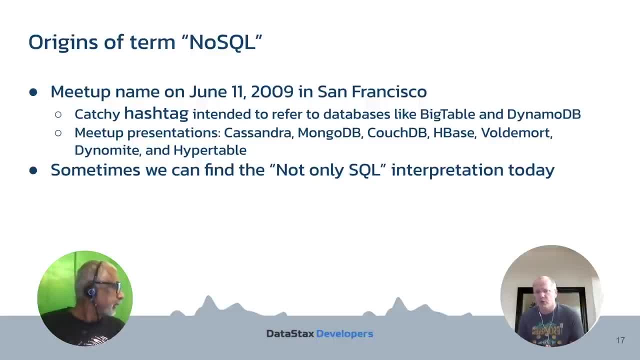 san francisco. the presentations were on: cassandra cassandra, cassandra, long db couch- db h base. long db couch- db h base. long db couch- db h base and so forth. and we are actually going to and so forth, and we are actually going to and so forth, and we are actually going to mention. 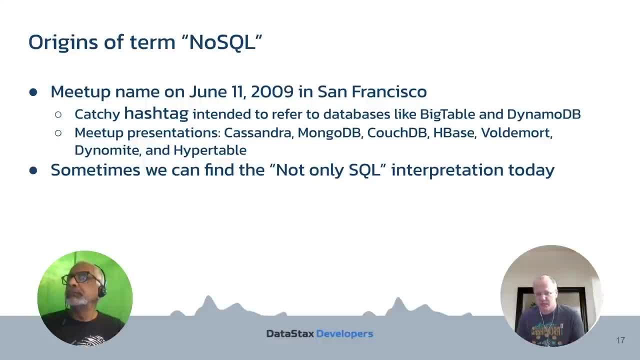 mention, mention those we are going to use one of those, those we are going to use one of those, those we are going to use one of those, and and we're going to mention the talk, and, and we're going to mention the talk and, and we're going to mention the talk about the other four. 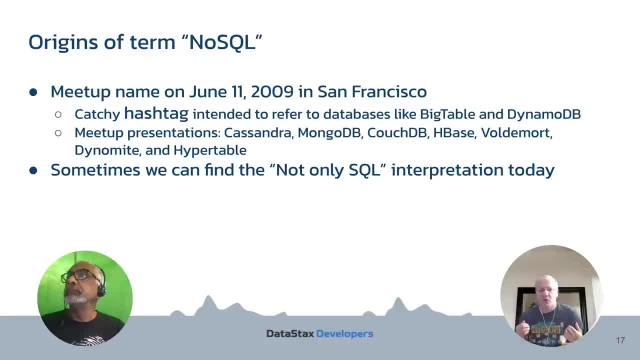 about the other four. about the other four. okay, sometimes we can also find okay. sometimes we can also find okay. sometimes we can also find. the uh note on the. the uh note on the. the uh note on the sql interpretation today, but um again. sql interpretation today, but um again. 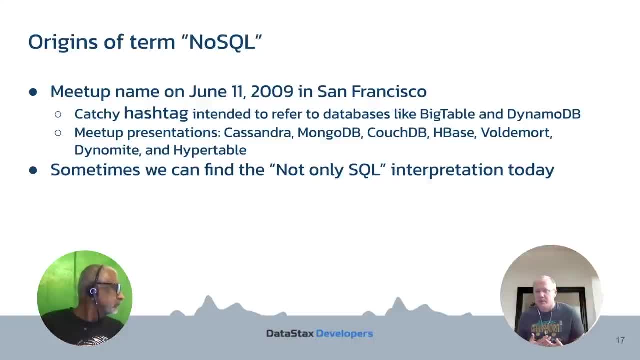 sql interpretation today. but, um again, it's not, may not be very descriptive. it's not, may not be very descriptive. it's not, may not be very descriptive because because, because relational databases they support, not relational databases. they support not relational databases. they support not only sql is. 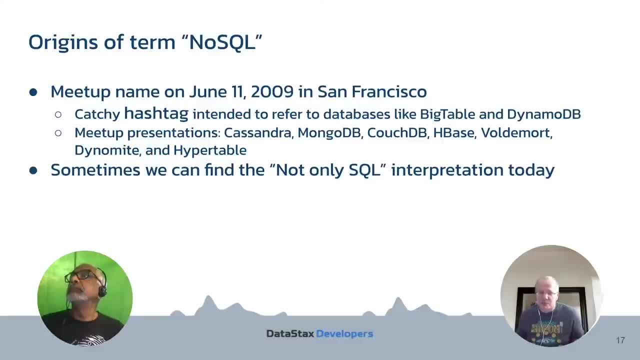 only sql is. only sql is. they can support other languages as well. they can support other languages as well. they can support other languages as well. if you, if you look at databases, if you, if you look at databases, if you, if you look at databases- relational databases like oracle- so what? 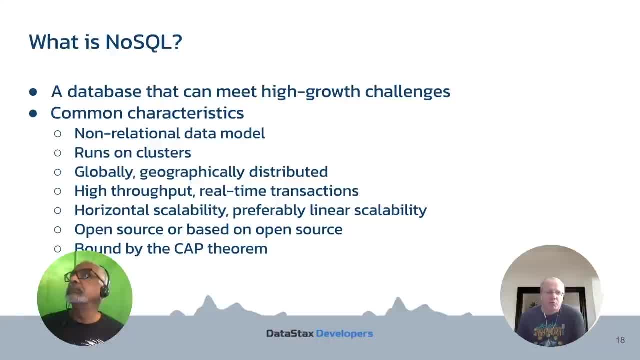 relational databases like oracle. so what relational databases like oracle? so what is really is really is really no sql. it's a database that can meet high growth challenges. we talk about high growth challenges. we talk about high growth challenges. we talk about performance and performance and performance and high and scalability, so that we can. 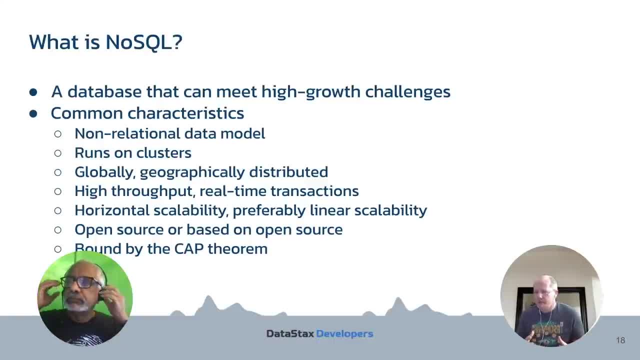 high and scalability so that we can high and scalability so that we can store and create massive store and create massive store and create massive data sets. okay, and those databases data sets okay, and those databases data sets, okay, and those databases commonly have these, commonly have these, commonly have these characteristics- uh, not, it's not. 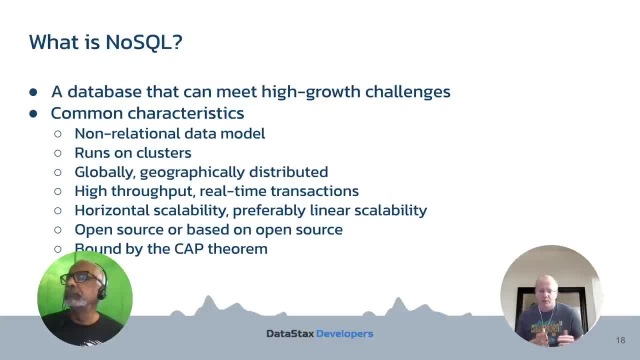 characteristics- uh not, it's not characteristics, uh not. it's not necessarily that each no sql database necessarily that each no sql database, necessarily that each no sql database will have all of them will have all of them. will have all of them, but probably most of them, okay, so they. 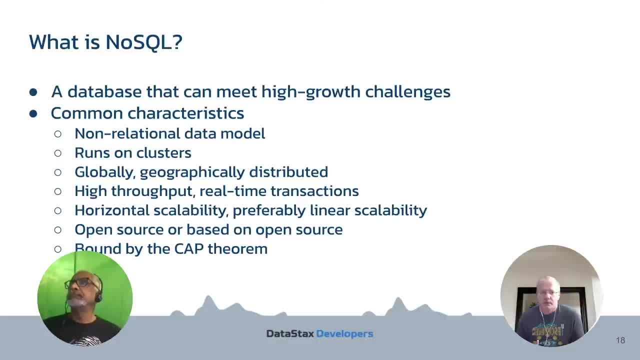 but probably most of them okay. so they, but probably most of them okay, so they have non-relational, have non-relational, have non-relational scale on a cluster horizontal right scale on a cluster horizontal right. scale on a cluster horizontal right non-relational data models. 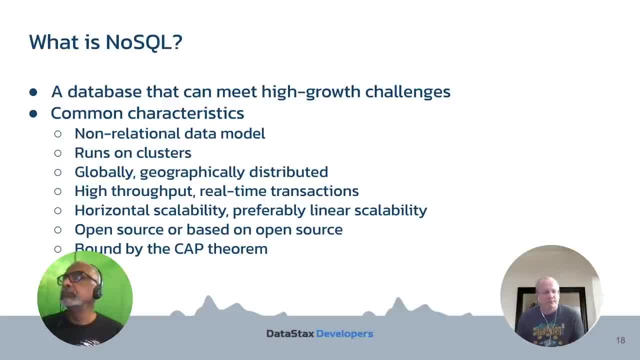 non-relational data models. non-relational data models. they run on clusters of machine of. they run on clusters of machine of. they run on clusters of machine of servers, servers, servers- they can be globally geographically. they can be globally geographically. they can be globally geographically distributed- different data centers in. 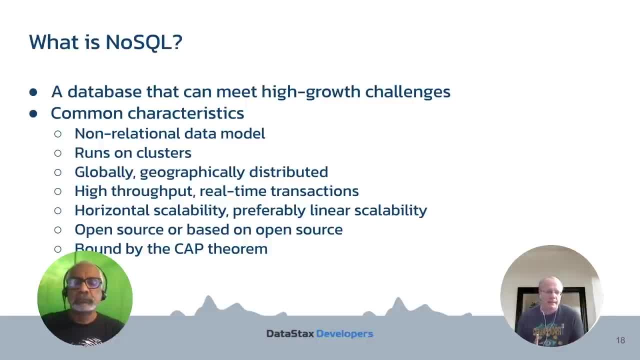 distributed different data centers in distributed different data centers in different different, different countries, different continents, countries, different continents, countries, different continents. they support high throughput. many, many. they support high throughput. many, many, they support high throughput. many, many transactions, transactions, transactions, real-time transactions per seconds. real-time transactions per seconds. 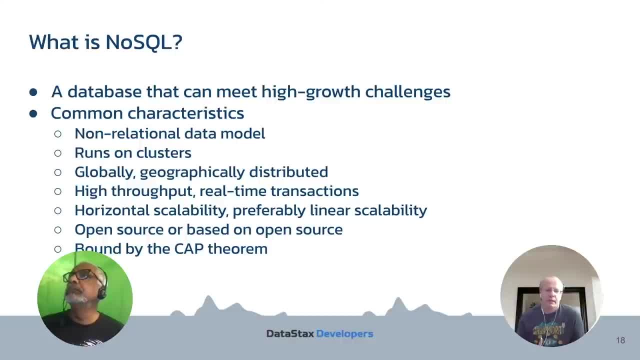 real-time transactions per seconds. millions of them, millions of them, millions of them. they scale horizontally and preferably they scale horizontally and preferably they scale horizontally and preferably linearly, linearly, linearly. so if, if the number of transactions that, so if, if the number of transactions that 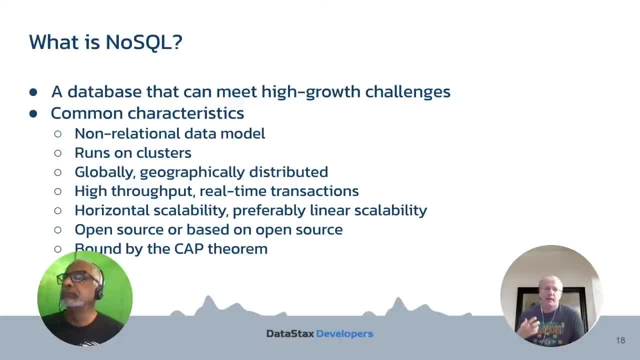 so if, if the number of transactions that you need to handle doubles- you need to handle doubles, you need to handle doubles- then you simply double the size of your, then you simply double the size of your, then you simply double the size of your. cluster, you add, cluster, you add. 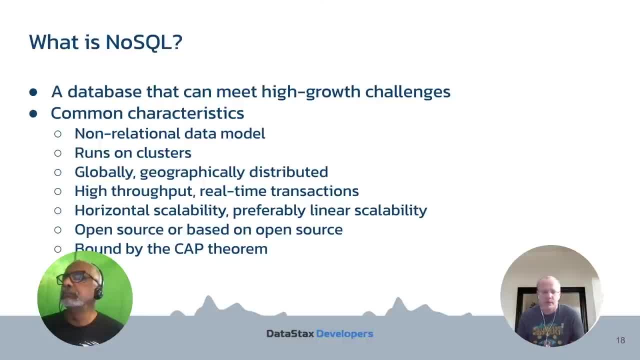 cluster, you add twice as many nodes, twice as many nodes, twice as many nodes to be able to handle that, to be able to handle that, to be able to handle that increased volume of transactions, increased volume of transactions, increased volume of transactions. they frequently open source. they frequently open source. 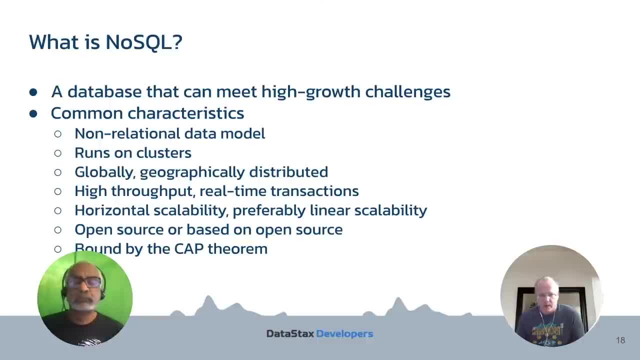 they frequently open source, all based on open source, all based on open source, all based on open source. but there can be, of course, some. but there can be, of course, some. but there can be, of course, some proprietary systems, proprietary systems, proprietary systems, the cap serum, and not always some of. 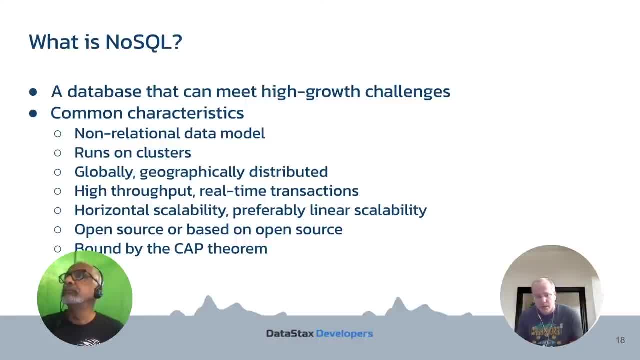 the cap serum and not always some of the cap serum and not always some of them. them, them, uh, some of them that that may be even, uh, some of them that that may be even, uh, some of them that that may be even famous, famous, famous. no sql databases in graph space in. 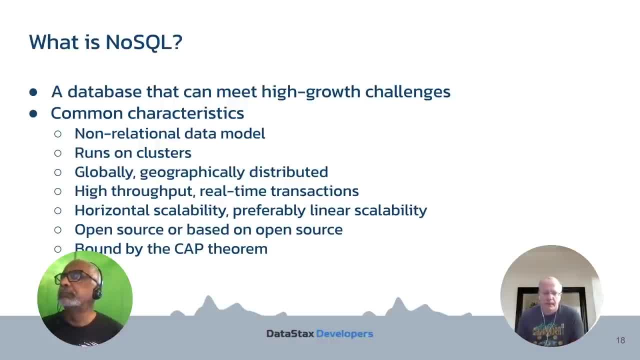 no sql databases in graph space. in no sql databases in graph space in particular, may not particular. may not particular. may not be fully distributed and may not be fully distributed and may not be fully distributed and may not comply with the. the comply with the. the comply with the. the cap serum. we will talk about cap serum. 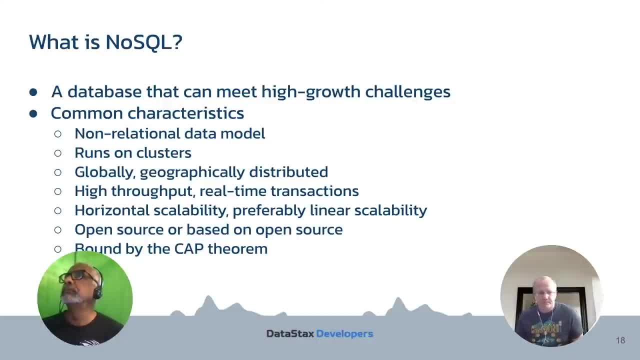 cap serum, we will talk about cap serum. cap serum, we will talk about cap serum shortly, shortly, shortly. so relational versus no sql, let's so relational versus no sql. let's so relational versus no sql. let's compare the these two relational, compare the these two relational, compare the these two relational provides standard relational model. 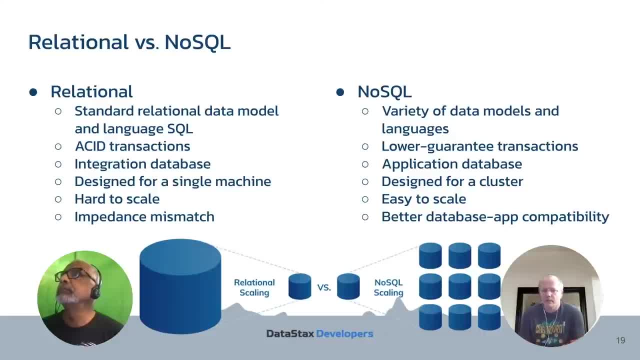 provides standard relational model. provides standard relational model. and language sql: no sql. and language sql: no sql. and language sql: no sql. provides variety of data models and provides variety of data models. and provides variety of data models. and languages, languages, languages. uh, then we have acid transactions for. 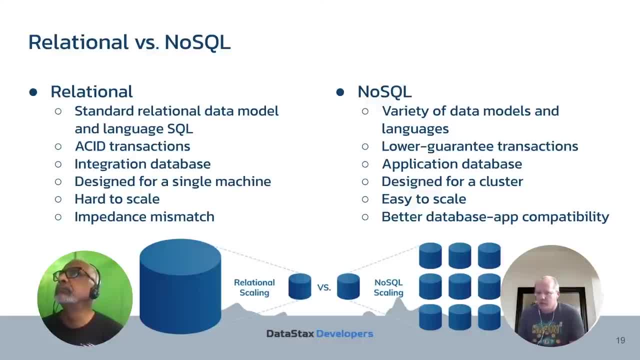 uh, then we have acid transactions for uh, then we have acid transactions for relational. we have lower guaranteed relational. we have lower guaranteed relational. we have lower guaranteed transactions for no sql transactions for no sql transactions, for no sql. because the again because of performance, because the again because of performance. 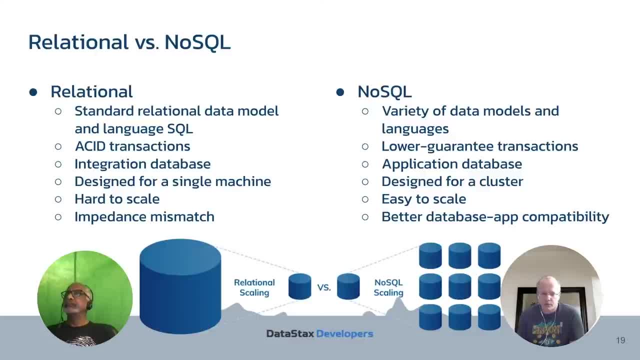 because the- again because of performance. yeah, the transactions and two-faced are. yeah, the transactions and two-faced are expensive. we have integration database on the relational side. on no sql site. we have application databases. so we design no sql database. we model our data specific to one application. we do not. 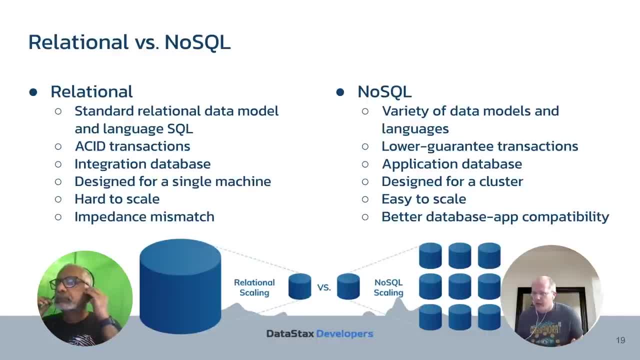 usually support five applications, uh, on the same set of tables or same set of json documents and so on. so it data modeling specific to application. relational design for single machine: no sql design for a cluster right away. relational- hard to scale, they scale vertically. sql- easy to scale. 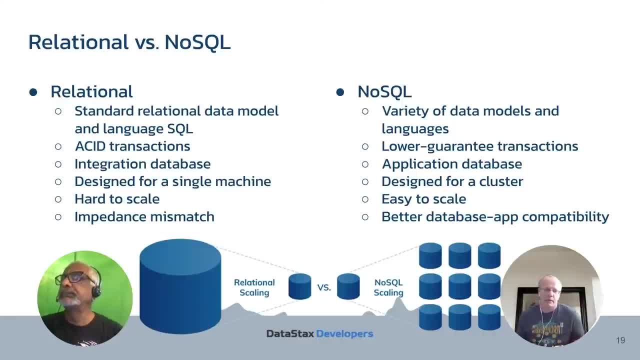 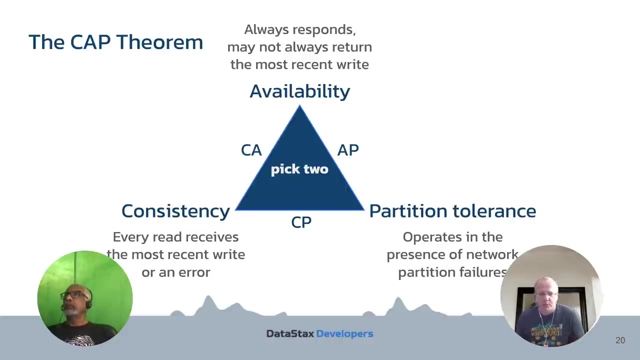 and and cost effective. they scale horizontally. relational have impedance mismatch, no sql have better compatibility between database and application data models. so, on this, if this image see that relational scales vertically, no sql scales horizontally. so let's, let's talk about cap, serum, serum and and, and we will do very shortly, we will have the first hands-on and we'll hit and no. 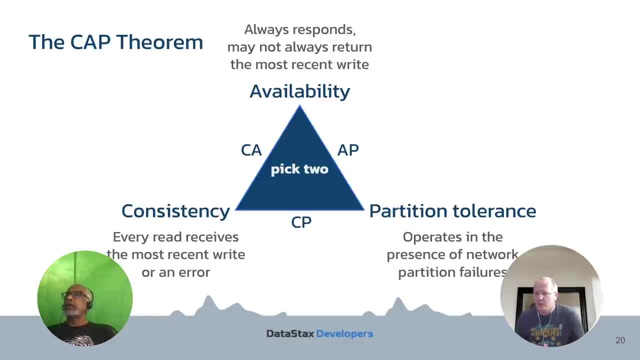 sql. uh, we'll use no sql databases, our first database. why? why is no sql popular amongst kind of like the big companies, like you know, like um, apple, linkedin, you know a lot of places, facebook, where it originated? is it because it was primarily because of the horizontal scaling aspect of it? because, you know, with a 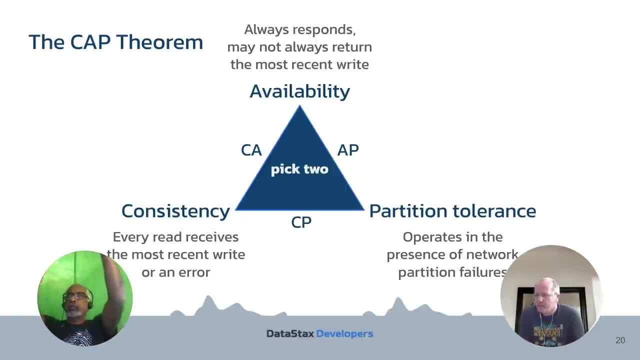 single database. you can scale it, scale it up, up and up and up and up only to a certain degree. after that, you know, it's just going to fall over and die right. um, is that one of the reasons, or are there a variety of reasons? you know, maybe you're getting to that, i well, the main reason is is: 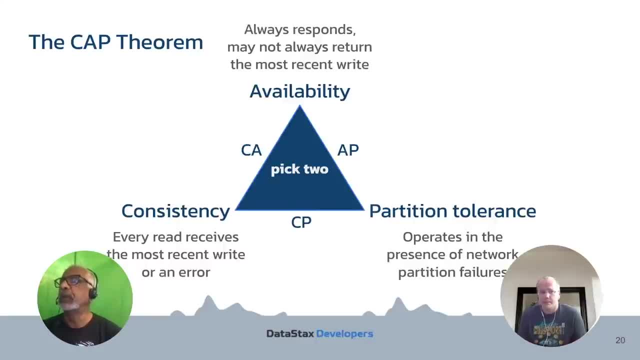 performance. that's the main reason. uh, yeah, if we, if, if relational databases could, could have that amount of data, there was no motivation to create something new. um, in in that case it. but the main is, of course, uh, scalability, it's horizontal scalability you, you hear about. 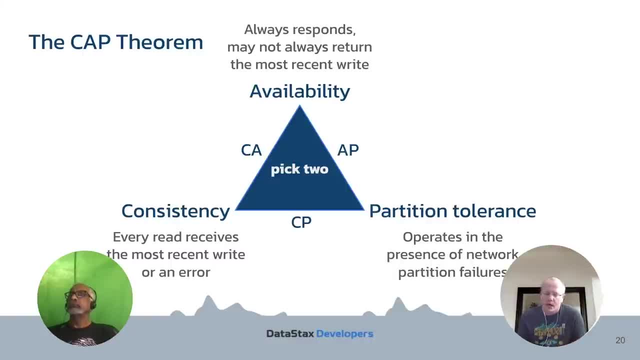 uh, um, thousand node clusters, um, for no sql databases like for, for example, apple running cassandra with, with uh, using many thousands of servers. but usually don't hear that for relational databases, right, you don't hear about thousand node server relational database serving some application. so use case, use cases changed, uh, the those 3v big data requirements changed, and we 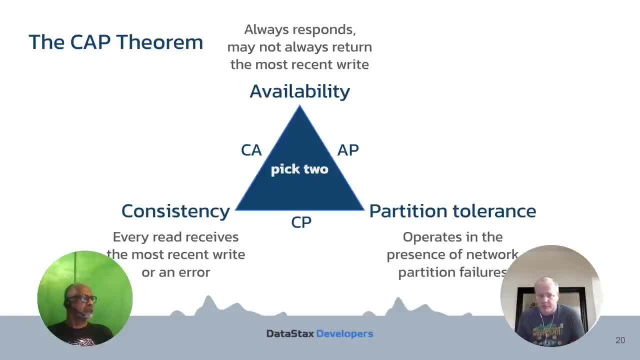 had to solve the problem differently. okay, so going back to the cap serum, uh, the cap serum applies to distributed data storage systems, distributed databases, and it basically states that, out of these three properties, a distributed database can only provide or provide two guarantees: two properties, so it can be available and partition tolerant, or it can be consistent and 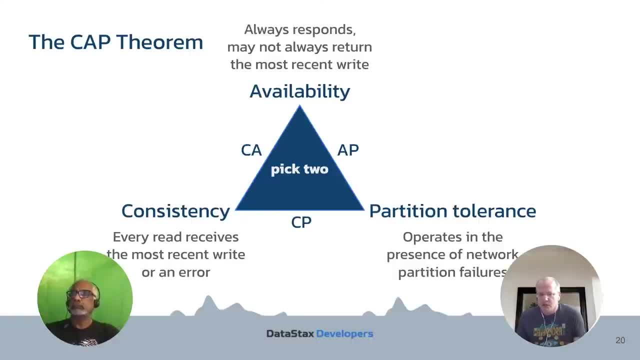 partition, tolerant, uh, usually not consistent and available at the same time. i will talk about it. so what are those properties? so you can, you can only pick two for for distributed database. the properties consistency: every read receives the most recent right, uh, or an error. so why? why are we? 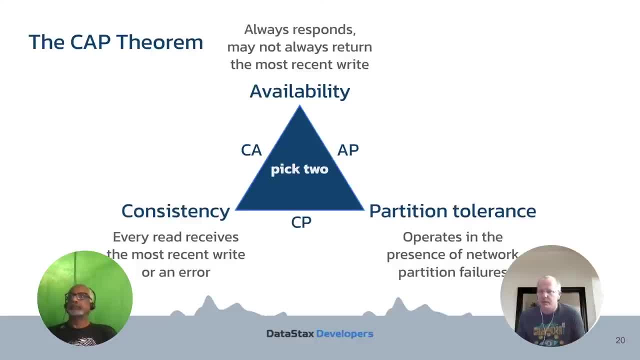 talking about most recent right. and all that because when you, when we're writing data into distributed database, it will go to several nodes that are replicated data and some of them will store the data in a few milliseconds and and maybe one replica will will have a lag and will store it in 20. 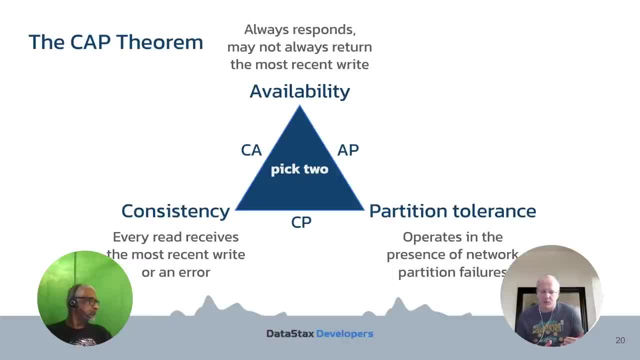 milliseconds. so when you read data, you with consistency, you guarantee that you will read the most recent one or there will be an error. an error means you, if the system is currently not available to, to respond. so that's why you kind of- uh, i'm going to select between 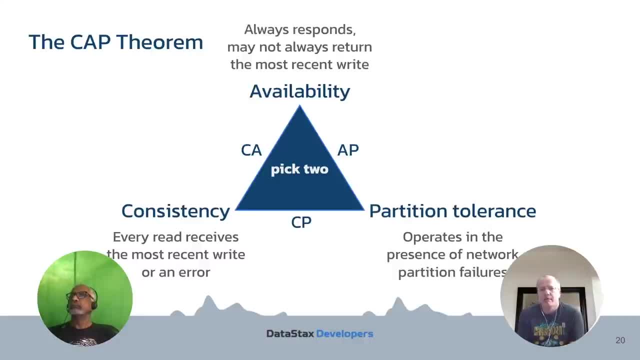 consistency and availability. availability refers to always. the system is always available to you. the system always responds but may not always return the most recent right. so it's always available, always gives you the result but may be inconsistent result. and then partition tolerance operates in the presence of network partition failures, if not goes down, if the whole data center. 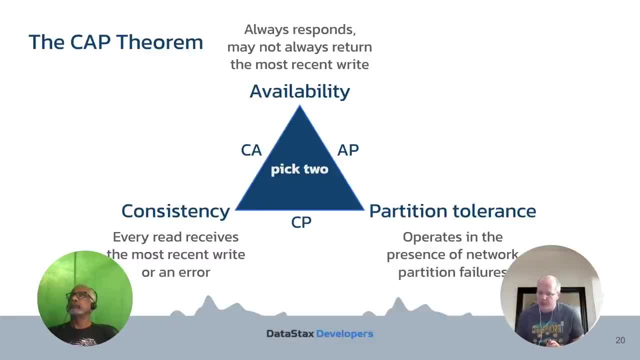 is not communicating with a different data center, you still can operate. so because these are distributed databases, you basically have to choose partition tolerance. we have thousand nodes in your cluster. if one goes down, you still want to operate, and one will go down for sure because it's a large cluster. so you always basically select partition tolerance and then you pick. 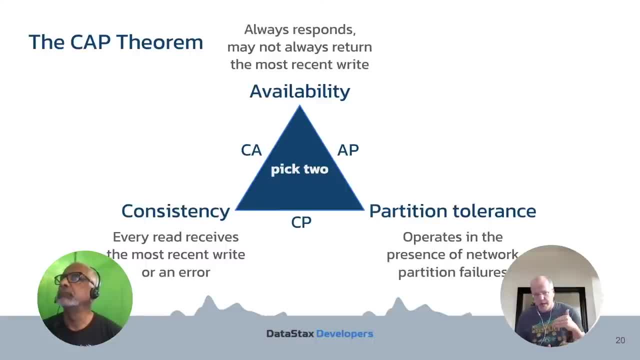 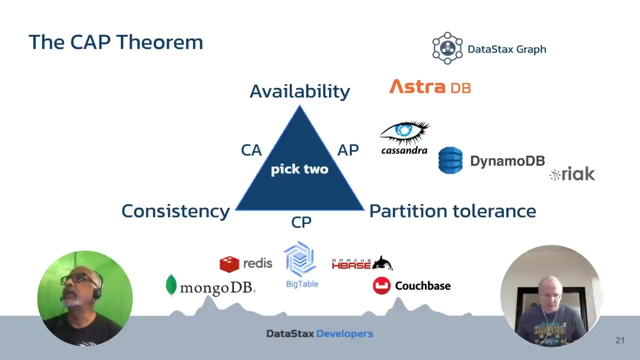 either consistency or availability, whatever is more important to you, and you usually so. for the reason of: because these are distributed database, you do not pick consistency and availability at the same time, because if just one server goes down, you lose the whole system. that doesn't work in in in a distributed environment. so so here's some. 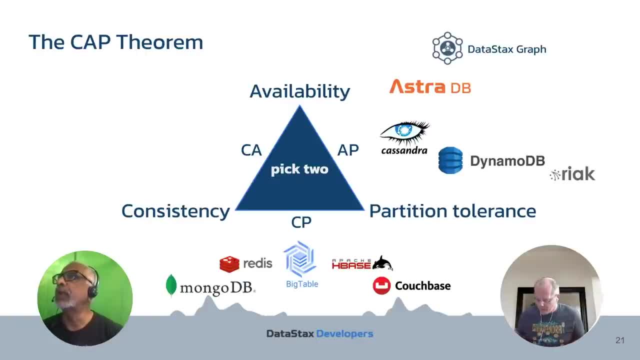 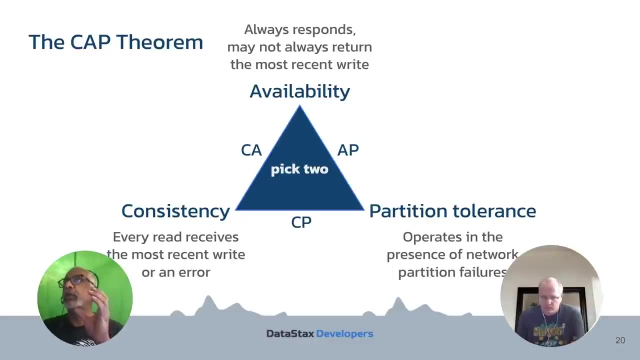 examples just again. most you know to talk about the cat theorem. uh, i think i think you can have all three you know in in like a working scenario when there are no failures and all that which never happens in distributed system. completely get that, uh, but but when a failure occurs, 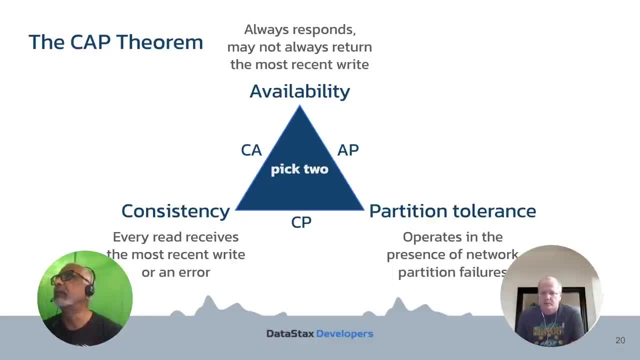 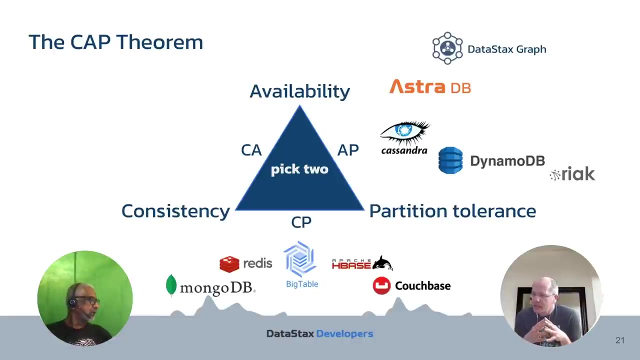 you can pick only two of the three correct. um, that, uh, something that makes sense. yeah, that's right. that's right, that's correct. and and um, nowadays, the, this distinction actually, uh, between cp, ap system can also be blurred. so many systems, they, they can actually tune your consistency and and trade it for availability and vice versa, so you can actually 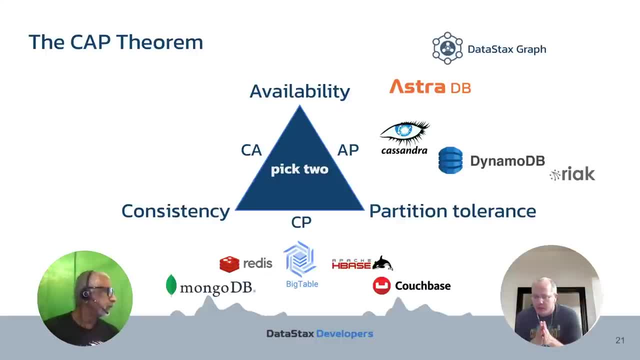 have a system that that um can withstand multiple nodes and even data center failure. but may uh, yeah, at this point i think mickey glory um, you know great, glorious name, you know- has a great question which is like: uh is no sql and transactions uh kind of mutually exclusive. in other words, uh with no sql, can you also achieve? 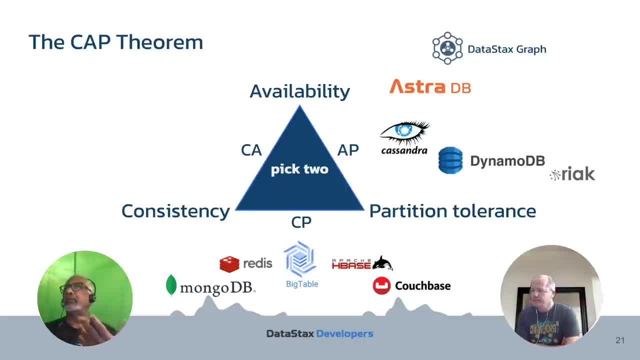 transactions. i know stefano already respond to that. um, responded to that, uh, but, but you know, if you want to add your thoughts, that'll be great. um, yeah, so you, definitely you can, but you have. you may have them implemented in the database, or they. they may already exist there, or you may have to add them or add some kind of. 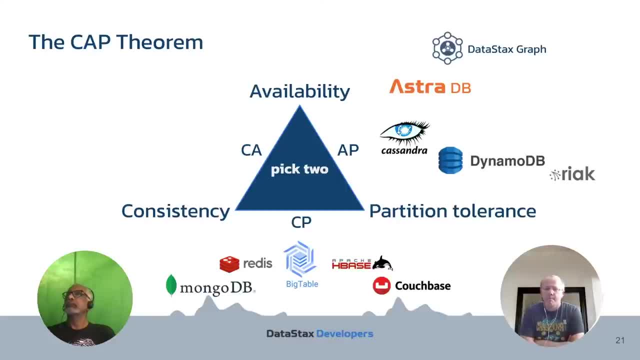 transaction process and framework. but uh just understand the reason why are usually not there is because of the um, they are complex and they will, uh, will, will not be performant enough. uh for no, no sql database to support the requirements that we talked about. so in, in, in. 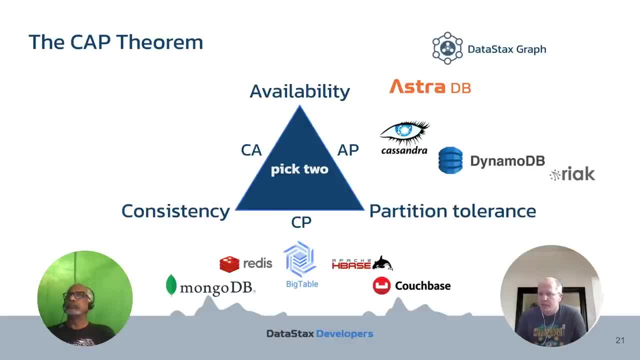 systems like cassandra and astro db and actually many others. there are lightweight transactions that use pexus protocol, which, which doesn't guarantee acid, but it guarantees some lower, lower. it has some lower guarantees for um transactions and acid and acid- for those who just you know not to insert anybody's intelligence here- is atomicity, consistency, isolation and 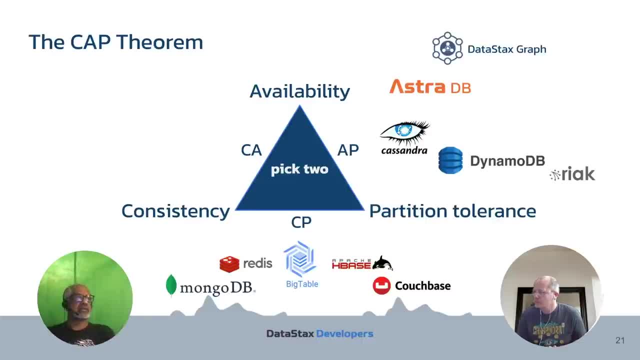 durability. you know that's the typical properties associated with the transaction. yeah, but you understand that transaction processing is kind of a separate from the database itself. you can add transaction processing on top of the database, so they can, but in many it may also in many use cases, uh, with no sql, that we think differently and 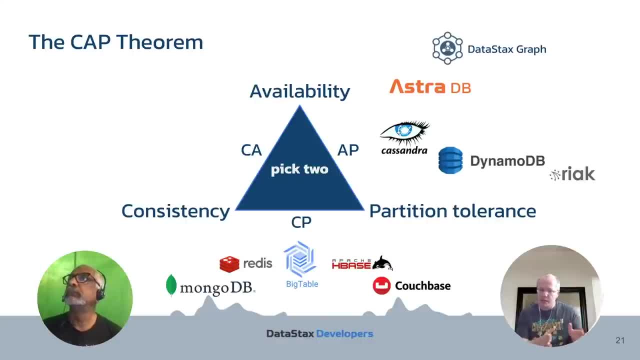 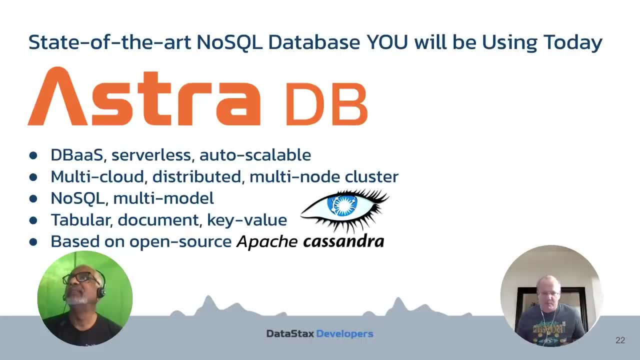 kind of do things differently so that we don't need asset properties and unfortunately that's. that's a big topic and i will not be able to cover it right now, so we will stay focused on our- and our- uh nose- introduction to no sql databases. so what we're going to use today is state-of-the-art no sql database. 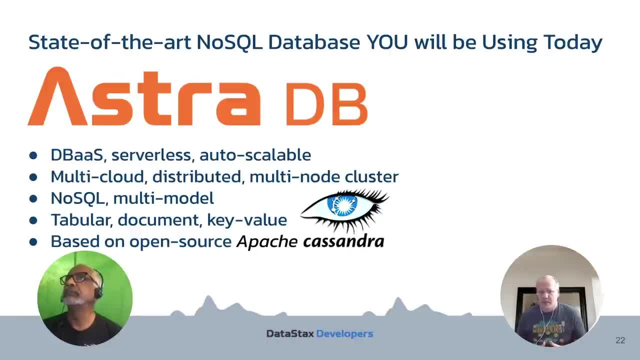 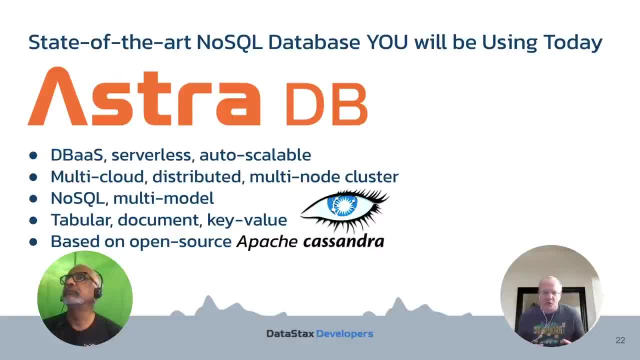 available, so you don't need to specify how many nodes in the cluster you will have. it will scale, it will. it will become a larger cluster or smaller cluster based on your workload. it's going to be free for you to use and it's a model. it will run in aws. it will run in in google cloud or azure. 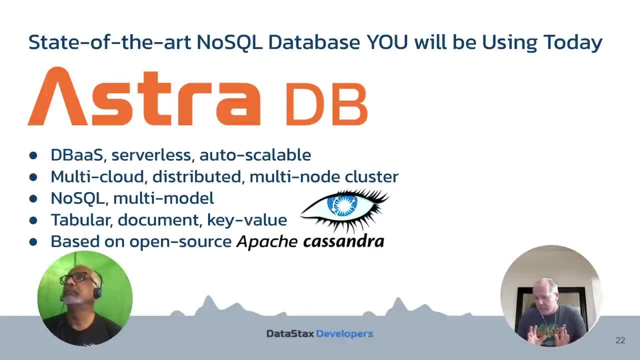 it's distributed behind the under the hood. there will be multi-node cluster, of course, and and essentially actually southern node, maybe southern node cluster that will handle multiple tenants and you will just be using three of those nodes and things like that. it's a no sql, it's multi-model, it supports uh tabular document and key baler we're going to use 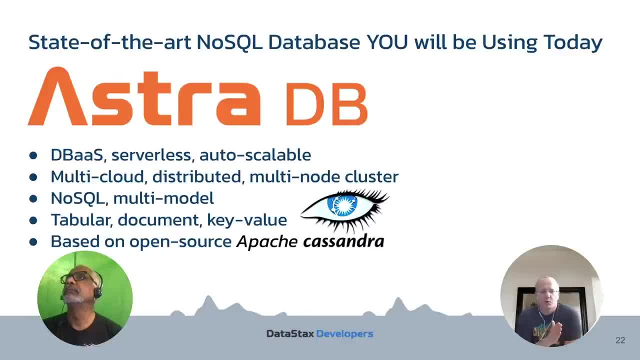 this database for all three of those types and it's based on open source, apache, cassandra it's, it's has linear scalability, high availability, uh can serve high throughput applications and so on. so this is one of the best uh and and unique, so this is actually the first. 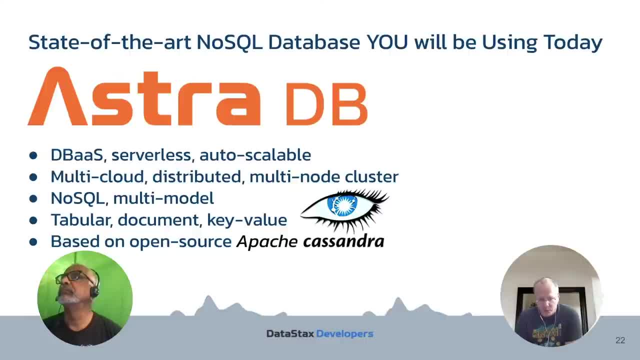 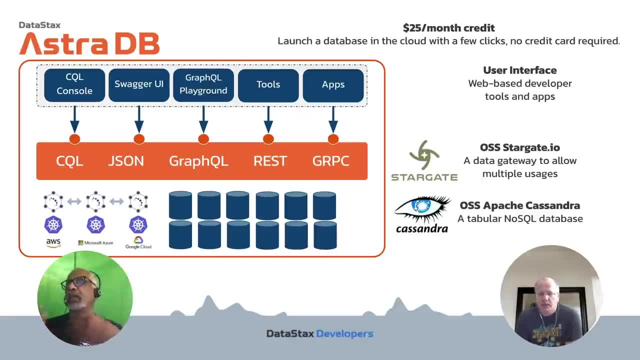 serverless database service which is based on open source. and one of the one of the cool things is, like you said, you know multi-region, you know disaster recovery, you know any of those you don't need to worry because we kind of take care of that for you. you know you may not get into the. 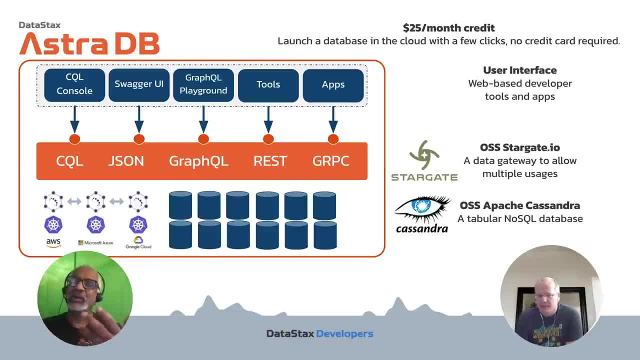 free tier. uh, you know, so, if you, but you can, you can, definitely, you know, get it if you want. okay, so you may have to put in a credit card or you may have to, you know, get a license or something like that, and we'll talk about that. yep, yeah, and this database is going to be free for you, you get you. 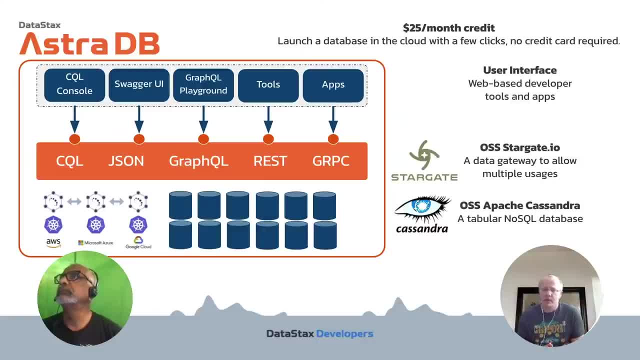 don't need to add, enter credit card or anything you get. you just need to register. you get 25 monthly credit. uh, 25 doesn't seem like a lot, but it's enough to actually run millions and millions and write operations. so definitely i'm not going to use even a single dollar today. 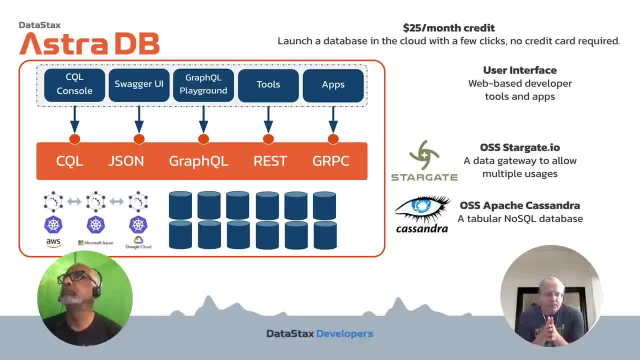 from that and we will use for our hands-on. we will use different uh web-based tools: cql console to to work with tabular databases using cql. cql is a cassandra free language similar to it's- it's like very similar, has very similar syntax to sql. we'll use swagger ui to work with. 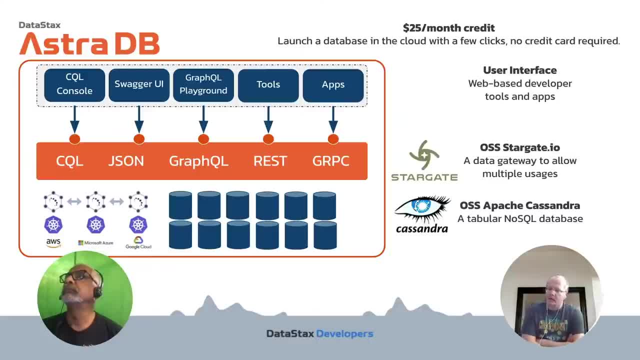 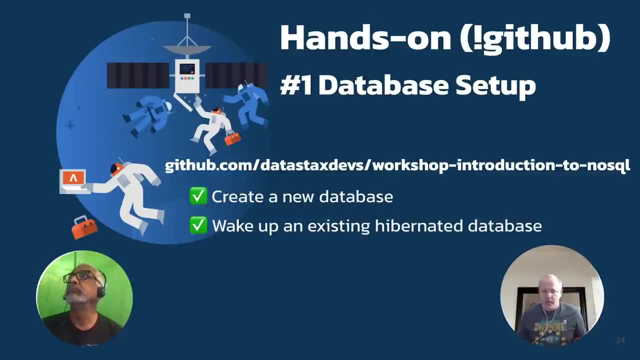 um rest api and document json api, and we will also use graphql playground, which is another web application that we have flying that allows you to work with graphql api. okay, and with that, uh rex is gonna help you with setting up your first database, or you can just: yeah, that'd be great. all right, let me um go to my screen and 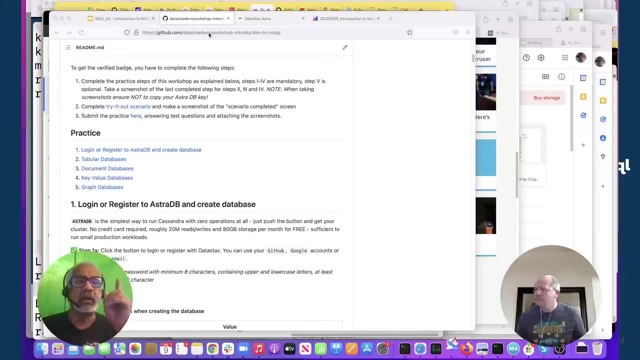 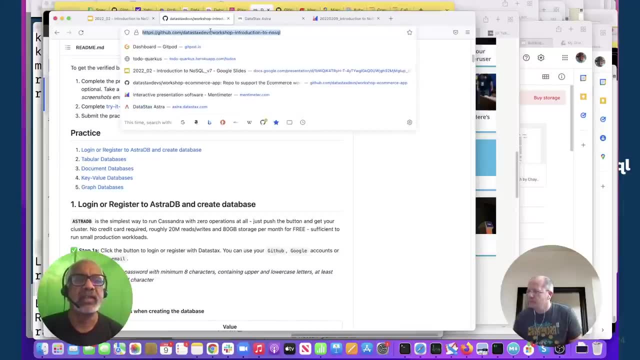 the place to get started is just hit uh pound or exclamation github- okay, in chat, and it will point you to this uh repository, okay, which is github data stacks, devs, workshop- introduction to no sql. all our workshops, you know, are on github and you can. you can just follow along. 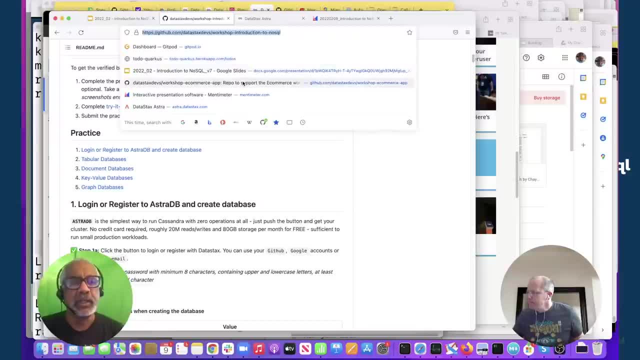 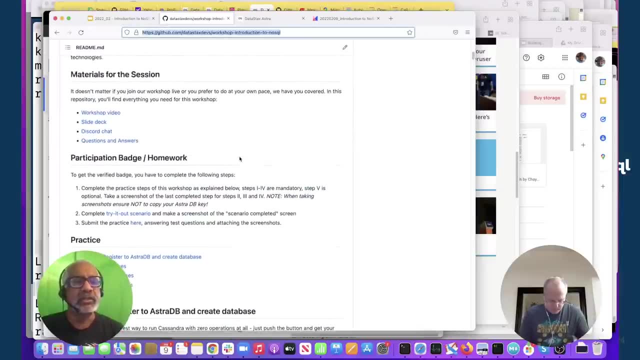 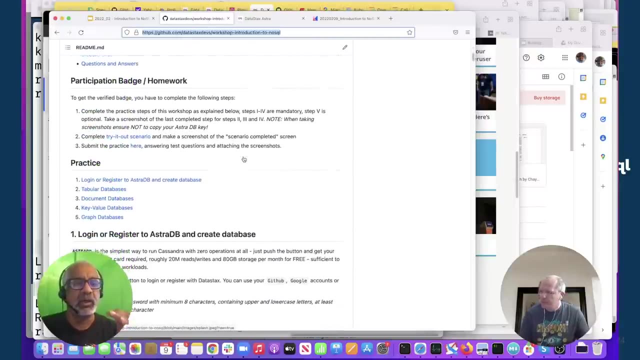 they are primarily intended to kind of do it yourself, you know kind of a self-help, um, but um, you know, you can watch the recording as well, whatever suits your fancy. okay, so this is all really. you know, i mean, i go to this, uh, you know, github link and then kind of follow along you. 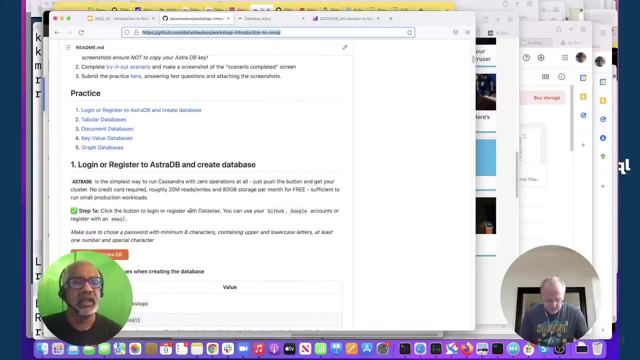 know, very easy to follow along instructions. the first thing that it's gonna. you know, and- and i think, uh, artem already talked about this- astra is the simplest way to run cassandra. one of the criticisms about astra, or rather cassandra, was that it was. you know it's, it's cool, it's linearly. 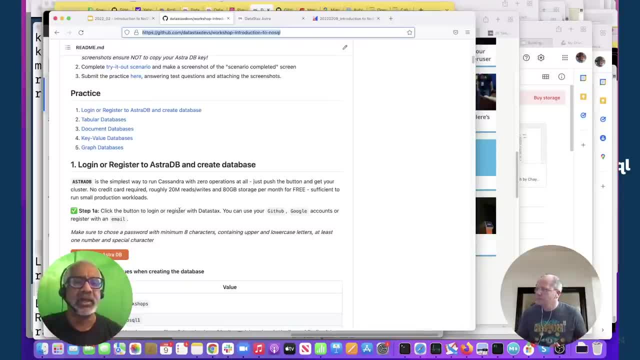 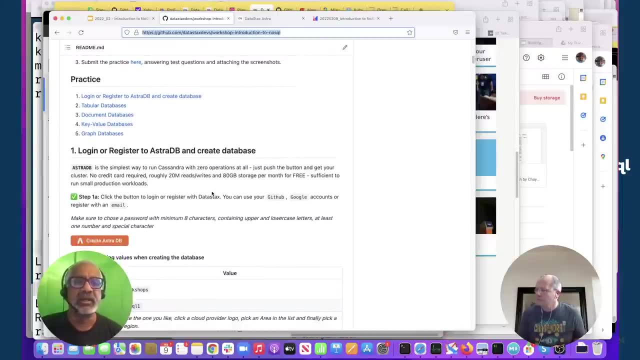 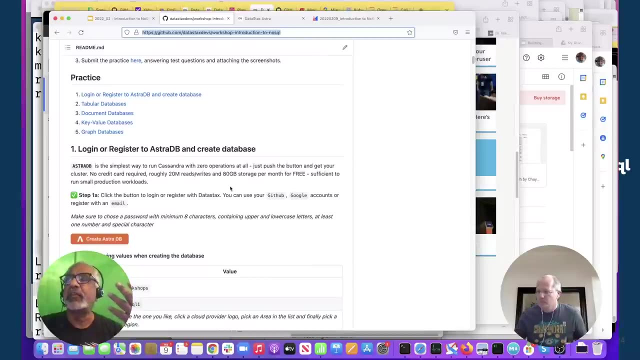 scalable. it's not easy to set up, right, so so with this you don't really need anything. you don't even need a credit card and, like what martin artem is saying, you can do 20 million reads and writes, as it says here, and about 80 gigabytes uh storage free per month. um enough to run some, some, fairly. 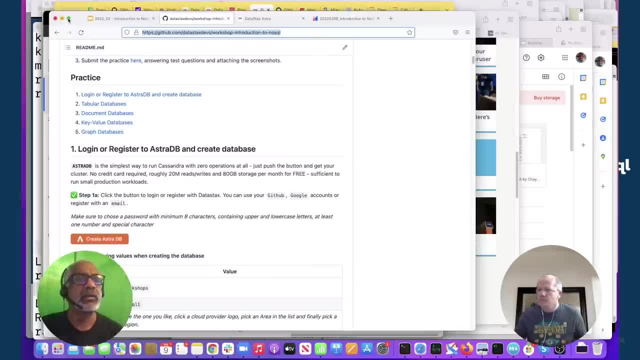 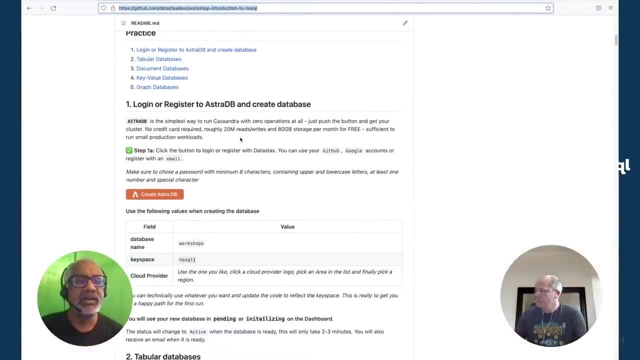 sophisticated production workloads. okay, so let me go into full screen mode and you see if you can see that, uh better, okay, so that's all i'm gonna do. i'm just gonna follow along. you know, take your time. you're gonna create a database, um, and a key space. 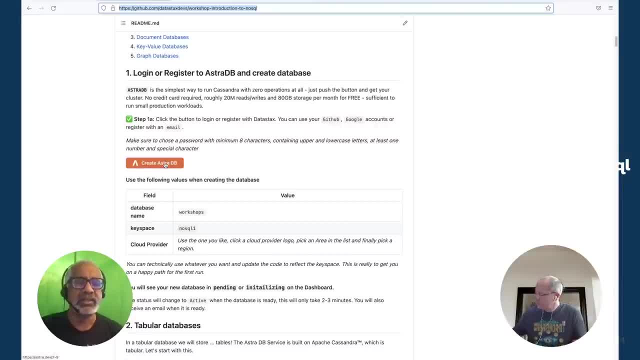 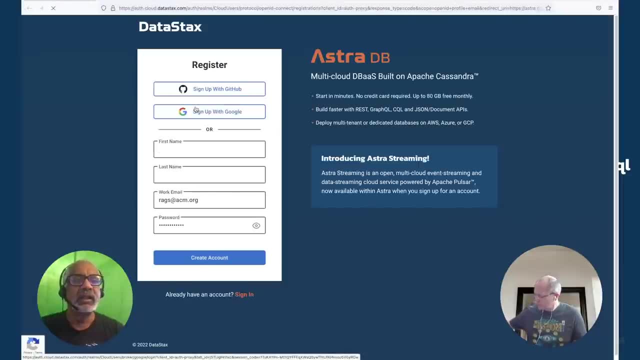 called no sql one. okay, all that you're gonna do is you're gonna click on this, okay, and i'm just gonna click on this and say open link in new window, okay, and you it'll take you to this particular screen, okay, which is basically a registration. 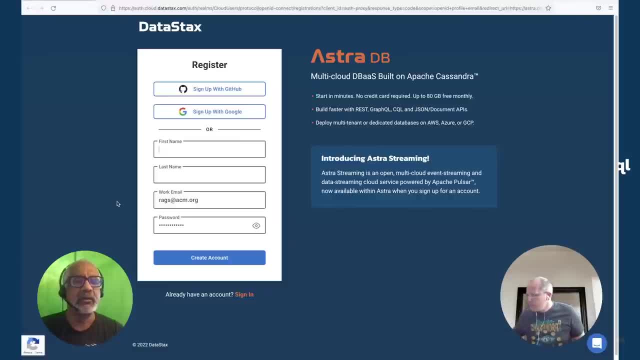 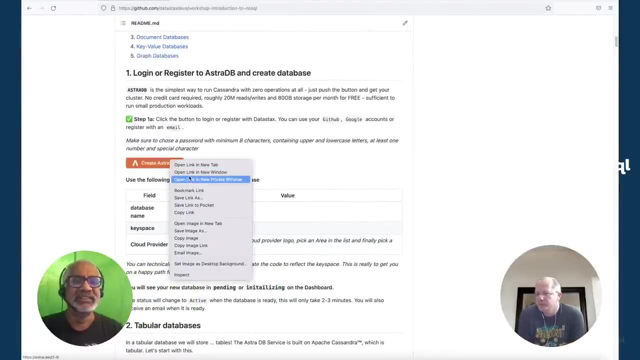 all that you need to do is put your email and your password. okay, because i've been here before um, you know it knows me um and i can. i can put it in right, but but you know i'm not gonna do that um. so once you um, actually let me do that anyway. all right, open link in your window, okay, and then um. 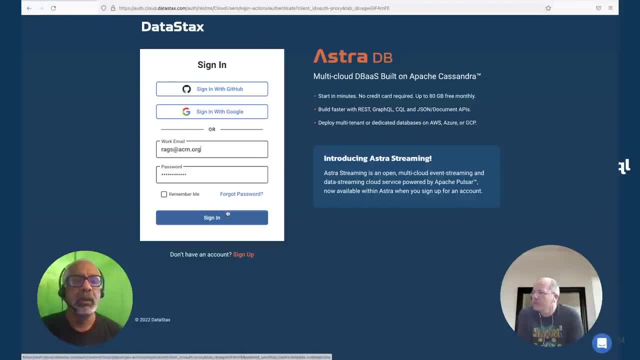 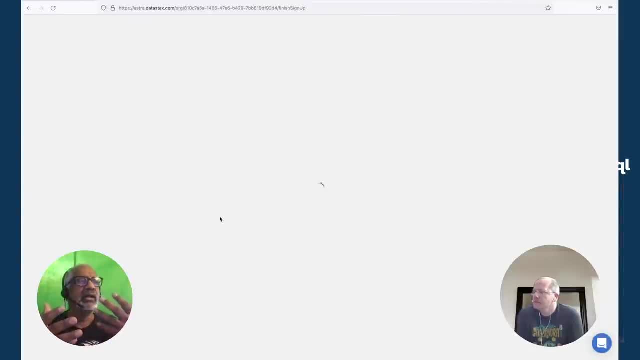 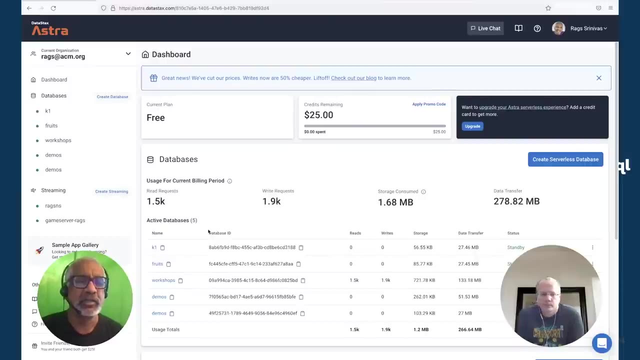 i just sign in, okay, so the first time around you may have to sign up. it may ask you a few questions about what kind of uh, um, you know, you know what kind of profile you are? are you more a developer? you know that kind of information, um, and then it will bring you into this. 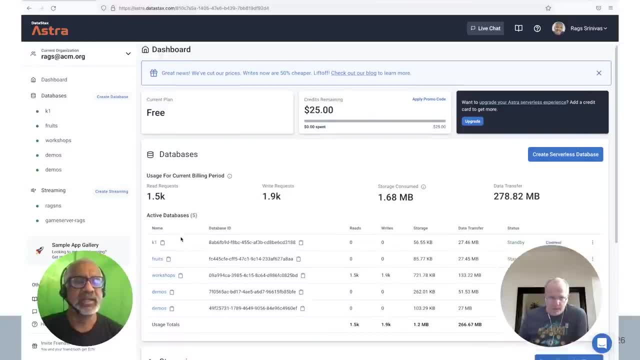 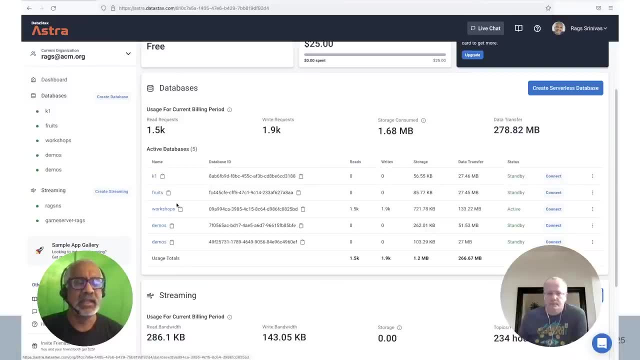 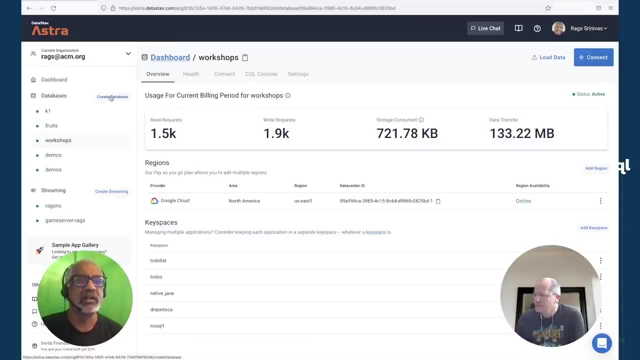 board. okay, so essentially, i have like five databases here and a bunch of key spaces in there, right, um? so, so what? um, as, as the instruction said, right, you're just going to workshops, right, and then create a key space um to be able to create a database. you just can create database. 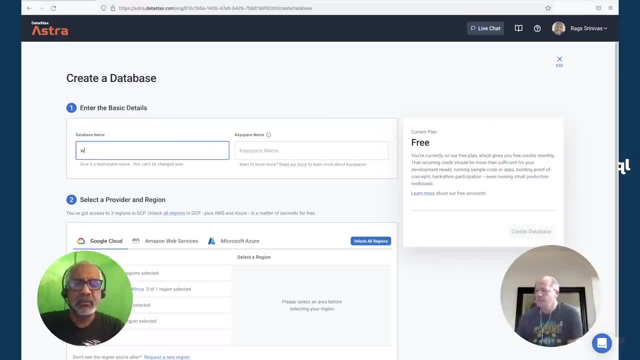 and magnus, you know, go through that here, but- but i believe it's correct me if i'm wrong- artem workshops and the key space is um. the key space is no sequel one. i've already done this, um, so i'm not going to go through this. 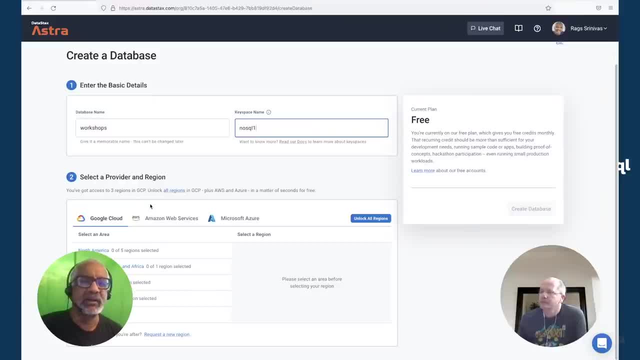 but you can pick any region, any provider, um, if some of those regions are not available and you particularly want that region, for whatever reason, you can just go and chat and ask. you know our folks to help you out. they will be able to help you out. or if you put a credit, 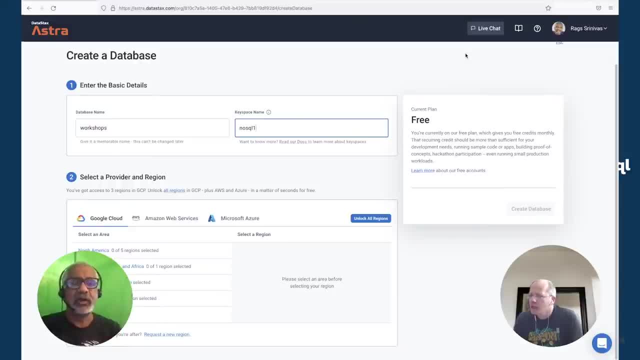 card. money always talks right, um, you can, you can create it in whatever region you want. uh, for now, what i'm, what we recommend, is just use the region closest to you. i live in north america, i live in boston, like i said, and, and either i picked the south carolina, uh, monks and march connor, um, or 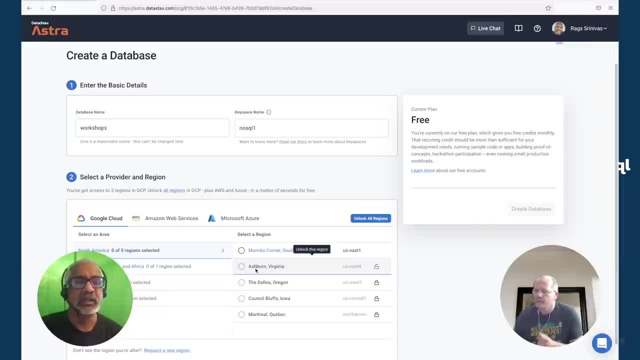 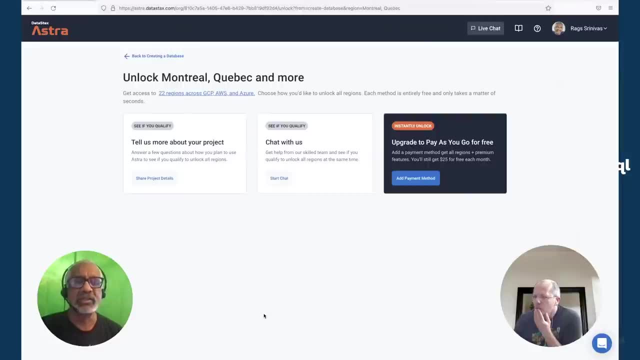 the virginia? um, ashburn, okay, ashburn, virginia one. i mean, really, you can, you can pick anything you want. you know, actually montreal is probably the closest to me, so i could pick this too. it doesn't really matter, okay. um see, like i said, there are some regions which are locked, so if you want to, 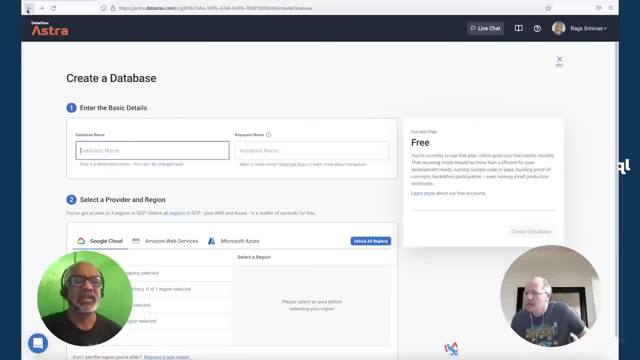 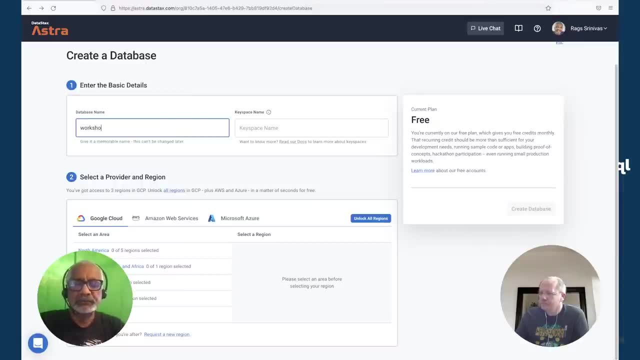 unlock it. you know you can check it out and if you want to unlock it you can just go and check it out. do that if you want, but but just pick something that's available and then, once you pick the workshops right and no sequel one yeah, and you may need to use. 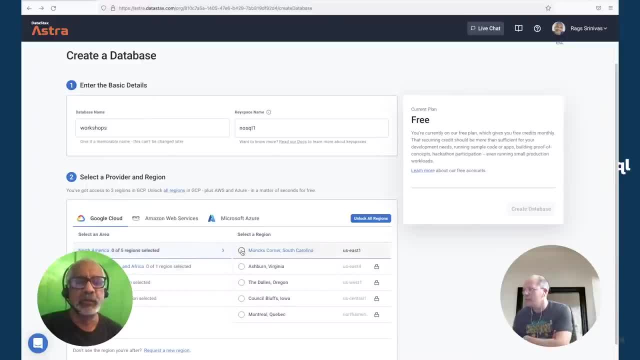 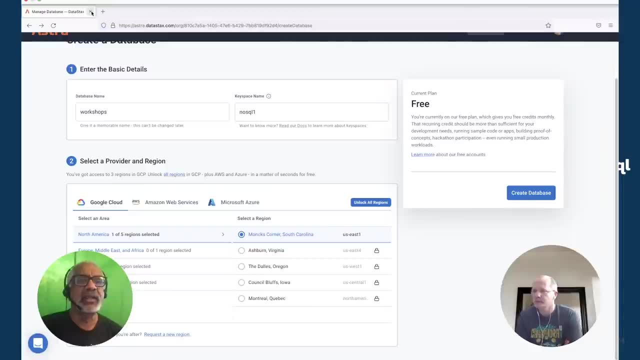 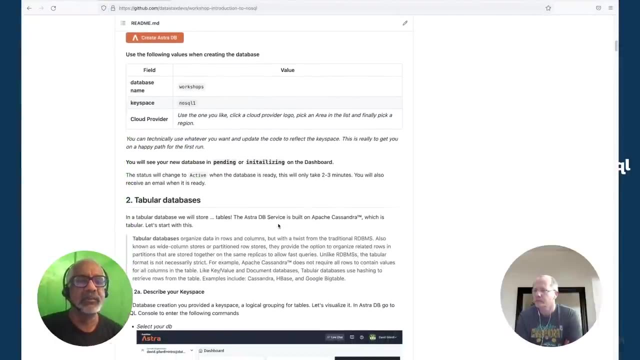 GC correct? yeah, because the other regions are lost. okay, so so what you can do is you can just pick this and then hit the create database and the database will be created for you, okay, so once you create the database- okay, let me get out of this- you're again going to be presented. you know something like this: 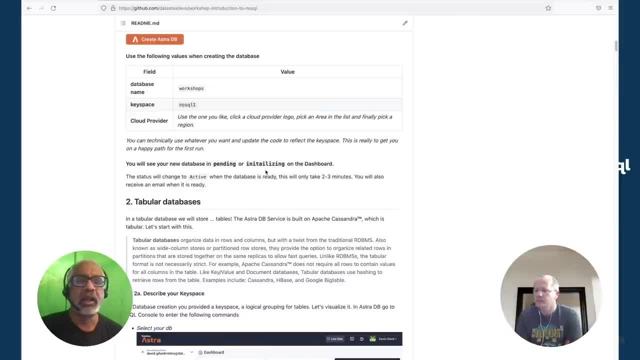 you will see a new database in pending or initializing on the dashboard. what we want to do is we want to make sure that you have set up the database and good to go. if you have already attended our workshops before you, chances are that you've already created a database. all that you need to do is, you know, make. 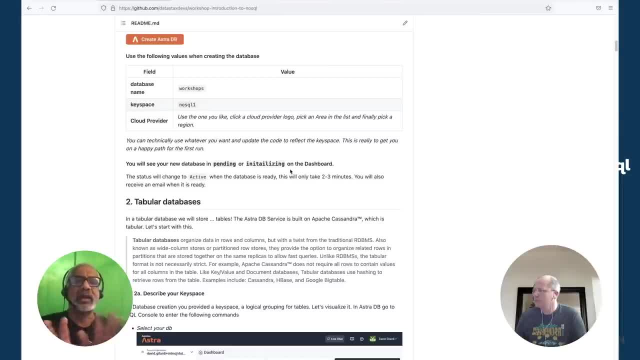 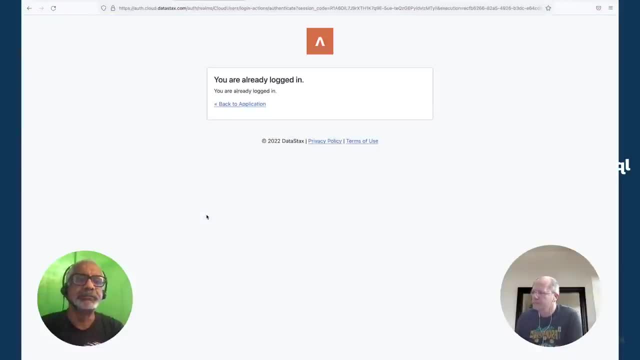 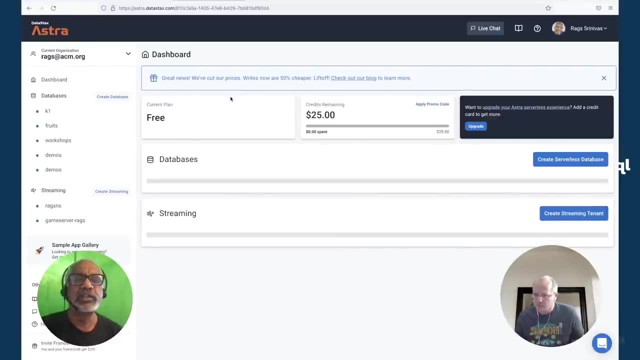 sure that it comes up. you know, and the best way to do it is now just go back into connect mode or something like that, and I can show that you in a second. so, basically, if I go back into so, I've already signed in right and you can see here. you know. 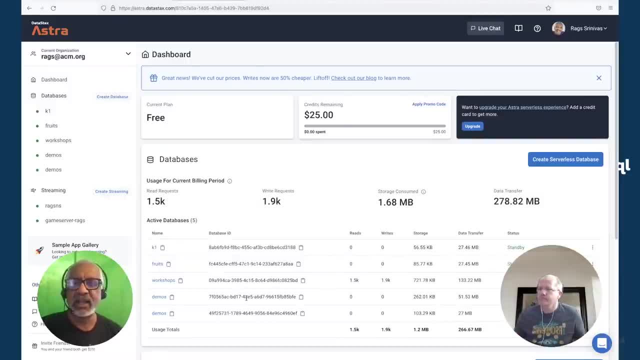 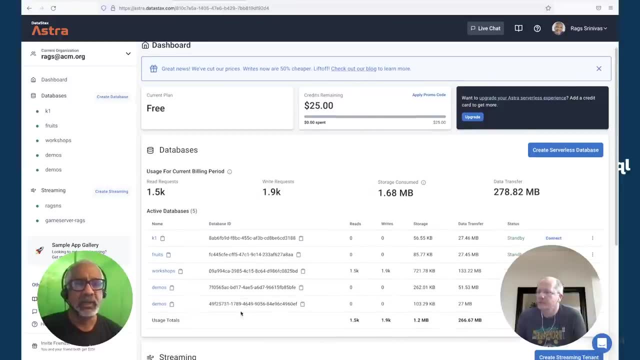 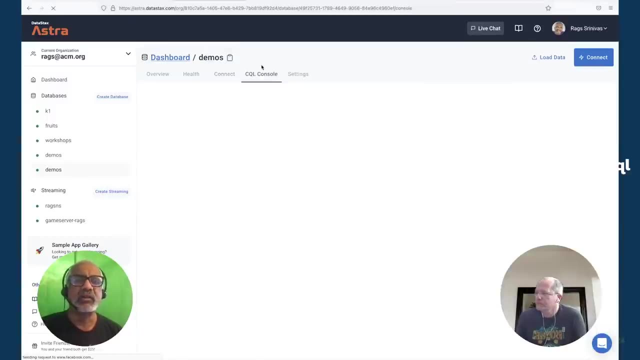 there are some of these in standby mode, right, so so let's say I want to activate this demos. okay, it really doesn't matter on. you know workshops is already in active mode, so it doesn't matter. so you can just hit connect and you can. you can just hit like a sql console or something. 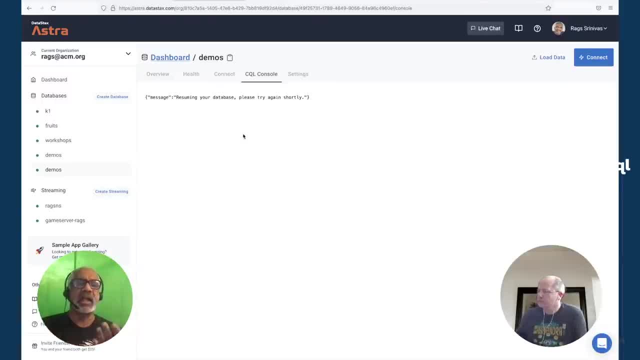 and hopefully it should tell you that it's it's resuming your database and if you go back you know you'll find it. but but if you're here for the first time, no worries. all that you're going to do is you're going to hit the create database, pick the region, um, make sure you have the workshops. 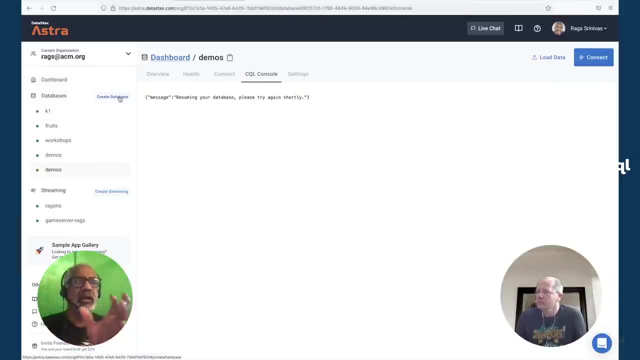 in the workshop and and no sql one in the key space. uh, i mean so workshops in the database and no sql one in the key space, and then you're good to go. okay, um, so let's see some thumbs up of uh people, you know, if it's still pending, that's fine. um, and, and then we can, you know, kind of go. 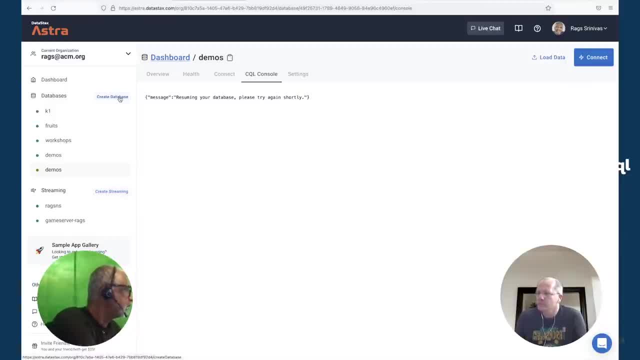 from there. all right, let's see some thumbs up. we generally tend to make sure that you know. we do a periodic periodic check to make sure that everybody is good. yeah, so we are doing. what we are doing here is just creating an, a empty database inside of astro db, and later we will create some. 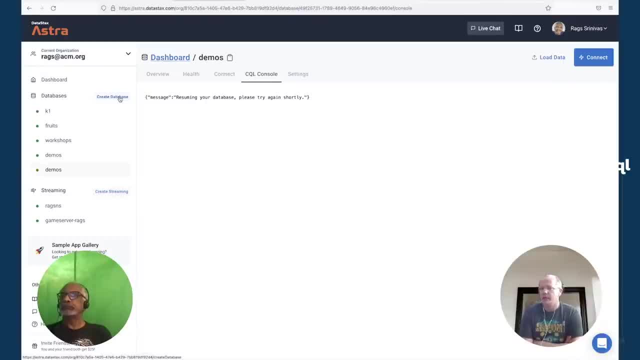 data there that will be either tabular or key value or document. so we will use three different types of data models to demonstrate how no sql can can handle those, because astro db is a multi-model database. we can do that and if you have time for graph, for graph that. 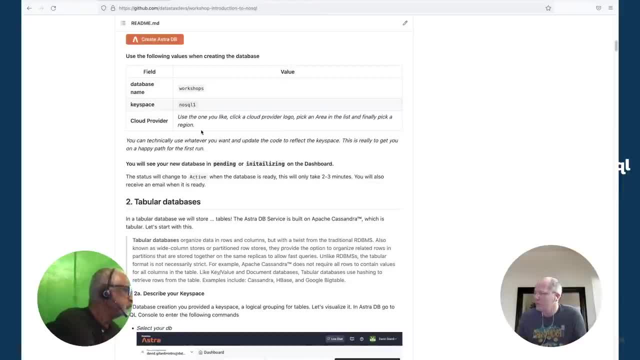 databases for the demo. i will also. we will use a different system for that, but right now you just simply need to create a database and it will take. so the. the message you are getting rags there in sql console basically saying that we're still initializing the database and yeah, actually, actually basically what it was. 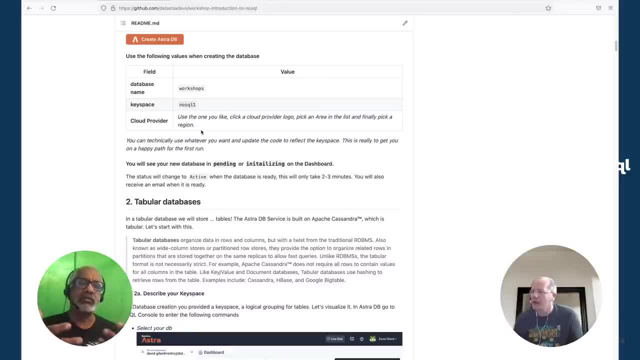 was in, it was in hibernation more, uh, because what we do is we try to, um, you know, basically save some dollars, right, and and that's why we hibernate and and keep it ready, uh, but if you're creating brand new, it will start impending and then it will go into active state. okay, and you will see that. so 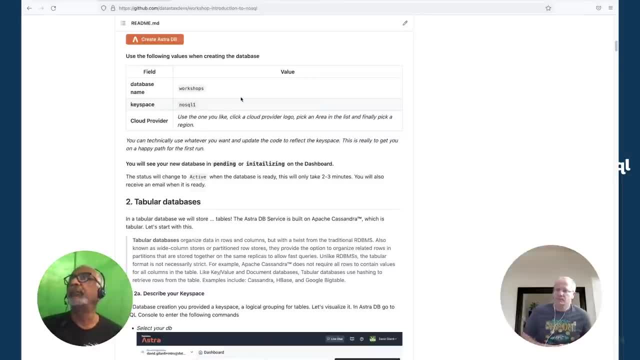 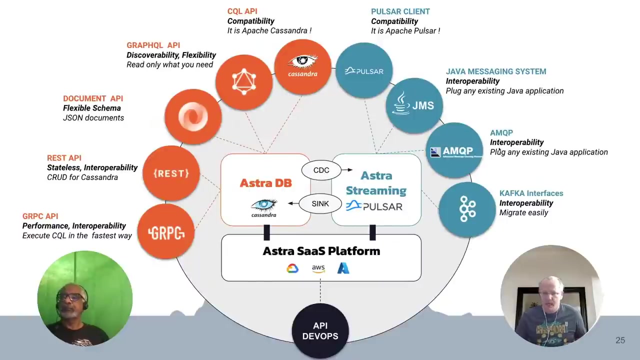 we see a lot of thumbs up. that is. that is pretty cool. um did. was i supposed to go to the tabular database, or is it? um, yeah, give me a second here. if you give you this control back, all right, you're good to go, sir, okay, so, um, so, what you just did is created that database in astro db, and astra itself is a is a. 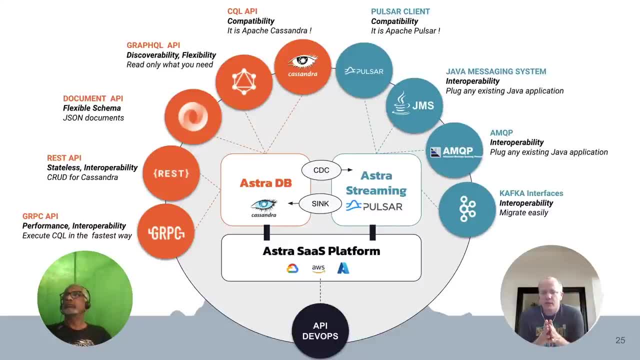 platform currently has. it has two services: the astro db database as service and also astra steaming as a service. astro db is based on cassandra, which is apache- cassandra open source, and it supports many different apis. we will use several of them: uh, today and uh. if you're interested in streaming, then then um, astra streaming supports is based on. 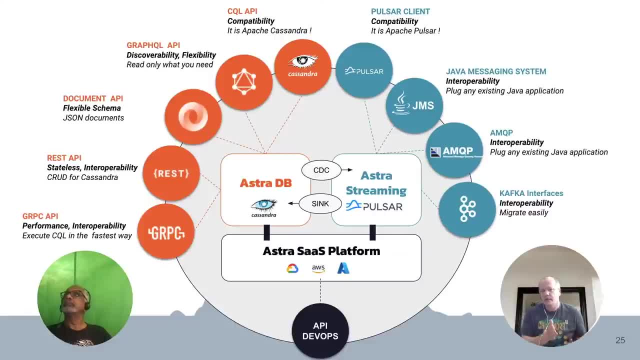 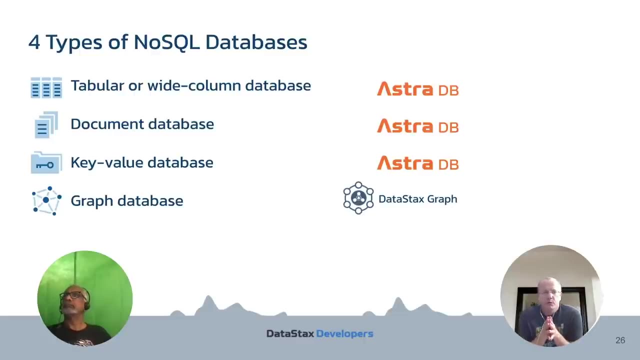 apache pulsar, and it's also compatible with a number of systems like, like kafka- maybe you heard about it. so that's something that you you may be interested in exploring in the future, but today we're going to focus on these four types of most equal databases. we use tabular. we'll create tabular. 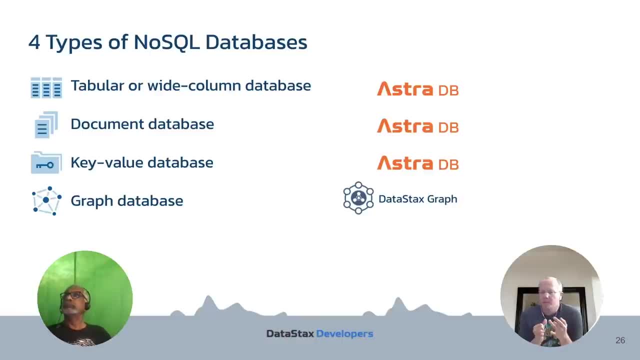 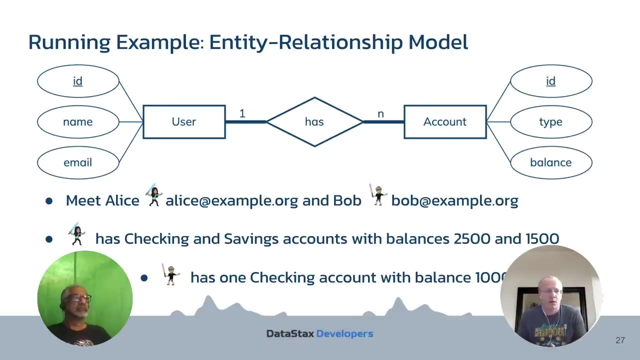 database. we'll create document database, keyvaluer database, all in astro db, and we can also do the graph database in using in in data stacks graph or. if we don't have time, then we will leave it as a homework. okay, so running example, so i'm going to demonstrate you how those data models work and 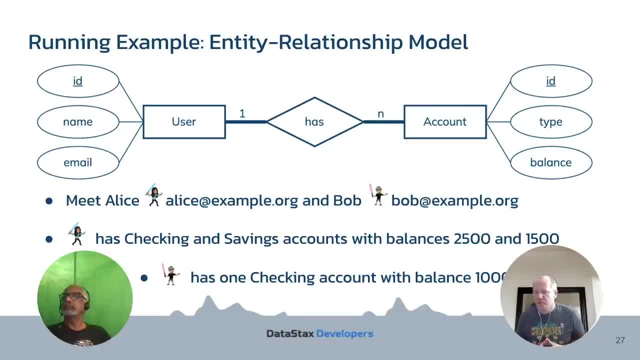 the running example is entity relationship model here which has- uh, it's very simple, users can have, user can have, multiple accounts and accounts can belong to. they always assign an account assigned to to one user. user is uniquely identified by id. has name and email account is uniquely identified by id as type and balance. so people familiar with relational this is should feel. 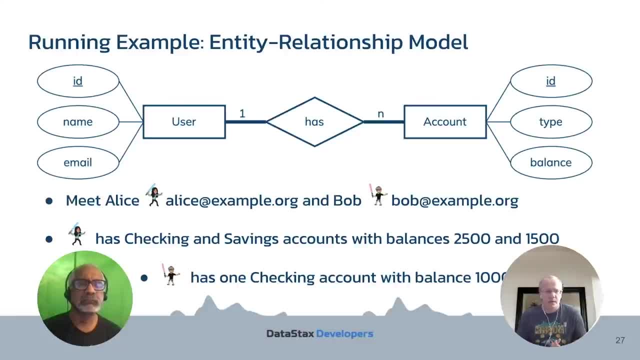 right at home here we use this example with two basically two users alice with email that particular account will only copy inside the id and account so when the uh the data is added the anti- compos ID indicates that the data is stored with the matching port on the oilÿ 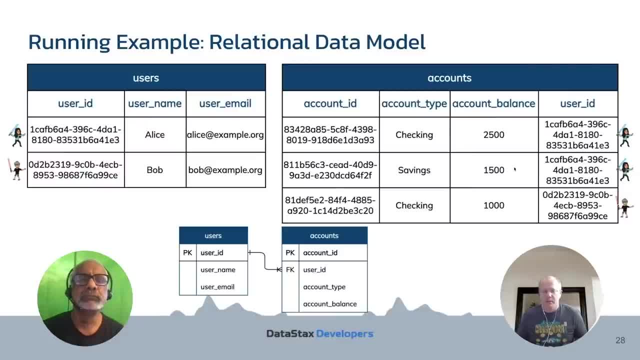 need and alice will have two accounts, checking and savings, with balances 2500, 1500 in some currency, and both will have only checking accounts. so how will this look like in relational database? first, right, so for relational database. uh, there is another er small diagram here which basically 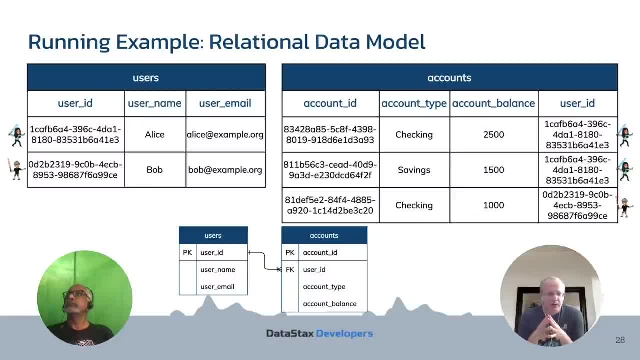 users table with primary key user id. accounts table with primary key account id and user id is also added into accounts table. it's a foreign key which references user. this is this is how relational database would store and whenever you need to retrieve accounts of alice, you will have. 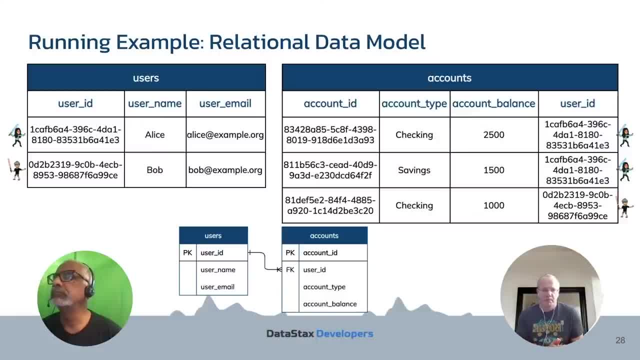 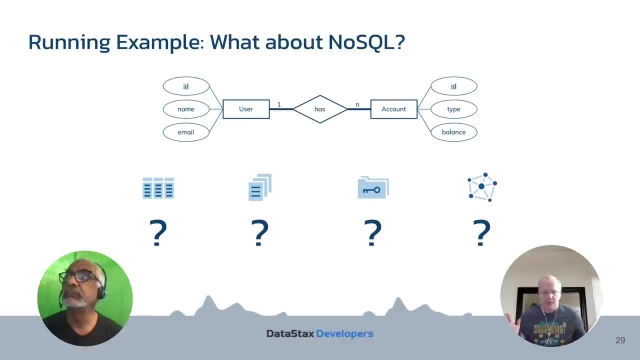 to join users and accounts using user id, column right, so they will be joined, involved there to retrieve that data. so our question, big question, uh, actually four questions. how are we gonna store the same data using tabular- no sql- in document json, using uh key value and using graph? 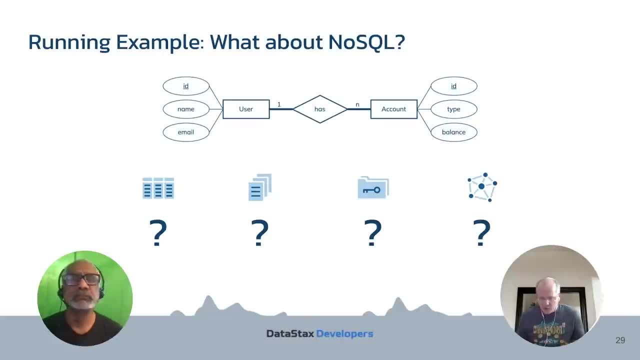 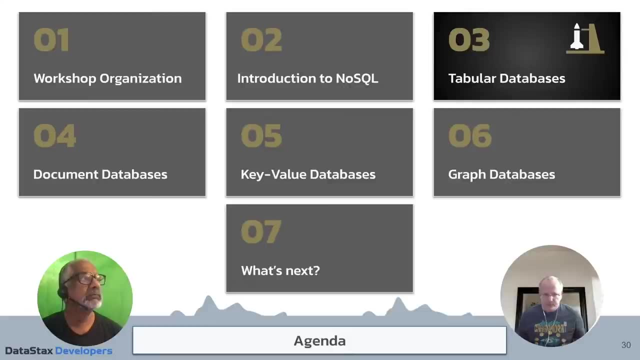 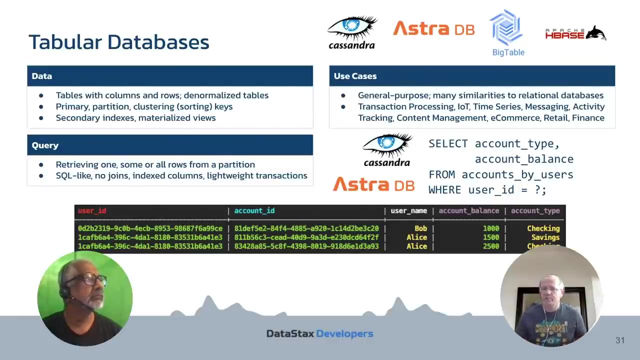 and this is what we're going to talk. for each of those types we're going to use the same example, starting with tabular. so what is tabular databases? some examples include cassandra, astro db and bigtable and apache hbase. so tabular devices use tables with columns and rows. should be quite. 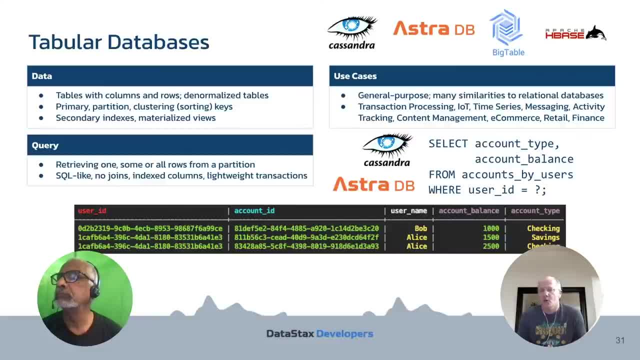 familiar. they are closest in similarity to relational databases. they, however, they do not normalize tables. they use the normalized tables that are designed based on queries that they need to support. another difference: besides the prime key in the table: they do not have foreign us, so log and a cross. 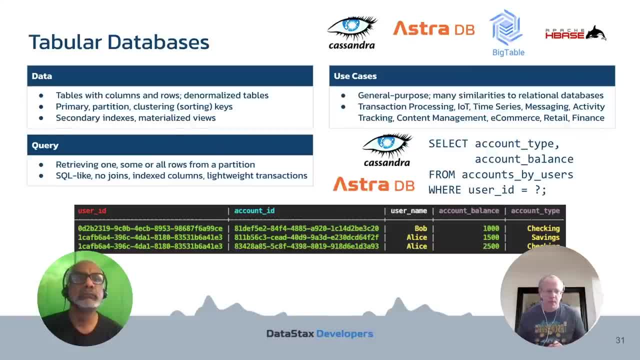 and r of those rows within a partition. So in this example we have here, we have user ID, user ID, account ID. So user ID is a partition key, account ID is a clustering key And together they form primary key in Cassandra or AstraDB And you can see that basically, user ID alone cannot be a. 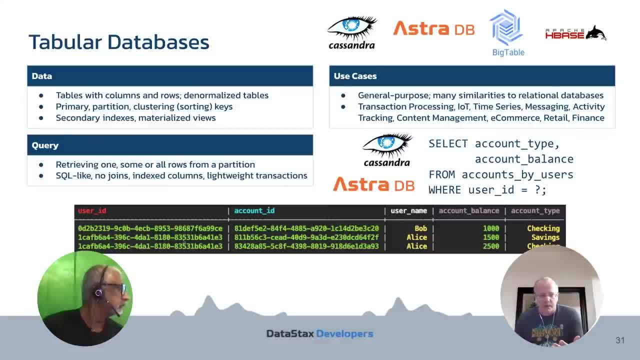 primary key. It doesn't find uniqueness here, right, Because there is a repetition, But together with account ID they can be, can form a unique primary key. Okay, In terms of creating tabular databases, you can retrieve efficient, very efficiently. you can retrieve one row from a. 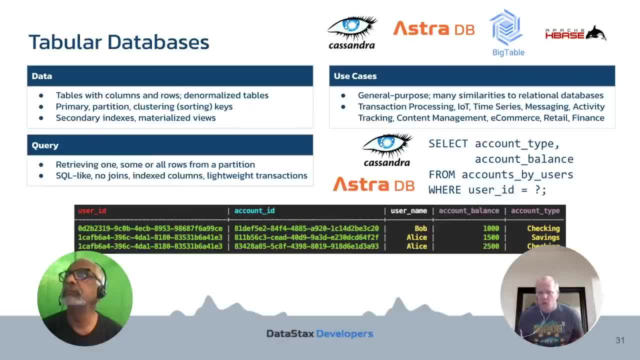 partition, subset of rows or even all rows in a partition. So retrieve one partition. So this is done based again on primary key, partition key, clustering key, And. but there are of course secondary indexes, materialized views, if you need them, And the language, and there are lightweight transactions. 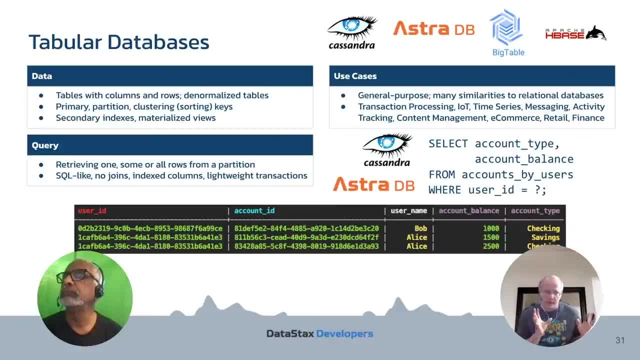 And the languages that are used to create are usually SQL-like. They have select from where just shown here. This is Cassandra query language, where we select account type, account type- and then we select the query language And then we select the query language. 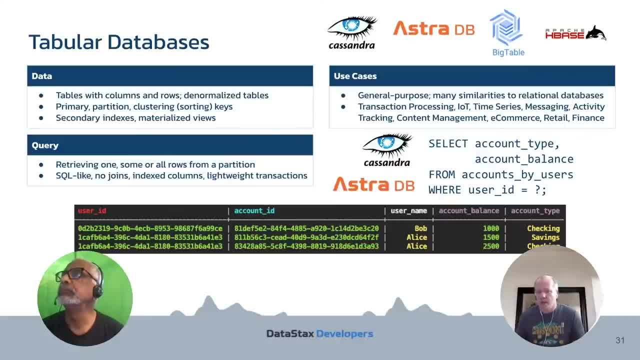 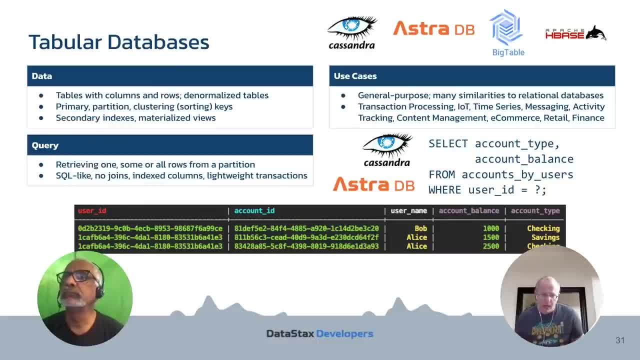 joints, but you can at them. you can first of all. if you understand how joins work well, you may be able to do something in the application itself. But there are other frameworks you can add, like again Spark SQL, for example. 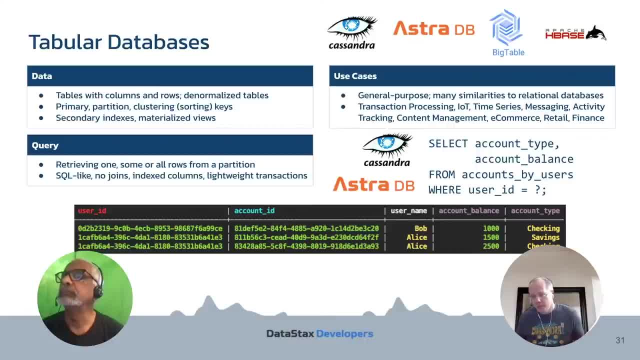 add joins, but they still will not be super efficient, So they are not for OLTP transactions. real-time processing Use cases. This is a general purpose database. It basically handles many cases that relational databases do, but those use cases where you actually need scale and 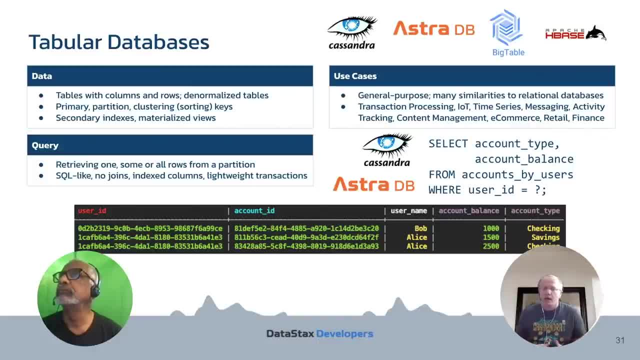 performance. So transaction processing, IOT time series, messaging, activity tracking, content management, e-commerce and so on and so on, So that basically all types of different industries will have an application nowadays, because we collect more and more data for each individual person. 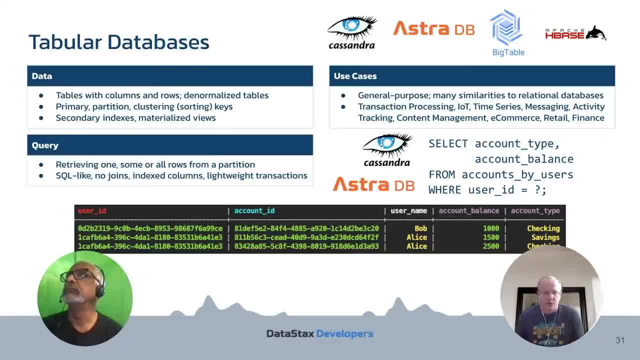 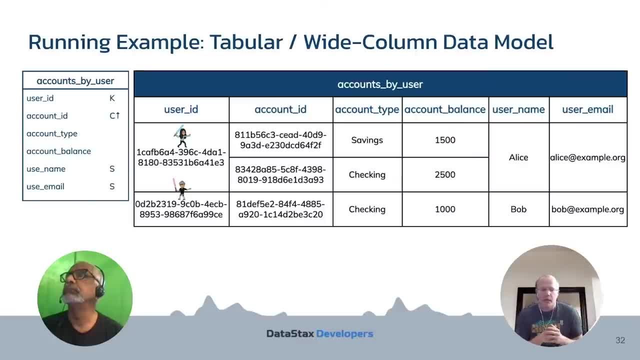 for transactions and so on. Okay, Okay, Okay. So, running example, how are we going to present that data that we had for Alice and Bob? So here we have kind of a schematic definition of the table accounts by user, with user ID as a partition key, account ID as a clustering key, and you can see there is 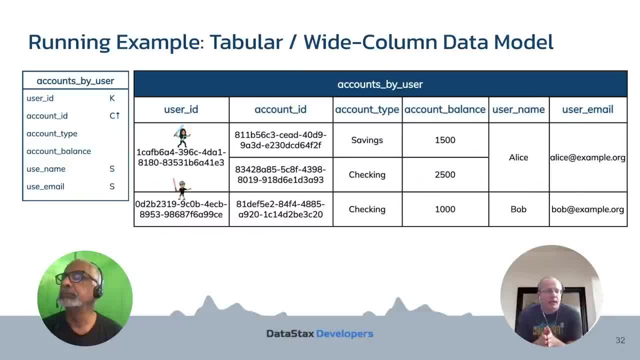 error, so it's sorted, Okay, And then account type, account balance, just regular columns. username and user email: It's recorded. if you want to change it right, And your name is your first name and if you want to change it you should enter that formology. 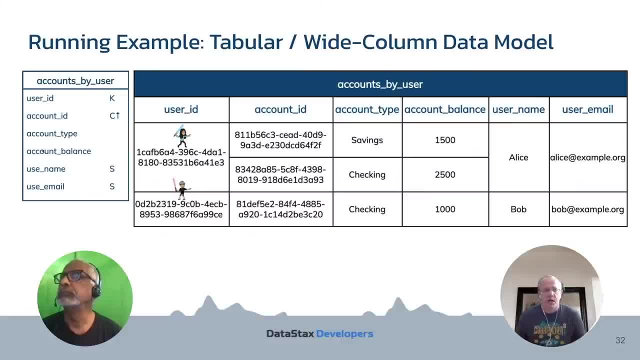 So you should be talking using a custom version of the code. Okay, So when we use partition key in a article chart, that's the 1990s, but many people think we do it this way. you'll see some fans talking about data files, So let's have a look both in the article charts and and in the catalog chart. 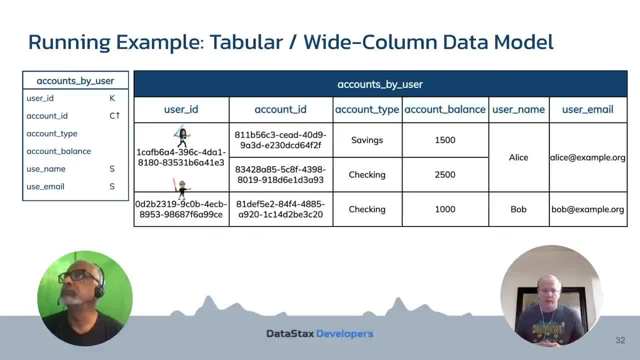 retrieve both of them, because they will be collocated, stored together. For both we only have one row, but you can see this static column, ellis and email. These columns basically belong to partition rather than individual rows, So what you may have noticed, here we only needed one table. 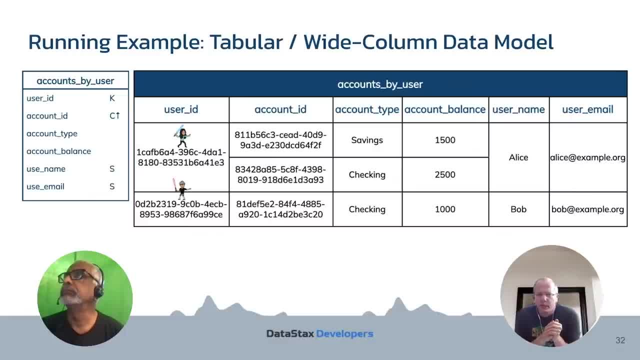 here right and we didn't do much duplication, denormalization that we usually talk about when we talk about NoSQL, because it's not that it doesn't always have to be a lot of duplication and denormalization. So what this table was designed for is to support specific query. 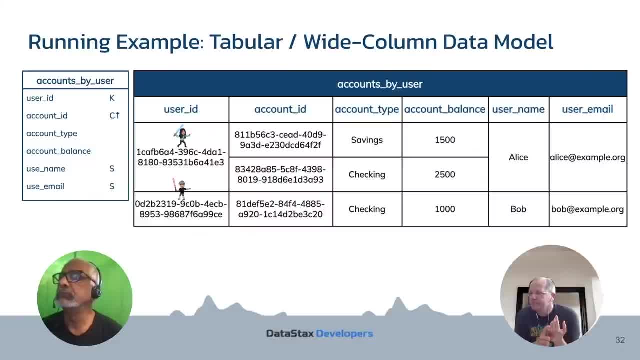 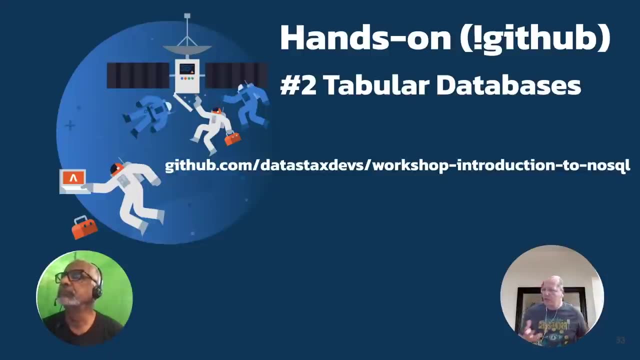 retrieve all accounts for a particular user. okay, all accounts for particular user. it can do it very efficiently. So, no two tables, just one table. there will be no joints, because we do not support joints, and with that said, we have second hands-on where you can actually create. 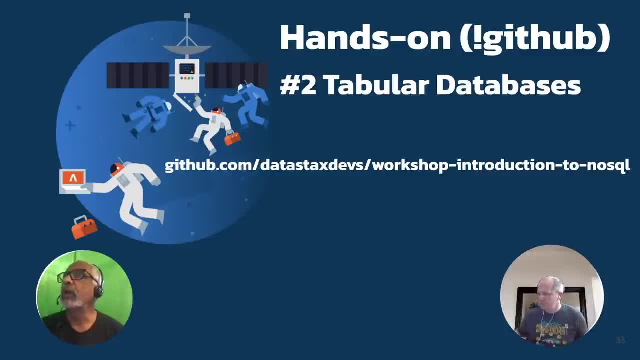 a few, a couple of tables in astro db. oh, okay, before i jump in the hands-on, i know there was a question from programmers away: what is the key space? um, you know, really a key space is a is a logical container, if you want to think about it that way, um, where you kind of group tables together. 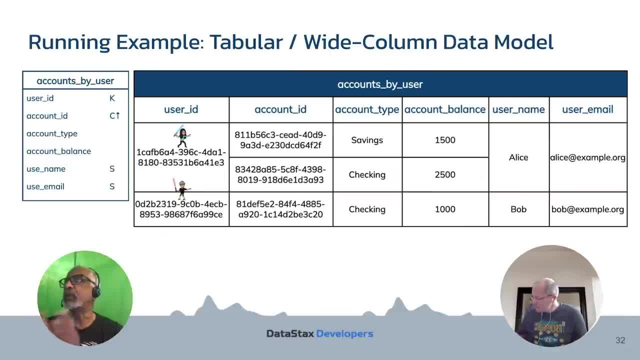 so that's really what a key space really means. i don't know if you want to add more color on that and i will get to that in a second, but but you know there are other things that i think you know. you know we, we have a saying within data stacks which is: like you know, friends, don't let. 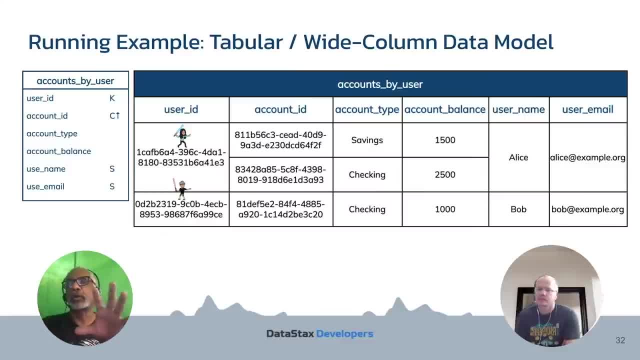 friends. shard, you know, i think artem talked about uh like partition key and several different keys. uh, you know, typically from a sql world, you know from a relational world, you're you're aware of primary key, but but in, in the no sql world, um, actually the partition, 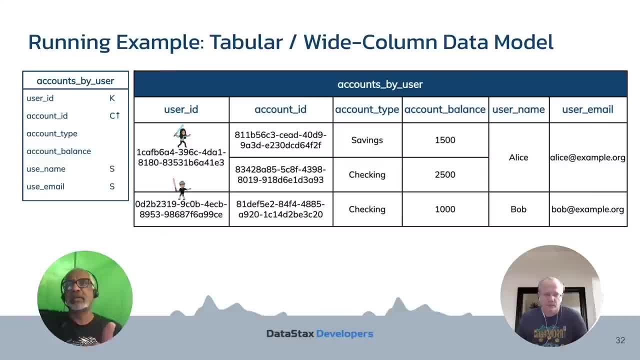 key is very critical because that is how the data is distributed. you know, if you want to think about data being distributed across different nodes and all that, it's based on the partition key and then within the partition- um, you know, you have the clustering key that, uh, that artem talked about. 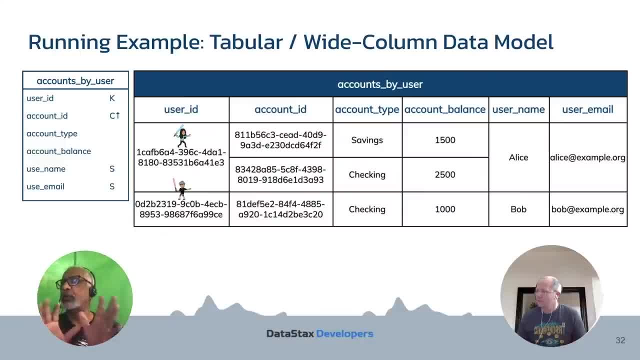 we have an entire workshop, you know, devoted for that, so we don't, we won't have too much time to talk about that, uh, but but if you want to add a little bit color, uh, artem, uh, feel free and i will set myself up for the next exercise, yeah, so so what? this is just introduction. 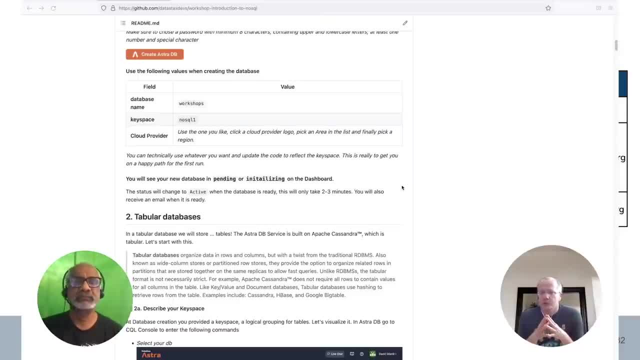 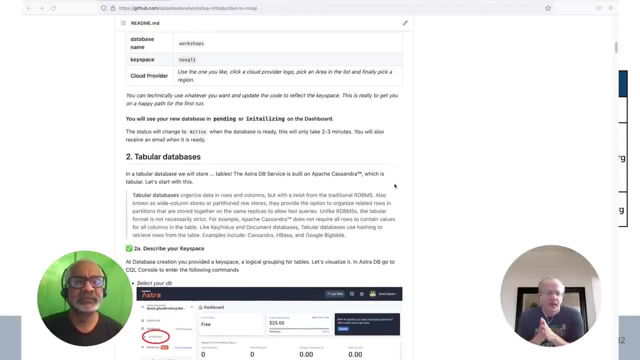 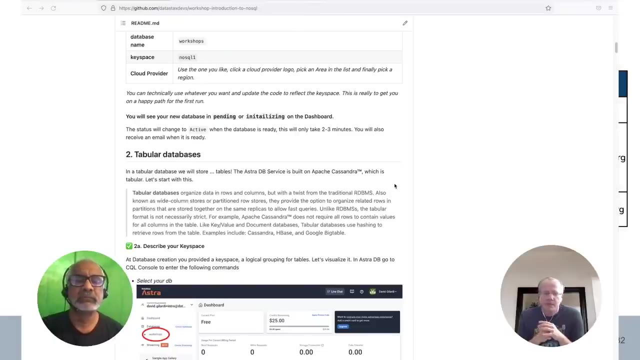 we have two slides on tabular. that's. that's not enough to to become like a super fluent in the tabular databases in no sql. also, white column, uh data model, so. but what you can notice is you're still using tables, you're still using columns and rows, but there is there is a primary. 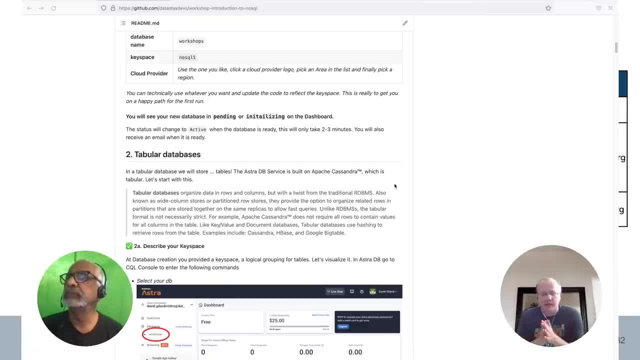 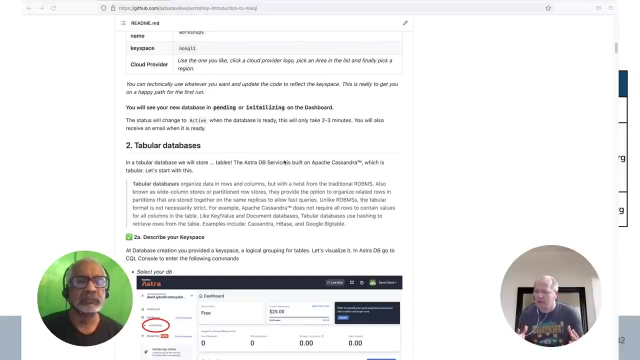 key, but there is also partition key and clustering key and what what rex said is true and it's right, but we will need much more time to explain them better: how partition key does the, how it affects data distribution, how clustering key can be used for sorting and for adding, for guaranteeing uniqueness of a primary key, and all of that. 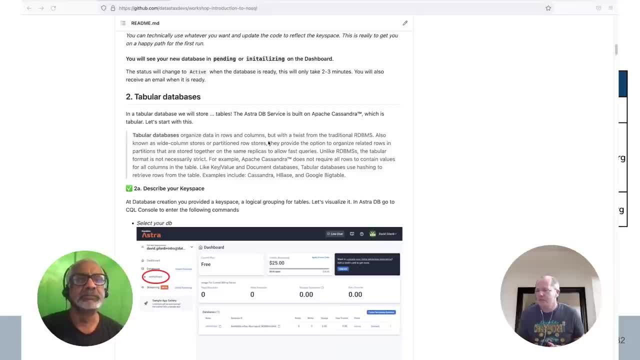 so, for now, just realize that it's just a table, it's just like relational, with a few important differences. so one other things i wanted to mention here: the user id and account. they look, may look, strange. these are: these are so-called universally unique identifiers. they are generated, uh, automatically by the system, uh, by an application, uh, the reason why you want to. 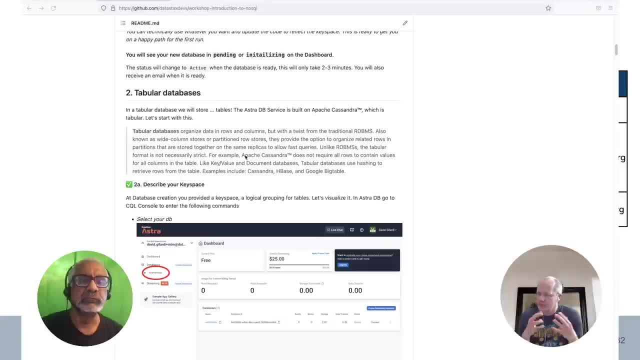 use uuids universally unique identifiers, because this is distributed system. you cannot just do like auto increment or something like that. intellectual perfect. so again, i know that you guys can't wait to get to. you know, get your hands dirty, right? uh, go back to same github link, you know? if you don't know where the github link is, just 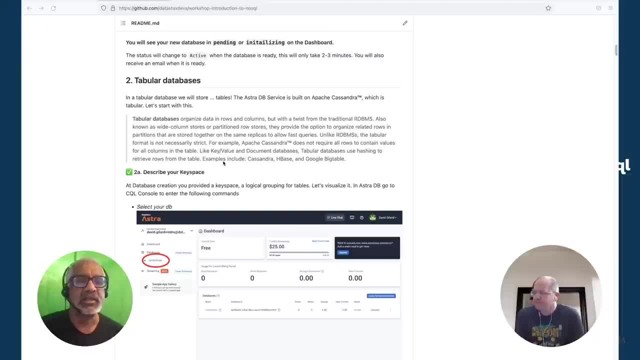 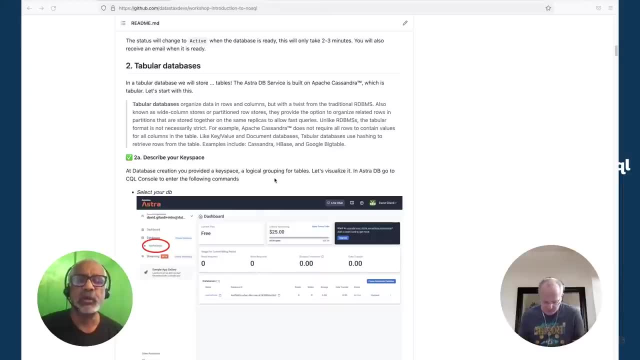 hit exclamation github and you should be the first question that it's going to tell you. i mean, the first answer to your question is going to be: what is your key space? is key space, as you can see, is a logical grouping of tables. okay, so let's go and visualize, uh, visualize this using what is. 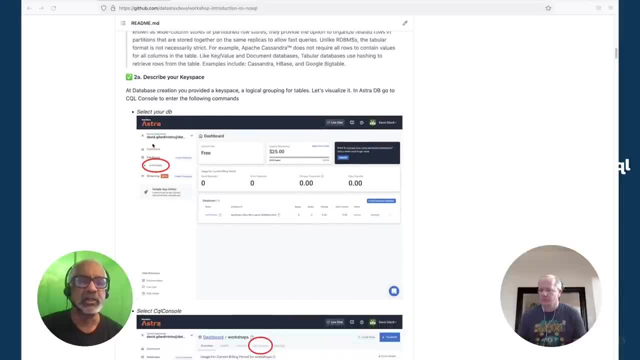 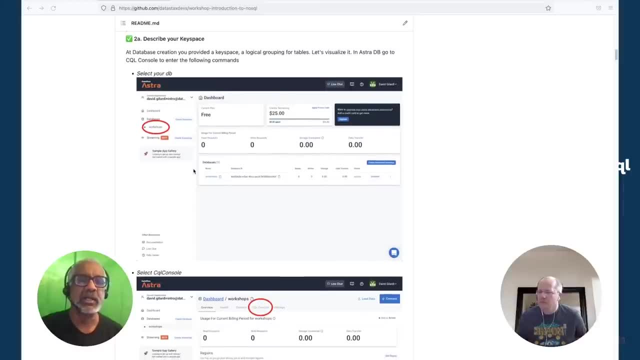 referred to as the sql, which is the cassandra query language console. okay, and, and it walks you through each of this step very clearly, okay, so you're going to click on it and you're going to click on workshops, which is your database. okay, and then click on sql console. you know which is the console? 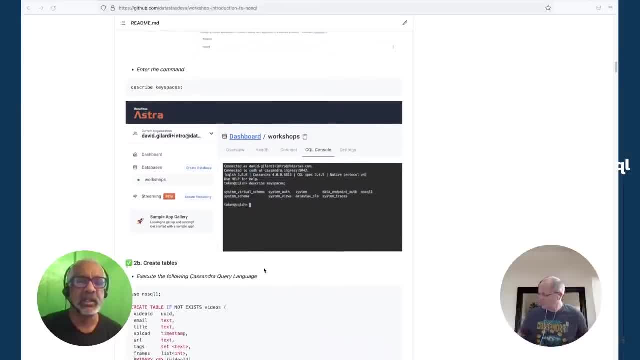 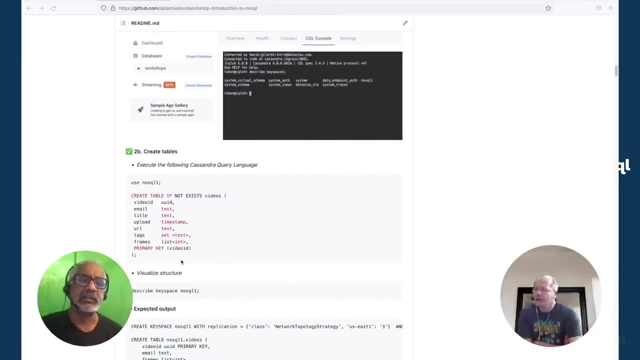 and it brings you, brings you into something like this: you know which kind of looks like this, okay, and then what you're going to do is you're going to use no sql 1 and then start creating your tables. okay, so let's do this one step at a time, right? so let me click on workshops. okay, 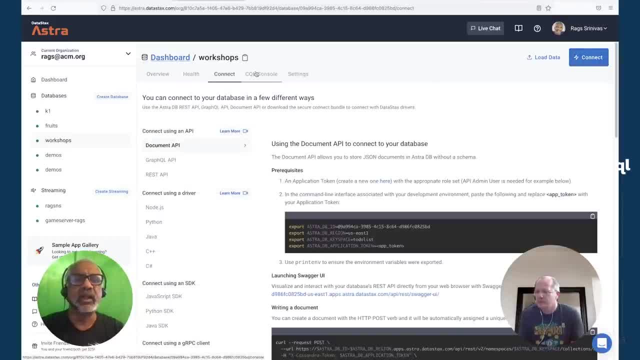 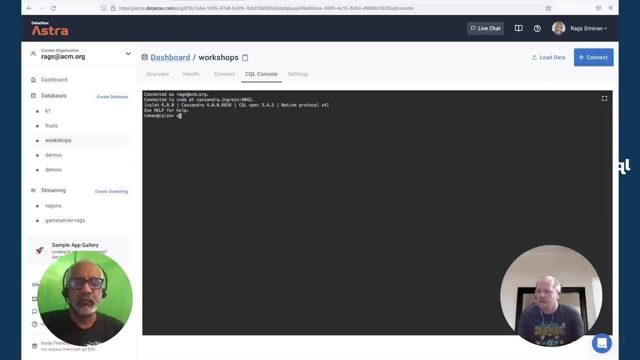 and then what i can do is you can hit connect okay, and hit sql console, all right, and this should bring you in in here, okay. and what you can do is you can just do a describe okay, and i've already created this, so it might be a little different for you. 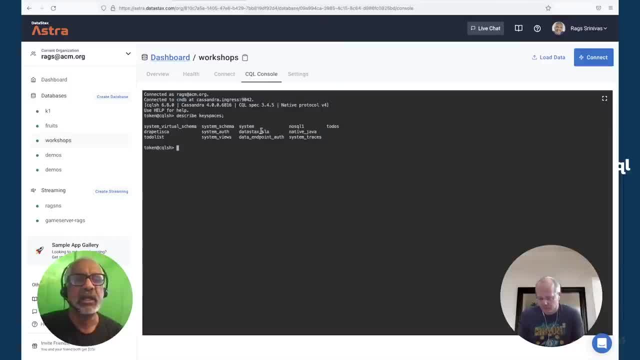 but if you just do a describe key spaces, you will see here. you know i have a bunch of stuff here. okay, this was for last week's workshop. um, i have some for tomorrow that i'm getting ready for, uh, but this is the key space that you're gonna use. okay, the no sql one, uh, and actually, if you have, 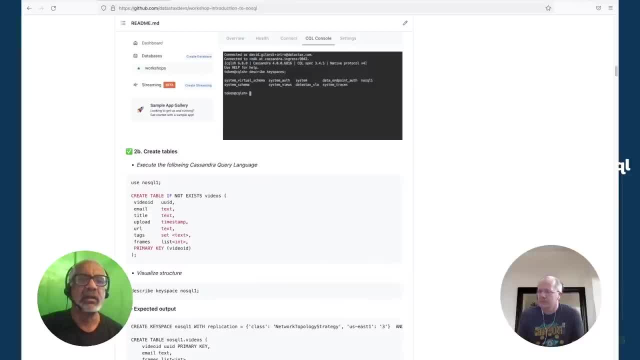 not created a workshop yet it before you will create it. um, very simple, you know: use no sql and then start, uh, creating the table. um, if it uh, if it does not exist- and it's always a good idea, it's always a best practice to create a table, if only if it does not exist. right, so that you know. 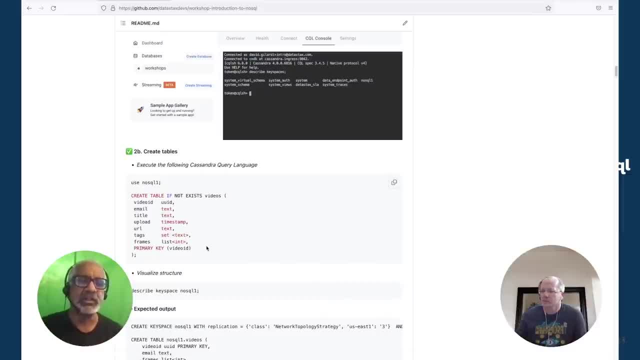 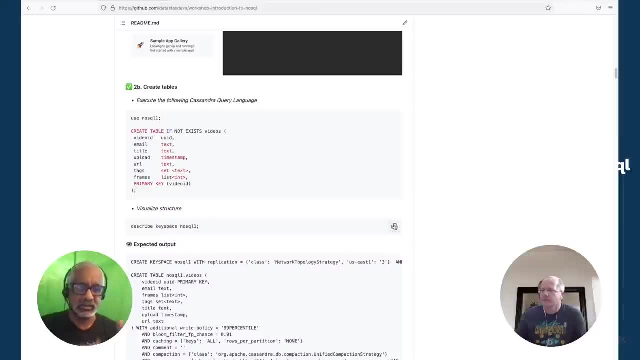 you're not going to overwrite something that's already there. um, always a good idea to do that, okay, so now let me go in and describe the key space. no, sql one and again. all that i do is take this from the instructions and put it in there. okay, so if you hover over here, you 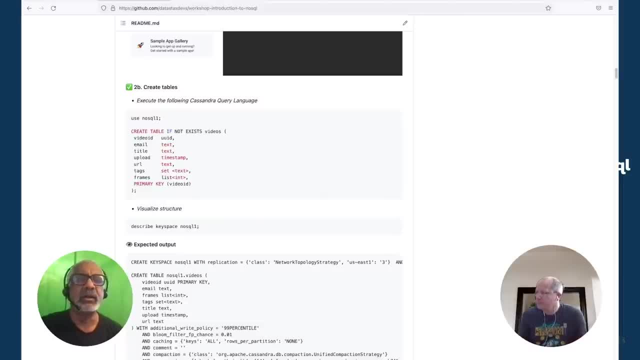 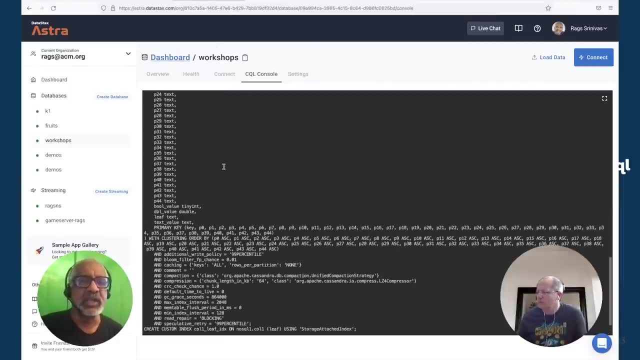 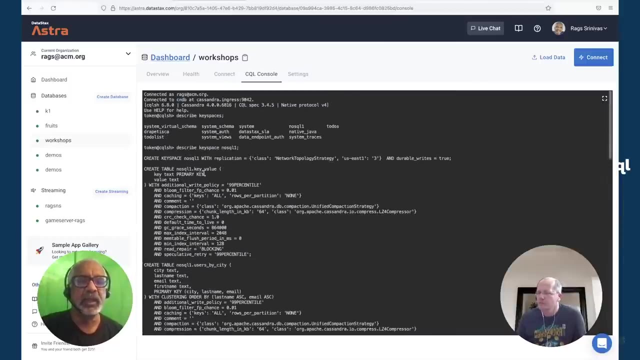 will see like a you know cut and paste and you're gonna grab that and use that here, okay, so if you describe the key space, okay, um, it will, it will tell you, um, you know what, what kind of um you know. it will give you more information on the key space. okay, so there are. 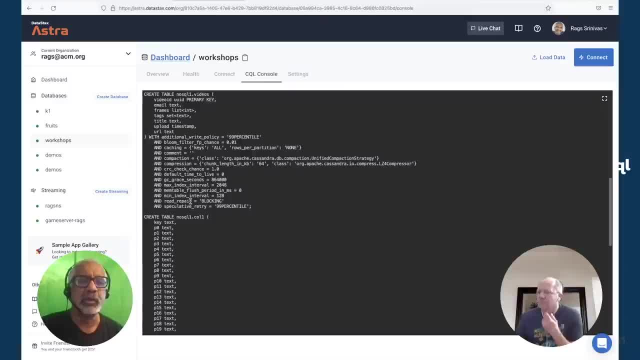 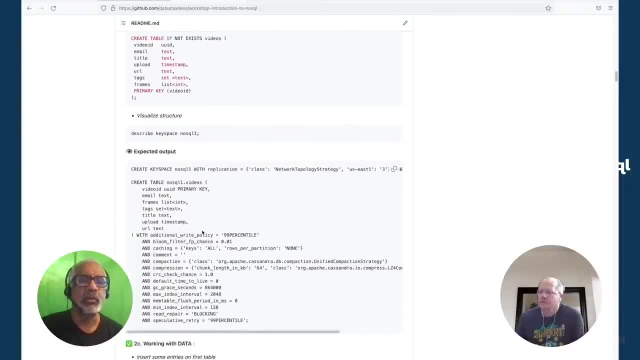 different tables that have already been created. the first time around you'll be probably won't have any, so you don't need to worry too much about that. so you will see something like your expected output will look something like this: right, you just have just the videos. you know the videos table, okay, and you have 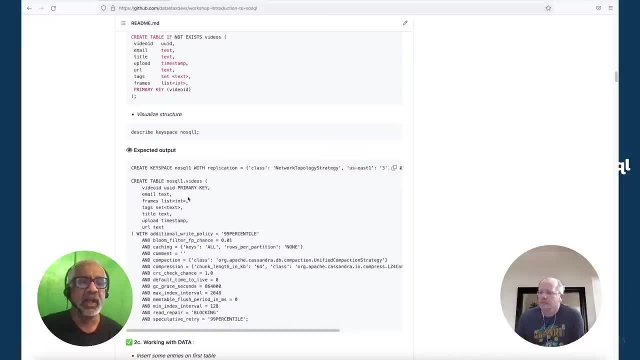 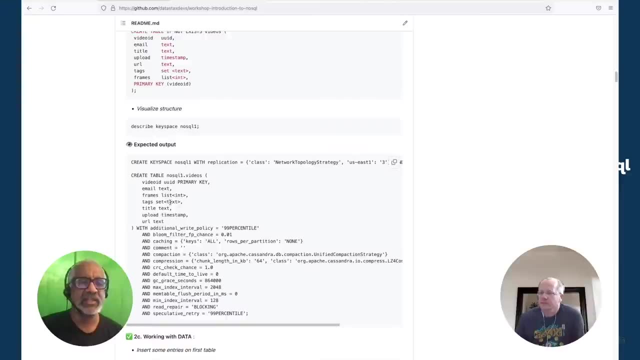 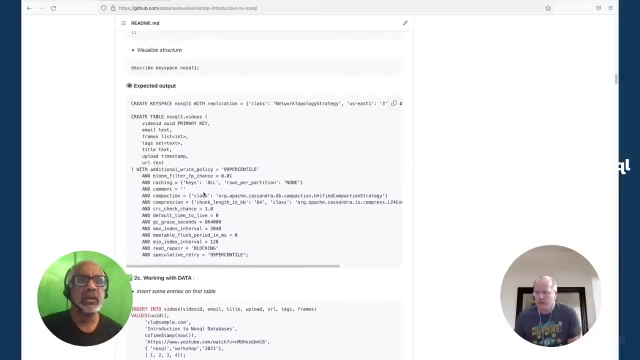 the video ID is the primary key right, and then you have text, you have a list of integers, which are frames, and then you have tags, which is a set of integers, and so on and so forth. okay, and you will see here, you know that that essentially the the partitioning is going to be based on, you know, the video. 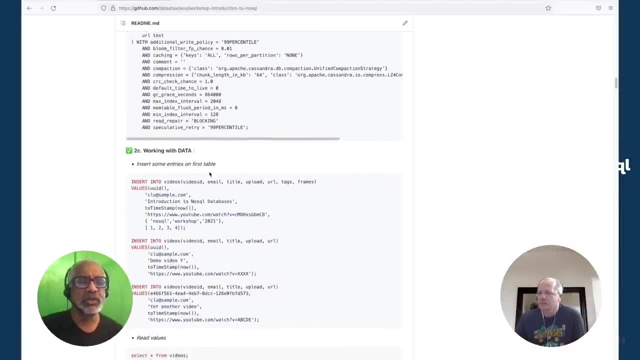 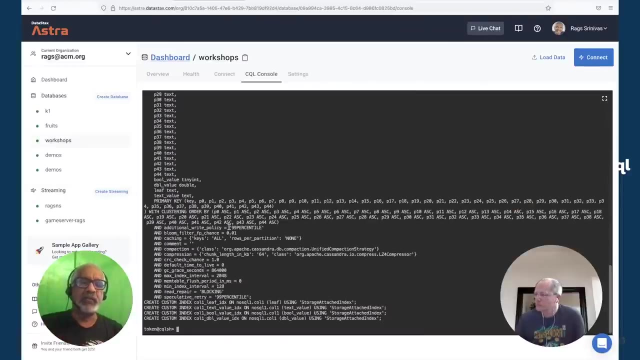 ID. okay, so. so what you can do is, you know just again, basically grab from here and go into your sequel console. okay and again, if you can, if you can wait for a little while, and then you can go back to your SQL console. okay and again, if you can, if you can wait for a little. 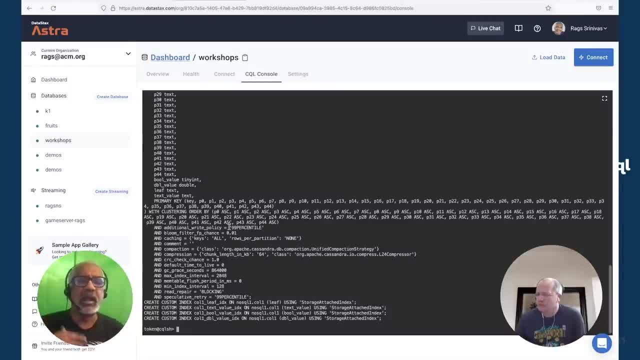 bit and not get started. you know, listen to me for a little bit, and after that we'll turn you loose, and then you can give us some thumbs up, okay, so? so now what I'm gonna do is I'm gonna go to the next step, which is really what I'm doing. 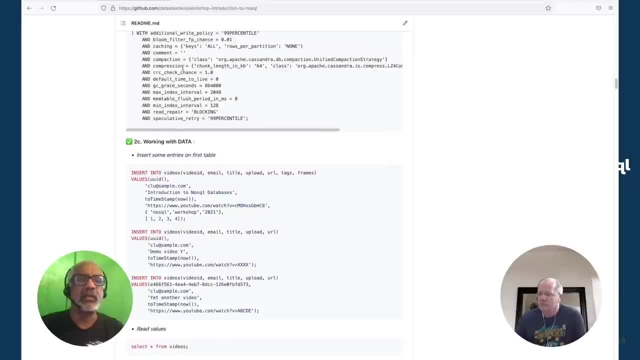 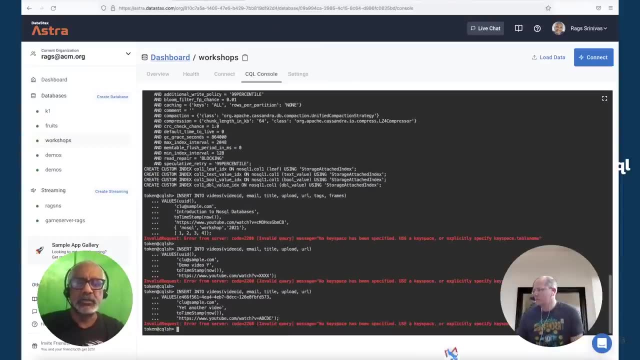 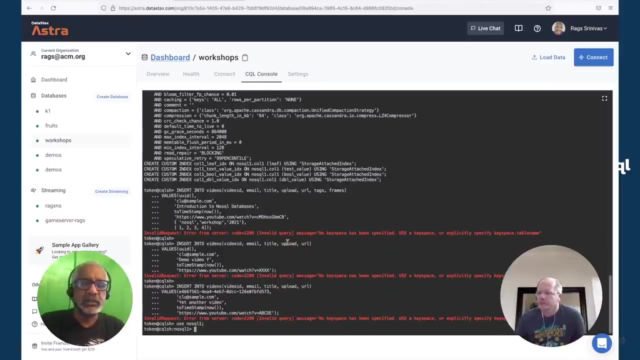 is, I'm inserting some entries on my first table. I mean I've already inserted this, so hopefully you know it should. it should work fine. okay, key space has not been defined, so so use right. because I didn't use the key space, it gave me an error, so just do the. 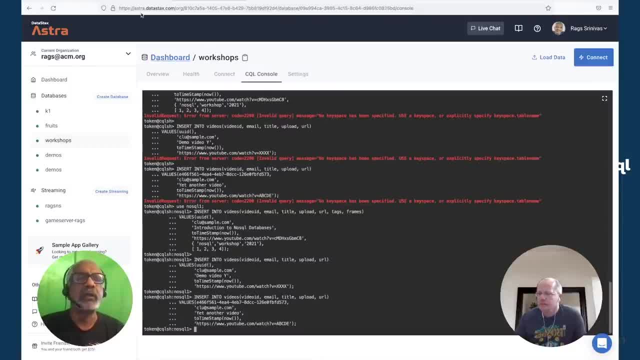 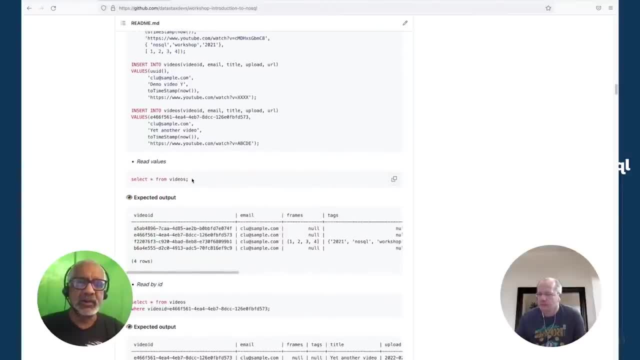 same thing now and you will see that it's been inserted. okay. so once it's inserted, we we don't recommend this for your actual production, because when you say select star from videos, you're actually going to each of those different partitions and pulling data together. it's always better than. 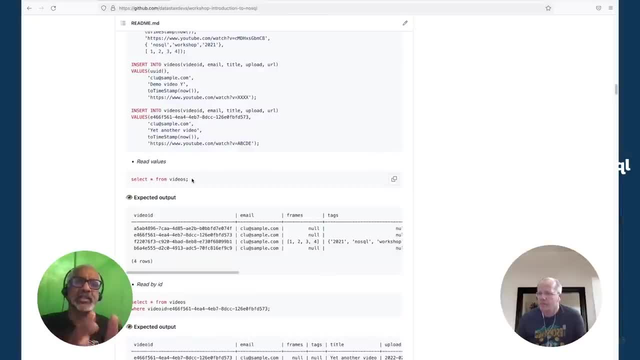 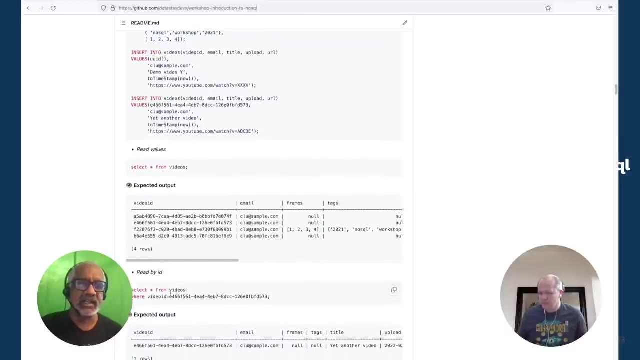 always recommended to go to a partition and and get the data from there, rather than go to every partition, right? so typically what you would do is you would select star from in your table and specify the primary key. okay, like for example you will see right here: select star from videos where a video ID is. 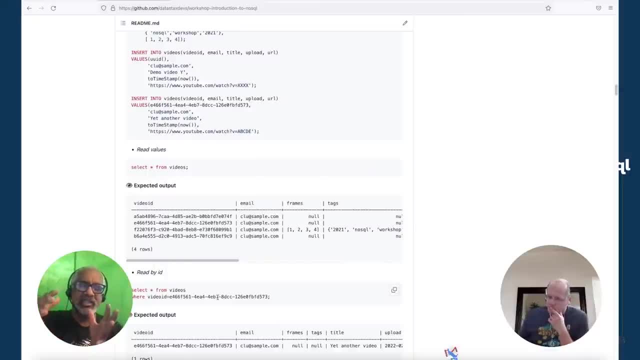 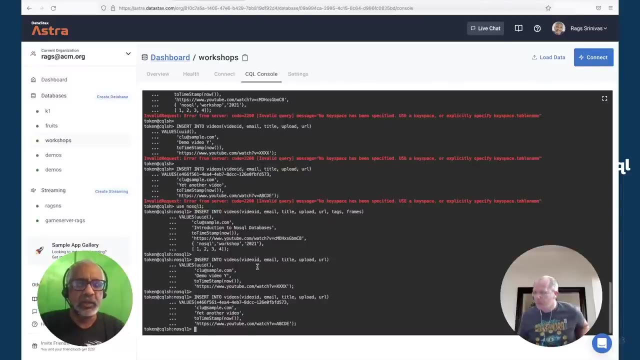 equal to whatever. and now the video ID- you know essentially as we call it, is hashed into a particular partition and from that part, a particular partition, you can get the information. okay, but since we are learning here, we are still in learning mode, right, we are probably okay to do this, right, so you can see. 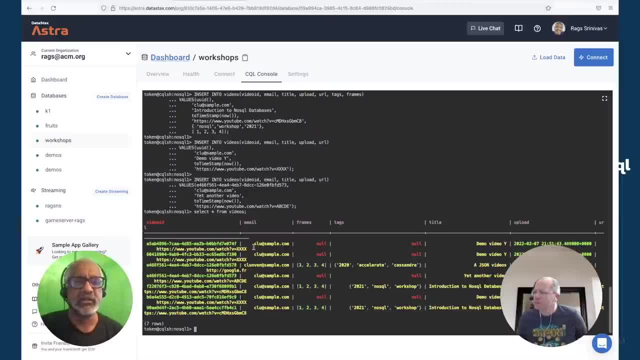 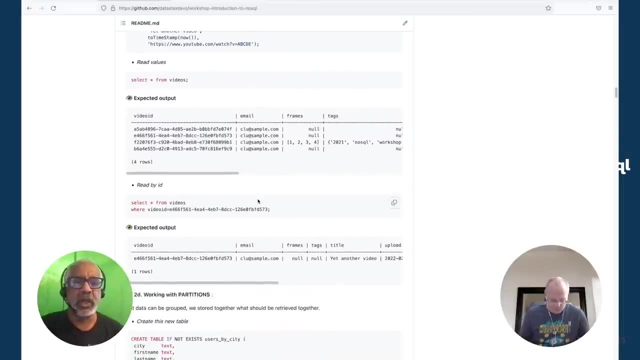 here. I have already created a you know bunch of entries here, and you'll see all the entries: video ID, email frames, tags- you can pick and choose. this is kind of somewhat similar to SQL, if you have used this before, but obviously there are some critical differences as well. okay, so now what I'm going to do is I'm 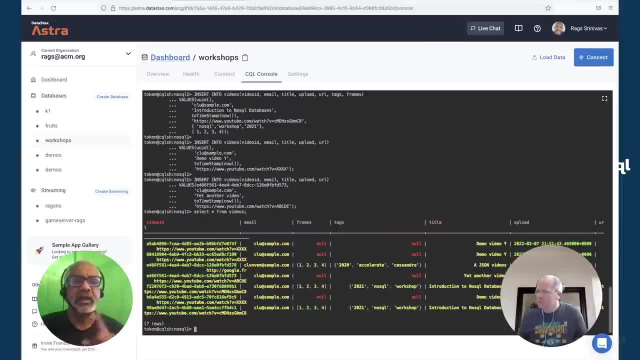 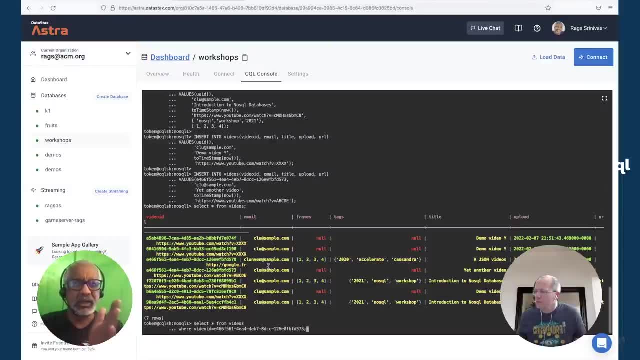 gonna pull. I'm gonna go to a one partition, right, and I'm gonna pull the data from there. so this is what I'm doing: select star from videos. where? select all the table, I mean all the columns right from this particular table where I'm going to a particular partition, hitting the partition and 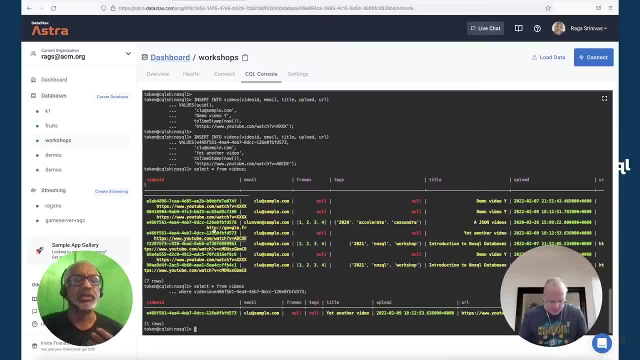 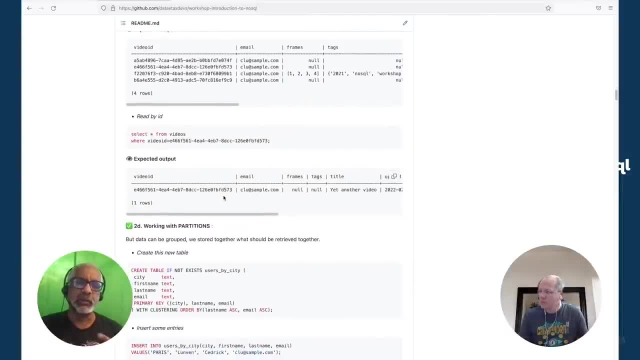 getting the data from there, and there you go, okay, so, so this is a lot. you know it's a. it's a better practice to observe, because that's typically how knows no sequel works is. you know, you have the the case, the use cases kind of defined by the primary key. 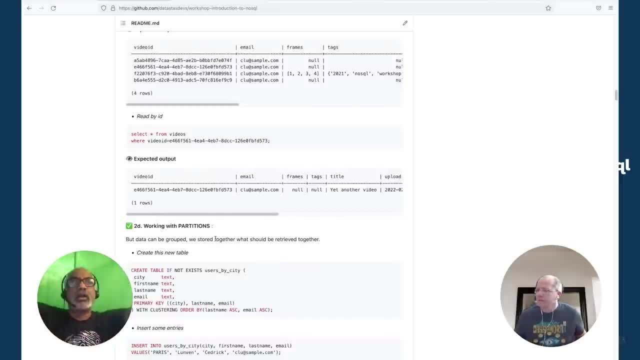 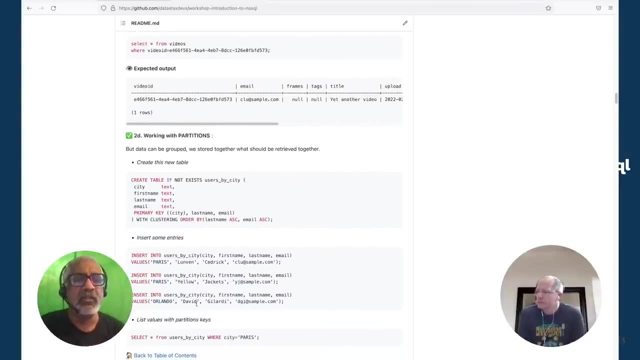 or the partition key, so that you know you don't do a whole lot of looking around the entire cluster, but but you go to a specific partition. okay now, obviously, based on your use cases, you may want to create new tables, right? so again, you know the same formula, right? if it does not exist, then you create. so 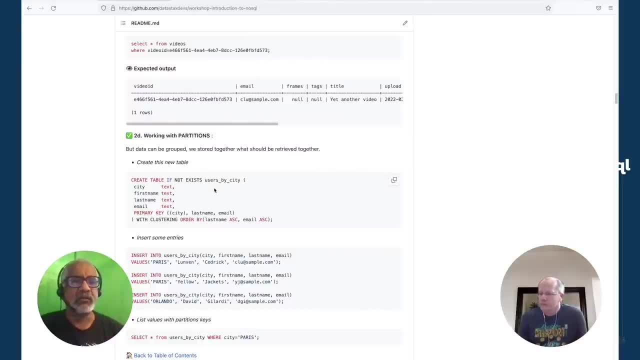 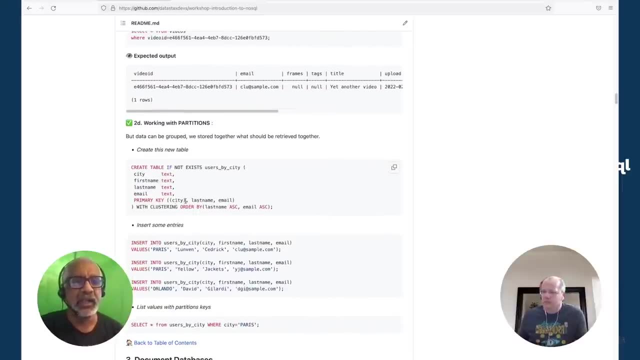 what you're doing here is you probably want to. you, you know, kind of look through the user by city. okay, so create table, if not exists, and notice here my primary key is based on city, and then you have a last name and email, which are really the 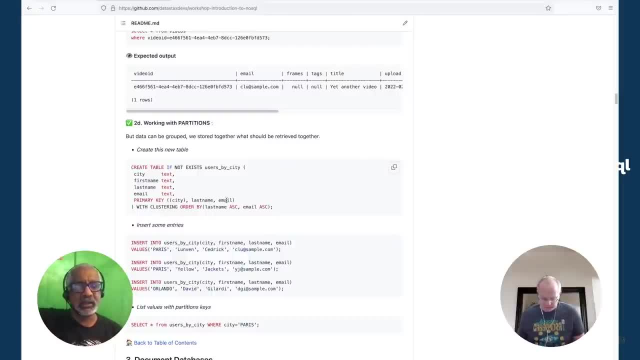 clustering key. and now what you can do is: you can, you can you know if you're producing a report? you can. you can produce a report where the last name is ascending, but but you know, if you want it descending, you can do that as well. you can do that in the query. but essentially what, what this does, there are 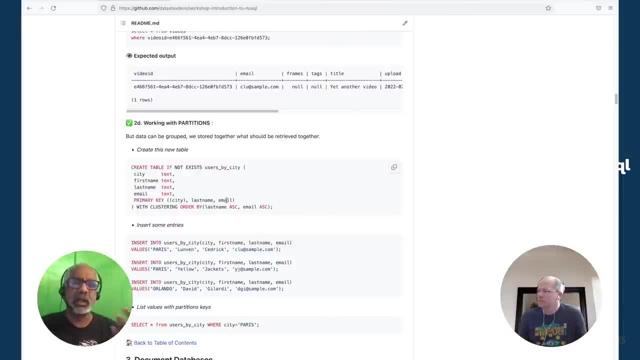 a number of rules for you know, primary key, clustering key and object closure key and so on, but but the idea is that you let your use cases define your keys, rather than the other way around. you know, in the typical SQL way, what you do is you can adjust your use cases based on the data model which 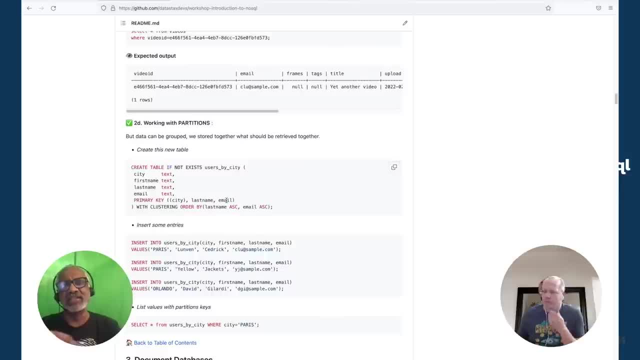 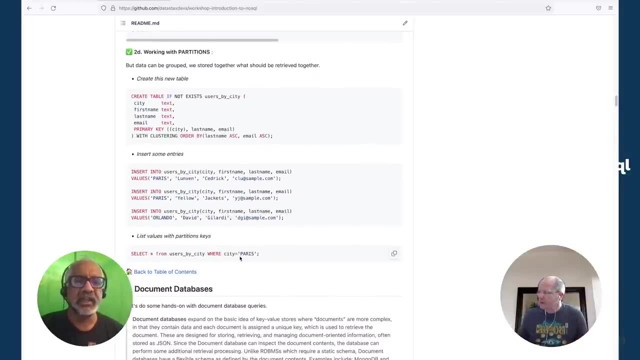 is really not the ideal way to go. you would rather be use case as define the you know data model. okay, so I think I've said enough, but let's let's take one look at this: Yeah, where city is equal to Paris, right? 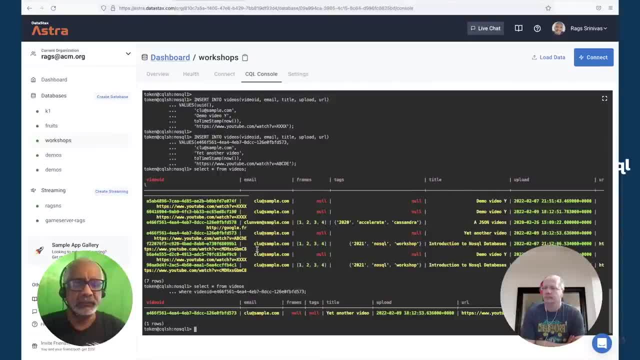 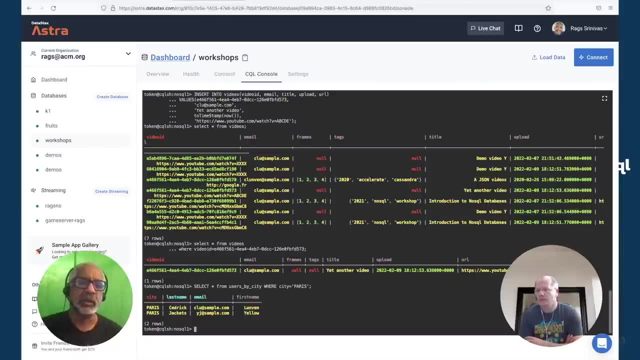 Same thing again. you know you're gonna do the same thing. right, Select star from users by city where city is equal to Paris, right, And you should see a couple of those, okay. So let's again see a few thumbs up after you get to this. 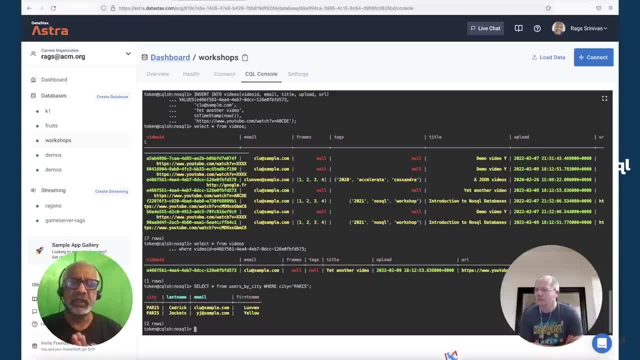 This is probably gonna take a little bit longer. So we will, you know, be a little bit more patient. I know that we are. I think we're doing reasonably okay With respect to time. But you know, Artem, do you wanna add any color here? 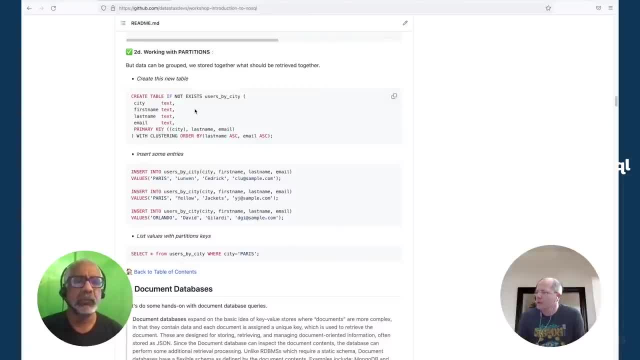 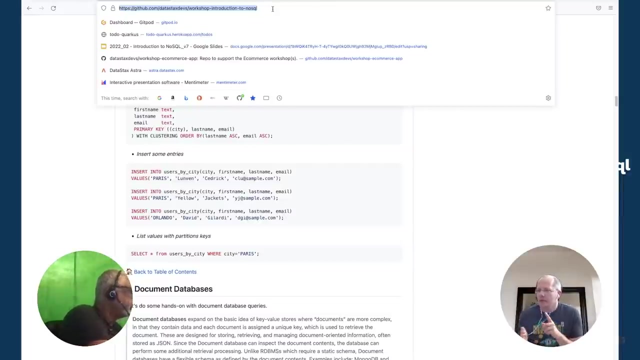 Did I miss anything major? We had a few questions and I'm gonna answer them. They basically are questions about where do we get these scripts and instructions? They are on GitHub. We posted that link multiple times and somebody will post it again, And Rex was switching between the instructions on GitHub. 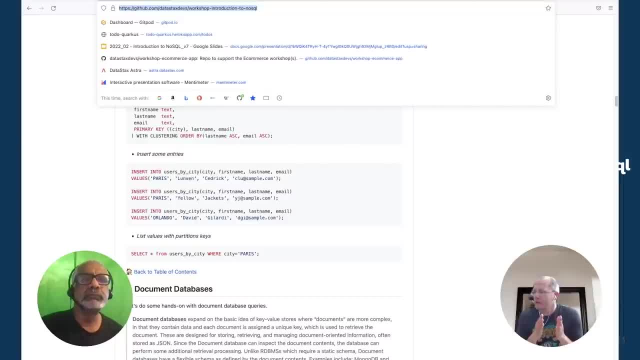 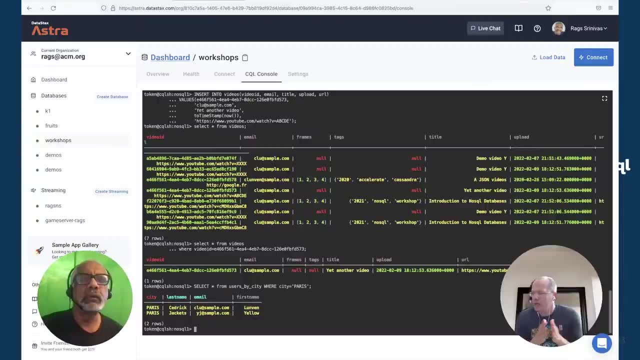 and the AstraDB interface, in particular CQL console, which is, in that case, web client that supports-. No, that's a great point. I think I didn't mention that. Basically what you know. you can see this better now. 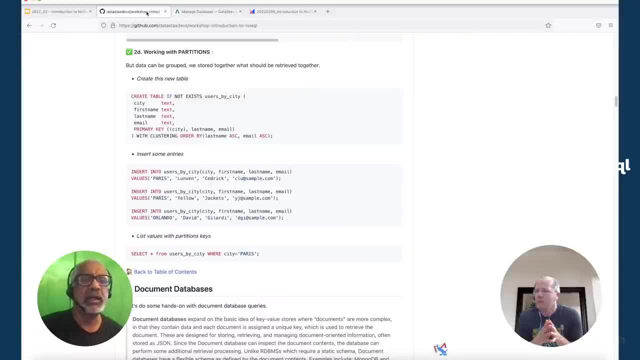 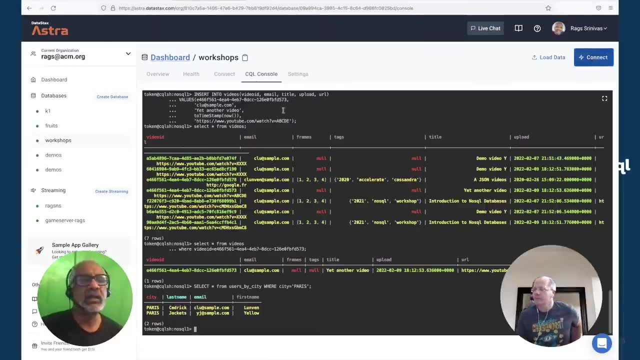 I have this in two different tabs, You know, one tab is my GitHub instructions and the other tab is my Astra database. essentially what I've done is I did a connect, I clicked on the workshops- you know the database- and then I did a connect and then I hit sequel console. 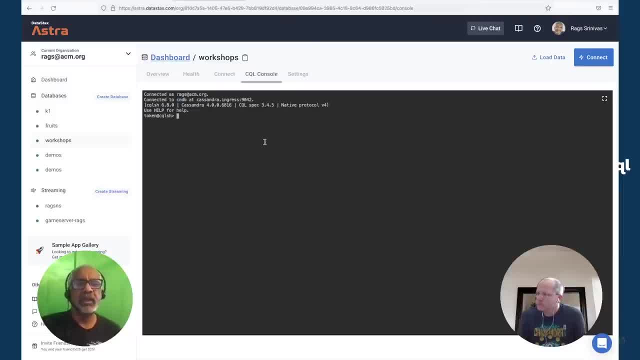 and then I'm good to go here, okay, and then what you do is you use the key space, okay, and you can do a whole bunch of stuff. I'm just gonna describe the tables here, okay, you'll see here there are different ones. key value, users by: 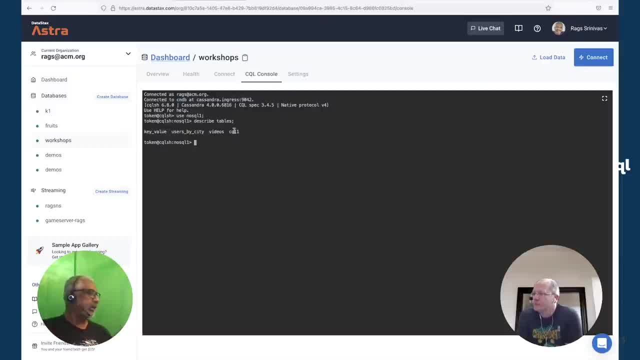 city videos. okay, all right. so another question: if somebody is following that, following these instructions and doing the hands-on, do they need to take screenshots for for the homework? at the moment, and again, you know this is not going to take too long, so my, I mean different people learn. 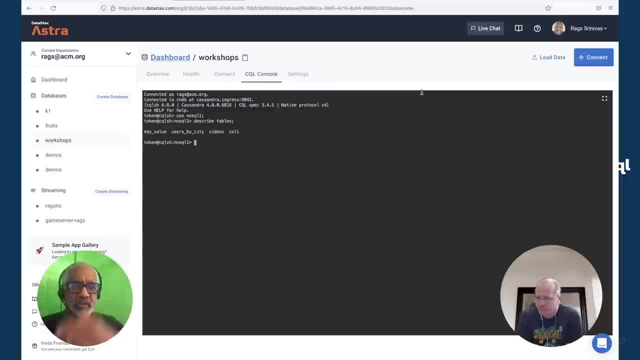 differently, right, I like to kind of go through it once and then go back again and then take screenshots. it's just easier. I mean, whatever style works for you, that's fine. yeah, if somebody got lost, you can just look at the demo and then, as a homework, you can follow those. 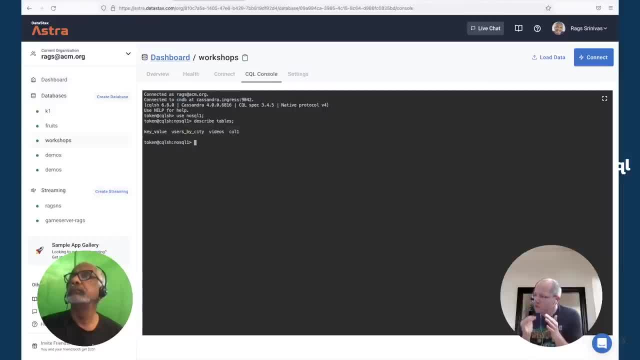 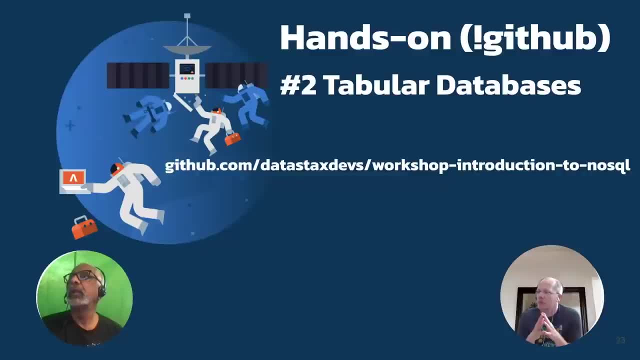 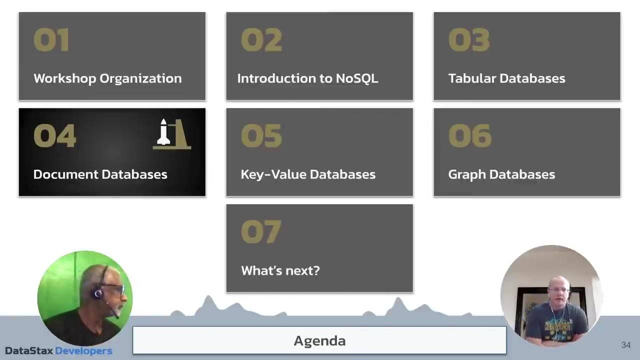 instructions. they work so there. if you just follow them properly, you should be able to to do the the this same same work. so there should be no error. right back. you are done. yes, you're good to go. yeah, so the next one we're gonna look at is document database and what are. 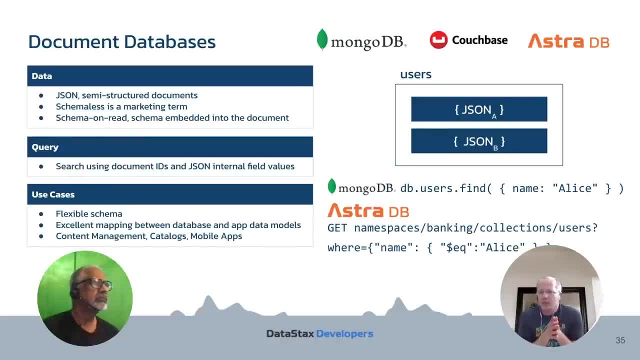 those document databases. examples are MongoDB, Couchbase and AstroDB, okay, and the, the data model is essentially a semi-structured document. usually it's in JSON, in JSON format, so most common. it can be some other format, XML, for example, or some something else, but JSON is the most common, very convenient, and we're going to use JSON. 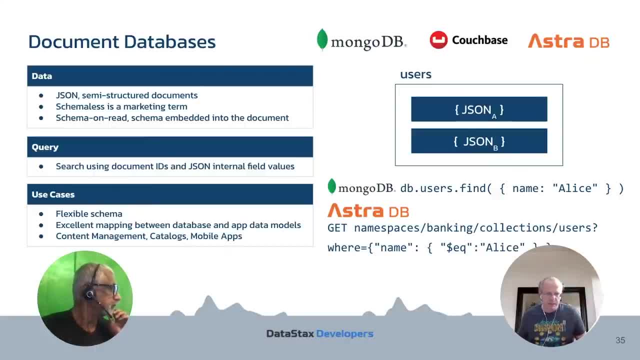 these databases are sometimes called schemaless, but it's so as if they do not have schema, but that's more of a marketing term. they do have schema definitely, because otherwise, what? how are you gonna process that data? how are you gonna query? no, there are fields there, inside of JSON, there are even data. 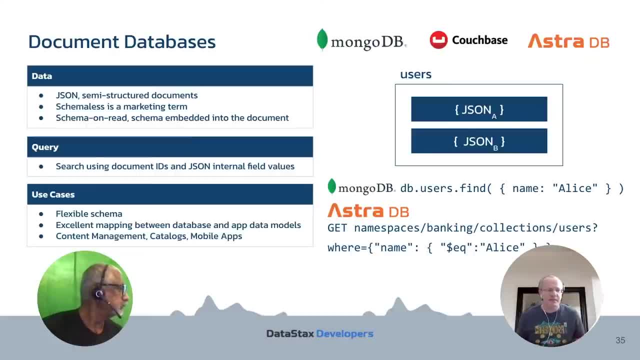 types like array data types and things like that. So the schema is actually you do not define. you don't need to define the schema in advance. You can store your data but it's already organized and structured in JSON document and you actually data model in advance and you think how you're. 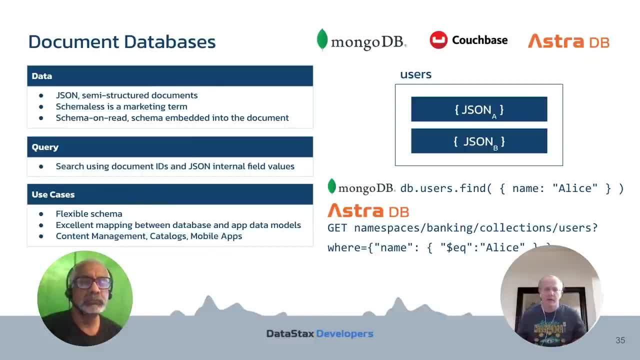 gonna retrieve that data, how you're gonna organize it, how you're gonna use it in your application. So, when you read the data back, that's when you process it, and it's basically like schema on read, schema embedded into the document itself. That structure of the document is the schema. 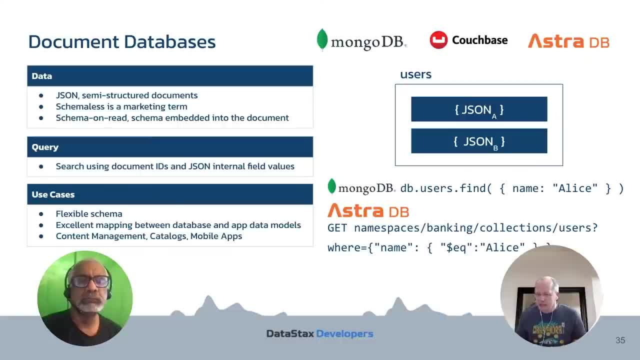 So those JSON documents usually have IDs. IDs can be generated automatically by the system and you may never need to use that ID, but you can also specify your own ID if you prefer. You can also specify your own ID if you prefer, and you can also specify your own ID if you prefer. 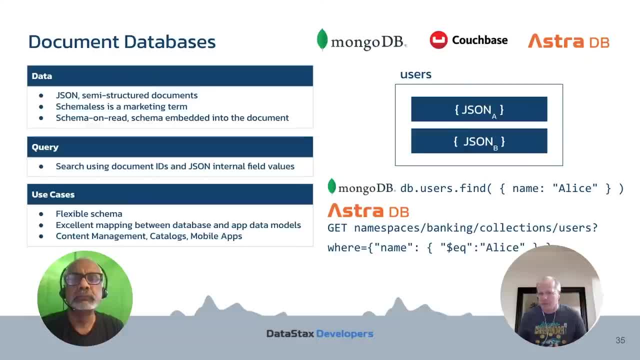 and use it in your application. that will be very efficient access pattern. but the difference. but, however, the document databases frequently use queries that that basically retrieve multiple documents, potential multiple documents, based on fields inside of the document. so they use a lot of indexing schemes that allows you to query fields inside of those JSON documents. okay, so 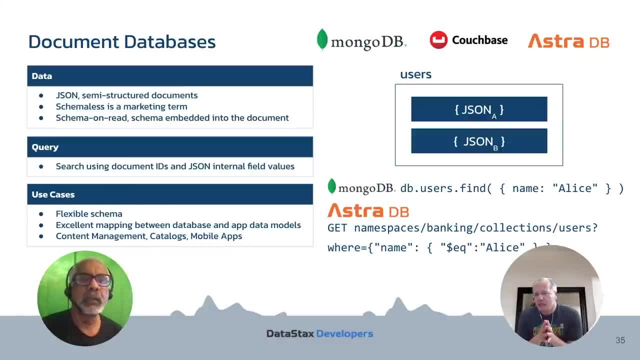 these are query access patterns. also, those JSON documents are usually organized so a number of them can be can be stored into container, which is called a collection. so here in this illustration we have users, which is a collection of JSON documents, and one of them has IDA, the other one has ID. 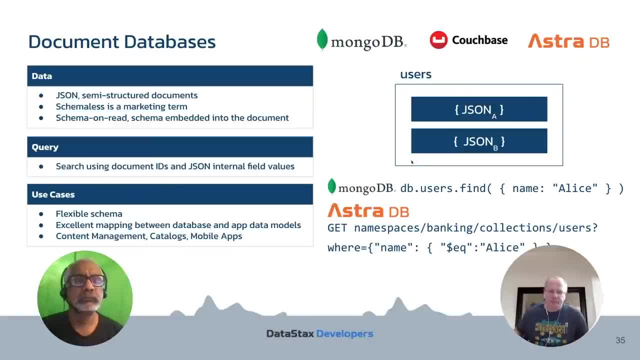 view be something like that. but here a couple of examples of kind of what types of views you can use in MongoDB. here we using database collection users. we find all JSON documents where there is a field name with Valor Ellis. in s3 DB the same will look like this. so this is the rest API we're gonna get and document. 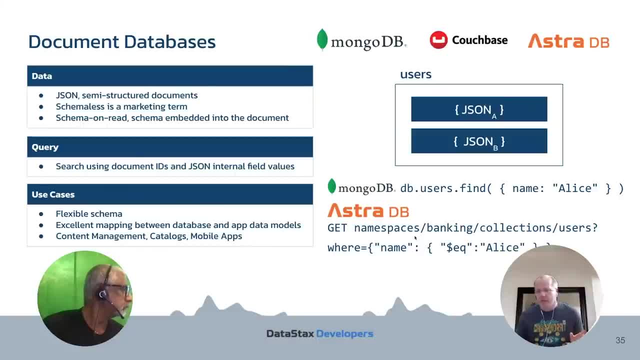 API. at the same time gonna get namespaces. namespaces basically like a key space banking, and then collection users and then where name equals Ellis. okay, so the use cases for document databases will benefit, or everything that, anything that benefits with less structured, semi structured data. so it's it's. it's more flexible. 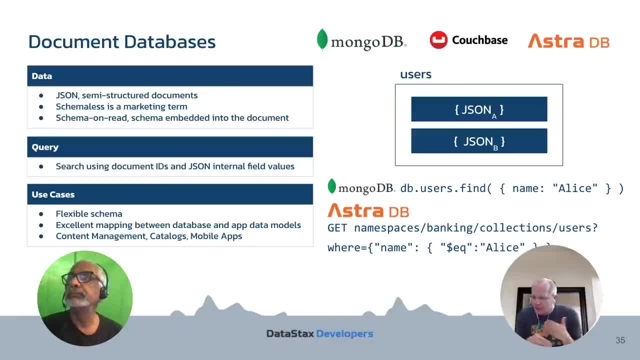 schema. so mobile application applications that will evolve frequently, maybe gaming applications, some catalogs of data, content management and and and so on, but essentially the you. you nest a lot of relevant data into that JSON document, you store it and then you index it and you will be able to create it based on different fields. 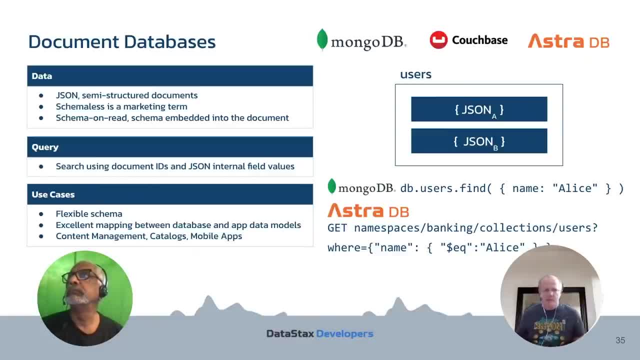 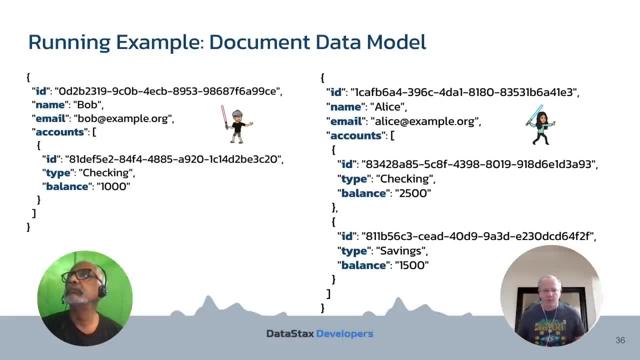 or document IDs. so how does, for our running example, how? how does document model looks like? we have JSON document for Bob and we have JSON document for Ellis, and it's it's. you can see: there is ID of Ellis, there is name, there is email, there are two account. there is array with two accounts that have ID type and 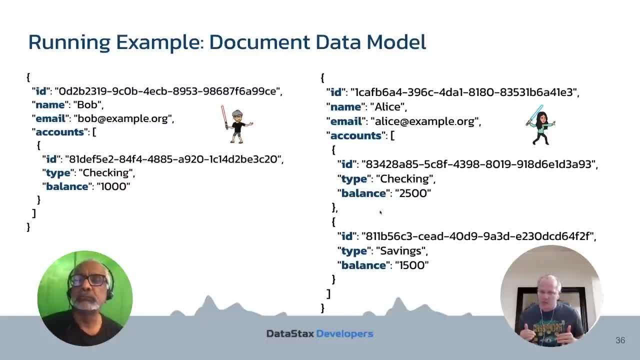 belts, and we can, and the system automatically indexes those fields and and you can create based on name and email, or the system also automatically assigns ID, or you can specify what kind of ID you want for the whole document, so there you can efficiently retrieve it again. there are no, we're not looking at. 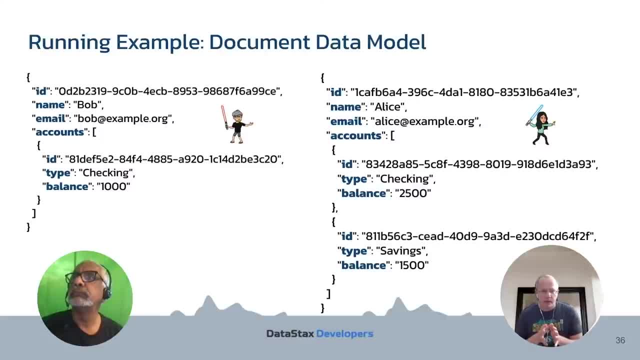 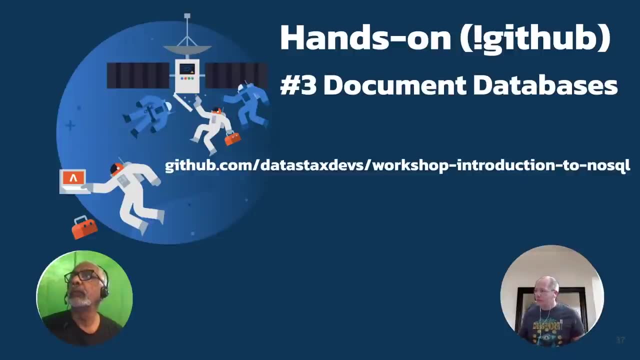 the joins here, just the, the, the. there are no two tables. there is one collection of those JSON documents for for users and that two JSON documents store. there are two JSON documents for your users and that two JSON documents store and that two JSON documents store. and do we have any questions? oh yeah, good question I want to bring up. 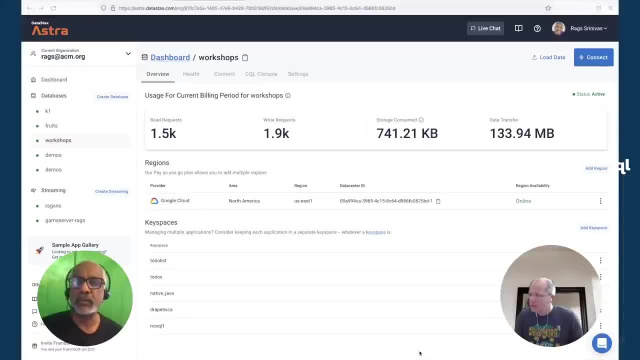 something that I forgot to mention in the previous, and and maybe the best way to do that is to just show this to you. you know, I know that some of you are struggling with the key space. I mean not all of you, but but some of you, if you. 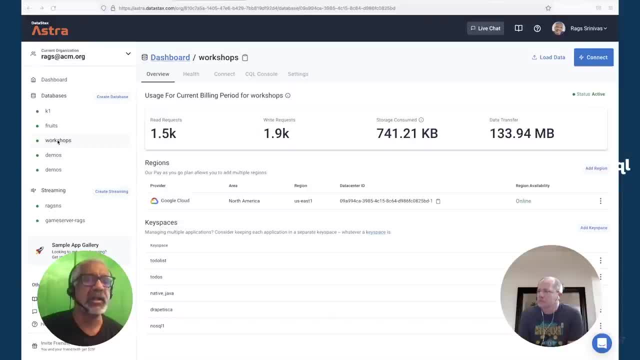 already created a database called workshops. right, you know chances are, you know you will see it on, you know on the left side, and then you know, make sure that it's active. and once it's active, you all that you need to do is you can just say: add a key space. okay, if, if the workshop is a, then what you can do is: 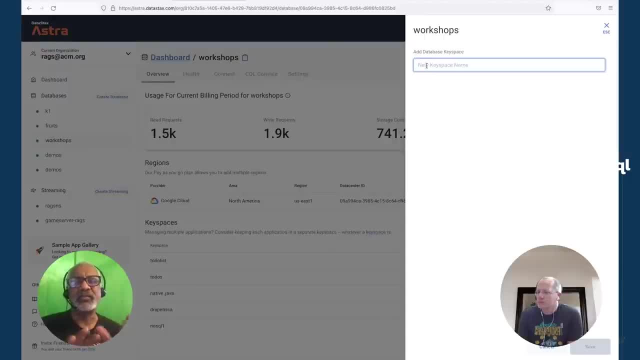 you can put no SQL 1. so if you, if you find that the, that the key space is not there, okay, chances are that you know you've already created the database. if you, if you're brand new to this, no big deal, you know everything will work like. 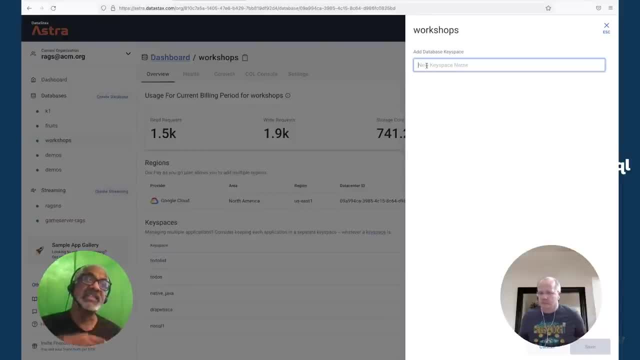 in the instructions. but if you have been to our past workshops, we ask you to create a new database and typically you know we use workshops. you will need to add this. so here you're gonna put no SQL 1, which is the key space, and here it's taken because you. 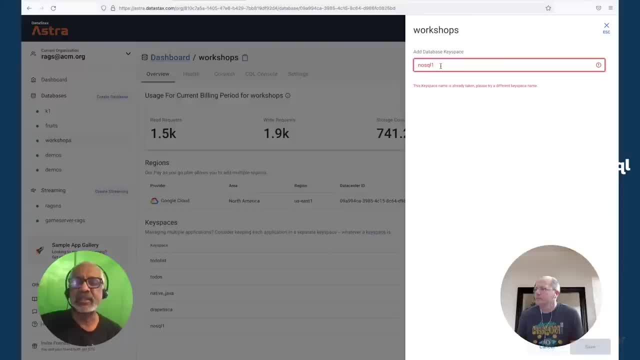 know, and the key space is already taken, but in your case, you know, if it's not there, you will add it. one other thing, you know, just use the case as is, because you know there are ways in working and working around it, but but you know it's. 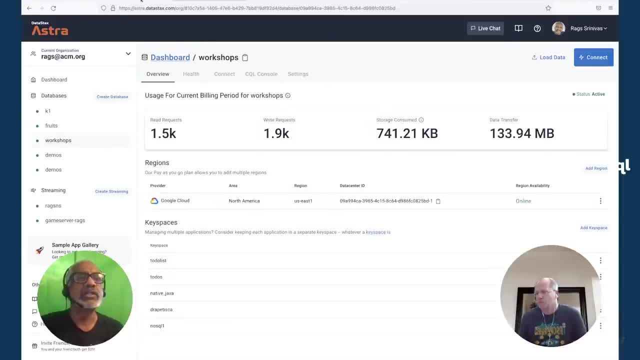 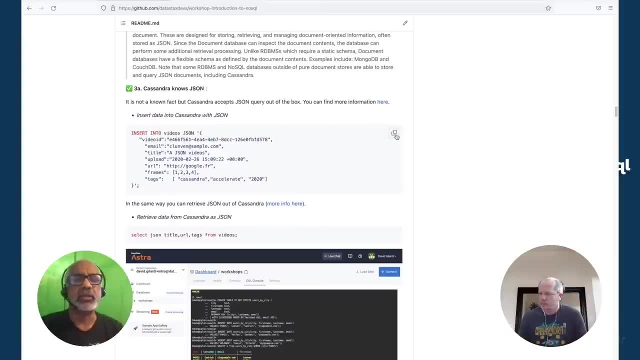 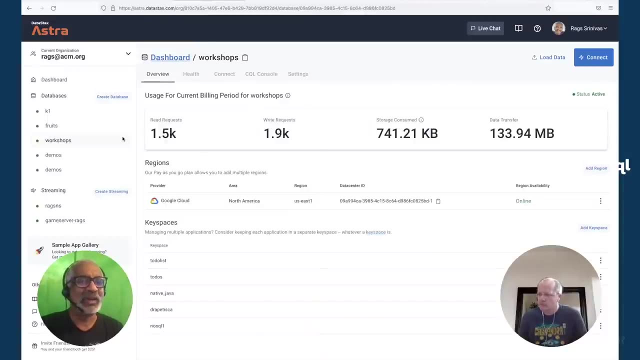 just easier to use the case, as is okay. so, with that said, let me jump to the next part, which is really the exciting part. right, you know, I think Artem talked about JSON, so I don't know why JSON is exciting, but but it is right. so, again, what I'm gonna do is I'm gonna go to workshops, right? no, 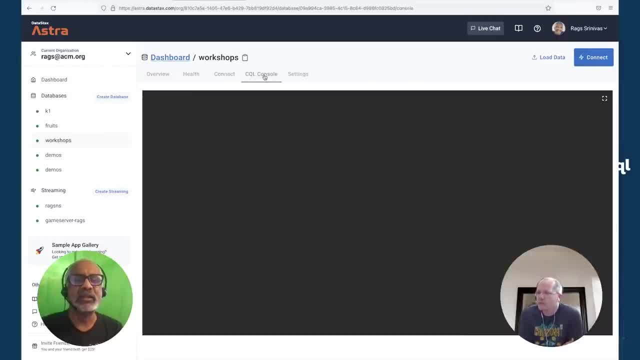 big deal right connect, and then I'm gonna hit them sequel console right and use no sequel one right, and again I'm. I cut from the instructions and I pasted it right. that's all I did. so what I'm doing here is: you know, remember I inserted into videos and it was not in. 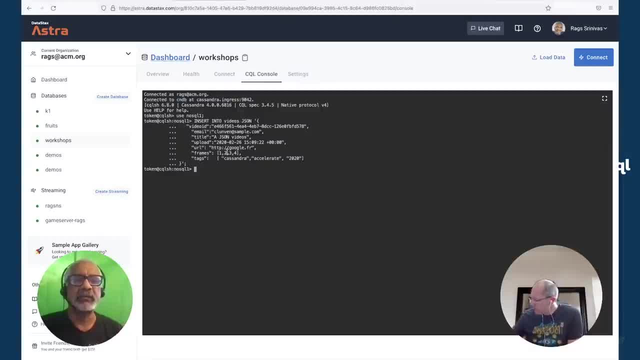 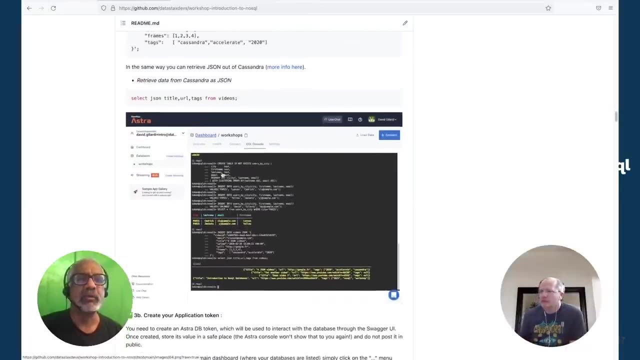 JSON format. right, but here it's in JSON format, okay. so some. sometimes it's easier, especially if you're doing some programming and things like that, to insert JSON directly. but you know, if you want to insert data, that's fine as well. okay, so you can try that out, okay, and and 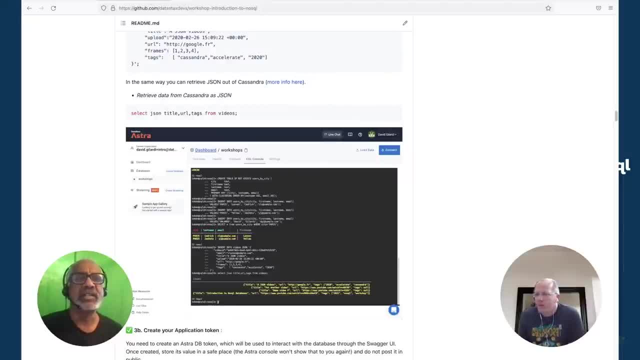 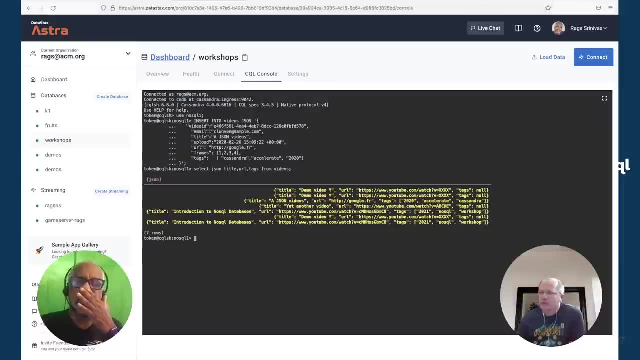 if you want to see the JSON, you can do that as well. all right, so here you know. you can see the information you know. remember it was all in columns right before, but now here it's in JSON, so if I just do select, I believe this should. 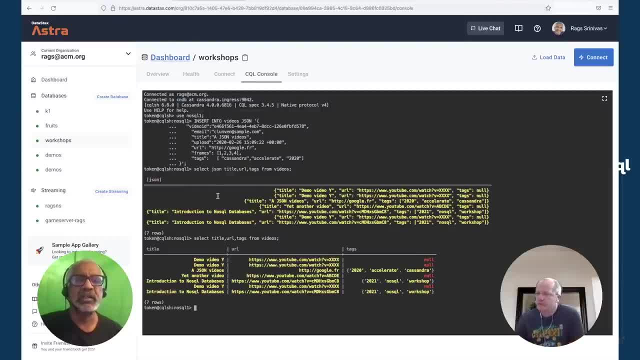 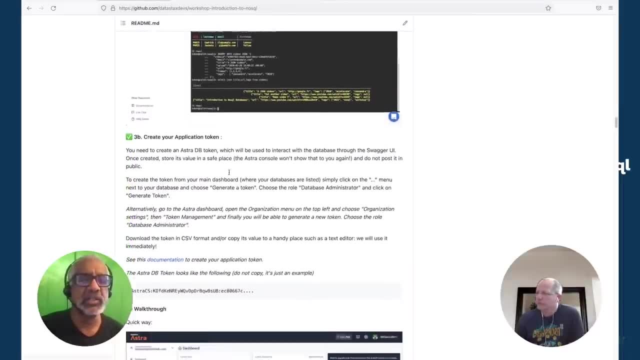 work right, so you'll see only as columns, but here you will see it as JSON. now the next part is a very critical part and I appreciate if you can pay some attention here, because this is probably the most complex part of the workshop, even though it's pretty straightforward. 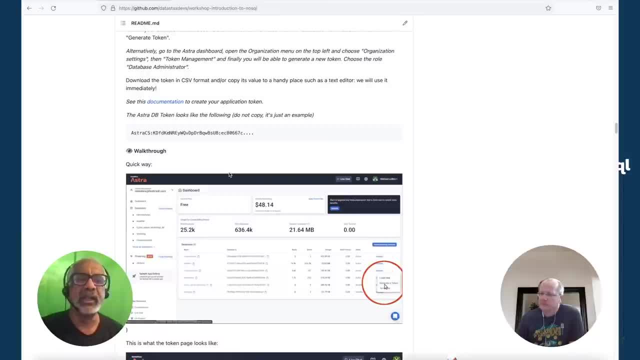 okay, so what you need to do to be able to get access is to have what is referred to as a token. okay, and this is typically how you know. a lot of the API is rest based API is work. okay, so what you can do is you can generate a token. 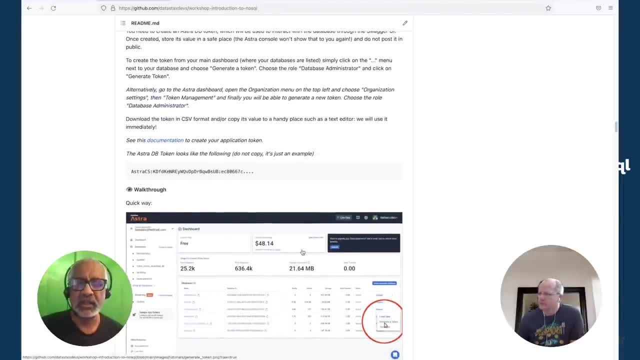 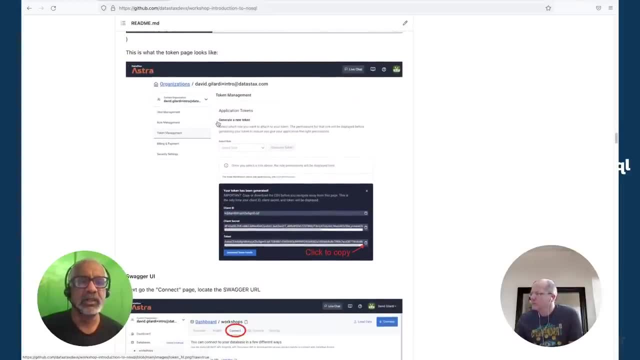 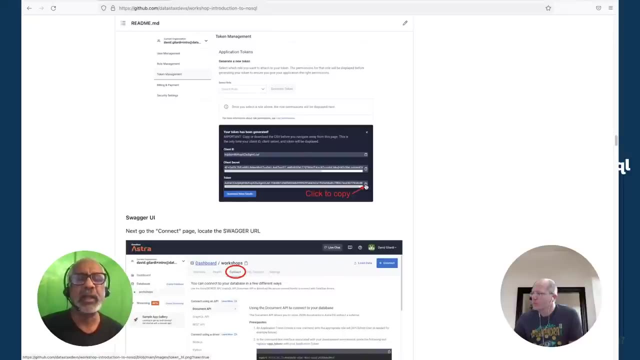 and, and you know the steps are in there. so you do a generate token and then you just do a click to copy, okay, and and basically pick a database administrator as the role, okay, and then what you do is you do a click to copy- okay. typically what I do is I take this and paste it somewhere so that I can always have. 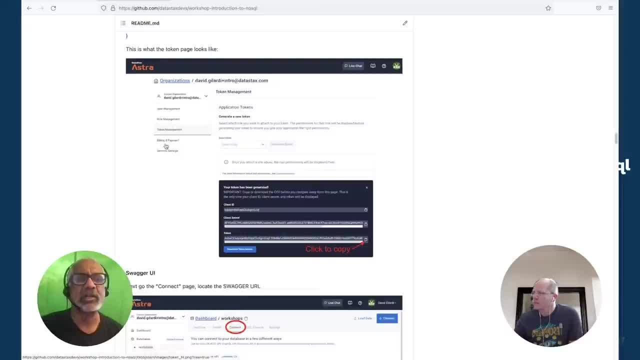 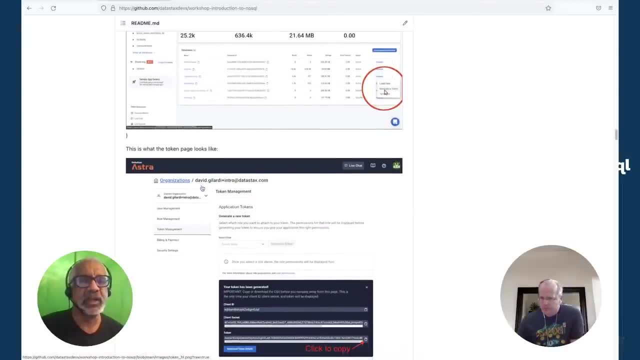 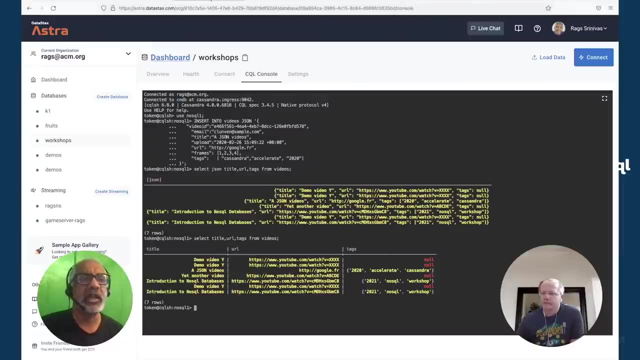 access to this token, and you're going to probably use this token throughout this workshop today. so that's my suggestion. so, again, what you're going to do is you're going to pick the database administrator role and then you're going to select the get something, a page that looks like this: okay, so let me show you an action. okay, because you 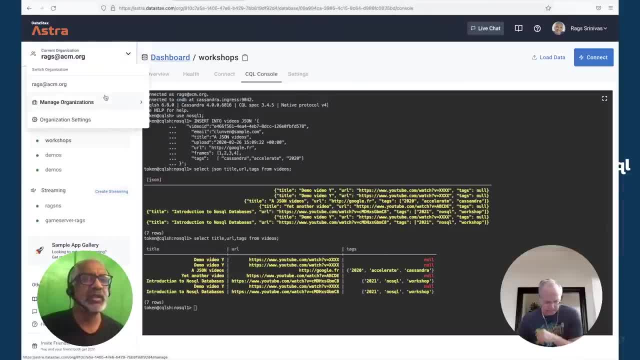 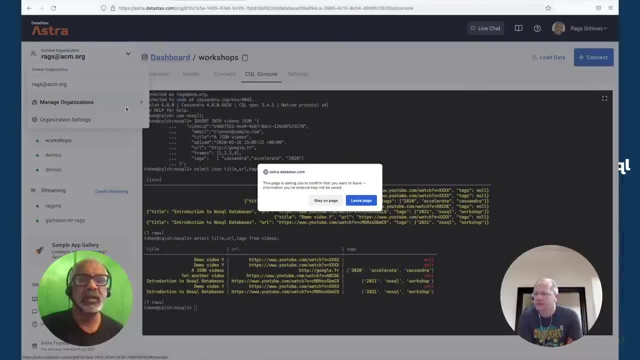 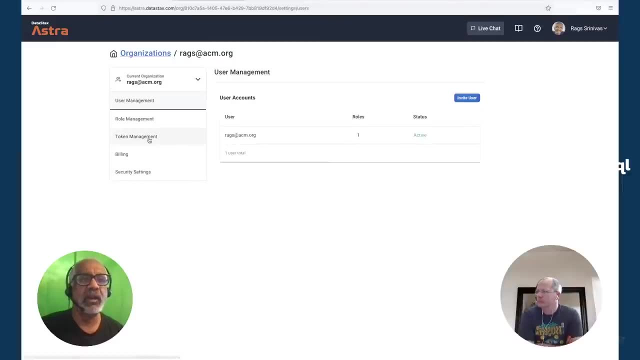 can always create one, so go to. there are a number of different ways of doing this. basically, what i do is i go into here, manage organizations- no, i don't want to look so organization settings right- and then i go to token management and generate a new token. 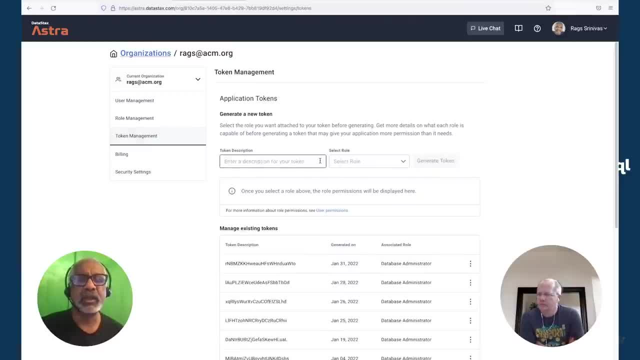 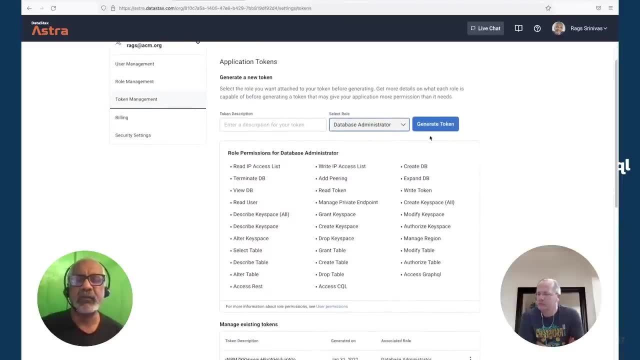 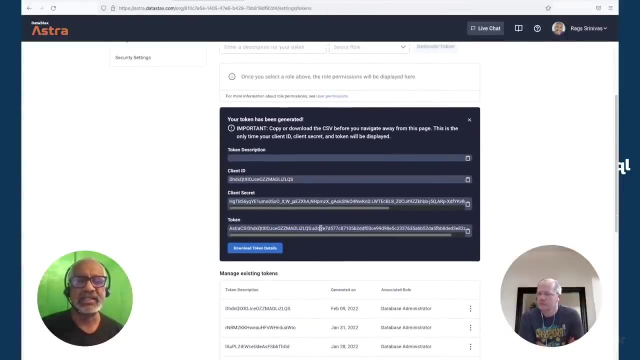 okay, so token management, and then what you can do is you can, you can enter a description if you want, but pick the database administrator right and when you hit the generate token- okay, you will see something like this. so what you can do is: you can grab this. um, the only note of caution here is: 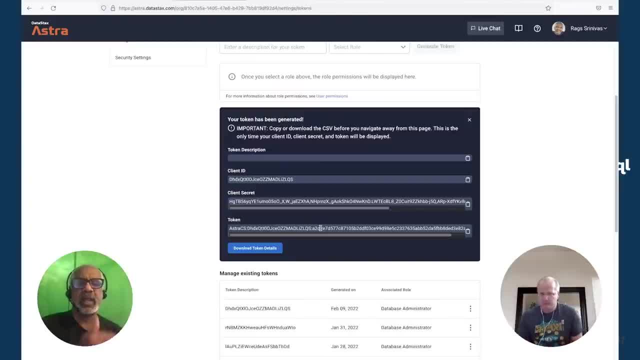 if you wander away from this tab or from this page, you are not going to be able to get back to this, so so make sure that you copy the token before you wander away. or if you, for some reason, you wandered away, uh, you always, you probably will have to create a new token anyway, okay, um. so, with that said, uh, let's get some thumbs. 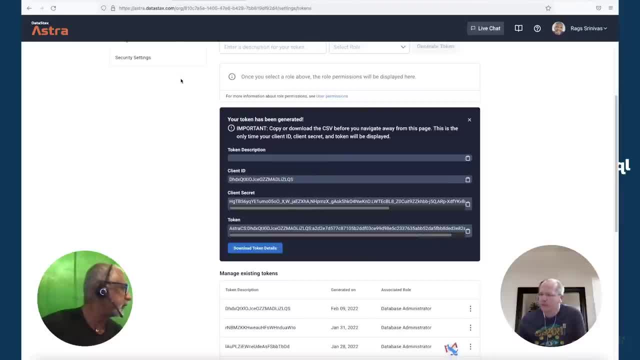 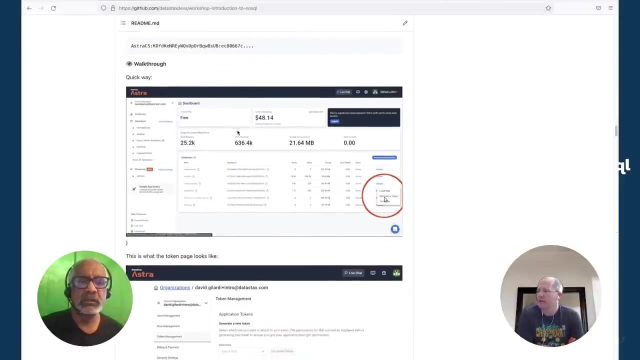 up of when you have copied the tokens and then we can proceed from there. how about? how about we take a brief little pause? uh, i know we are kind of running up on time, right. yeah, we're running off time soon, so i suggest we just do demos and um, you, you can do homework if you, if you prefer. so you, you have exactly the same. 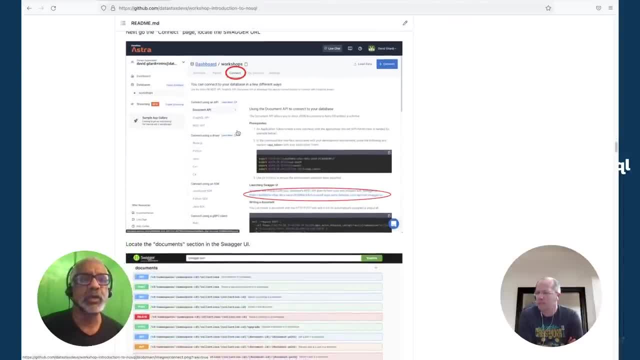 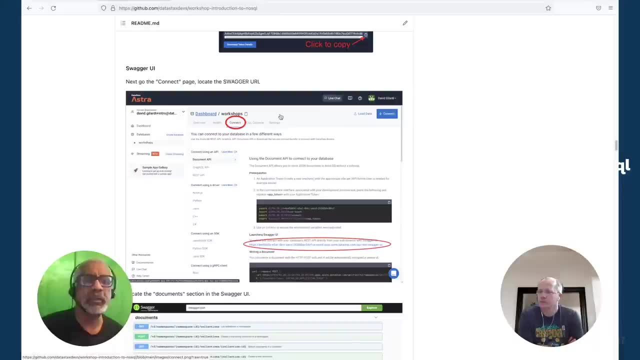 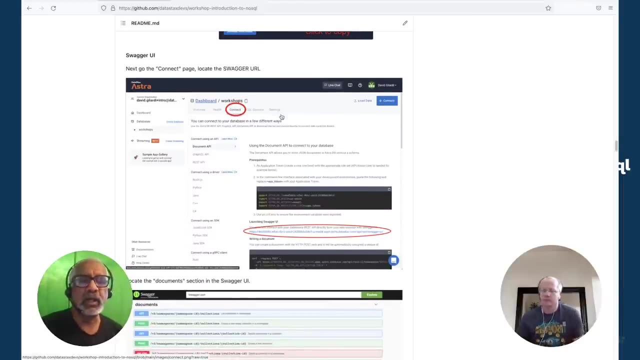 instruction. yeah, yeah, so not to worry at all. um, okay, so what we're going to do next? um, maybe, maybe, if i see some couple of thumbs up of of people able to copy the token, then we can proceed. uh, i just don't want to leave everybody behind, right? but uh, but like what, artem? i think it might be a. 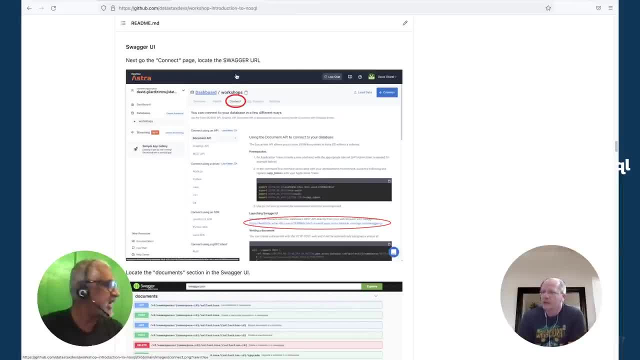 good idea to just, uh, kind of proceed. okay, so, let's do that. okay, so, let's do that. okay, so, let's do that, okay. so next what we're gonna do? okay, couple of thumbs up is all i want, okay. so next, what we're gonna do is we're gonna locate the swagger url here. okay, so, let's see. go back here. okay, i have. 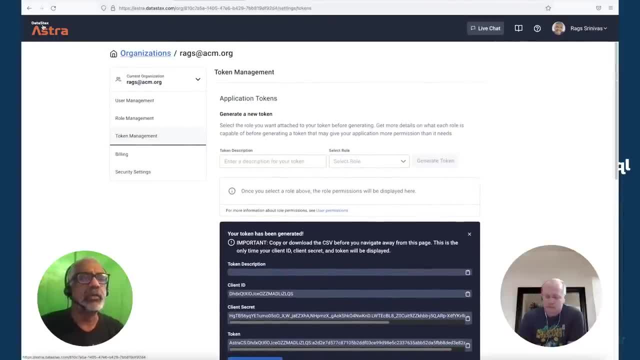 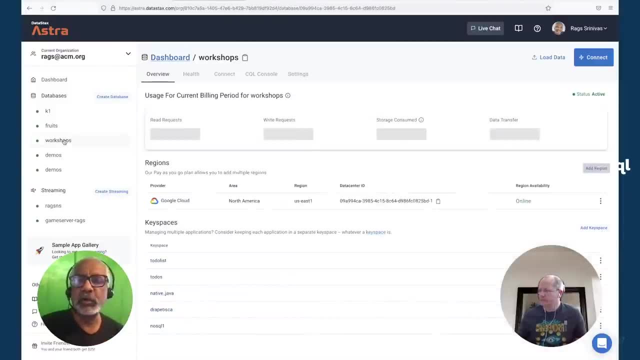 copied the token, so i'm not gonna worry too much about that. so i'm gonna go back to my dashboard, okay, and i am worried about workshops, right, and what i'm gonna do is i'm gonna do the connect again, okay, and you should see some of the tokens that i have copied, and i'm gonna do the connect again. 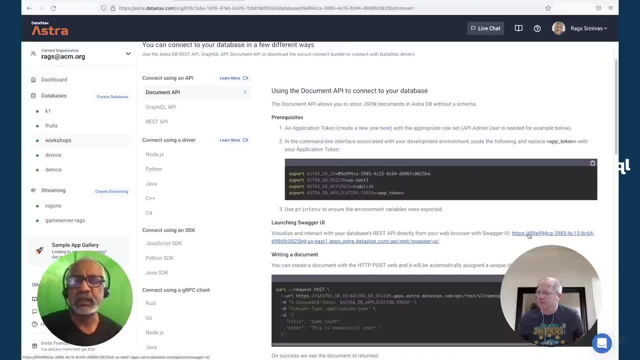 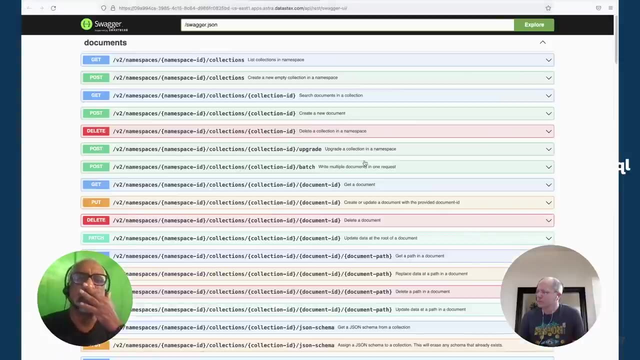 somewhere here there is a swagger url somewhere in between right launching the swagger ui, so just click on that. if you want to click on that new window, you can do that as well. whatever. whatever suits your fancy, okay. so just click on this. okay, it will bring you to a new tab, which is basically: 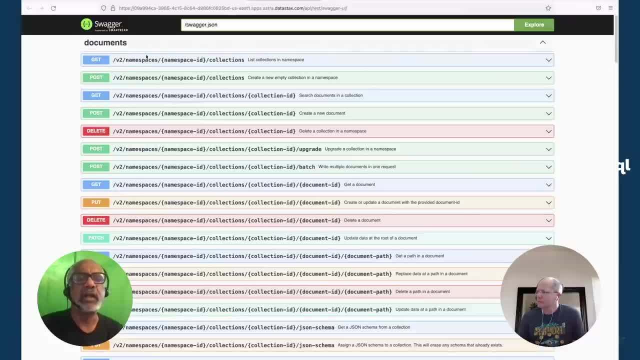 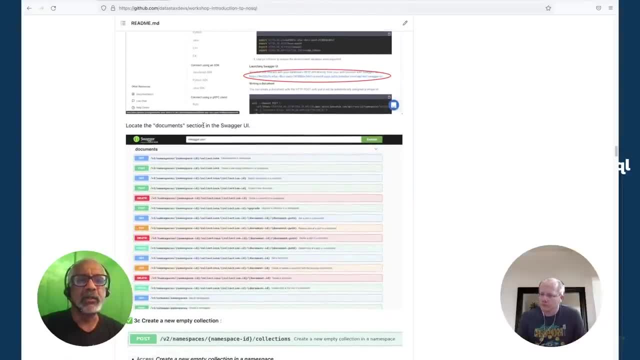 the swagger of all the apis that are available for you and we're going to try some of them. okay, i'm not going to go through all of them because i don't think we have the time for that. uh, looking at the document section in the swagger, ui right, so let's go back to locate the documents. 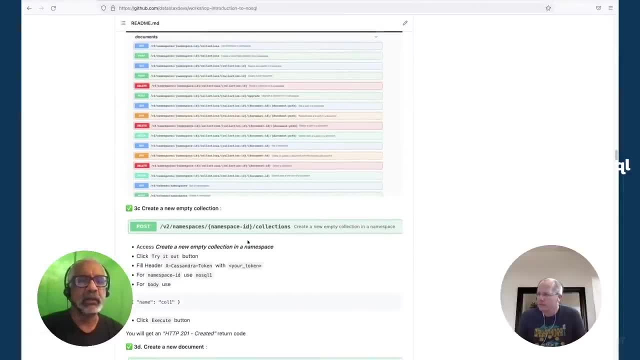 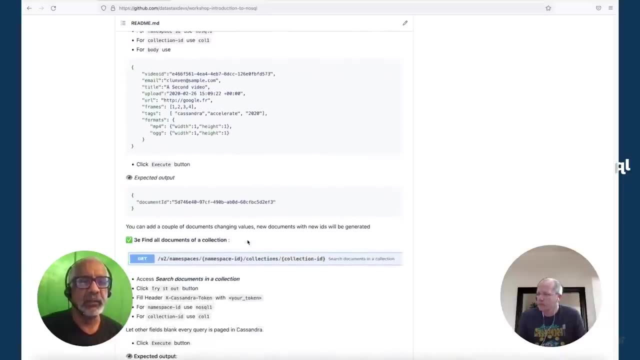 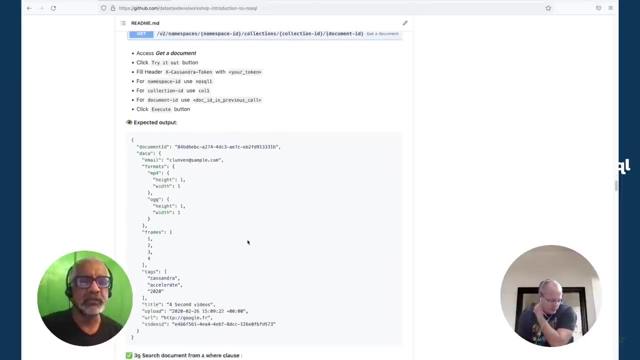 and and essentially, actually, let me um, we are going to take a look at all the uh. are we going to create a, um, a new empty collection? okay, um, but um, yeah, i think i think that's good. we'll, we'll create a new uh collection. i was just wondering if there is actually. let me show you something, a. 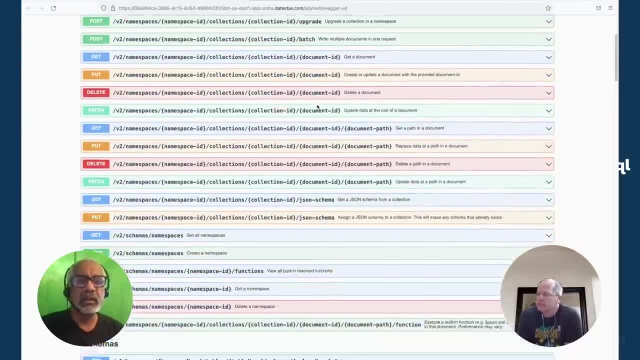 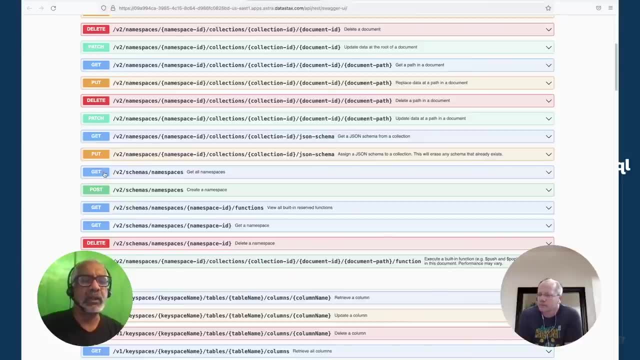 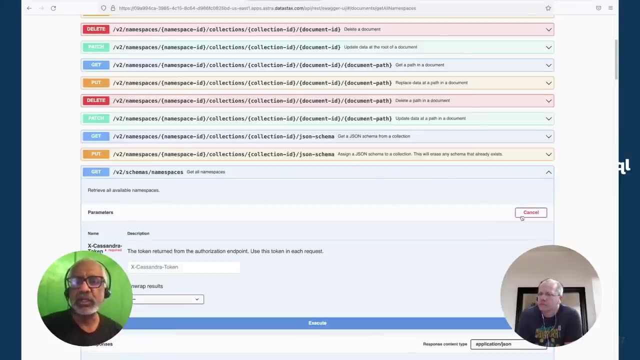 little bit more um, easier. so what i'm going to do is i'm going to get all the namespaces in this particular key space, okay, so all that you're going to do is you're going to click on it, you're going to do it, try it out right, and you're going to hit and execute. okay, and if you hit and 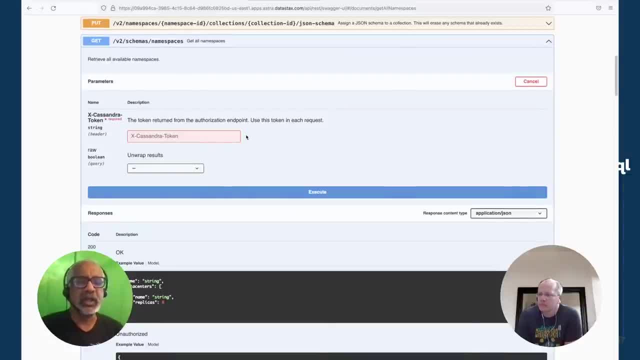 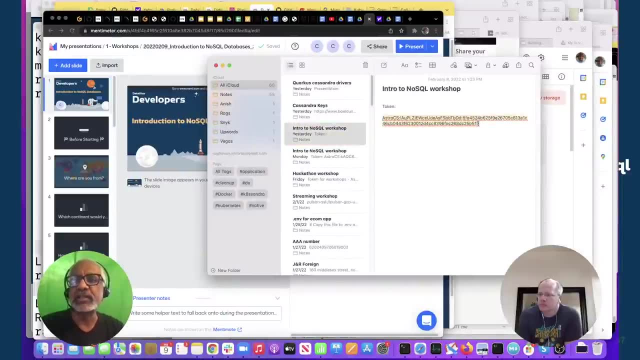 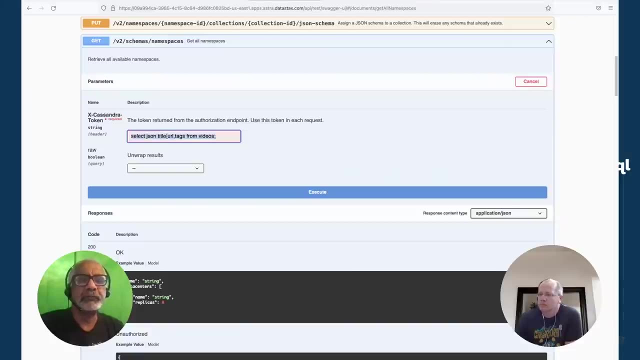 execute, you're going to get an error because you know don't have the token there, right? so what i'm going to do is i'm going to grab the token, okay, and i basically destroy this after this. so i'm going to go back, okay, and i'm going to put the token- oh, that's long one, i did not grab it properly. 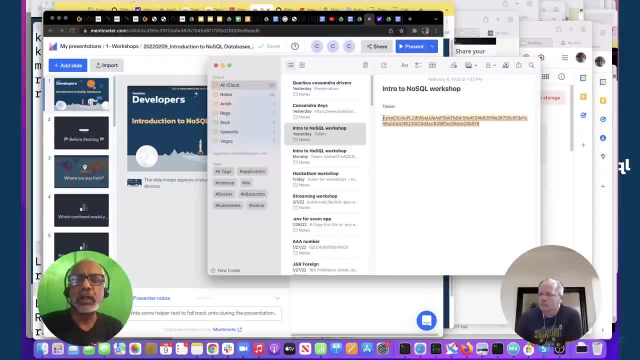 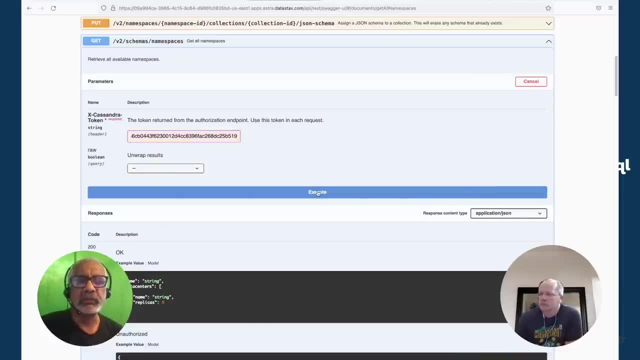 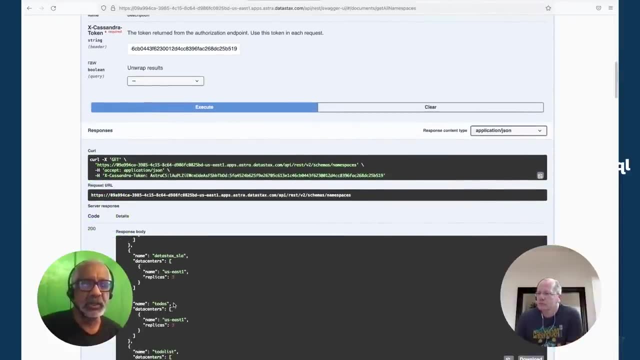 so let me grab it properly, okay, and go back here, put the token and now i should be able to execute. okay, and you'll see here it's the same information that you got before, right? uh, you've got system auth. you had to do's. you had the to-do list, all the different key spaces. 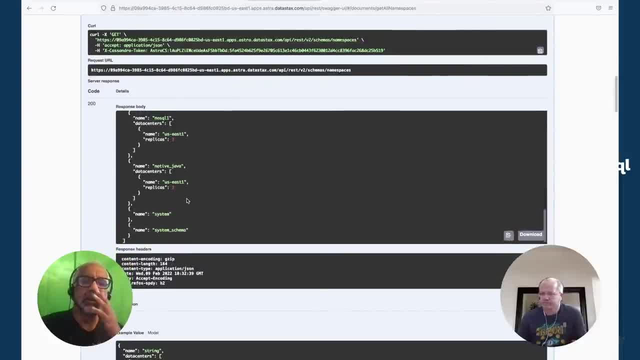 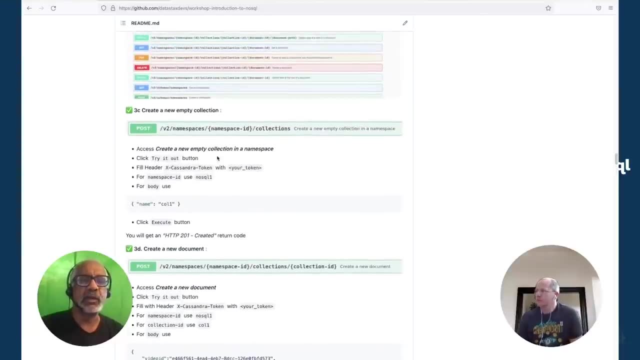 you know, in that particular, you know database right, so all the different key spaces are available and and you can dig into each of those key spaces. so so let's create a collection like it suggested, and then maybe i can skip the other ones. okay, so create an empty collection. so how do i create a? essentially what you're going? 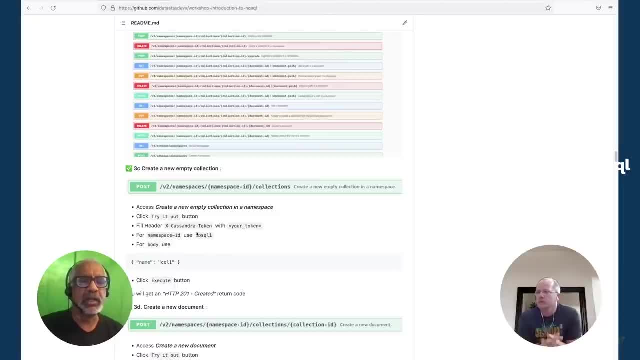 to do is for the body, for the namespace id- we use no sql one- you're going to use the token and then you're going to specify the name is collection one and if you get http 201- which is typically how swagger works, you know it gives you the all the different http codes. 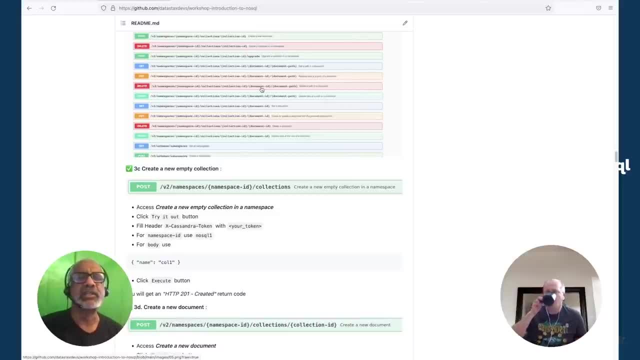 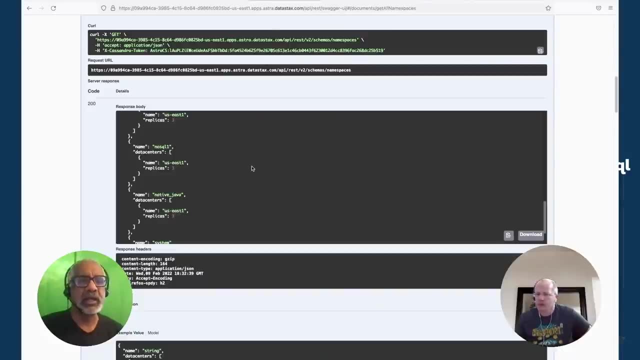 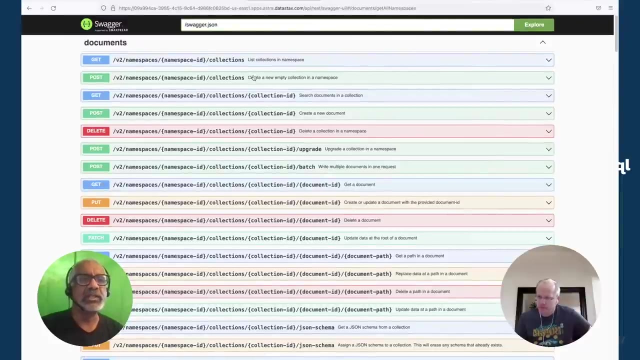 um, you know, if you get a 400 or something, you'll get an unauthorized and so on. um, you know, it'll tell you, it'll give you information on, on what's going on. okay, so let me go back to my swagger id, um to my swagger ui, okay, and find the was it post collections. 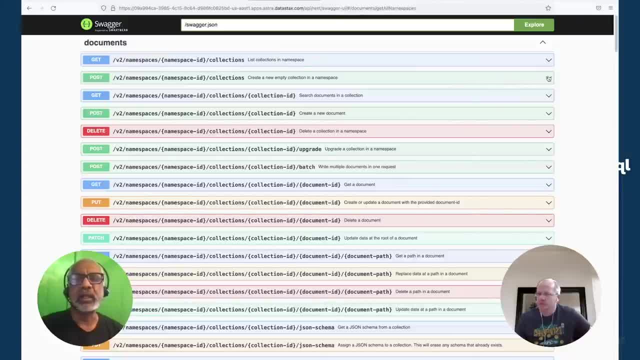 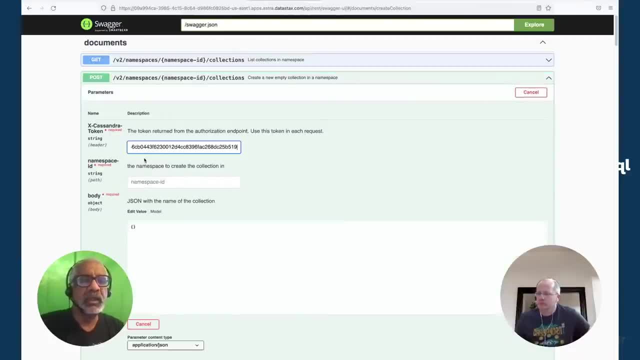 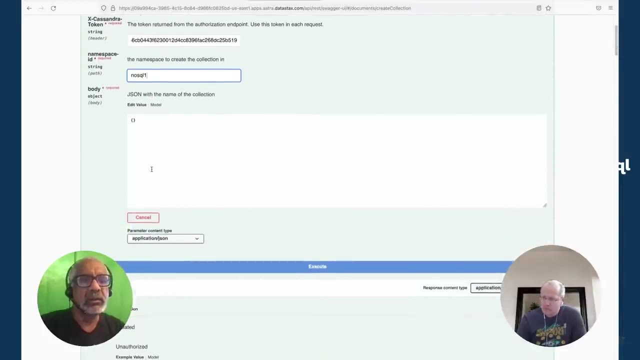 yes, let's try that anyway. create a new empty collection, right? so let's try it out. okay again. post the token: all right. namespace id is no sql one, right? um, did i get it right? all right. and then a collection one, right, so? so let's go back to the collection one. 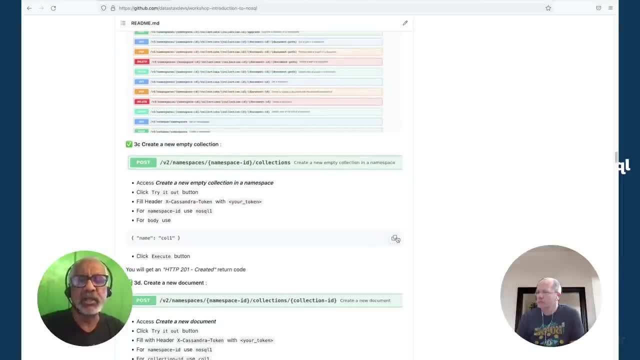 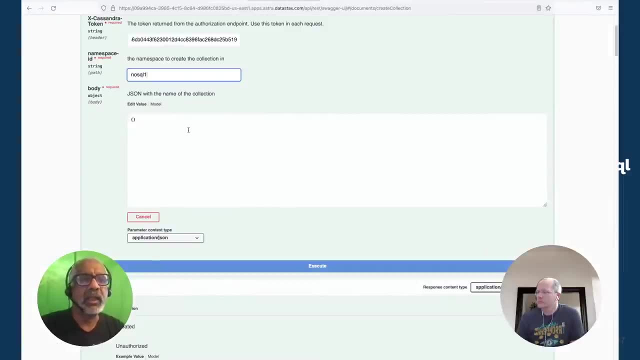 and go back to again the instructions. the name is collection one, very straightforward, like again, cut and paste. that, okay, and go back to my swagger ui and you know, instead of this i'm going to put a name: collection one. so i'm creating a collection one in the 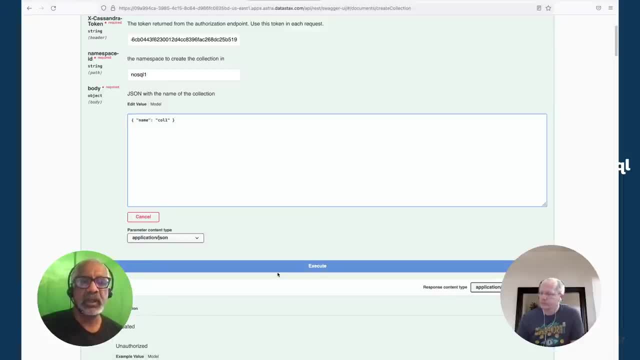 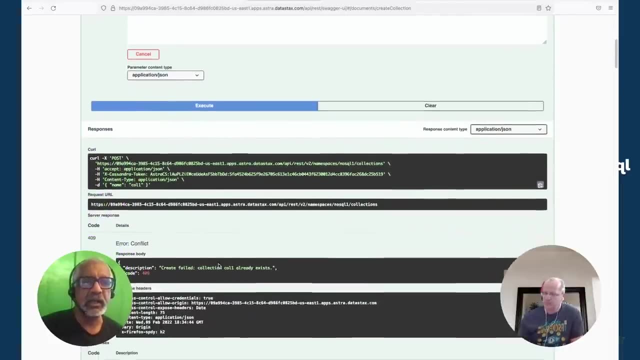 keyspace, no sql one. using this particular token, and if everything works fine, i should get a 201. okay, so you can see here, i got a 409 and i'm going to create a new collection because i created something that already exists, right? so what i'm going to do is i'm going 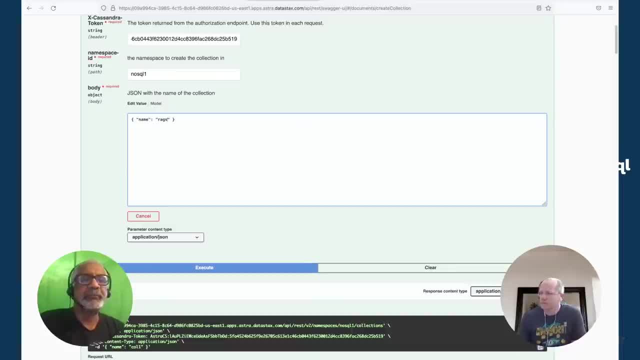 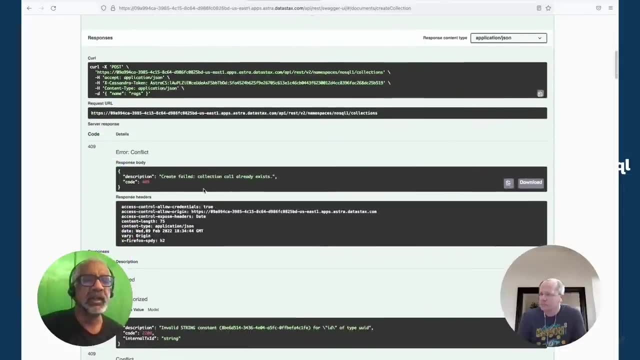 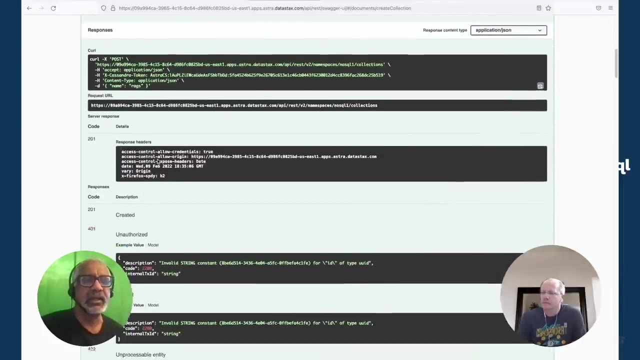 to create a collection called rags instead. right, and let's see what happens here, okay, so, so it's, it's pretty useful. you can try all this um and and hopefully now you should get a 201 created. okay, so it created the token and and you're good to go. okay, uh, did i did? 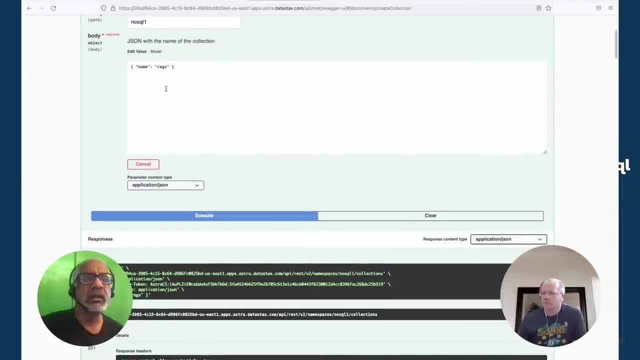 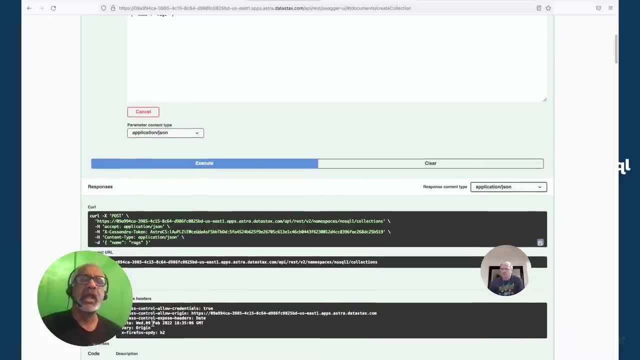 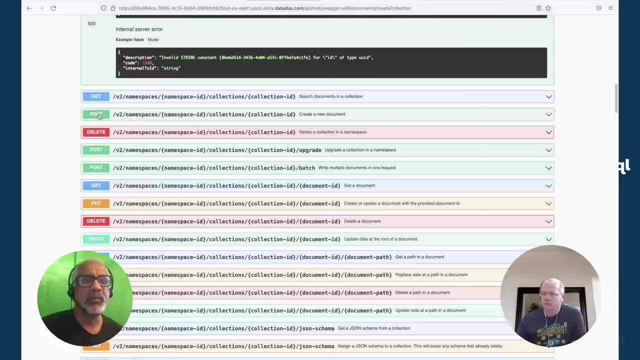 it, create it, create it, create. yeah, so 201 the response headers are there, and and you're good to go, okay, and then you can. you can go query the collection. um, let me show you, uh, what all you can do with this. you can get, you can post, you can delete the collection id. so what i can do is you know? 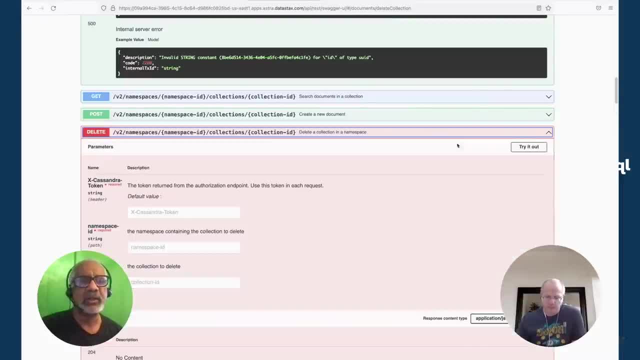 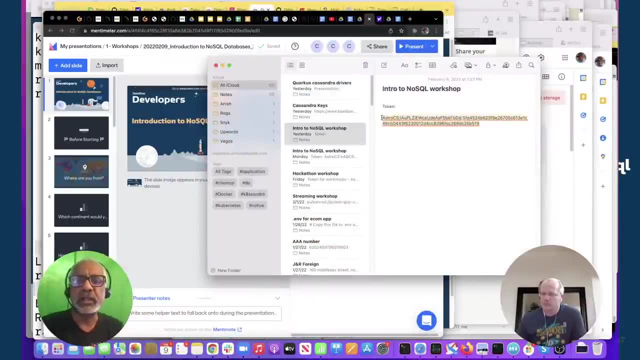 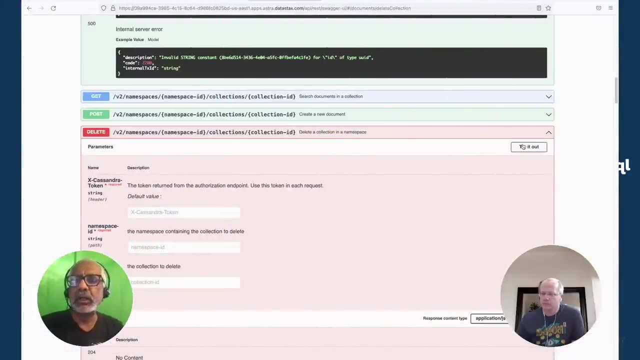 i can go here and just give you an example of delete right, because i can again. you know i have to go back, grab the token, right? you know, remember the token is very useful, so so keep that handy, go back here, put the token and hit a. try it out. hit the token. 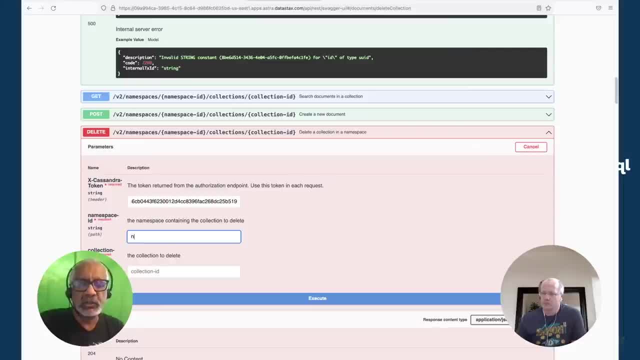 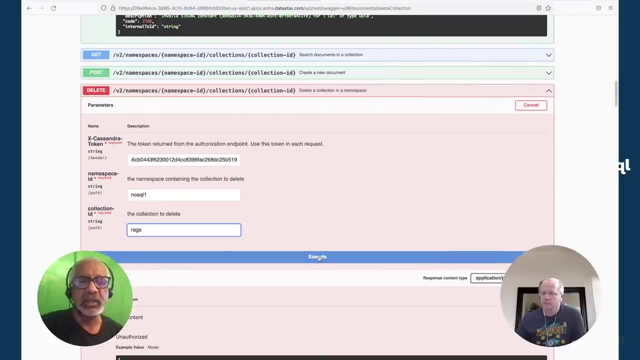 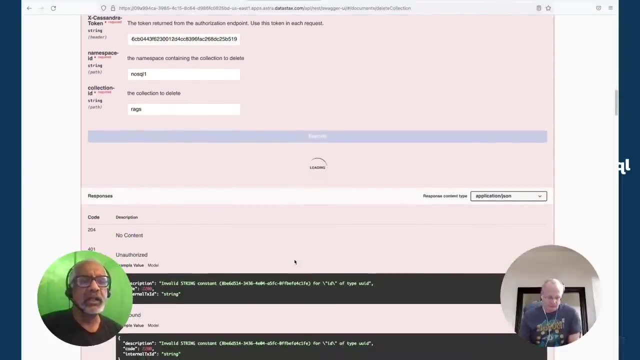 namespace ID is no sequel. one right, and let's see if this works, racks right and let's execute that. okay, so so all that you're going to do is: you know you're going to pretty much, do you know exactly this? you're going to follow the. 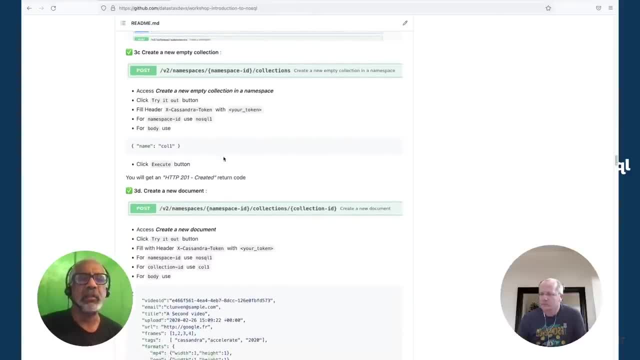 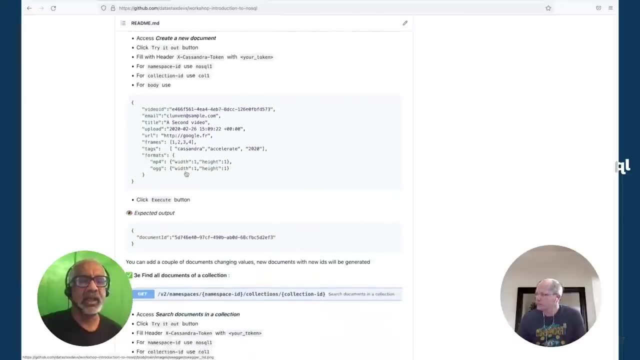 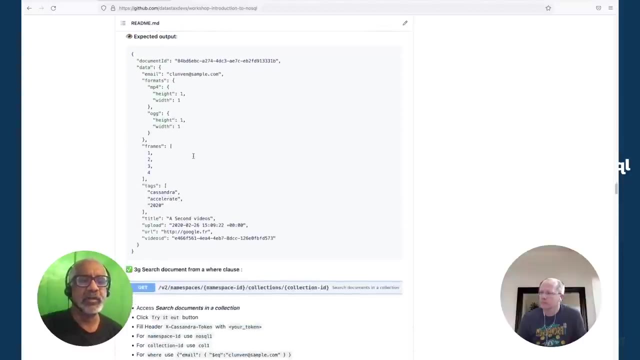 instructions that are outlined in the github page and basically what it does, is it? it lets you create a new collection. it lets you create a new document, okay, and then you know you can find all the documents of a collection you know within a particular collection and then retrieve a document from its ID you know, search the document. 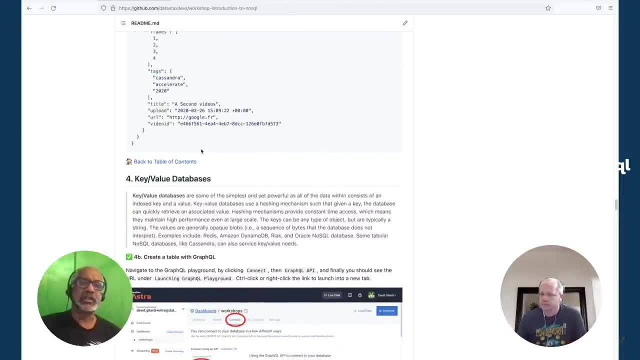 from the where class and so on and so forth. okay, so a whole lot of things that you can try out. my suggestion is: let's move on to the next you know section and then you know, you can, you can, you can try it at your own pace. okay, that seemed. 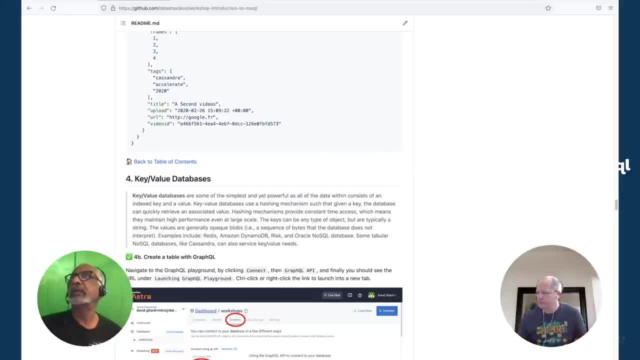 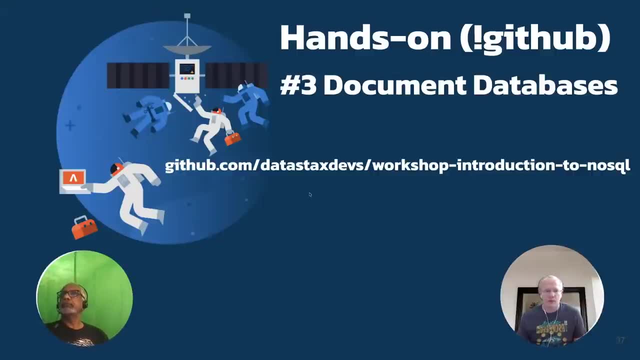 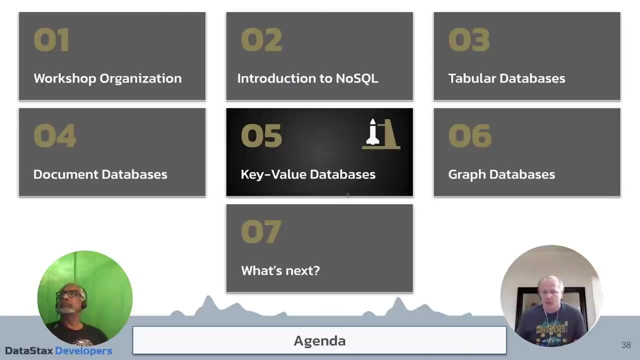 like a idea. yes, I support this idea because you can follow the instructions quite precisely to do the same thing. that ranks the thumbs up of people already have tried this out, so so with that, I come back to you. I think you're good to go now. yeah, okay, so the next one is key valuer databases: key valuer. 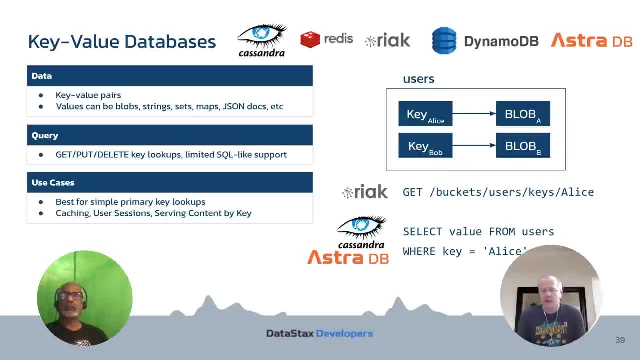 databases- the simplest one because they essentially use key valuer pairs and key is unique and, and usually the valuer can be in the simplest form- it's just a blob with some kind of data that is structured, semi-structured there, but the database doesn't look inside of the blob. however, nowadays we have key valuer. 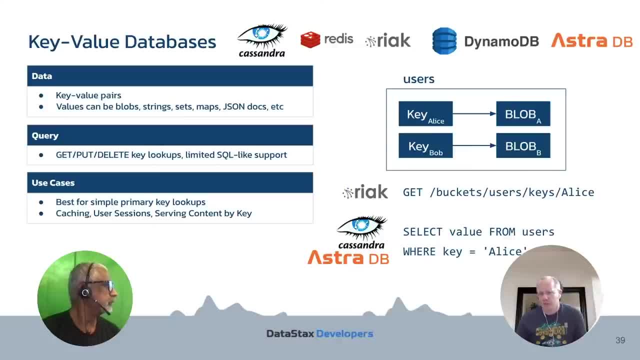 databases that actually even support indexes and full text search. so they have sets maps, they can store JSON documents again. there is this blurring between different data models, but here, yeah, we have this illustration here where we have the key, that based on the key, you can retrieve some valuer for this database. 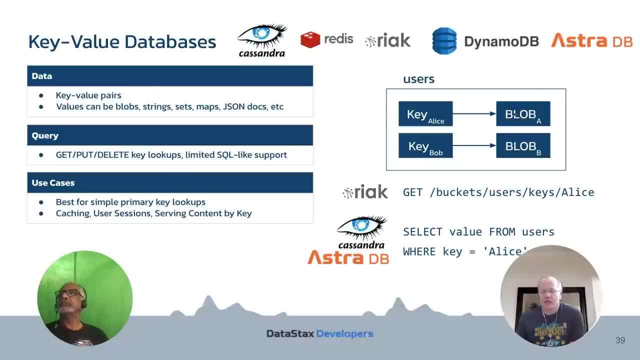 the queries are quite simple, based on key. again, as I mentioned, there are all kinds of indexes nowadays that that allow you to use key valuer and you can look inside and create a base on what's internal structure of this valuer. okay, examples here from react. this is how you can. so the users here we have. 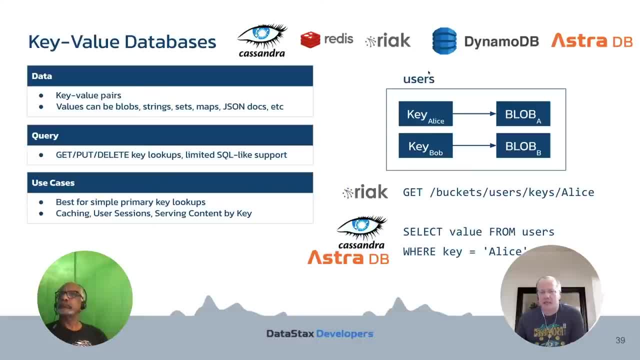 collections for document databases. here with some, some databases call these buckets. so there is a user's bucket and we can retrieve based on the key. with valuer Alice, we can retrieve the key based on the key: Alice, we can retrieve valuer blob for that particular pair. 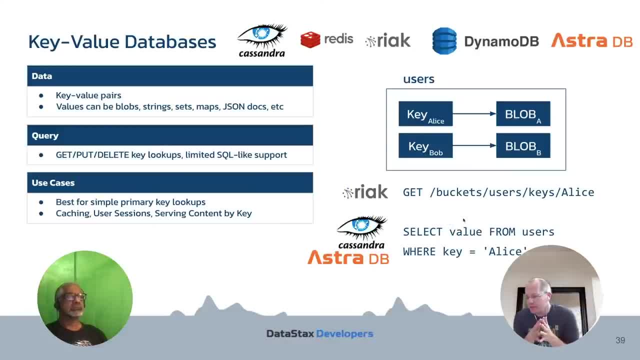 okay. but also, if you look at, if you think about key valuer pairs, it's basically like like a table with two columns where you have primary key or partition key and you have the, the column for valuer, and this is exactly what we can do in. 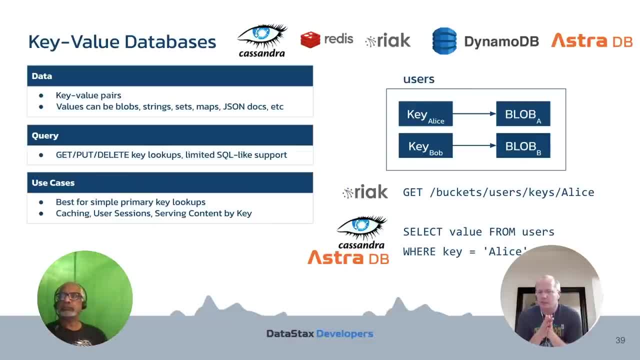 Cassandra and AstroDB. we simply create the table with users with key and valuer columns and we can retrieve that valuer based on the key. so this looks like SQL again and this is in particular in this example. this is Cassandra created language or CQL. so 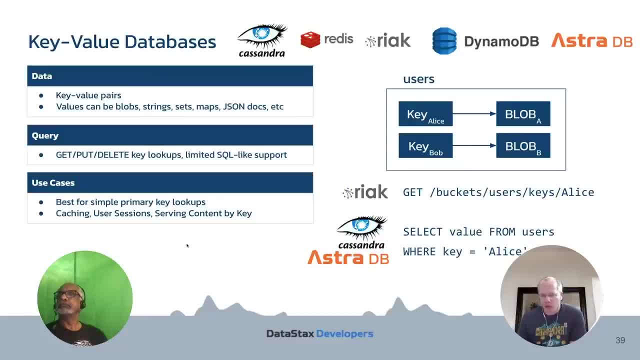 these databases are best for simple primary key lookups. even so, they may support all kinds of indexes. still, the the whole reason you want key valuer database is to retrieve very efficiently based on the key. and we can retrieve based on key. otherwise, if you need to create inside of the structure, then 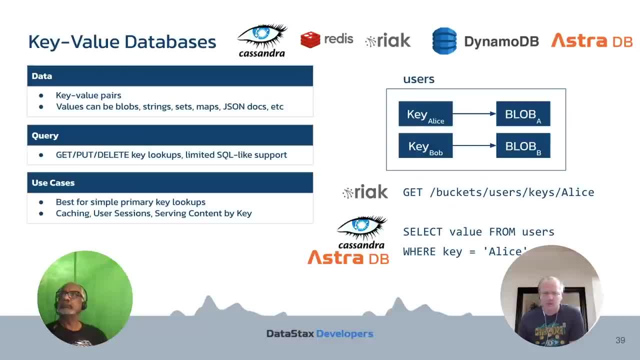 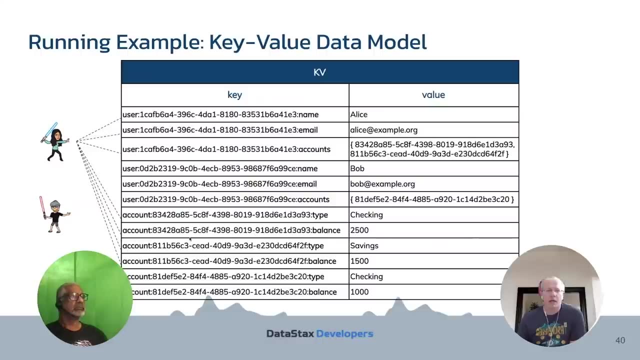 maybe you just go with tabular database or document database. that is designed specifically for that. so some use cases caching you user session management and serving content by key in general. so for our running example, this is only one way how you can represent our data set. I chose this this way. 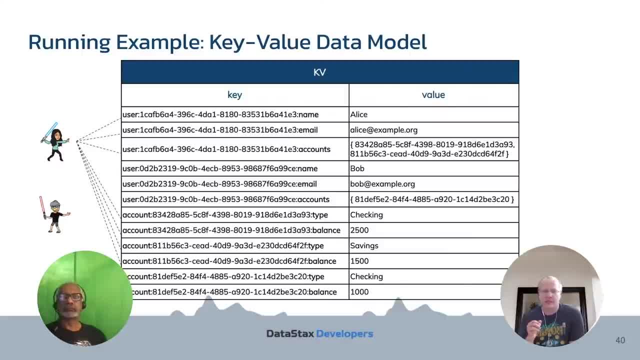 just so that you can see how to encode that thing, because the simplest way I could have done is just key would be user ID and failure will be all the information about user and user accounts, just like similar to what we have in JSON. but here I broke down. I basically each attribute is a separate key. you can. 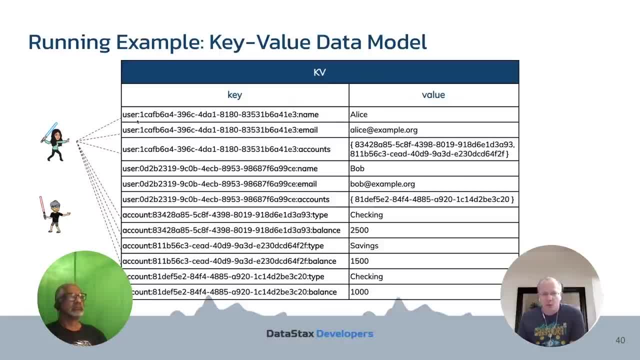 see that we have entity of type user with this ID, with attribute name and valuer Alice, and we have another user, essentially an entity of type user, the same user, the same ID, but email is a different attribute and it's a different key valuer pair. okay, so it should be. 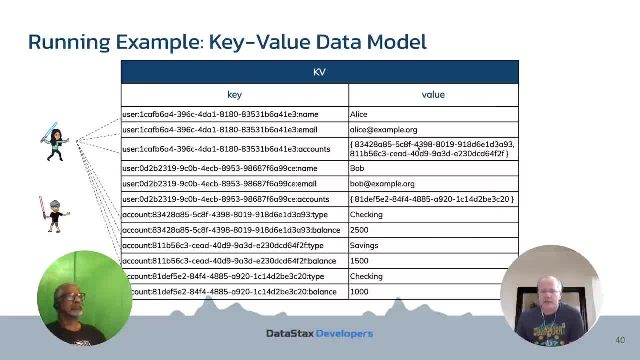 quite clear how to use it. here we have the, the set of accounts for the for Alice attribute accounts. we have the set. so it should be quite clear how to represent the same data set using key valuer data model, and should be should be suggested to you that if you're gonna use key valuer data model, then you 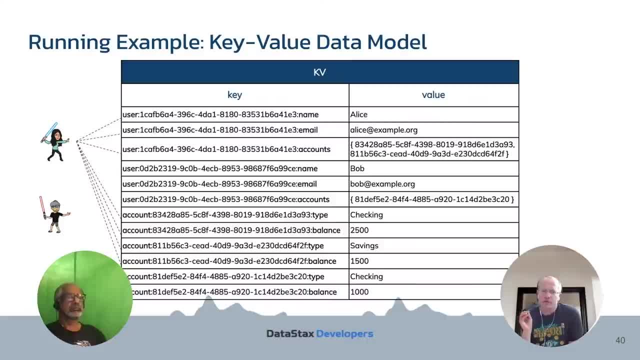 probably will be retrieving those individual failures very quickly. so this is like this: user management, session management and something like that. so you just interested in one parameter. you are not interested in a bunch of failures for that user, otherwise he would probably use a different type. so I don't mind that my over simplified view of this again coming from like a 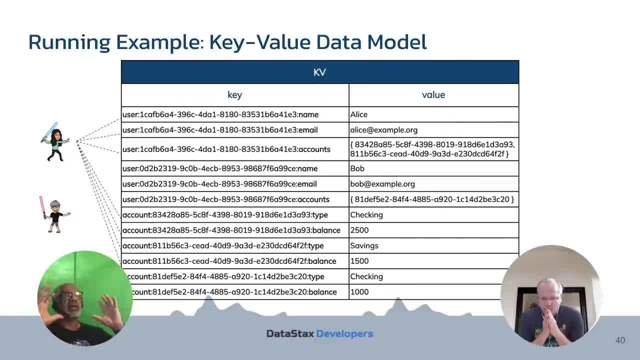 programming world is that you know, a key value database is like a distributed hash table, if you will right. so essentially that's exactly what we do: we hash the key and go to a partition and retrieve it. but now, of course, there are a bunch of details that you have to worry about, like how do you persist the data? 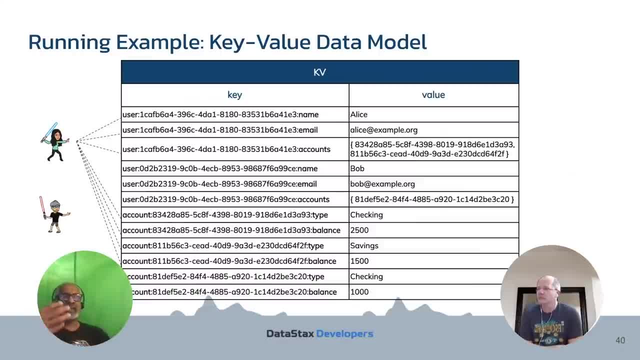 what happens if that particular node is down? do you have? second reason: all that, and that's exactly what a key value database buys you. you know you don't need to worry about any of those, but you, you know, in your head you think of it as a distributed cache or a distributed 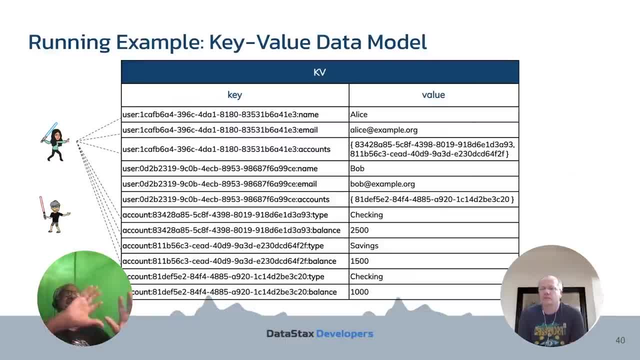 hash table and, and you know, the system will take care of retrieving the data for you automatically from whichever partition and, like Artem was saying, you know repeatedly, it is like you know, a constant time for retrieval. you know, because it's really going to the partition hitting the key, returning the 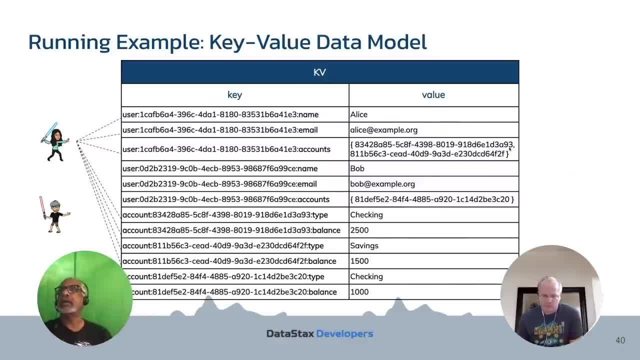 value, that's it period, right, and it's great for those kind of use cases. so, yeah, it's a great way to do that. yeah, all right, do we have? yeah, go ahead, that's a good point. yeah, that's a good point. I don't know if you want to do. 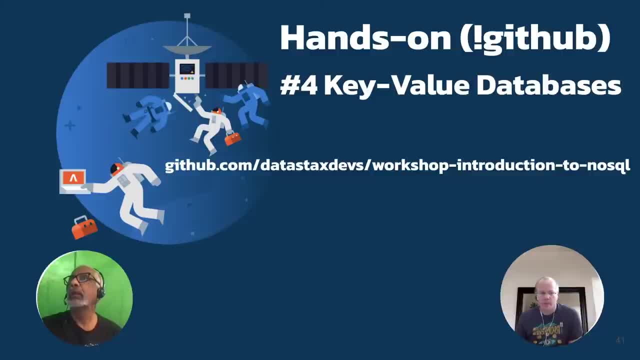 this exercise, just for the sake of time. how about we skip it? my suggestion is: let me walk through that. walk through meaning I will. I will not do it, but but I'll kind of walk through the instructions, okay, and then. and then what we can do is: yes, we can jump to the next section. is that reasonable? yeah, 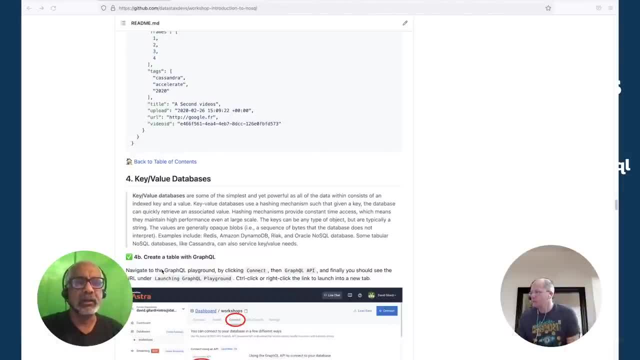 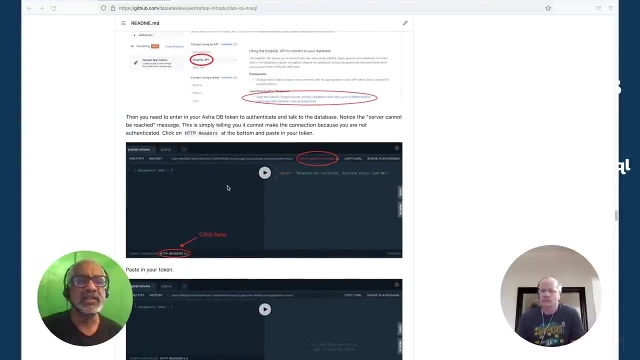 All right, That's good. So let me go back here. Okay, and key value databases. again, very simple to understand, very easy to use, But this, you know, using this GraphQL schema- and GraphQL is a little bit hard to use, you know. 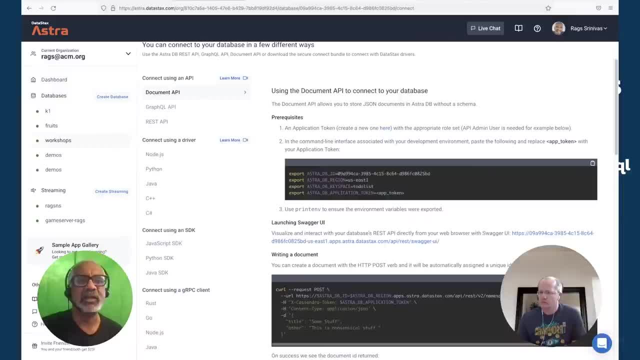 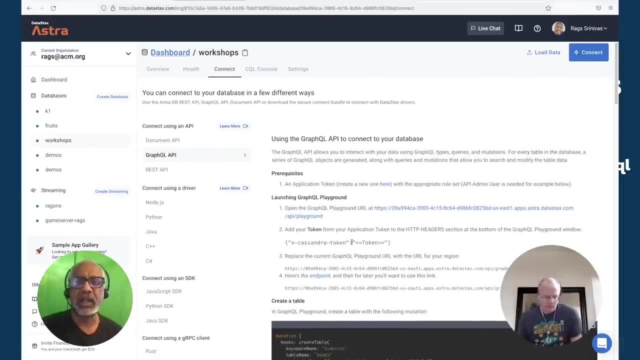 I mean not extremely hard, but at the same time you know it takes a little bit of getting used to. The first thing you're gonna do is you know you're gonna go to GraphQL API and then you know basically connect. 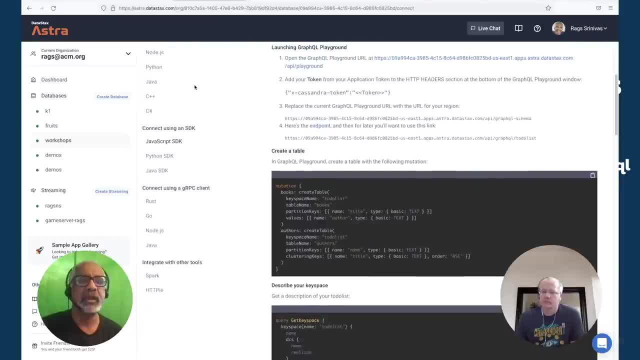 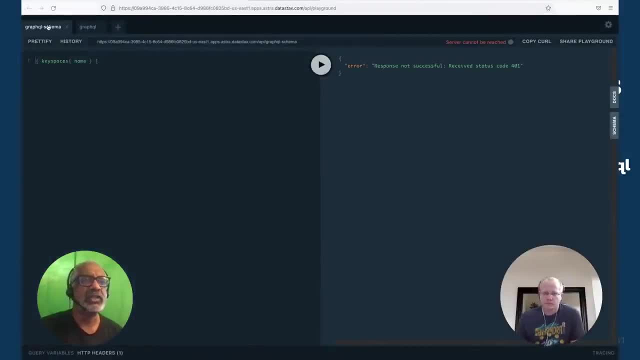 And all of the instructions are in there. so you're gonna do that. You're gonna connect to the GraphQL playground- you know which kind of looks, something like this, right- And then you're gonna have these two tabs: the GraphQL schema and the GraphQL. 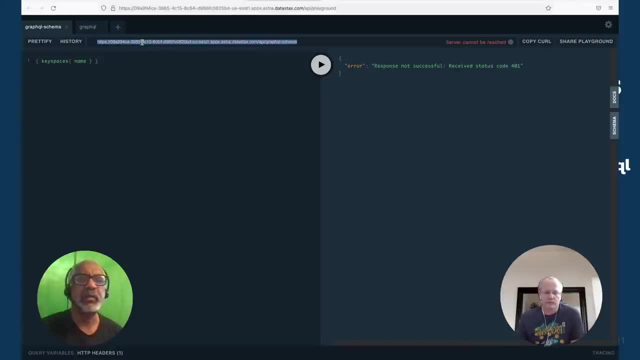 My suggestion is, you know, take this, this URL right, Because you're gonna be using this. you know when you're trying out the instructions and keep it handy because you may wanna get back to it. This uses the database. 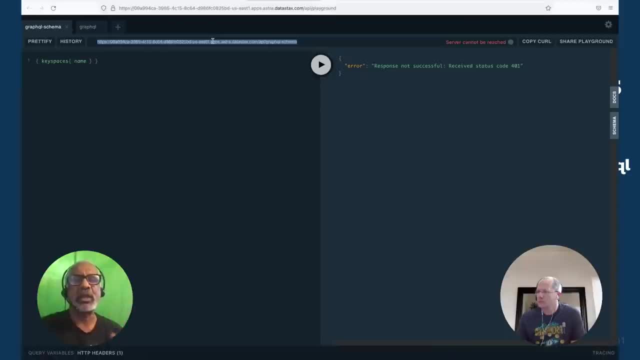 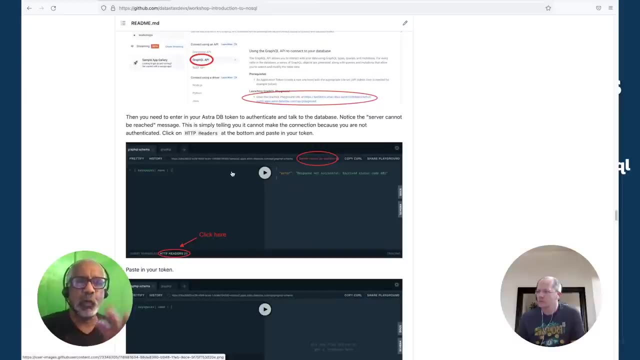 database ID, you know which region it is and all that. But I don't need to worry about this, just keep it handy because you may wanna get back to it at some point. But this kind of walks through the whole thing, right? 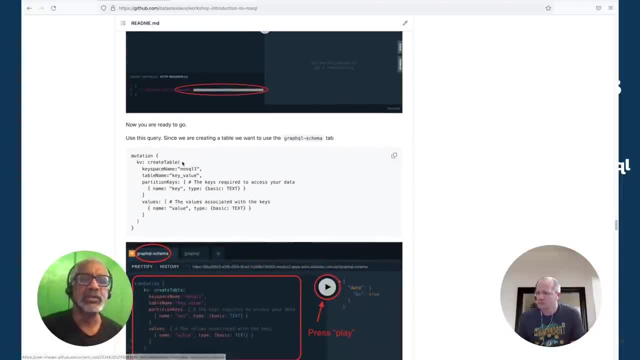 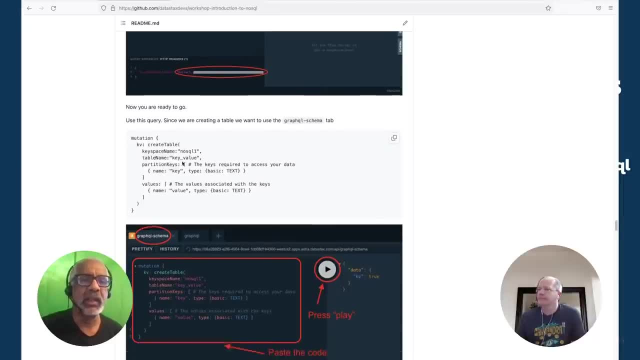 You know GraphQL, and then what you do is we use what are called as mutations, And this is the way you know in which you can do a whole lot of stuff with GraphQL, And essentially what we are doing here is we are creating a table called KV, right? 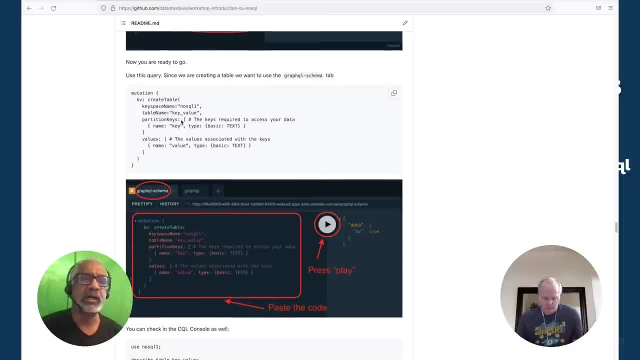 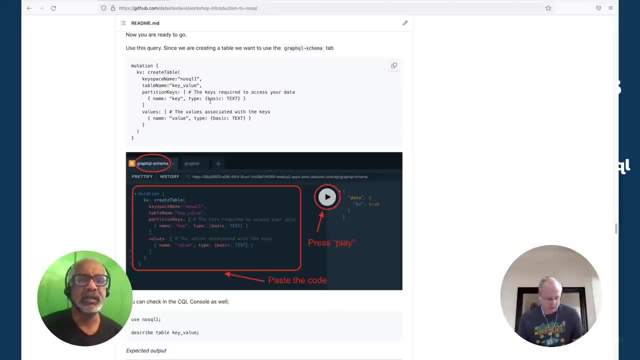 Okay, and the key space name is nosql1, which is really what we used before, And then we have a table name called key value And essentially here you have a partition key called name type, basic text. Very simple, right. 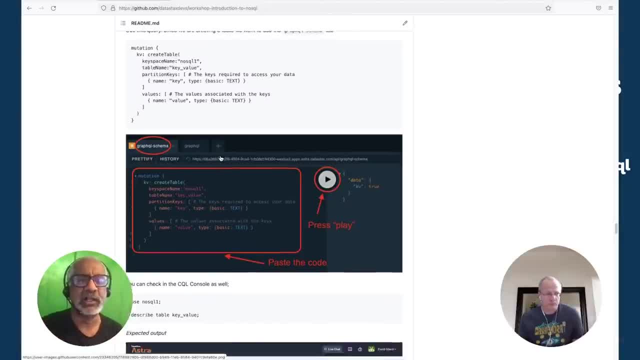 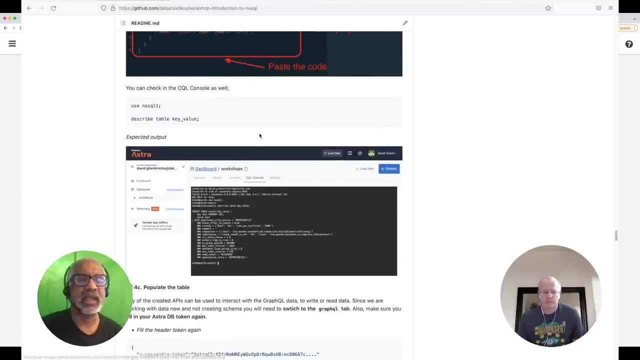 You have a text, text, a key and a value. That's all it is. And what you know, there's kind of you know. initially you create the schema and then you press the play And then what you're gonna do is: 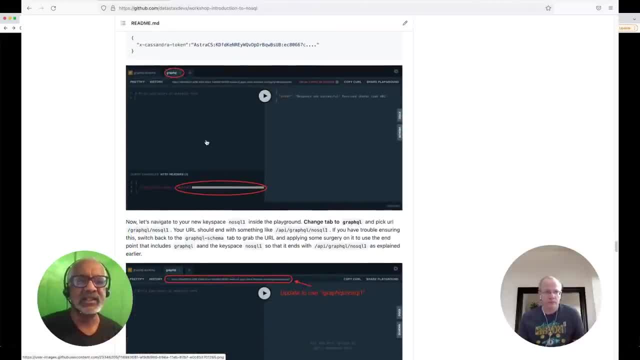 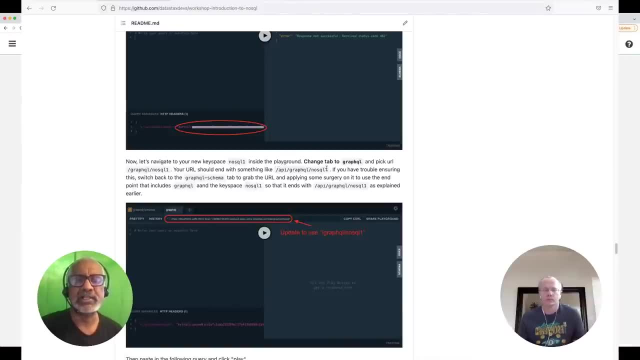 you're gonna go back to the GraphQL and then start inserting the values, And here's where you know your URL should end with something like slash API, slash GraphQL, slash nosql1.. Otherwise, you know sometimes what happens is, and let me show this to you. you know. 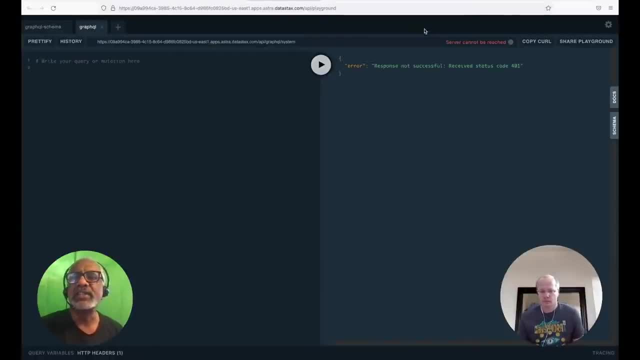 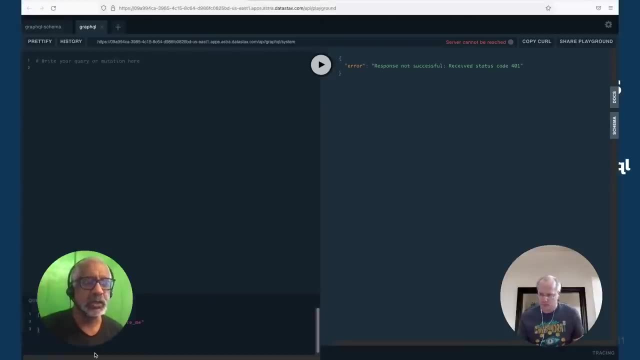 if you hit the GraphQL, you know you'll see an error like this server cannot be reached And the reason behind that is because I haven't pasted the token yet. So to be able to paste the token, you know you have to go and populate this particular token. 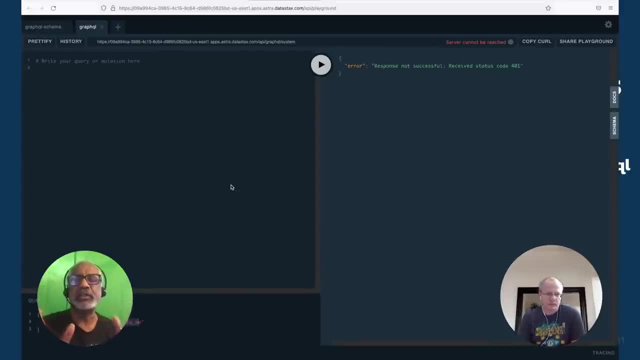 But sometimes you know, if your browser is not the full size that you can see here right, then you may get into some kind of issues. So that is why I recommend using this. you know, copying this, you know URL. 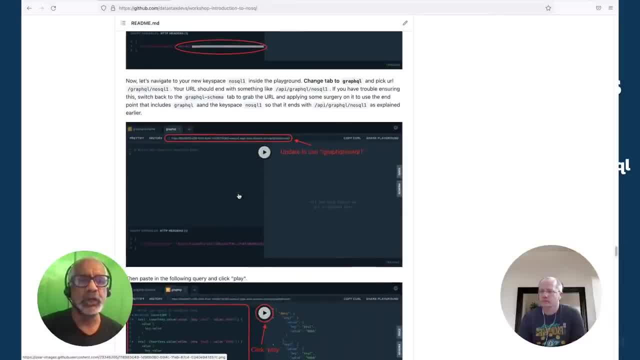 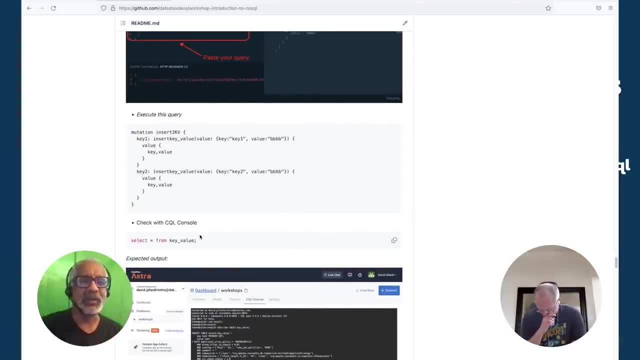 because it might come in handy later. Okay, So you're gonna create the table. Then what you're gonna do is you're gonna add- you know- values to it, And then this is the nice part, right? You know you're gonna go back to your SQL console. 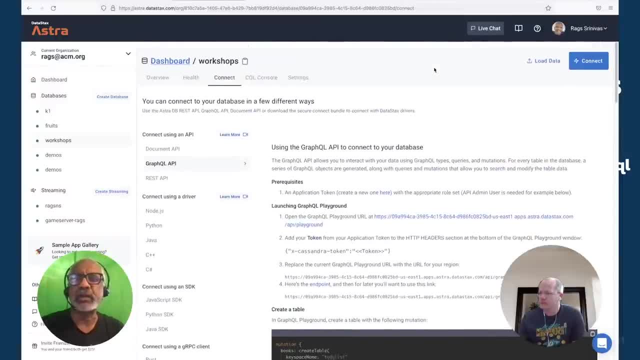 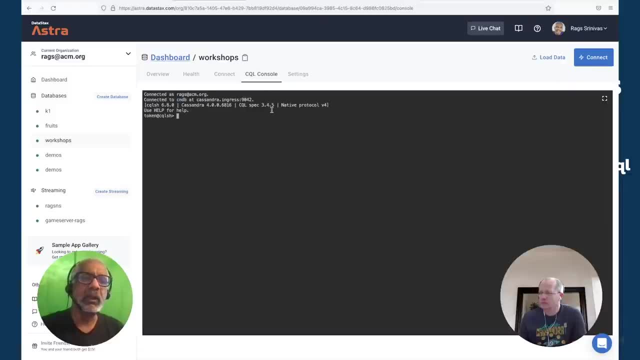 Okay, and let me show that at least in action, right, Because I've already created this, right? So I'm gonna go back, connect to my SQL console, okay, And I'm gonna use the same key space. no SQL one, right? 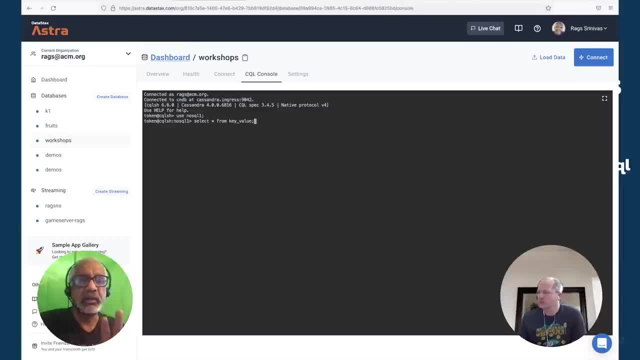 And I'm gonna cut and paste what was in there. Again, not a good idea to do select star, but you know, because what you're doing now is going to each and every partition, you know. So, depending on how big it is, 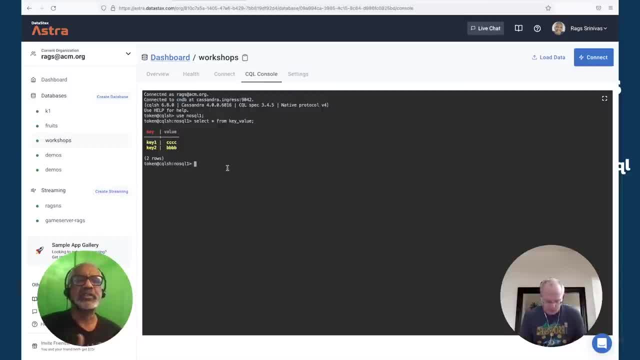 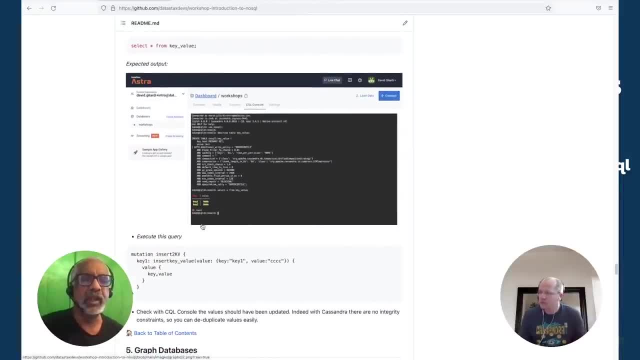 I mean, of course, I don't have too much here. So you know, for the purposes of illustration, this is probably okay. But again, you know what these instructions go at, pretty, you know length about. you know how to do this. 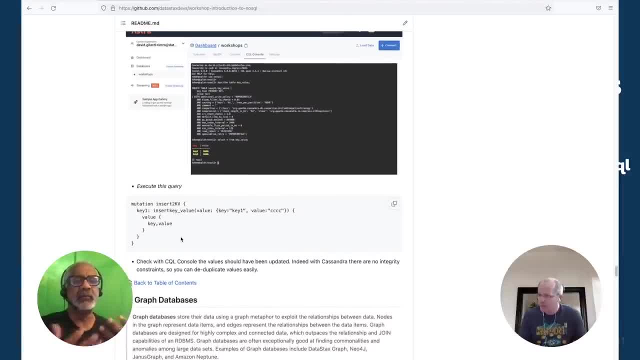 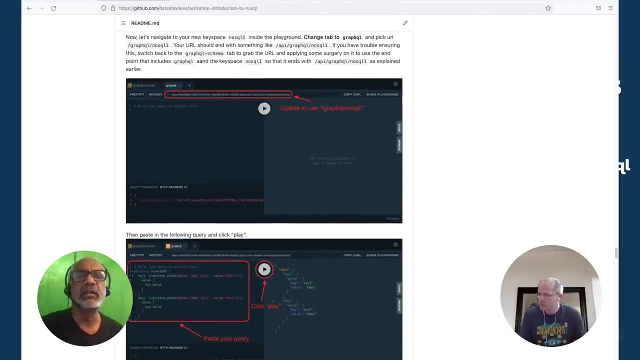 And you can kind of improvise this a little bit yourself and kind of change this around, But essentially what you're gonna do is you're gonna use these two, which is- let me go back here- the GraphQL schema to create the table and the GraphQL to actually insert the entries. okay, 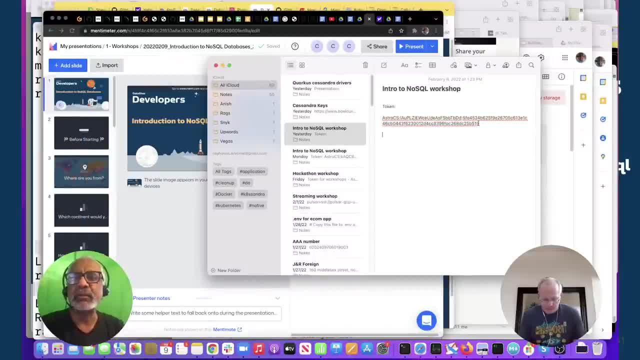 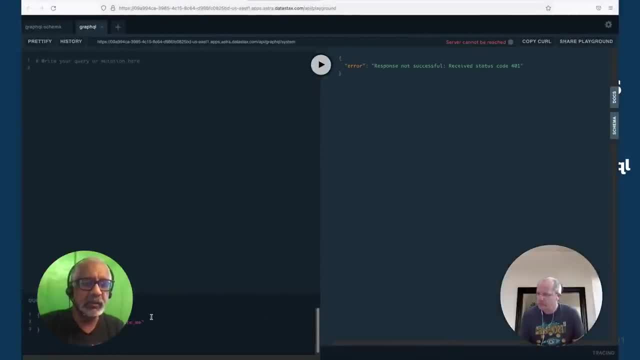 And let me you know, just so that I'm not pulling from thin air, I'm gonna copy this token, okay, And go back, and if you populate me, hopefully it should, it's actually. let me go back to GraphQL schema. 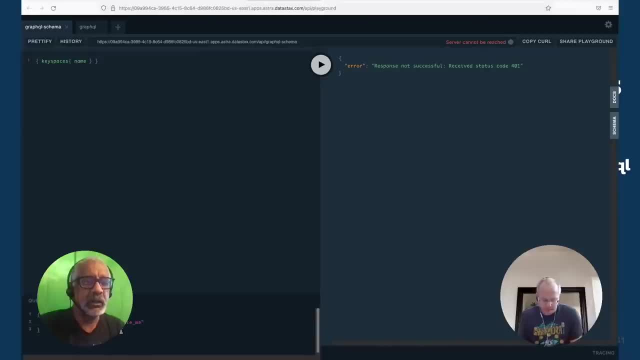 because you'll see the same thing there as well. Okay, And I'm gonna put the token and hopefully it should validate. okay, At least you know it requires authentication, but you're gonna get the idea. okay, You can, you can, you can get you know, you can do that. 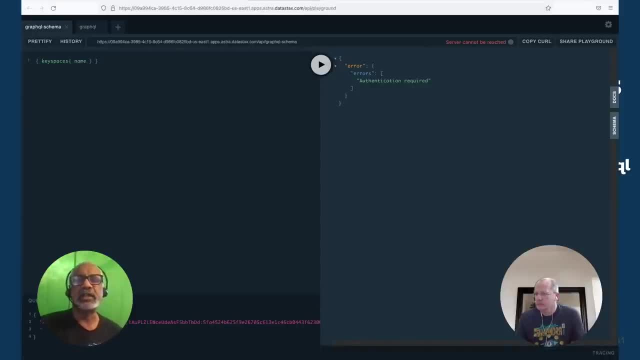 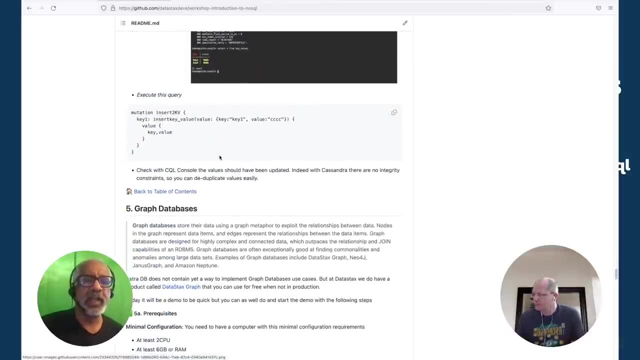 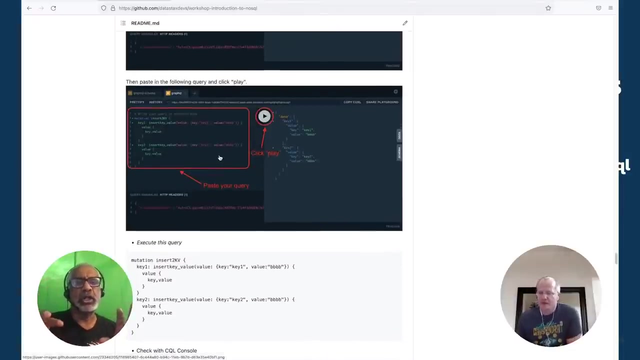 You will have to put this token first before you can get started, Otherwise your authentication is not there. I know it was a little bit fast here, but again, in principle it's the same. The reason why we chose the GraphQL Playground is because it does a whole lot more than this. 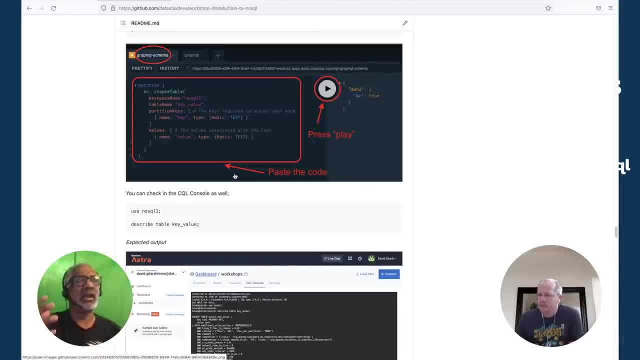 but again, to kind of give you a flavor, I know that Artem touched upon these different kinds of databases, but from a programmatic perspective there are different ways of accessing this as well, and that's kind of what we're showing here. 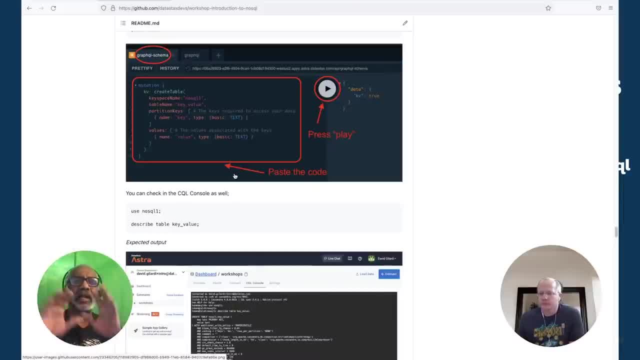 So once you start putting them in a matrix it becomes a little complicated, but the idea is that take them one by one. I think most of you are very familiar with SQL, now SQL Console, Get familiar with GraphQL and then you know. 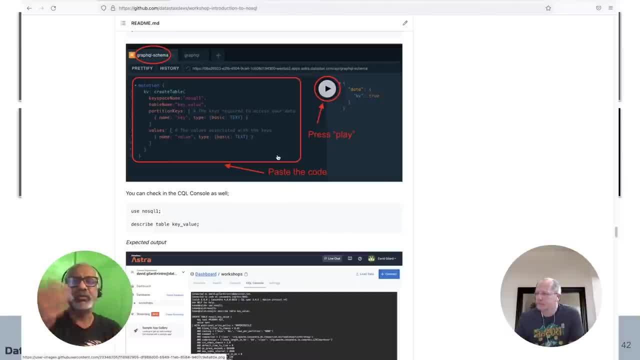 take them one by one, and then you know, take them one by one, and then you know, go on and use the swagger, or you know whichever suits your fancy. you know you can do that, I know. the last thing that we want to talk about is graph databases. 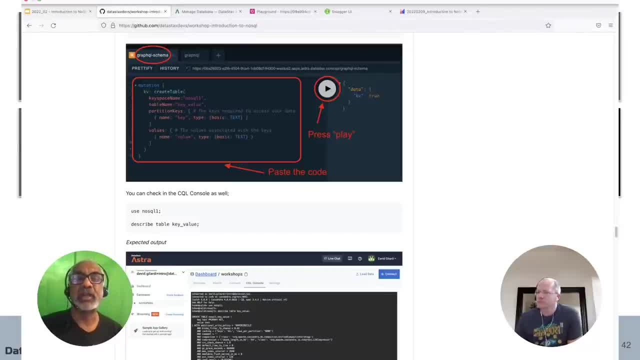 and I know that you know Artem prepared a demo. I'm not sure if you have the time for that, but I will hand control back to Artem and you're good to go Hold on hold on one second, Yeah. 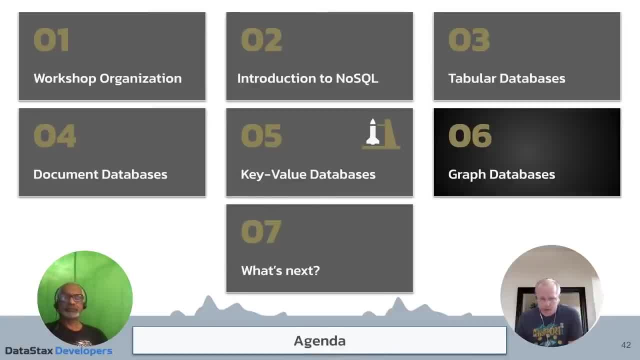 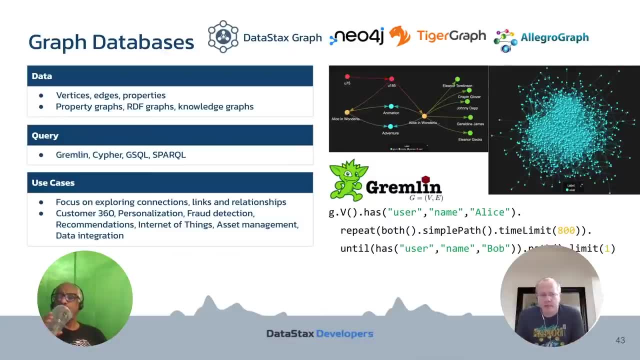 Yeah, So graph databases is the last one, And graph databases use graph as a data model. Graph has vertices or nodes. It has edges that connect those vertices or can be called links or relationships, And there are also properties that describe edges and vertices, basically like attributes, right? 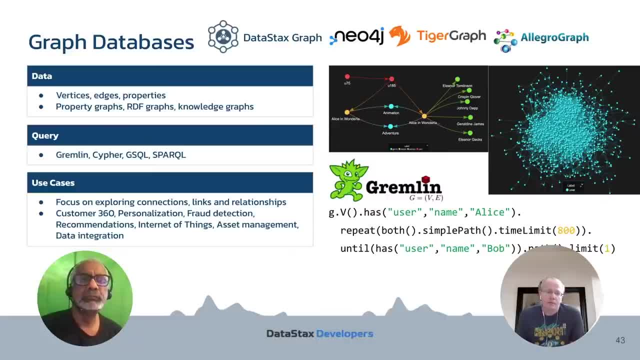 So there are different, also different types of graphs. So some databases use property, Some other databases use RDF graphs. I'm not going to talk about differences at this point, but here we have examples of data stacks: graph, Neo4j, AllegroGraph. these are property graph databases and AllegroGraph uses RDF as a graph data model. 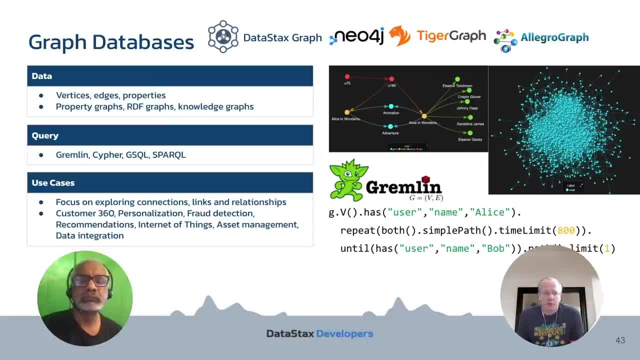 The query languages again can be quite diverse. There is a Gremlin that we're going to use, Yeah Yeah, Which is more like a functional language: Cypher and GSQL and Sparkle- three different languages, And you get GSQL, GraphSQL, so it should be similar to SQL. 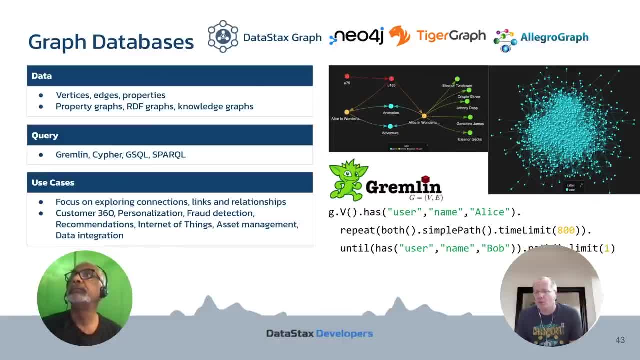 And these three, the last three. they are more of declarative languages, where you define a graph pattern that you want to match against your graph structure. But Gremlin is more like a traversal language, where you want to define how you're going to use it. 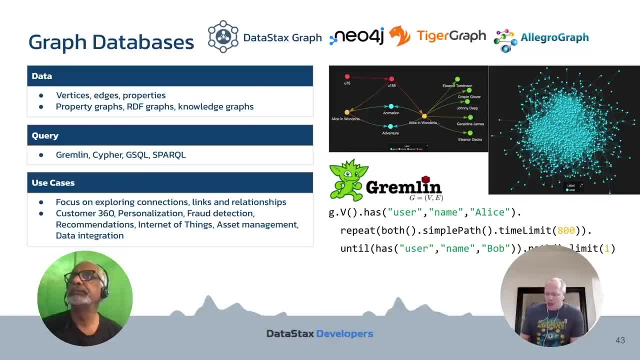 You define how you're going to traverse that graph structure. So use cases. so this example of Gremlin here let me just walk through. So, starting with our graph traversal source, but essentially think about it as graph, we get all vertices that have label user and name Ellis, and then we will repeat the following: 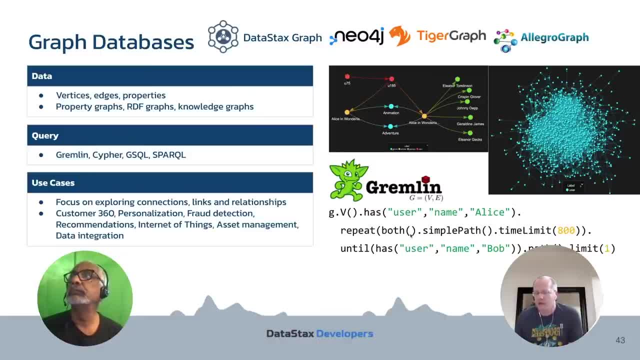 We will traverse in both directions, So edges have direction And we will make sure that it's a simple pass. There are no cycles, There will be time limit- how much time we want to spend 800 milliseconds doing that? And we will keep traversing until we see another vertex with label user and the property name is value of Bob and we will get the pass. 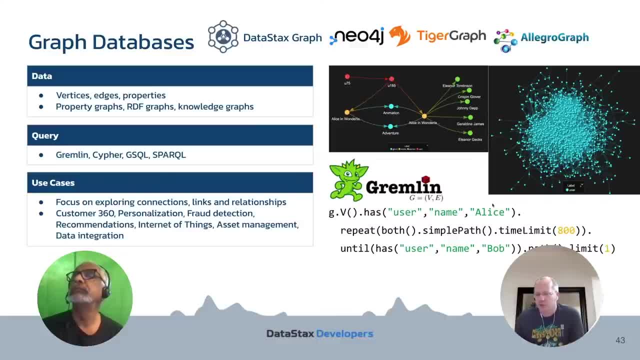 So essentially what we're doing here we're trying to find the shortest pass between Ellis and Bob vertices in our graph. So use cases here is exploring connections, links, relationships- they all have to be related to that. So it's a little bit more than just a simple okay, retrieve by key. 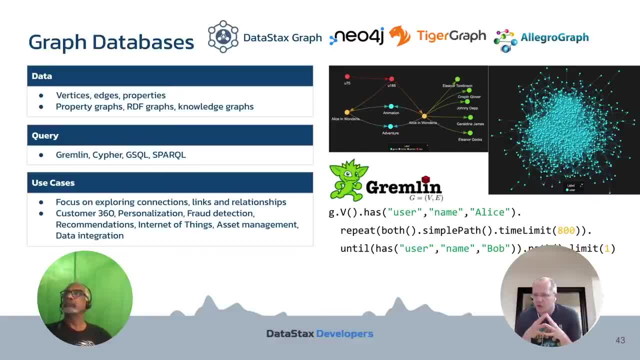 No, what's the connection between Ellis and Bob? And you don't know how many hops you need to take. Is it two edges you need to traverse, or is it five edges you need to traverse? So customer 360, personalization, fraud detection, recommendation and so on. 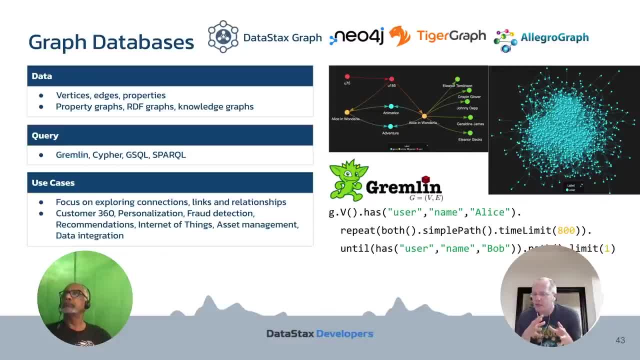 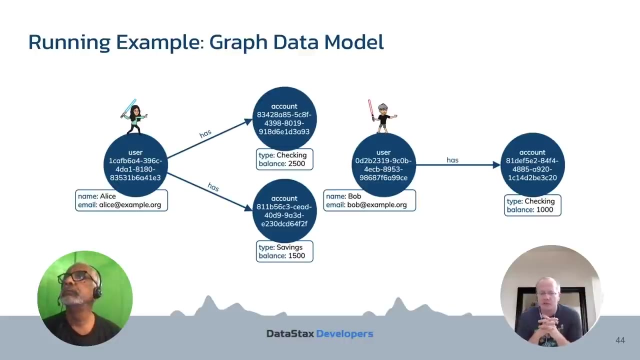 But you can see from these use cases, They frequently involve some analytical aspects, A little bit more than just collecting data and quickly retrieving it, but also kind of a little bit analysis starts to get used in those particular applications. So the data model is so flexible and can actually you can use it to capture any other data model that we discussed, including relational. 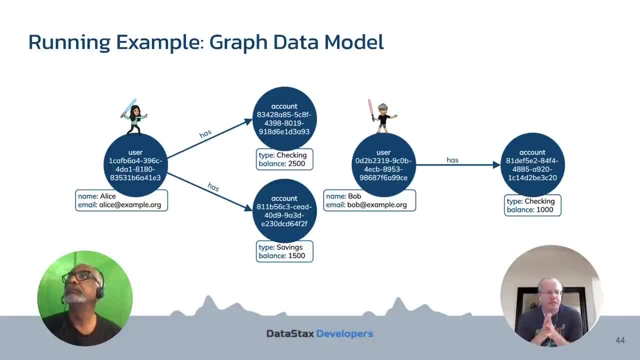 But there will be some disadvantages too. So here In our example we have user with particular ID. It has two properties: name, Ellis, email, and there is an edge with label. has user has this account with of type and balance. 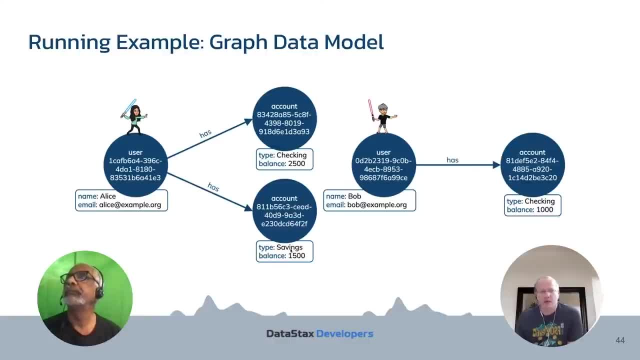 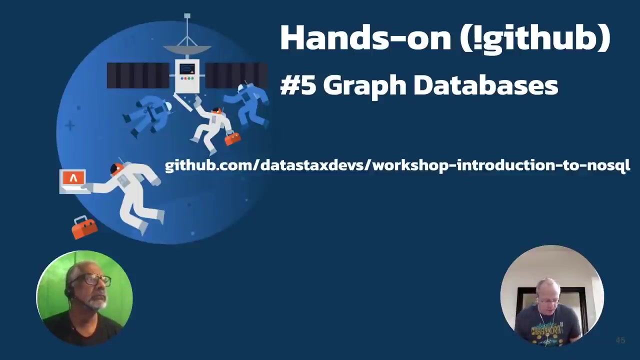 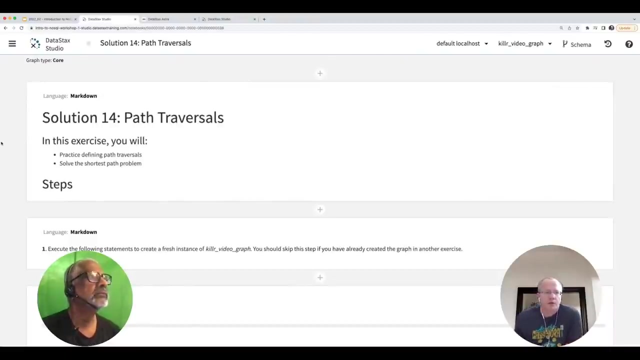 And the user has another account with different ID and there is a type savings and balance property. Fifteen hundred, similar for Bob. So it's quite Quite, It's quite easy to use, to model using that, but still there is. there will be data modeling involved and for the exercise, for the hands on, I'm going to just show you a quick demo using these so-called past traversal, so using gremlin and gremlin a kitchen, using graph traversals. 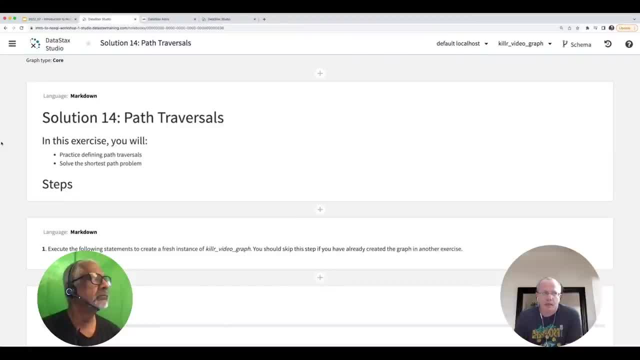 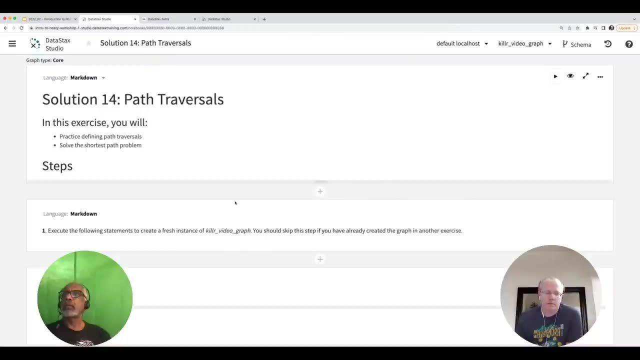 The. The system that we're using behind the scenes is data stakes- data stakes graph- And this is that client called Data Stacks Studio that allows me to interact with with the database. So I already pre-created the database for you, so we don't spend much time. 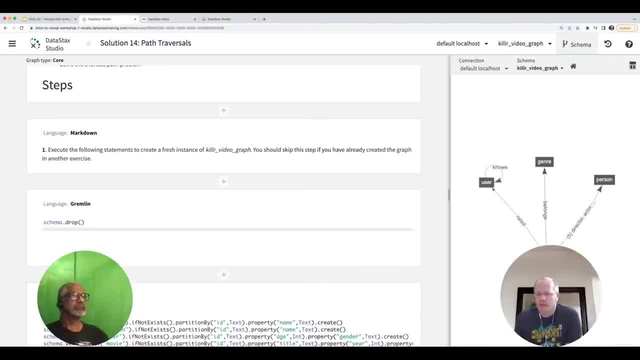 It has schema. The graph has schema, so it has vertices with labels: movie, user, genre and person And there are edges with labels. And there are edges with labels: movie, user, genre and person And there are edges with labels. 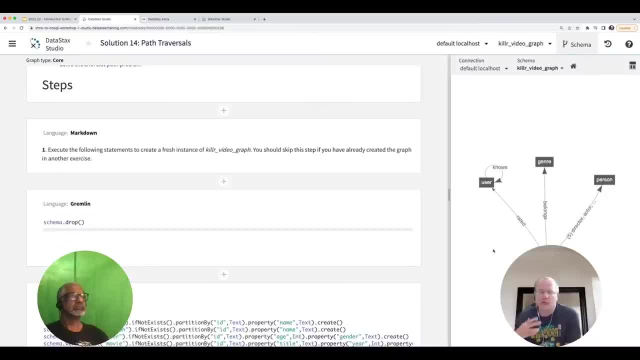 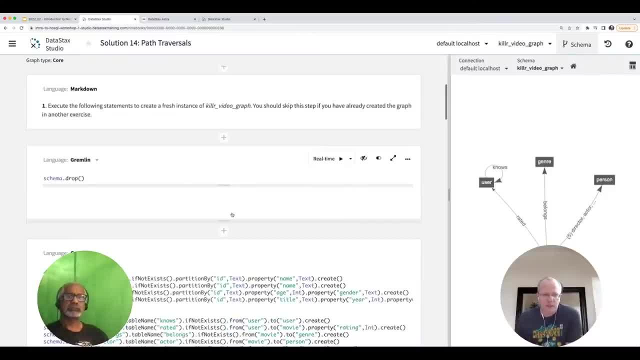 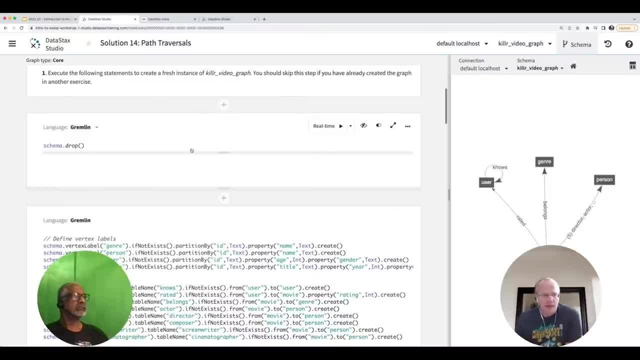 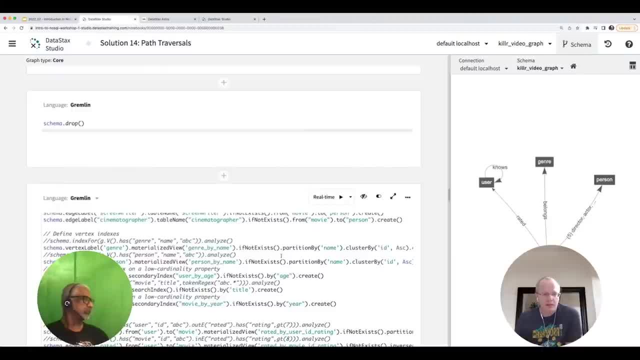 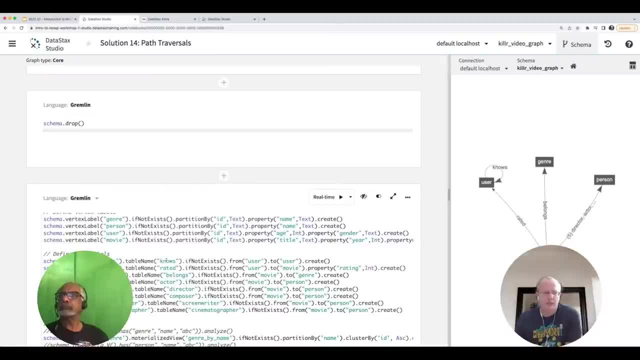 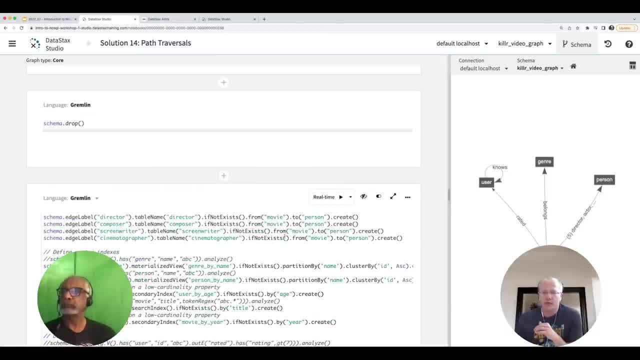 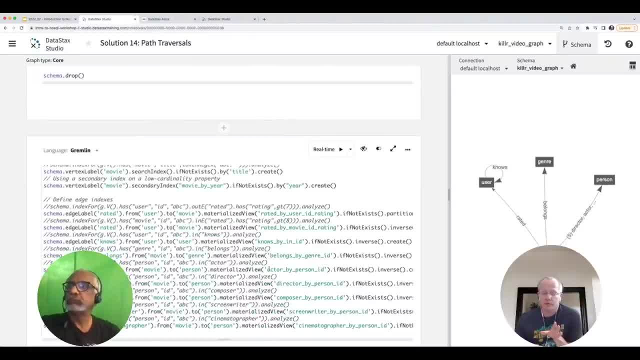 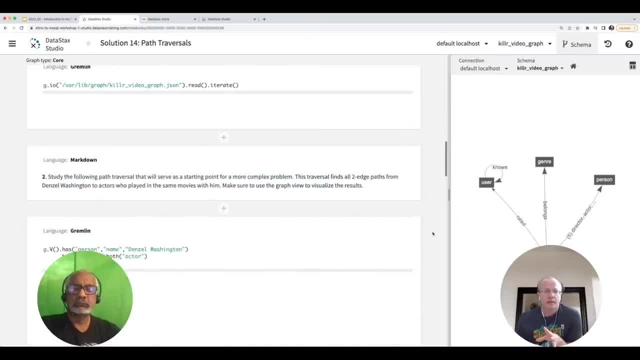 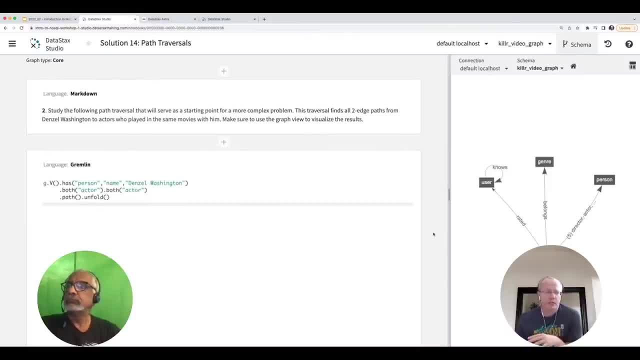 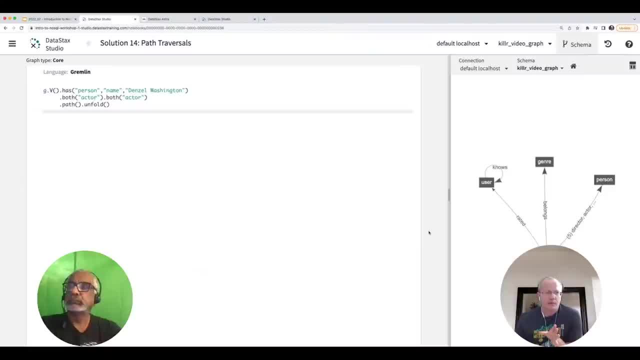 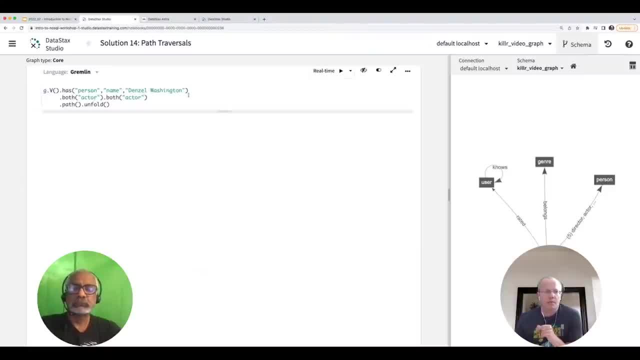 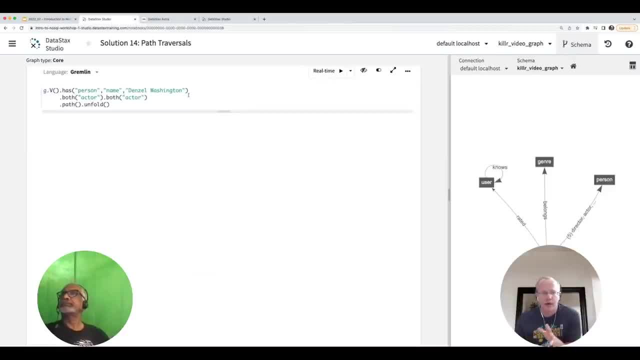 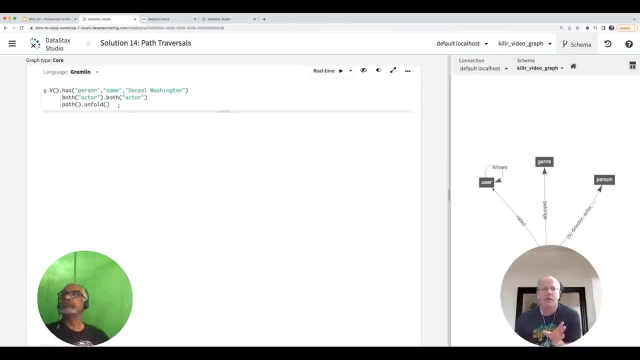 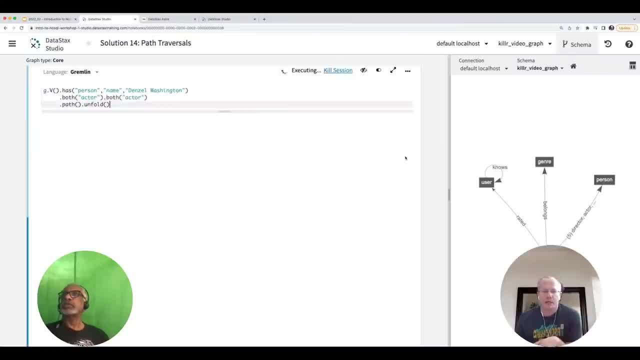 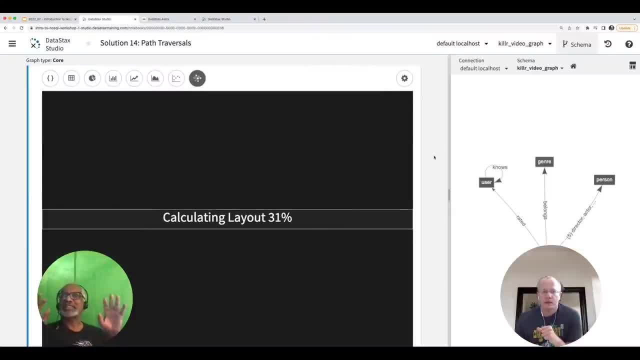 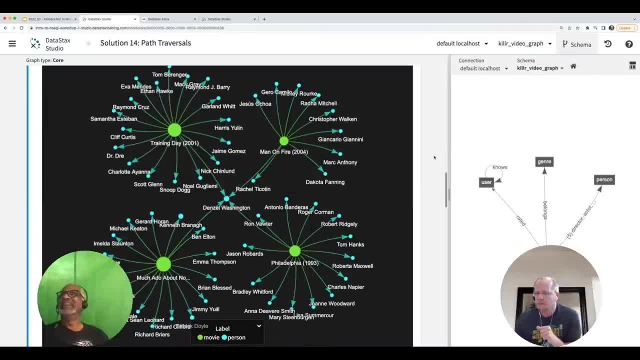 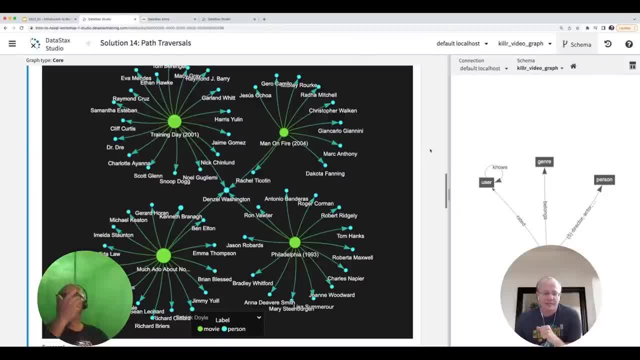 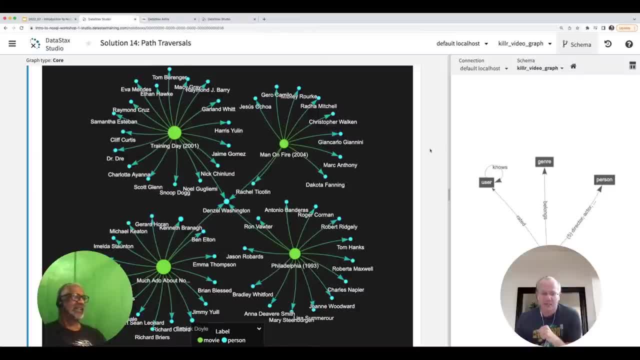 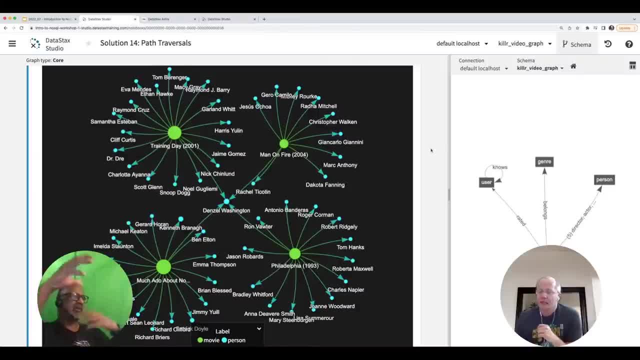 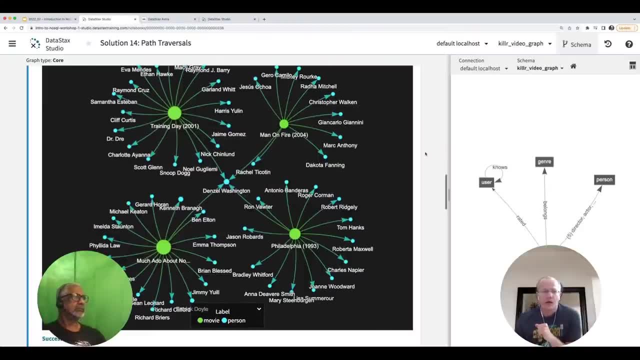 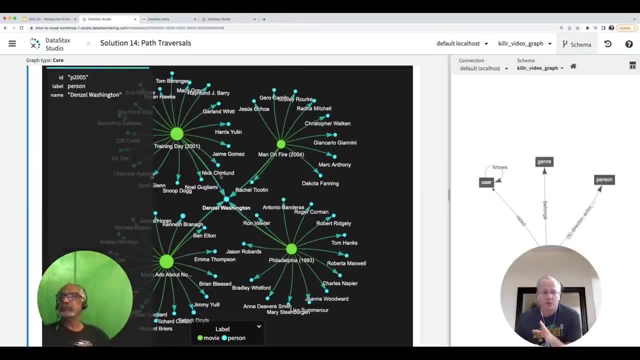 just looks so cool, right, It's really expressing all the different relations, different degrees and so on. Yeah, so what we did? we went from this vertex, Denzel Washington, and we traversed edges in both directions. These are actor edges. so we went to the movies and from there we went, traversed actor edges. 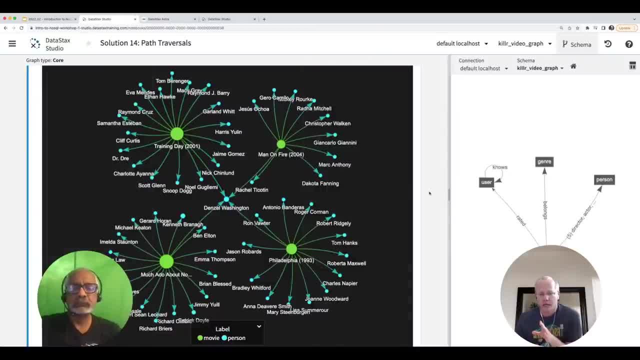 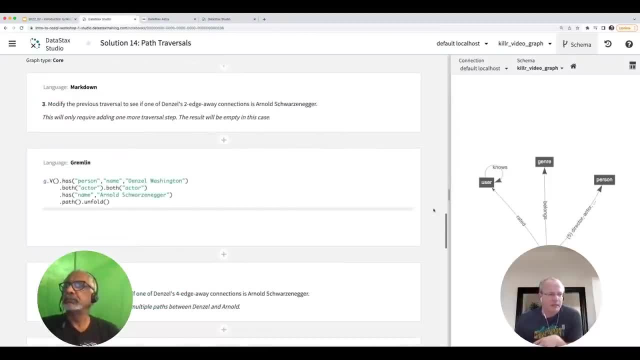 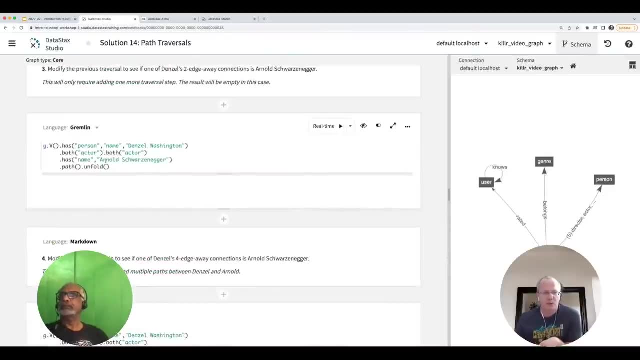 again. so we found all the other actors who participated in the same movies with Denzel Washington. So this is one example. Let me just select another example. So here is a simple example where we want to find the paths between Denzel Washington and Arnold Schwarzenegger and we traverse 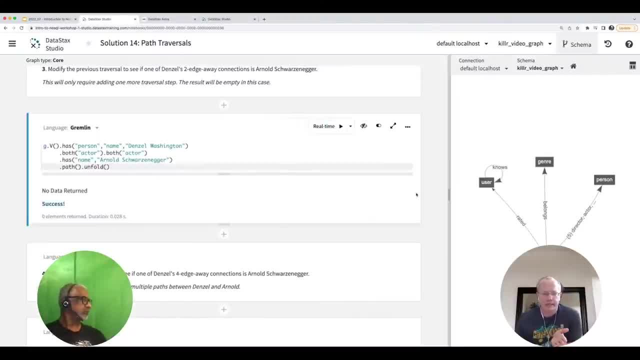 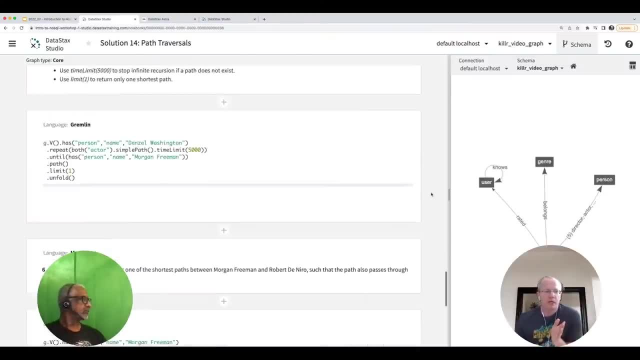 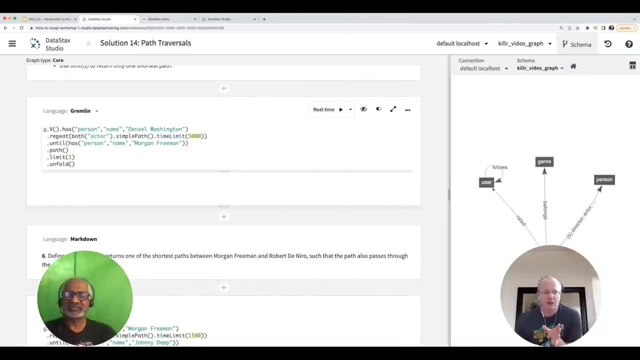 actor edges twice, but we will not find anything. There will be no results. The path does not exist. So what we do here is we- this is a simple example that you've seen in the slides, but essentially we will do the repeat construct here, repeat step. So it's like: 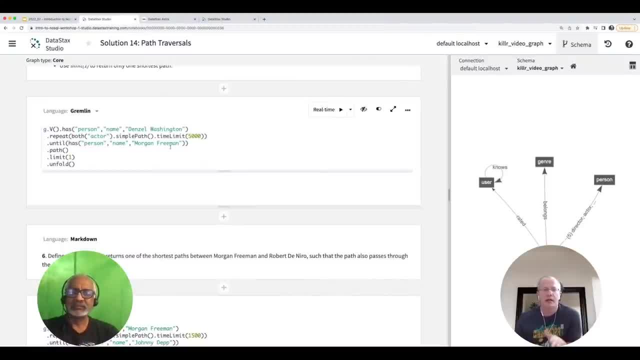 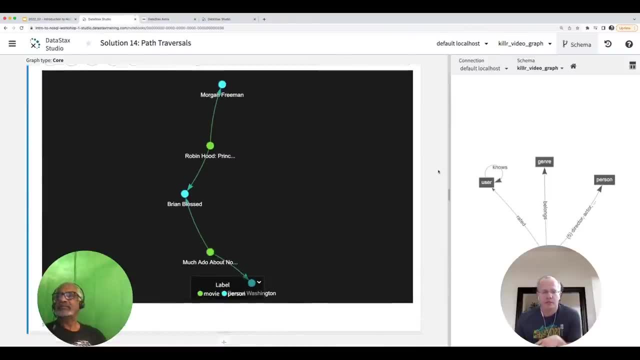 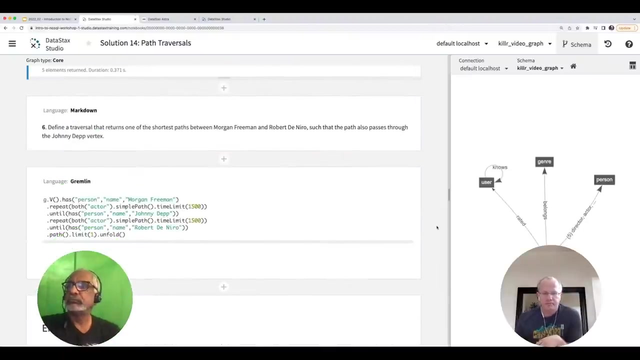 it's going to be a loop, we're going to be running it and to find that shortest path between two actors. And you can see it exists, and there are a couple of movies involved, but the path between the two actors exists. Okay, and so let me show another. 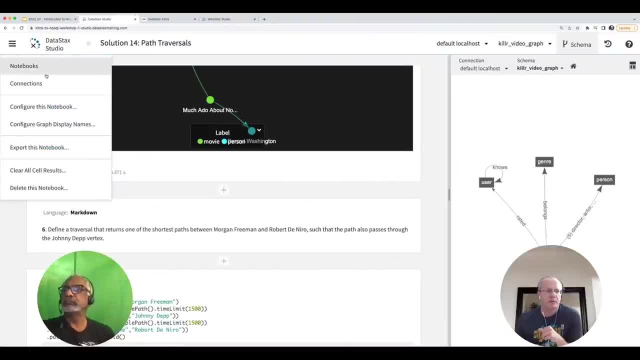 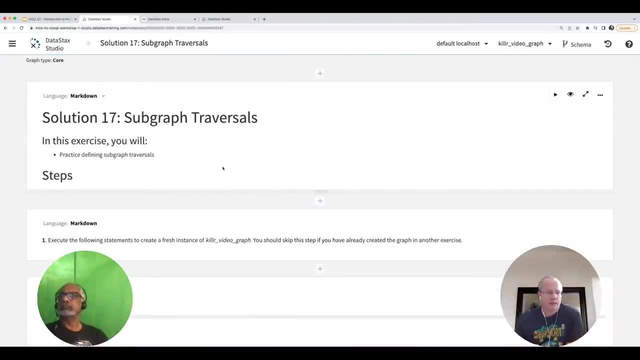 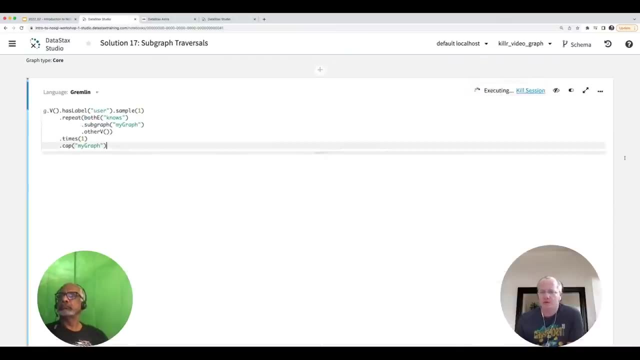 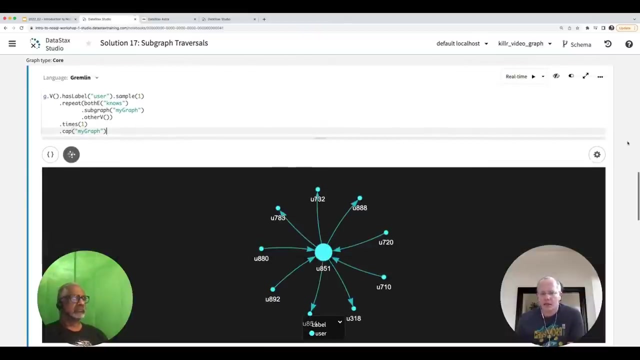 example. So let me show you a little bit of a maybe, maybe- subgraph traversal example. Okay, we're using the same graph but we're going to traverse users here. So essentially I'm going to retrieve the neighborhood of one user and it's a random user, And that first one was only new. one other user, So it's. 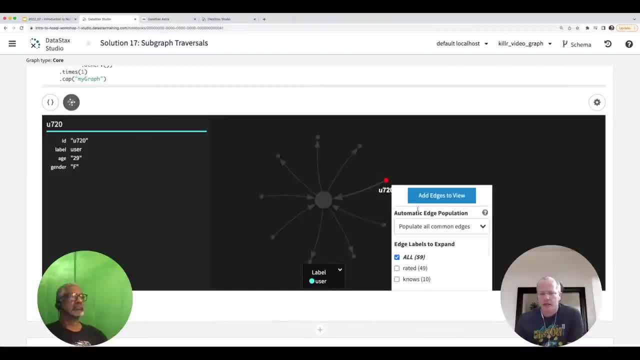 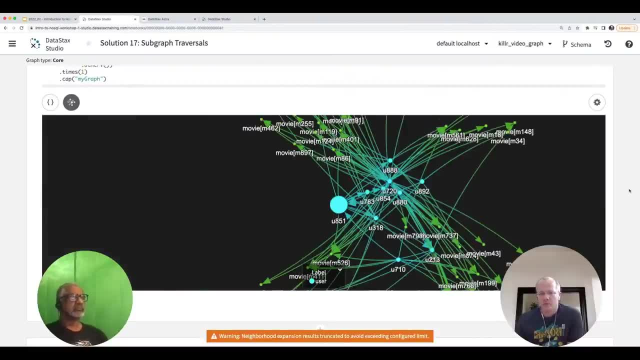 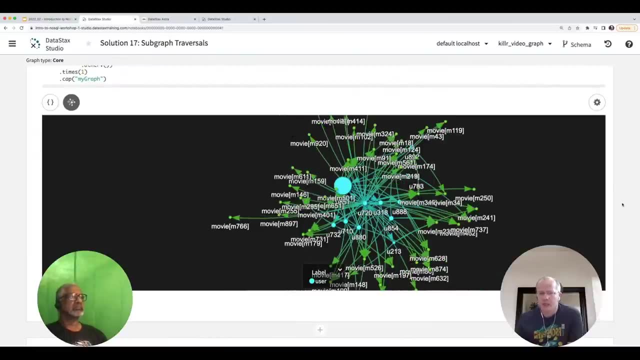 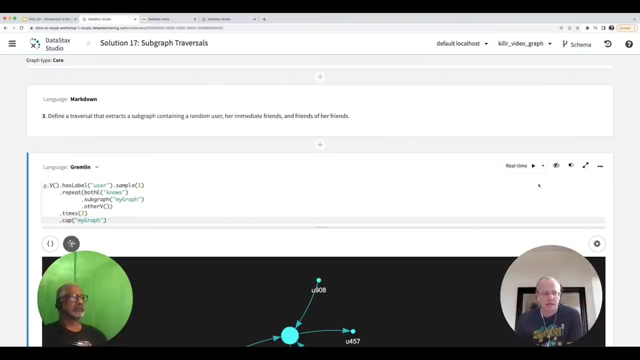 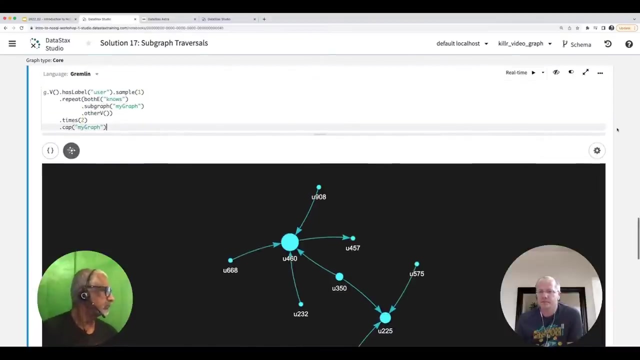 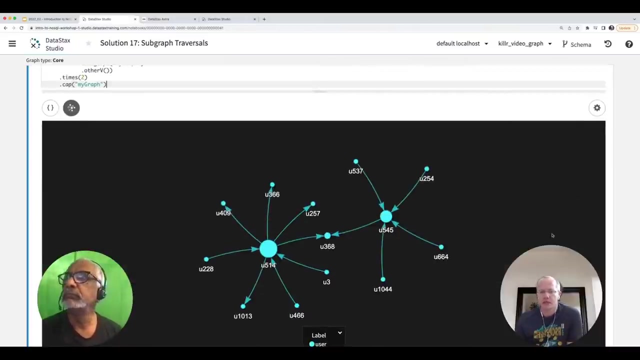 actually interactive so you can expand neighborhoods if you want and see larger neighborhoods. Let me take a little bit of time. So a more interesting example: maybe: finding friends of friends. so it's so, and again, this is a random- Okay, random- user selected and we find so the graph is different each time, okay, and 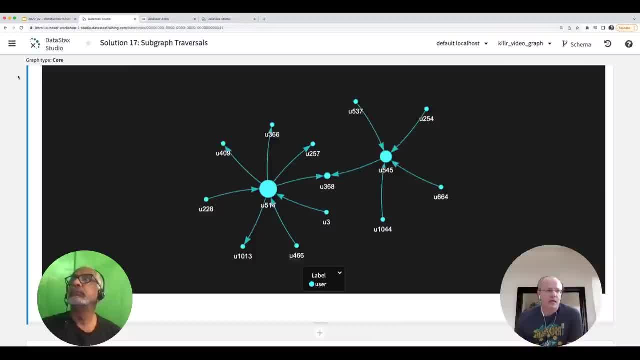 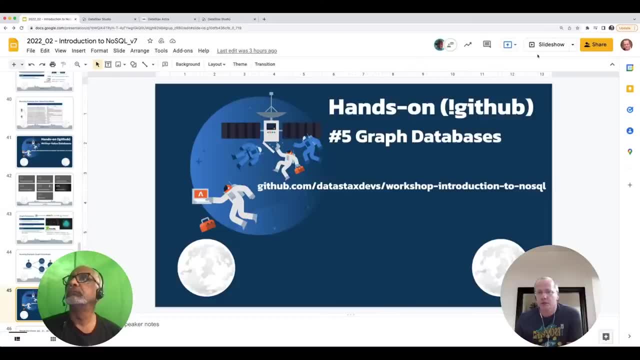 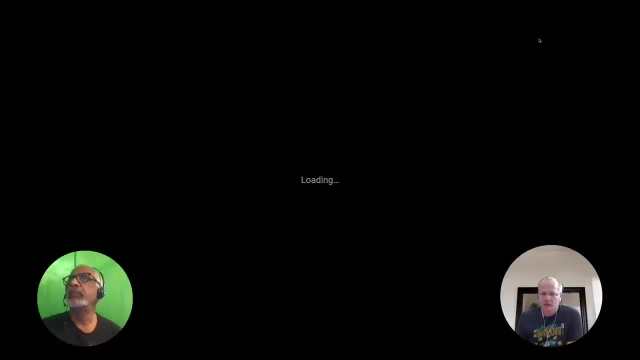 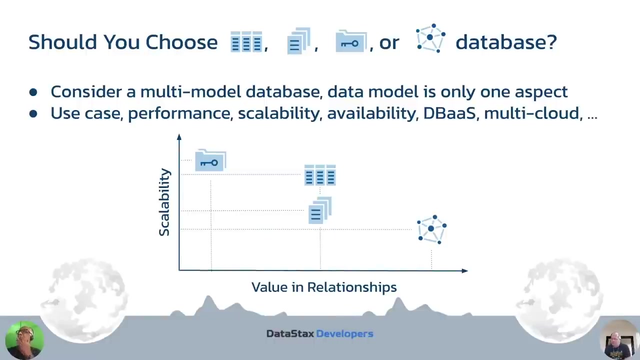 so on. So hopefully this helps to just get an idea of what is possible with graphs. So it's like doing the little bit of a social network type of processing in this example. Perfect, Yeah, I think that's great. Do you want to mention that our instructions don't really do? I mean, we have something. 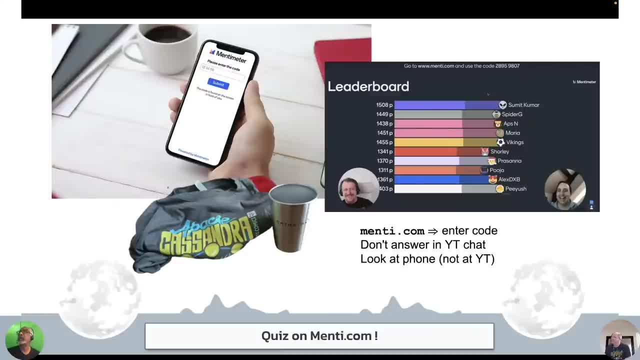 more involved with the Docker Compose if you want to try it yourself, You know. do you want to add a little bit? That's right. That's right, Yeah. So the demo I showed you is just running in the cloud and I'm just accessing that instance. 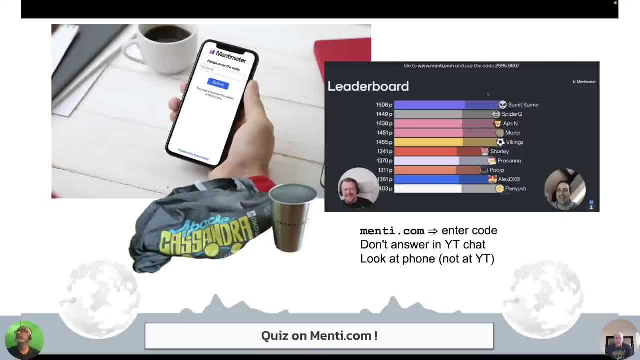 in the cloud, But you can also, if you follow the instructions. you can use Docker to basically have the image with data stacks graph installed and you can run it locally on your machine and do the demo, And this one particular is optional for your homework. 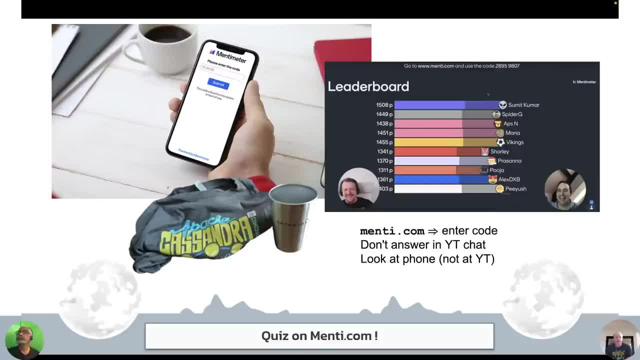 If you don't have time to do it, that's fine, but at least you saw the whole idea was here is to show you the capabilities, The capabilities of different databases, and get the feel, a look and feel, of how they actually work. 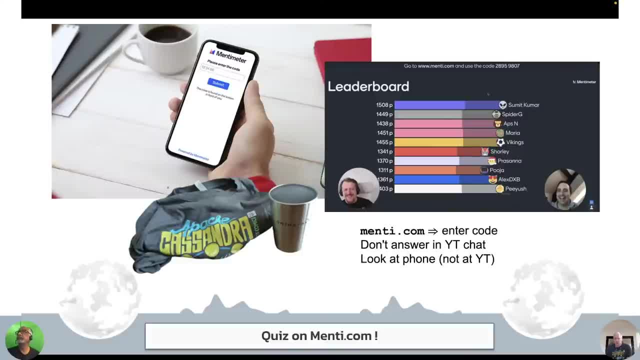 Okay, So now, which database are you going to choose? Which for your application, for a particular use case? Okay, So it would be a good idea to consider. So I think, am I Rex? am I still sharing the screen? 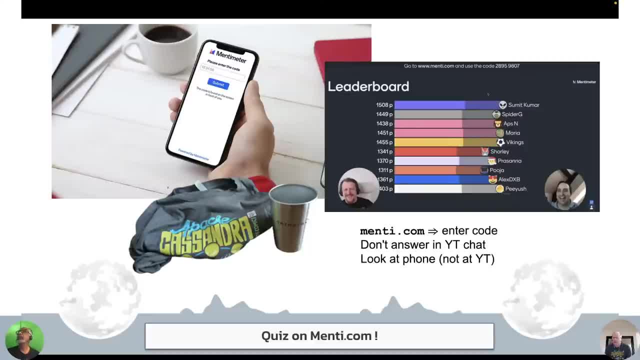 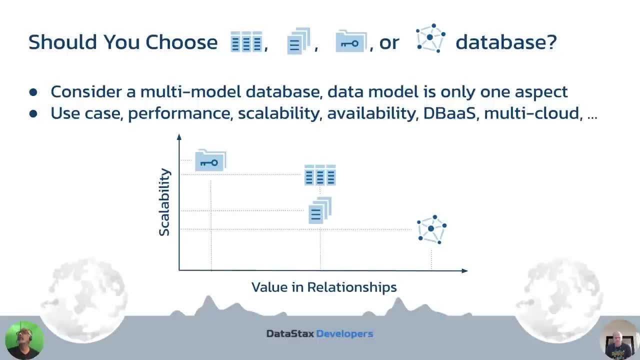 Let me do that for you. It's okay, But if you go to slide 46.. No, no, You go ahead. Finish. I will make sure my monitor is turned off and you can. yeah, yeah, sorry, go ahead. 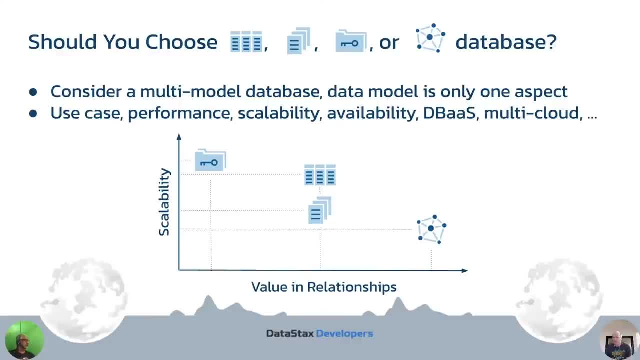 Keep talking, Yeah, Okay. So which one will you choose? The is, it is a tabular document, or maybe a key valer or graph. So consider using a multimodal database, Because different use cases will require different data model. 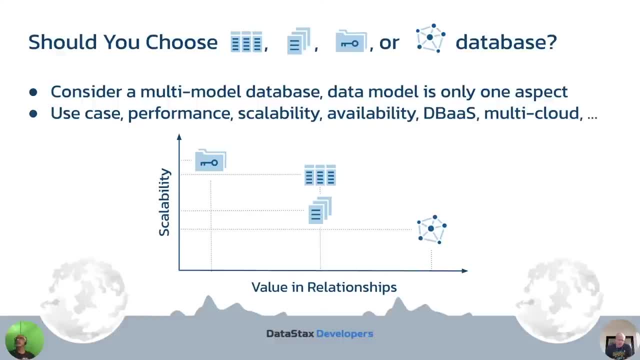 So if you're going to do session management, user session management for a web application, then maybe key valer is the best. If you're going to do traversals in the graph, you're going to look for paths between two people, connections between two people, then graph will be the best. 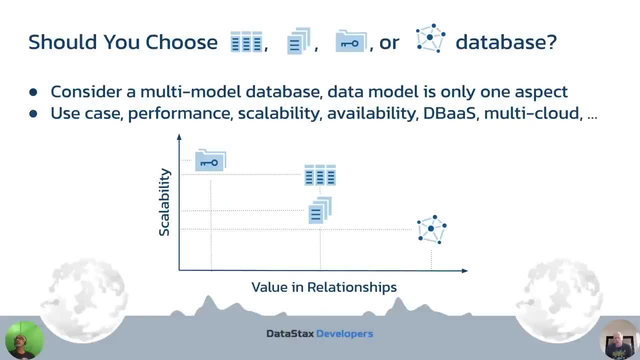 Most of the time tabular or document will be your choice. Okay, And they are kind of in the middle on this diagram So which compares scalability and value in relationships. So you can see graph databases they kind of have. they are more complex their queries. 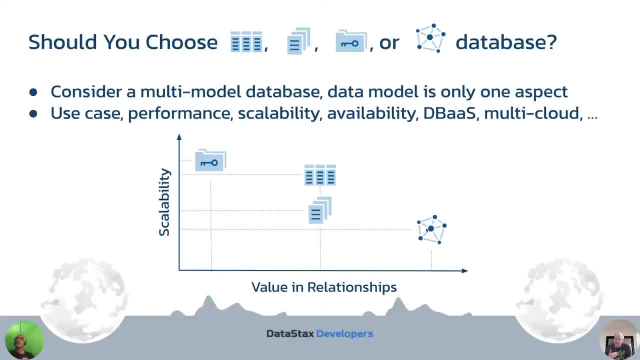 are more complex, So their scalability will be less than, let's say, tabular or JSON, And definitely the simplest one is key valer, so it has a higher scalability. Okay, And that is most of the time you will use. not most of the time, but if you're not only. 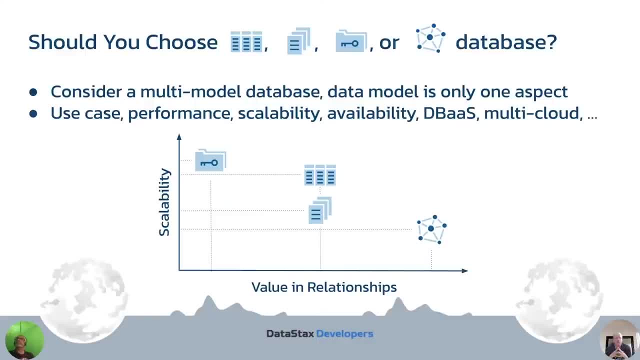 looking at one application, but you look at the platform. that involves multiple applications. like e-commerce may have multiple applications. fraud detection will have multiple applications that are doing different things. So sometimes you will use tabular and put key valer in front of it for caching purposes. 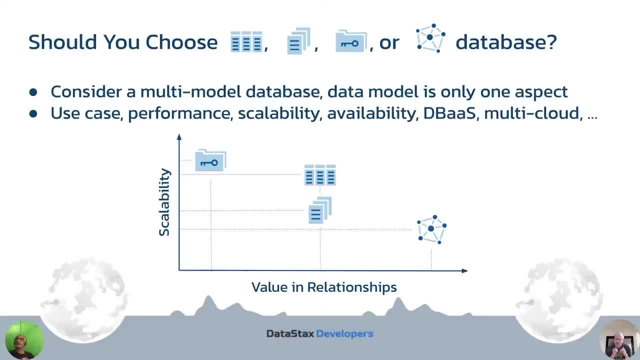 Tabular will handle more complex relationship, But for speed, Okay, You may only retrieve certain things using key valer, And certainly I've seen many use cases where you use graph for more complex things, but then the graph contains references that lead you to, for example, tabular database. 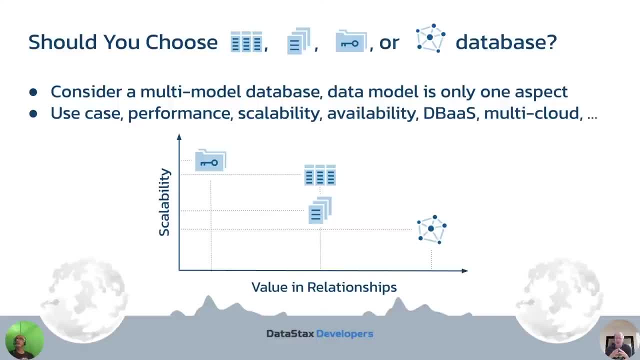 So, for example, you may have sensor network represented as a graph in a graph database, but the data that each sensor collects will be stored in tabular database. So it's not one model that's going to feed all the data. Okay, It's not going to feed all use cases. 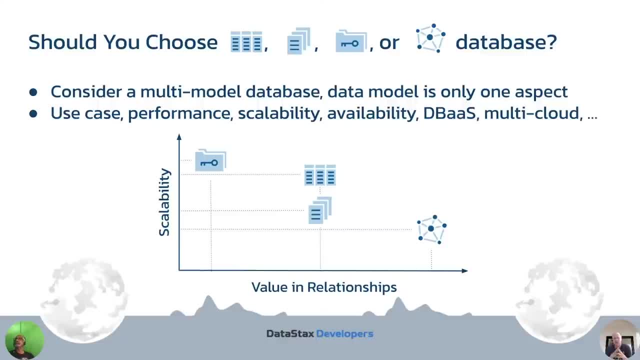 Definitely not. And besides the data model itself, you need to consider the performance. You need to consider use case scalability, availability that your application need. global distribution, multi-cloud: will it run multiple clouds on all or you find just one? 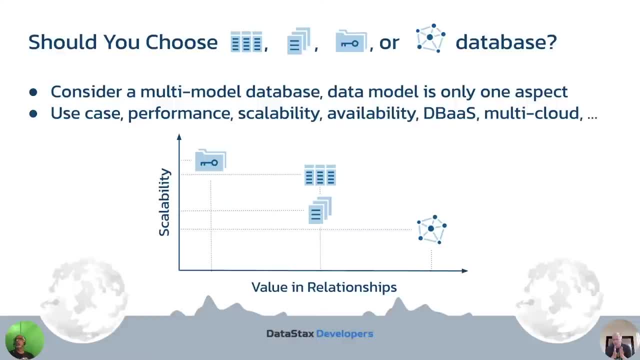 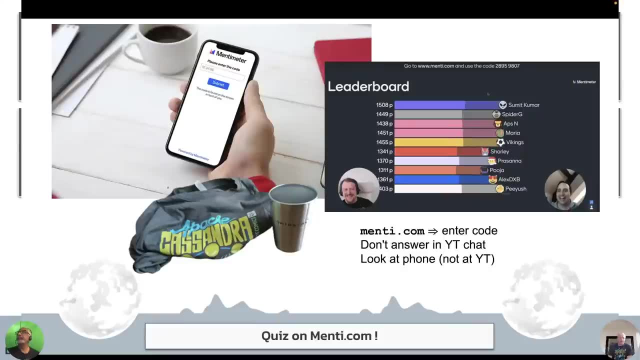 Whether you have database as a service offering on all of these. that will simplify your operations significantly. Okay, So, with that said, we are ready to talk about what is next And, Rex, you can take over Perfect. I know it's a very critical slide where you pick the database that you want, but please, 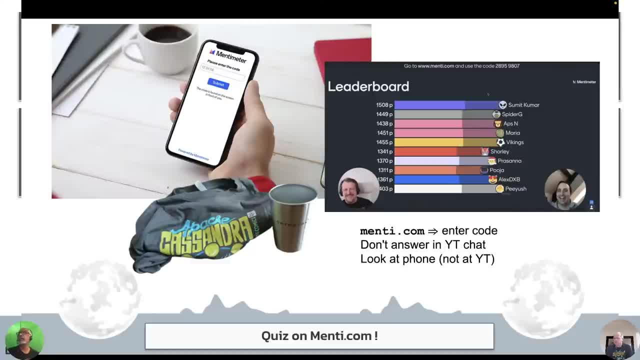 join us in discard, where you can get more information. We really don't have the time today and I want to be cognizant of time And I know that many of you join us because you want to do the mentee. Mentee is pretty cool. 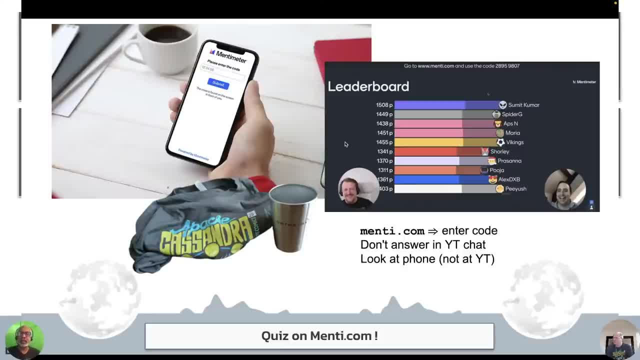 So we're going to jump straight into the quiz. Okay, So, as a special bonus, today we have top five. Okay, So usually we only give out swag to top three, but today we're going to give out swag to top five. 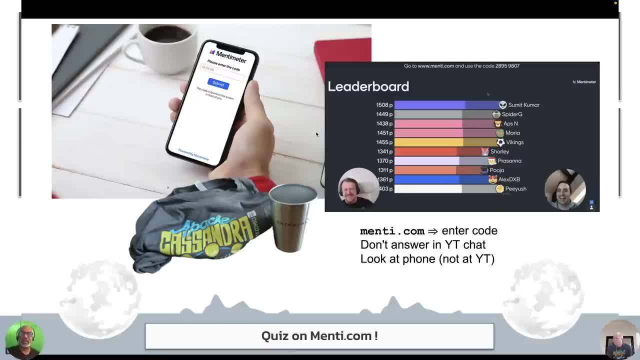 So stay here, because here's your chance to win swag and two more chances to win swag because, like I said, usually it's three, but it's five this time. Okay. So, with that said, let me jump to mentee. 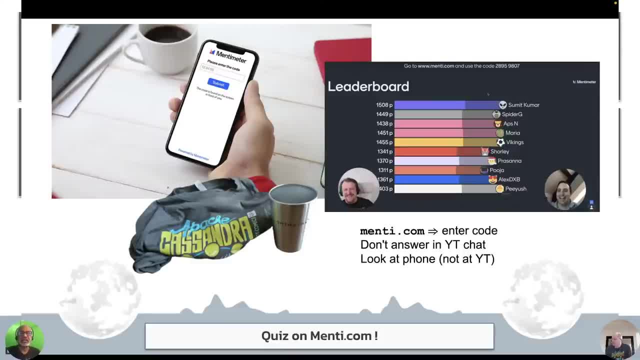 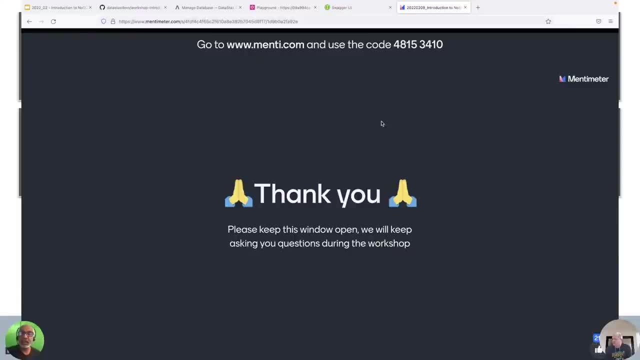 And again, if you don't have the code, ask Okay. So if you don't have the code, ask nightbot. nightbot is our, you know, basically our self-help system that will help you, you know, give you a mentee code, GitHub, you know, and so. 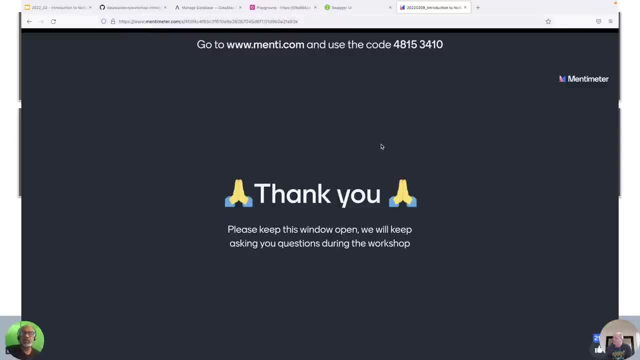 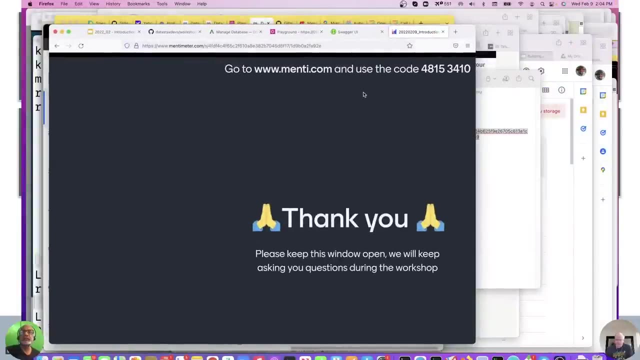 on and so forth, But if you want the code, it's here. Okay, Let me make sure I'm getting it right. All right, Okay, Code of mentee, use the code. Okay, Give me a second. Mentee is misbehaving for me right now. 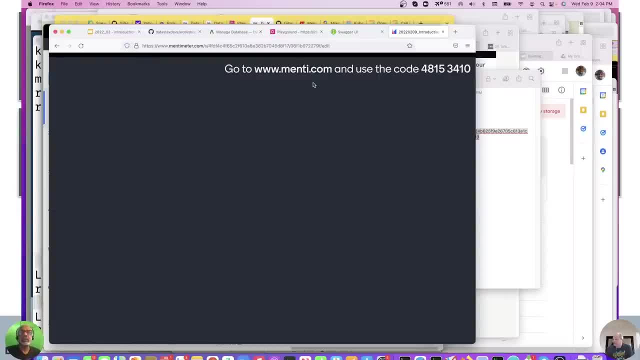 So let me start presenting and quiz time. Okay, Let me see how many people are joining. We need to have at least like I have about. oh all right, Leave the page Go away. Yeah, Okay. So here we are. 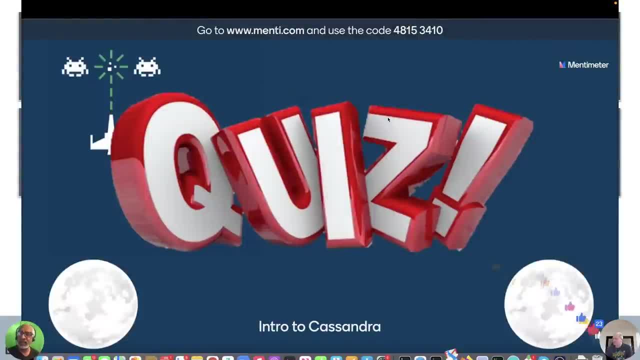 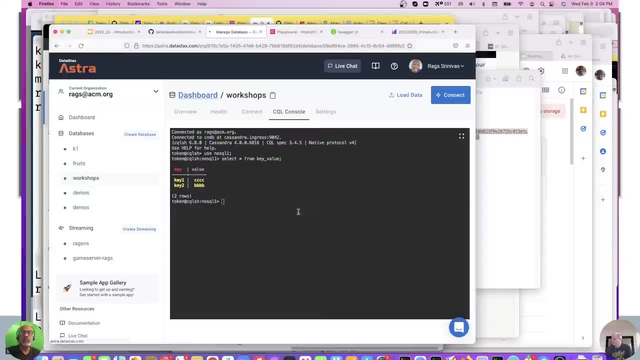 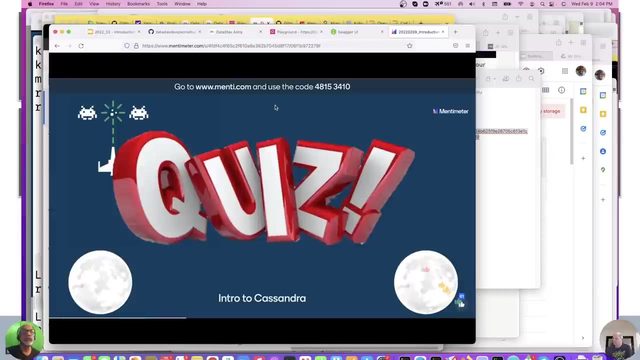 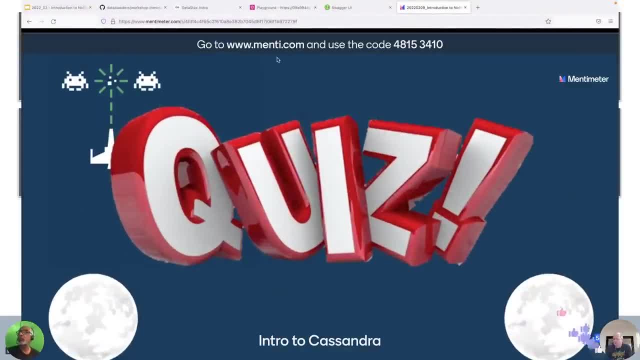 And again you can see 48153410. I'll make sure I'll turn on the music. We'll have some music here to play. Let me know if it's too loud and I'll turn it down. Okay, If somebody can give me a thumbs up that the quiz music is perfect. 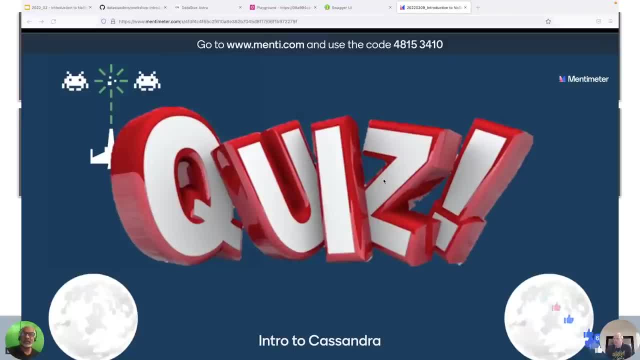 Then it would be great. I think I saw just one, Two, three, four, five, Four, five. Okay, with that said, let's jump to the questions, right? We don't have too much time, right? Okay, Come on. 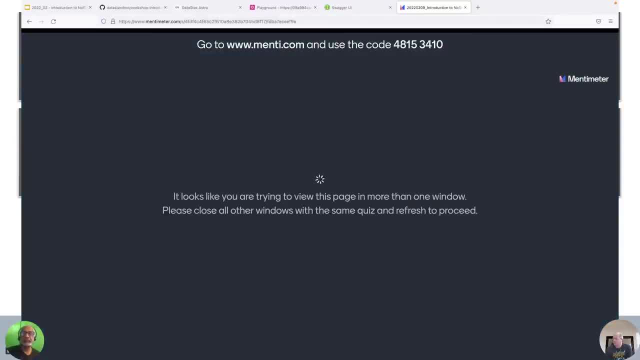 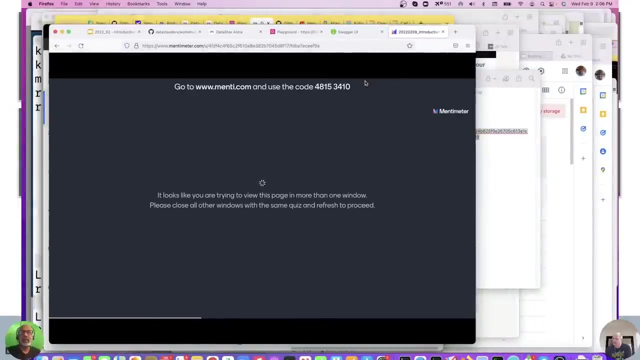 Okay, I don't think it matters. Hmm, Close the other window. That's all right. Okay, my bad, My apologies for this. Let me see if I can fix this. Let me try again. Let me see if it presents this. 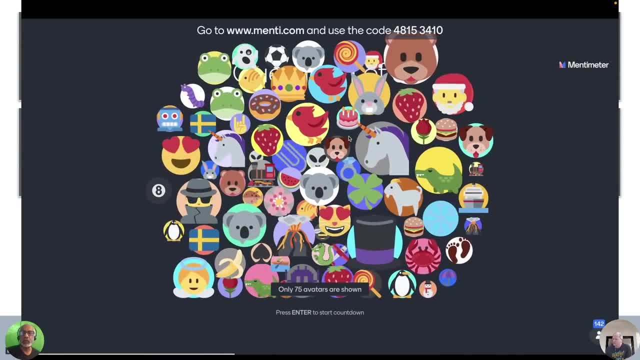 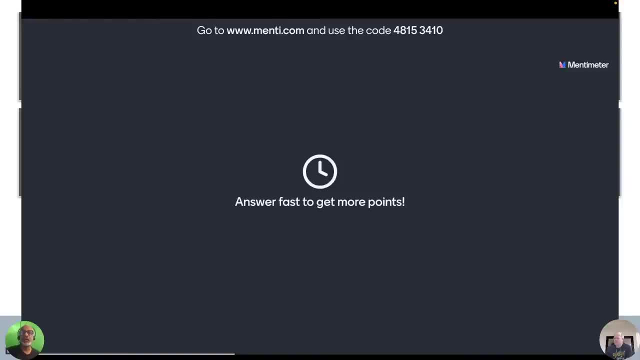 You may have seen some of these already. Okay, but let's keep going. Maybe it's a little finicky Sometimes. Okay, answer fast, but, most importantly, answer accurately. Which database should you use for high-growth applications? Aaron, you want to comment on this? 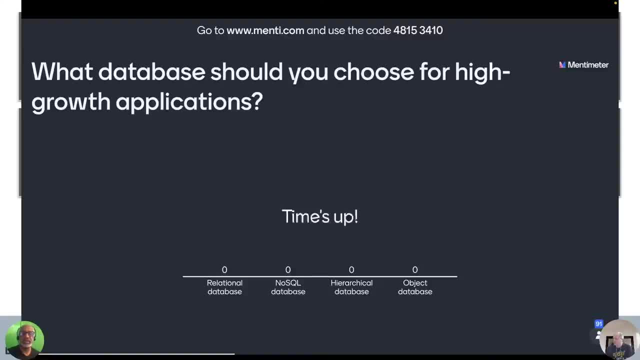 Relational database, hierarchical database, NoSQL database or object database, Perfect, Perfect. I think we have a few who said no, Not a NoSQL, okay, But I don't know if you guys are so passionate about those other databases, but I think NoSQL 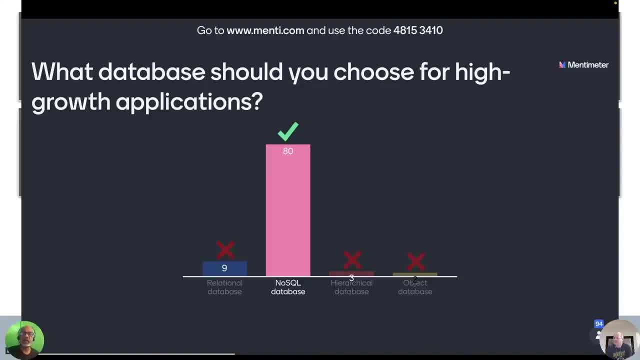 is really great for high-growth applications. Like I said, Facebook, LinkedIn, a lot of those born-in-the-cloud companies are using NoSQL databases in some form or another. Any comments you want to add? Artim, Yeah, There are some. 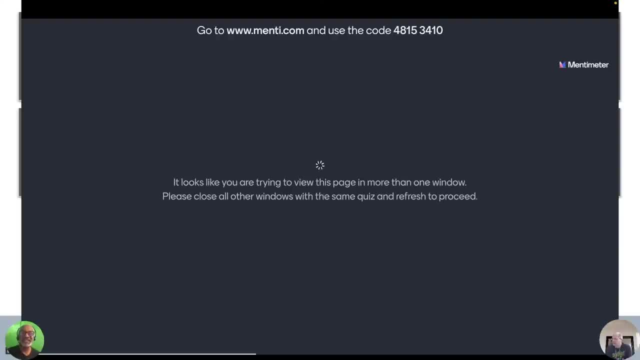 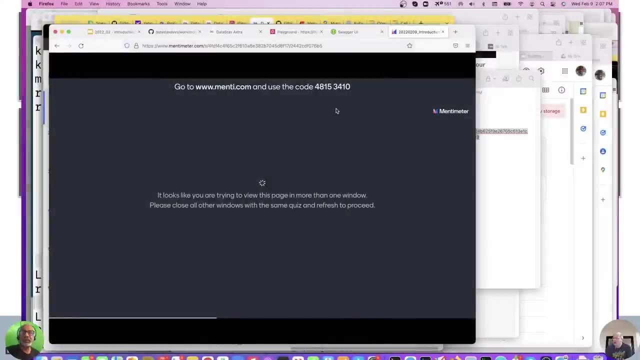 There are some Relational database diehards, Yes, So let's see how the leaderboard is working, Which is fine, And it's not letting me do this. I'm not quite sure what's going on here. Yeah, and by high-growth applications, we mean exactly the scalability and performance. 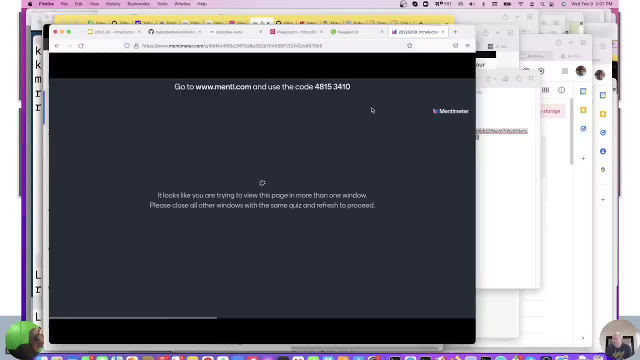 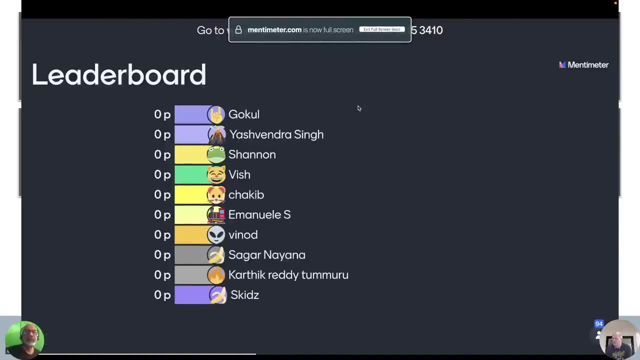 for large, very large data sets and large amounts of current transactions. So it's a high-throughput types of applications like you find in IoT or even in e-commerce, when the seller is serving multiple millions of customers, Exactly. So let's see how the leaderboard is facing looking 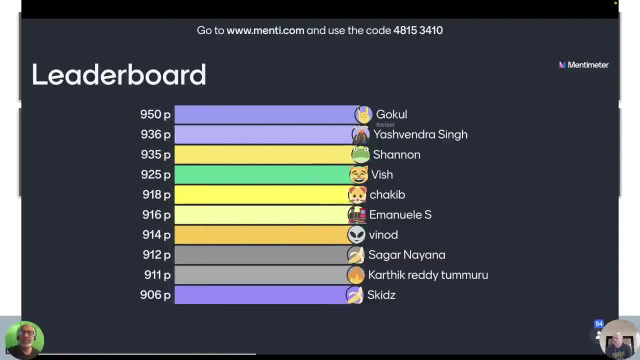 We have Go Cool as the fastest, Yeah, And on top of the leaderboard, Yashvendra is next and Shannon's kids could come through, you know, because the top five is going to get swag today. Okay, That's it. 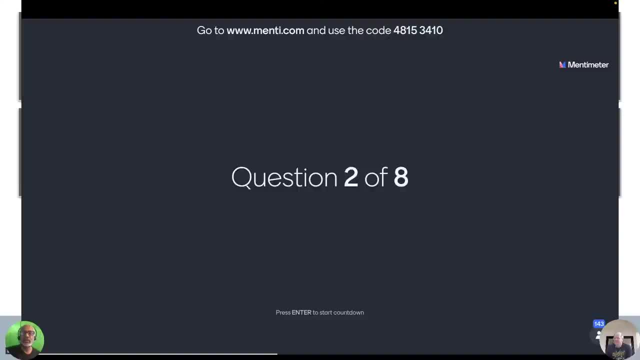 Let's move. Very close competition. It is close. It is close as always. Yeah, Question two of eight. Answer fast And answer right, All right. Additional benefit of NoSQL database. What is it? Look at your phone, not on the chat. 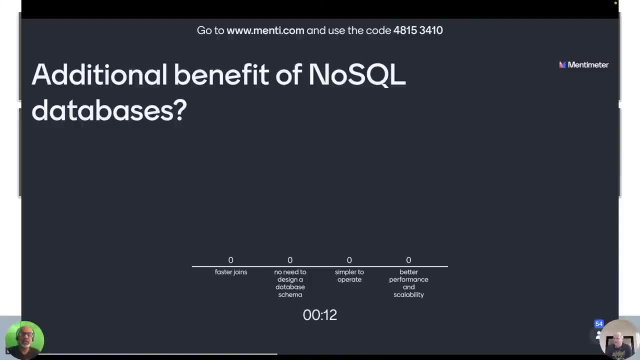 Is it faster joins? Is it no need to design a database schema? It's simpler to operate, Better performance and scalability. So you want to comment on this, Artem, Especially since a lot of people said no need to design a database schema. 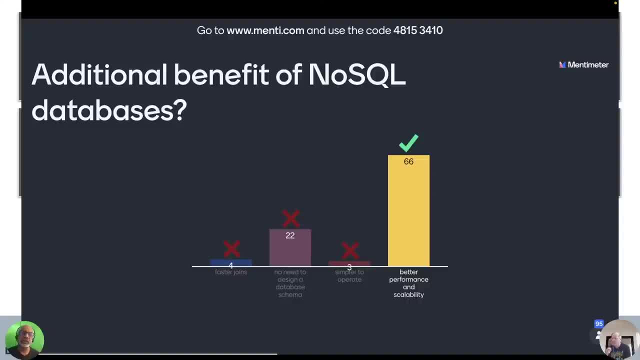 Is that? why would many people think that, Yeah, I have a bit of a delay, So but yeah, no need to design database. schema is probably the to document databases. Indeed, it can be one of the advantages, But just understand that you still need to think about structure of your documents. 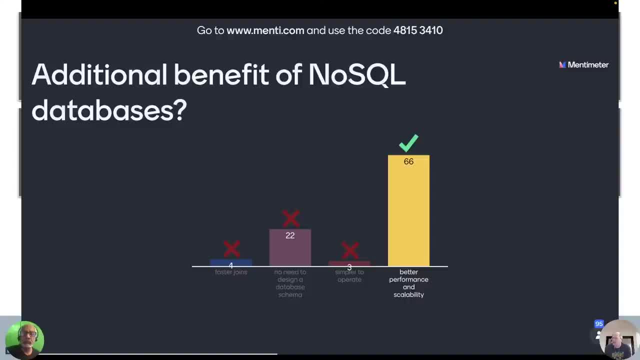 It's not just. you cannot just randomly put things there. You need to think about what will be nested where, what types of arrays you will use, how you're going to access data. Otherwise, it's always you design your, you model your data based on the access patterns. 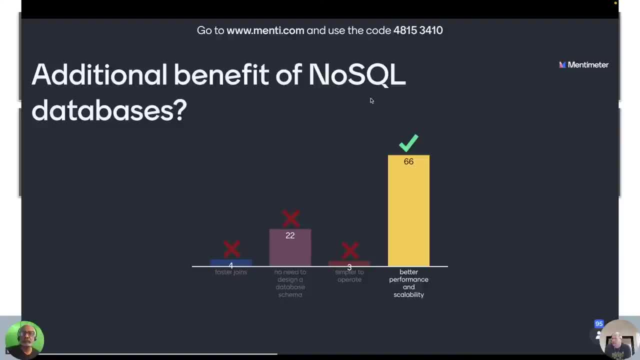 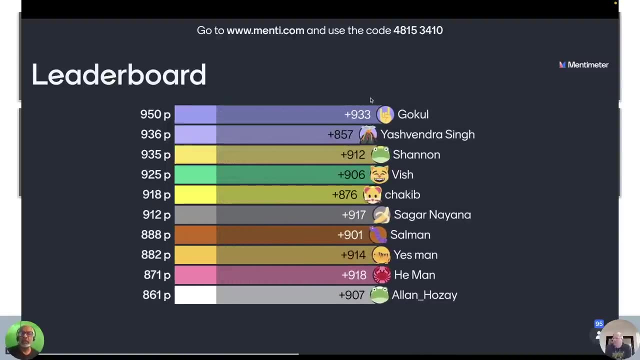 for any types of any type of nodes, SQL database. So you will still have to think about data modeling and schema inside of those documents. Moving on: Sorry, But indeed there is. Let's see how the leaderboard is shaping up. 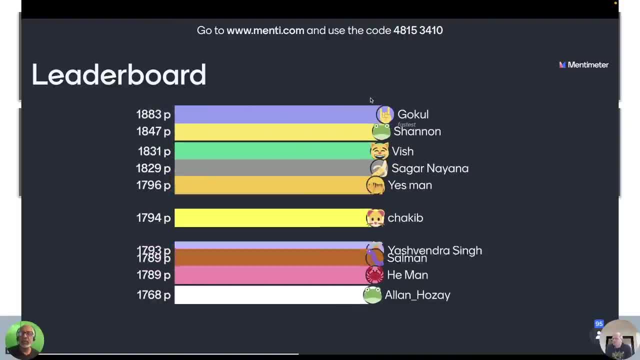 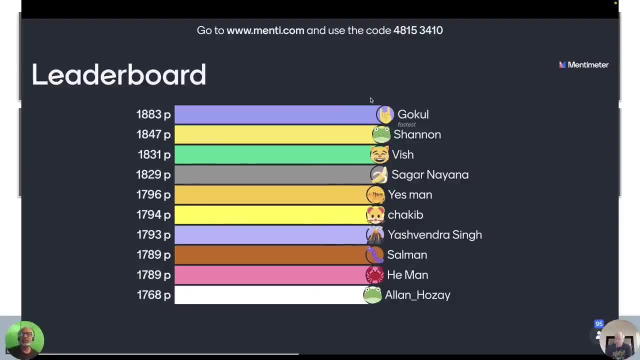 Let's move on. Looks like there may be some change, Maybe. Oh, Shannon, Tom jumps to second. Gokul is still fastest And you know he's on top of the leaderboard, But anybody's game at this point. 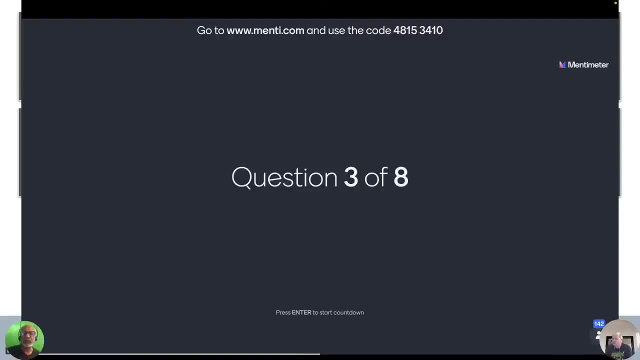 Okay, Moving on Next question, We have five more, I think, or six more, Right, All right. Answer fast, but, more importantly, answer correctly. What is AstroDB? It's a local in-memory version of Cassandra. Cassandra is a service on the cloud. 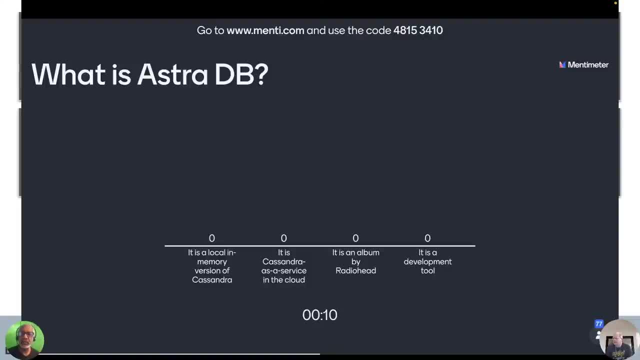 It's an album by Radiohead I distinctly remember. Maybe it is And is it a development tool? Is it maybe an IDE, Maybe an IDE? Wow, I think we did our job right. We got most people. Some people thought it's a development tool. 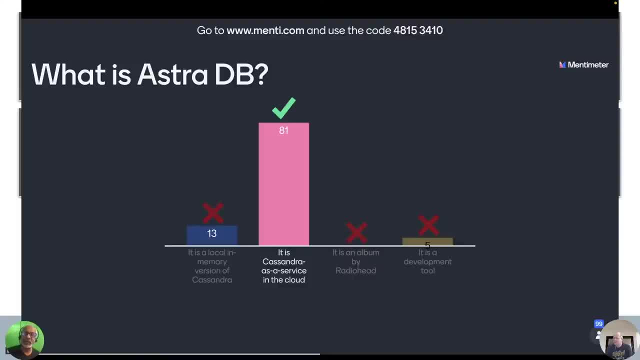 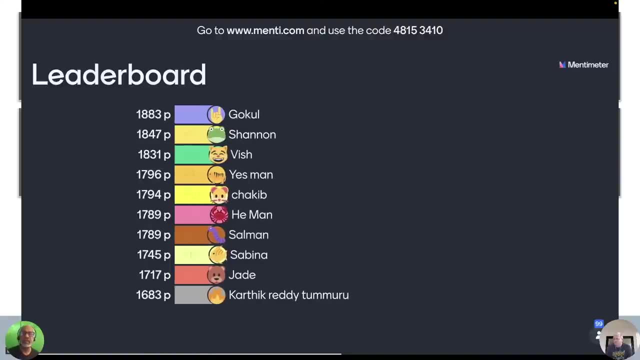 It is a development tool in a way, right, You know, but really it's more importantly, it's Cassandra as a service on the cloud. Let's see how the leaderboard is shaping up. You know we got to move a little faster here, right? 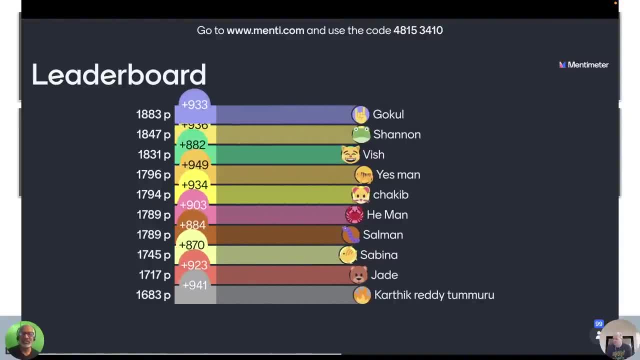 Database as a service. Yes Database as a service, Cassandra as a service, Database in the cloud. You know any of those Yes man, Whoa Was fastest And Shakib, you can still get to the top three. 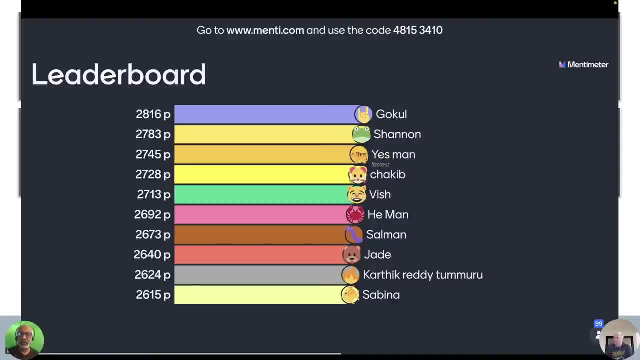 Gokul still maintains the lead. We have Karthik ready. Timuru is below but could jump Sabina. you know you could get to the top two. Vish anybody's game right now. right, There is He-Man and Yes-Man. 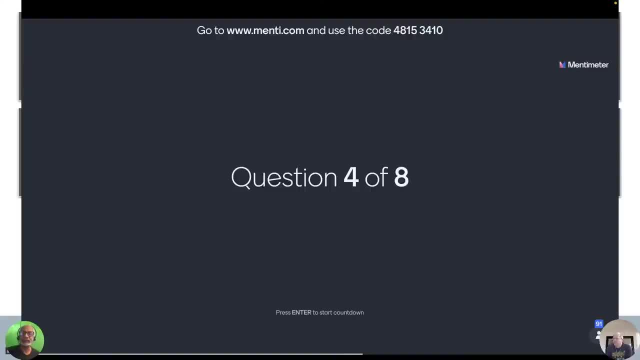 Wow, Interesting. Okay, Now question four of eight. We are at the halfway mark. Which NoSQL database organizes data into tables with rows and columns? Is it relational database? Is it a tabular database? Is it a document database? 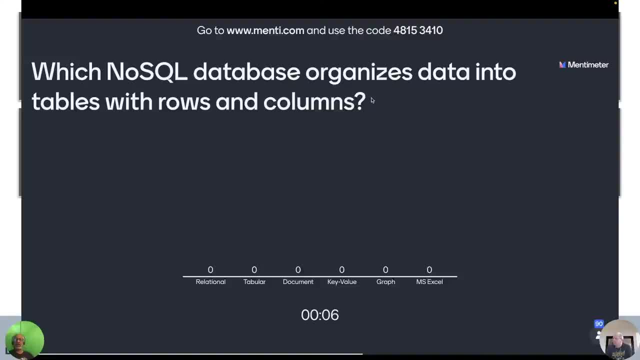 Key value Graph Or our good old friend Microsoft Excel. I wouldn't even talk about Excel, I know, Yeah, So thankfully nobody got Microsoft Excel, But I think most people got this right. Yeah, Excel is a desktop. 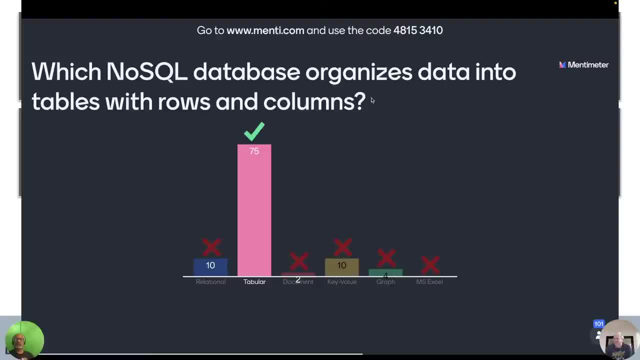 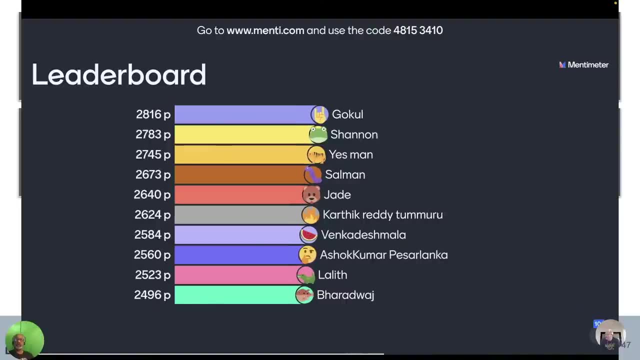 It's a desktop? Yeah, Anything you want to add color here, Artem? Yeah, All right. Moving on Leaderboard: Let's look at leaderboard. Let's see how it's shaping up. Ooh, It's shaping up. 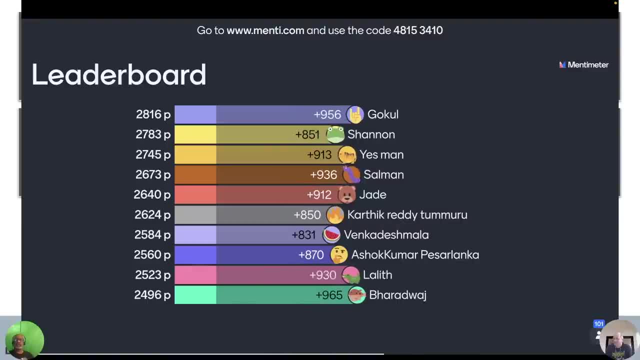 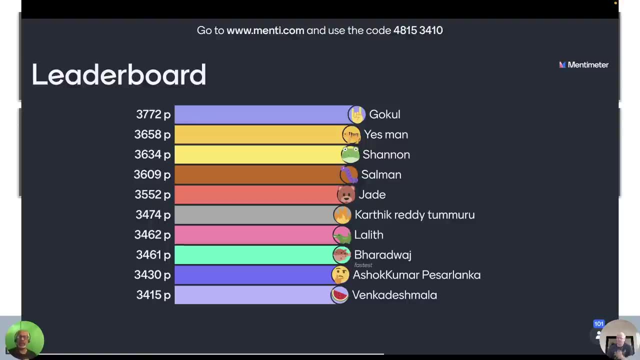 It's shaping up. It's shaping up. Ooh, Looks like Gokul might still be in lead Very close. Yes, man is making the move. Bharadwaj- Fantastic, He was the fastest. Then we have anybody else. 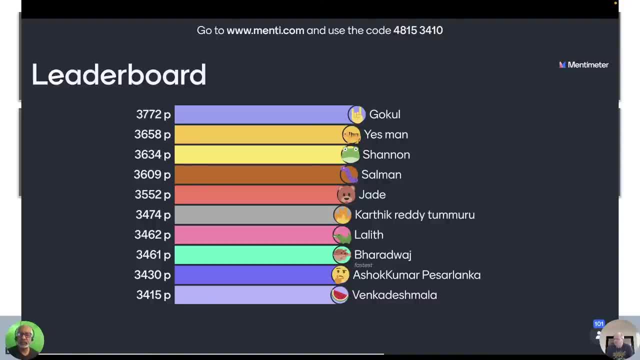 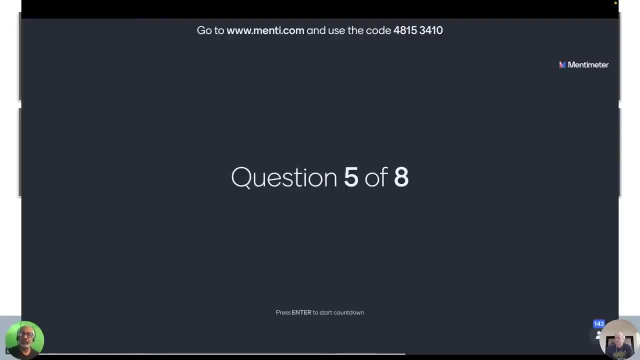 Venk Deshamala. you know almost there, Ashok Kumar, Anybody's game right now. We still have three more left, I think Three or four more left, Four more left, All right, Let's get through this. 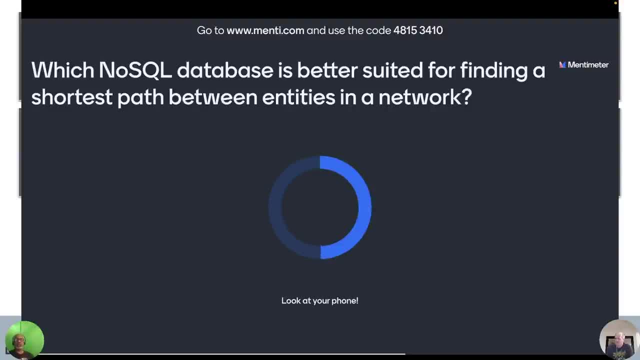 Answer fast But, most importantly, answer correctly. Which NoSQL database is better suited for finding a shortest path between entities in a network? Is it a traversal database? Could it be a document database, Graph, Key, value Or tabular? Seems like it could be any of those. 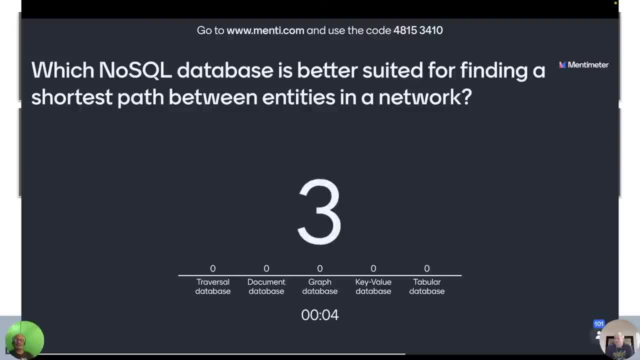 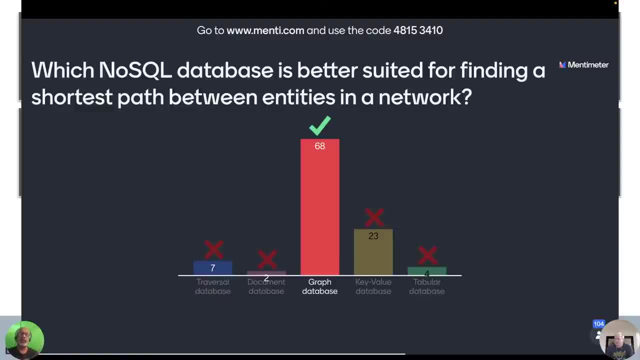 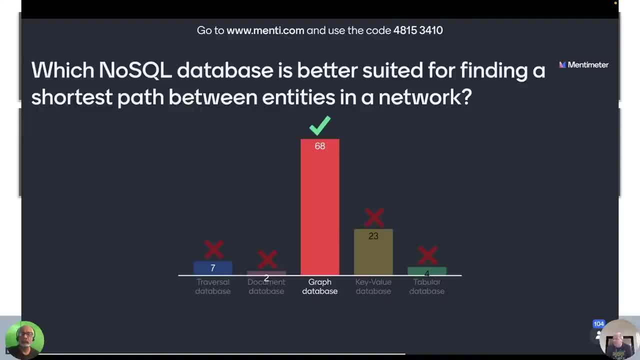 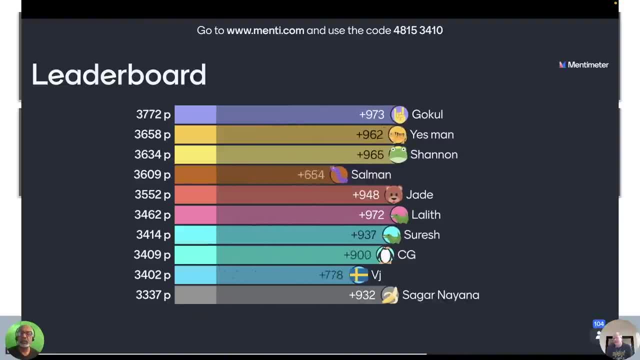 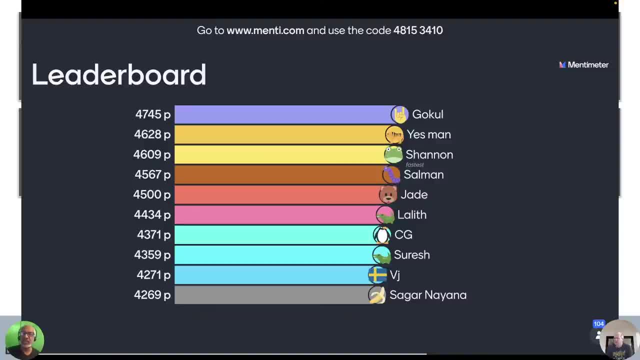 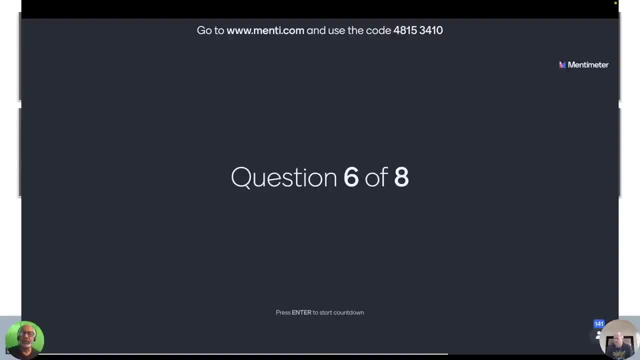 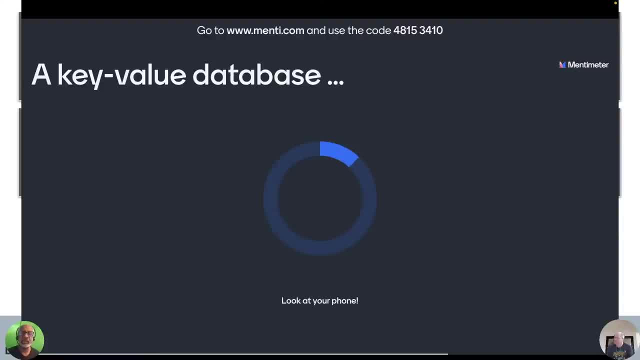 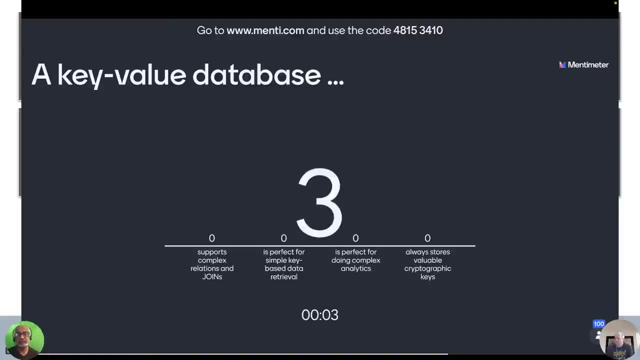 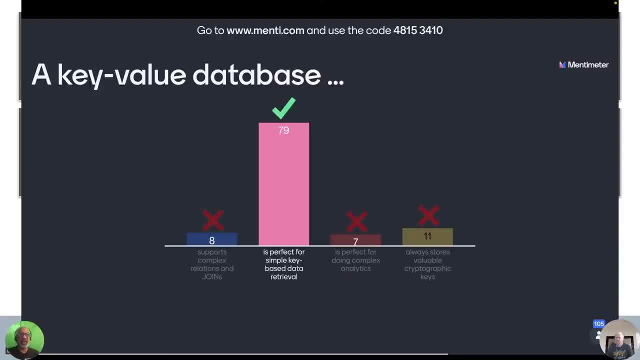 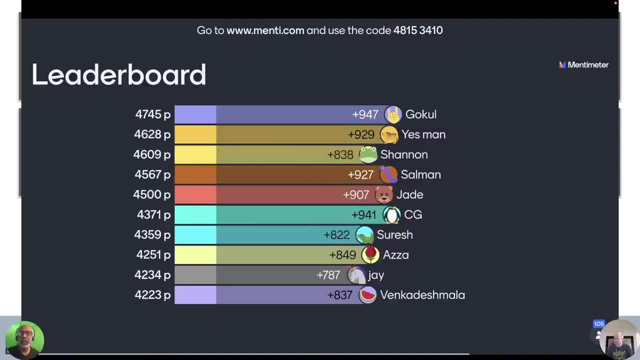 the leaderboard. will anybody be able to replace goku as the leader? maybe not. goku are the fastest, so there's no way you can replace. but there is still two more questions to go. yes, man could become the top man, so let's see how that goes. moving on, two more questions, seven and eight. 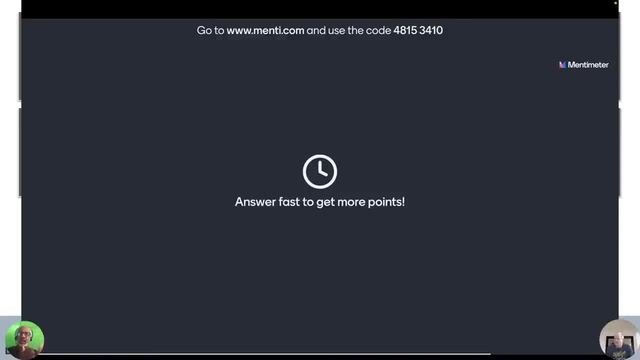 all right. answer fast, but, most importantly, answer correctly right. what format does astro db used to store and retrieve documents? ooh, this might be a tough one. this might be a tricky one. is it xml, is it json, is it html, is it binary or is it tabular? 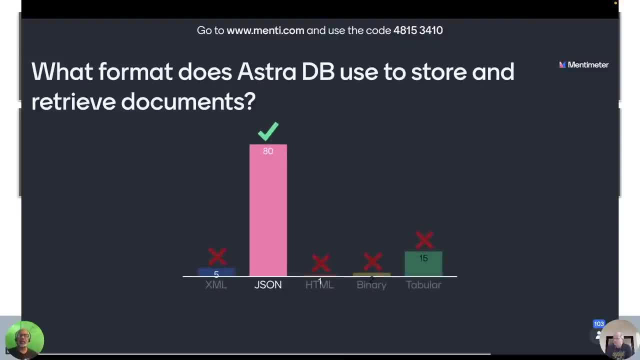 json, a lot of people got it right. you know tabular might be a little bit, uh, misleading there. uh, ultimately everything is stored as binary, right, i'm going back to my computer roots, right, but but you know, we store it as json, um, you know, and and uh, again, artem, um, maybe you should take over. 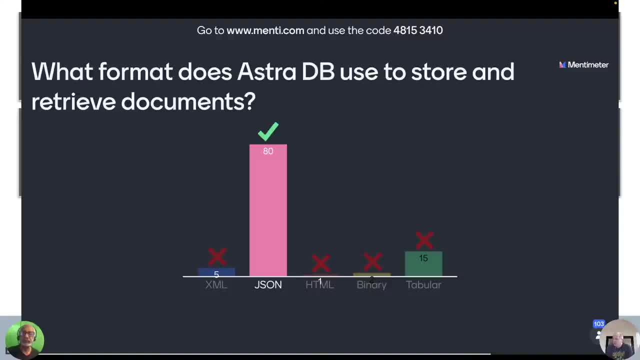 anything to add? yeah, well, for tabular. actually, you showed the example of how to store it in in um, just tabular in the table, right? so that's not another, not a incorrect answer. yeah, yeah, so maybe we should extend this and add both tablet and json. okay, yeah, you did. you did the insert for. 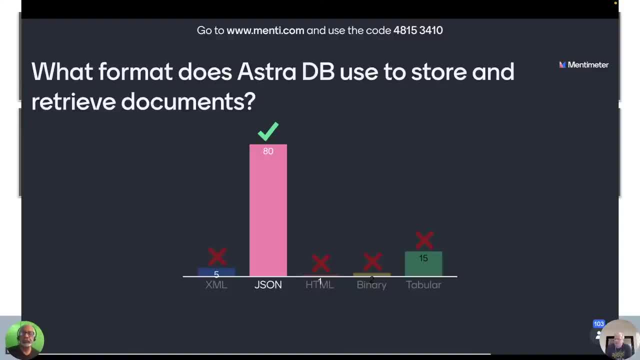 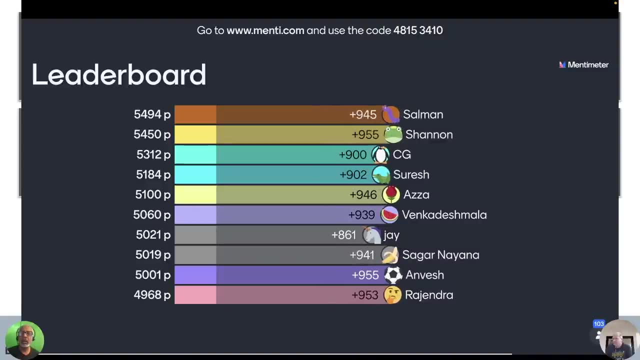 it's basically json data type for a column. yeah, all right, let's see how the leaderboard is. and for all the marbles, we have one more. oh, what happened here? looks like the leaderboard got completely changed here. wow, there are two fastest. i've never seen that before, at least not in the ones that i have conducted. 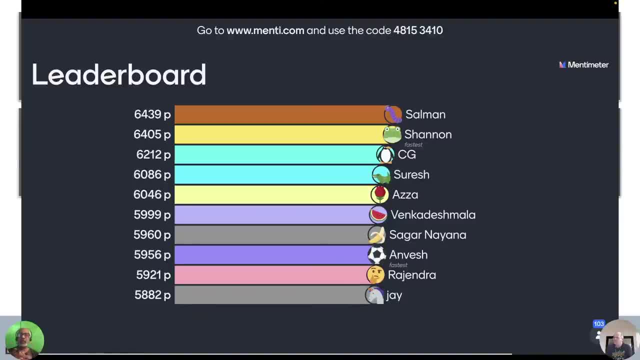 shannon and avanesh. so there is one final one. it could be anybody at this point. goku, you could still come back and and jump in. rajendra j, any of you can still make it. and remember we are looking at top five. so also this: you know, although the screen might say top three, um, you know it's going. 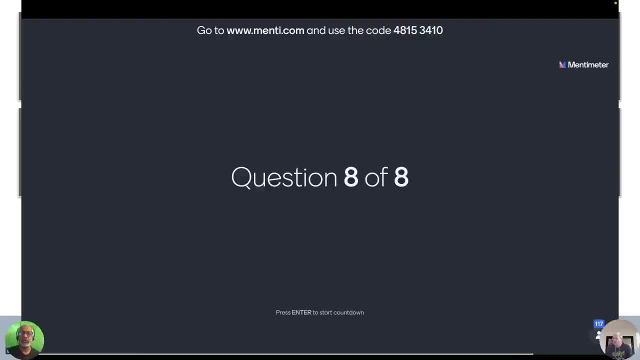 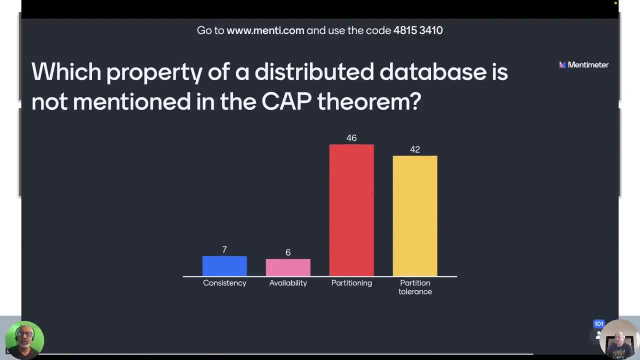 to be top five. okay, and we'll tell you what to do if you're the leader. last question: ready go. which property of a distributed database is not mentioned in the cap theorem? this is interesting. c, a, p, consistency, availability. is it partitioning or partition tolerance? i have a feeling it's got to be the last two. 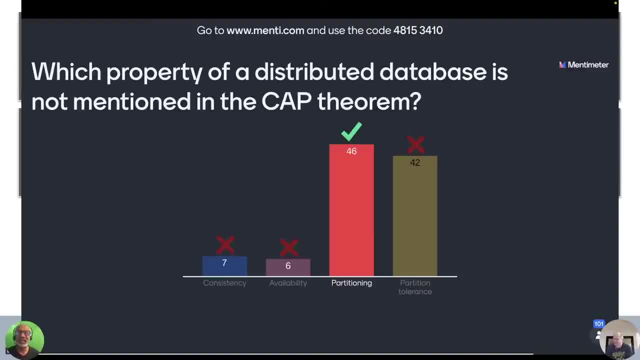 you really managed to trick them right. um, it's like partition, tolerance and consistency and availability is what is part of the cap theorem. partitioning is not part of the cap theorem, although you know when, when you talk about network kind of breaking up, it could, it could, kind of. 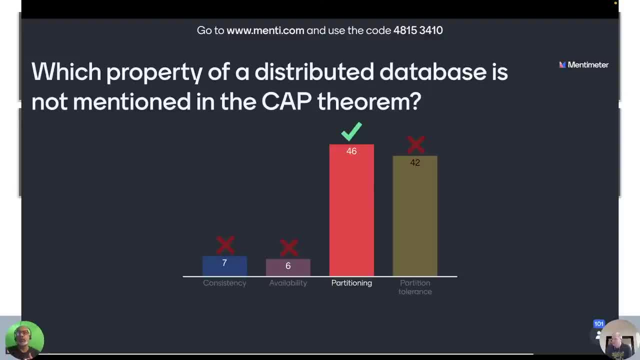 partition itself, right, but. but we are really more talking about the partition tolerance than the partitioning part itself, right? so the cap theorem really talks about the partition tolerance and not the partitioning in the traditional sense. partition tolerance, network failure: right. dividing network into sub networks, partitioning- 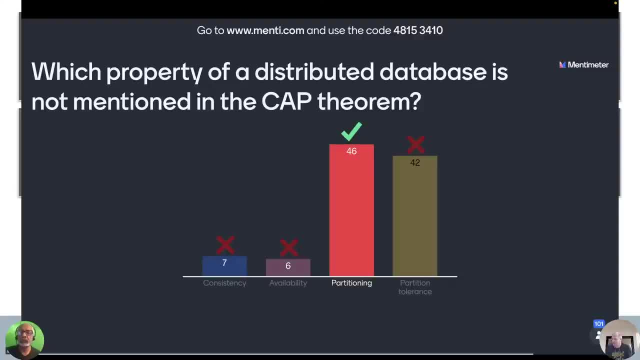 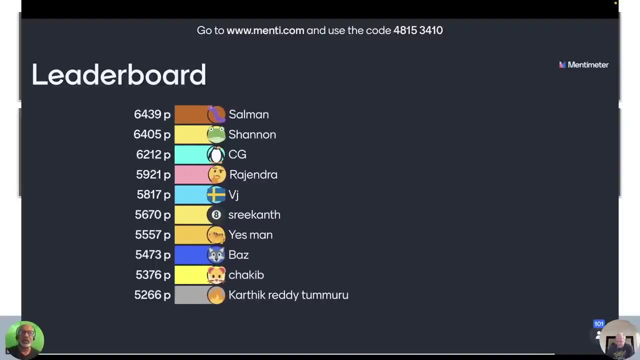 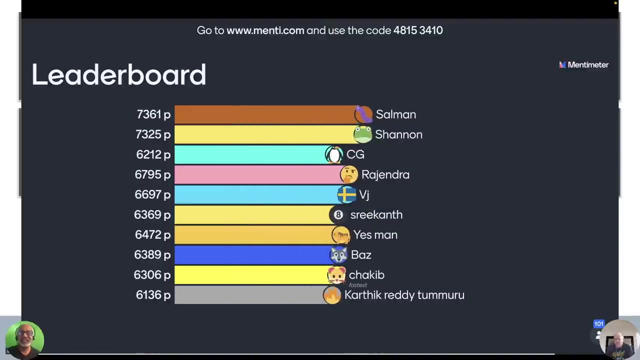 here we refer to data partitioning, dividing table into multiple partitions, or something like that. very, very tricky. you got almost the same number of responses for partitioning and partition tolerance. tricky, you. okay. you all right. this is the final leaderboard, but there may be surprises. surprises for sure, salman, congratulations, you are the winner. um. 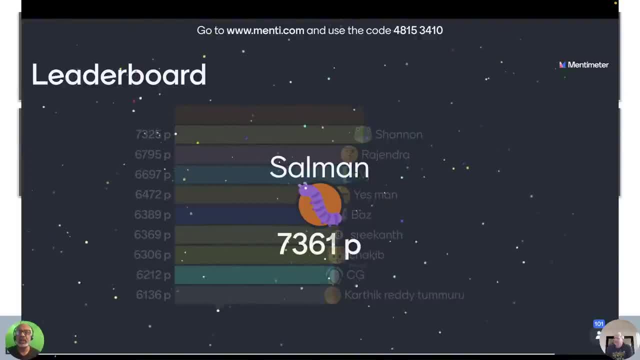 good job. so what, what i'll do is i'll, i'll let you guys, um, you know, take a screenshot of this, especially the first five, that is, salman, shannon rajendra, is it vj? and yes, man, um, take, take a screenshot and and we'll, we will tell you in a moment what to do with it. 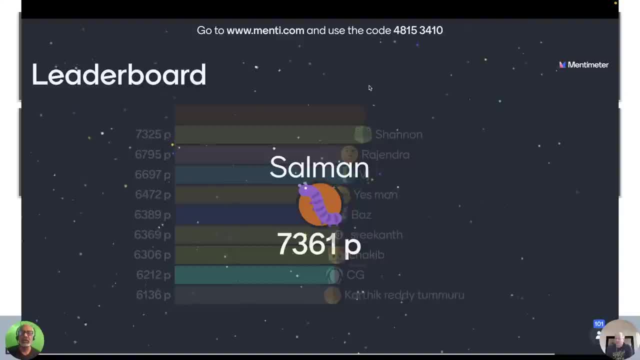 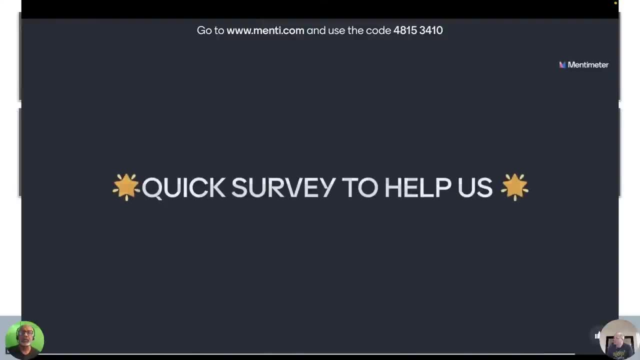 okay, um, i'll give you a couple of minutes or maybe a couple of seconds, uh, but, but i think it was a, it was a rather fun, uh, mentee. but in the meantime, yeah, if you can send us a quick survey, you know what, what? what do you like most? what should we improve? and we are pretty open. 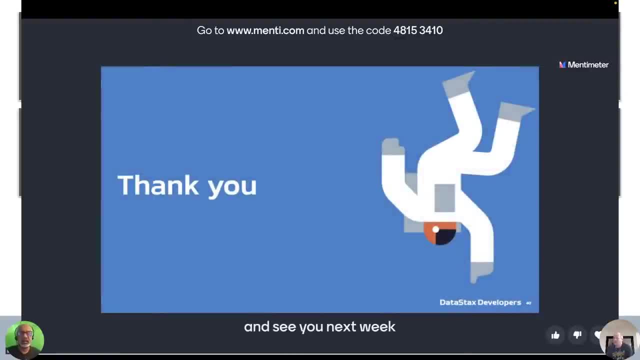 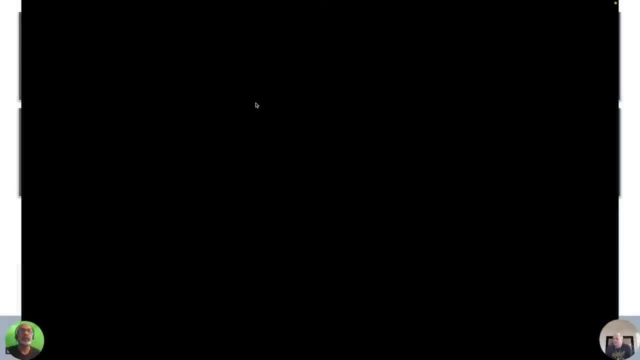 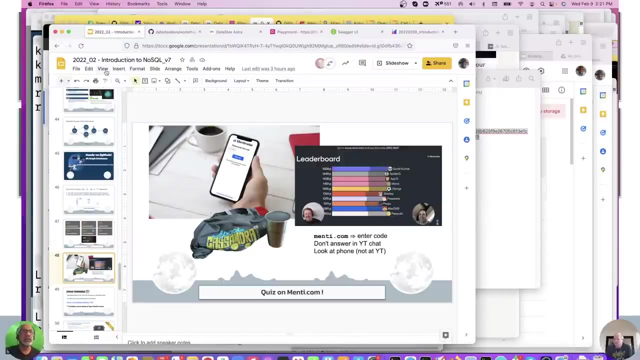 here, you know you. you should see the responses here. uh and and um, you know, let me go back to the presentation and we should wrap it up really quickly. okay, all right, let me go back to the presentation. we did the mentee and now i'm gonna wrap it up. 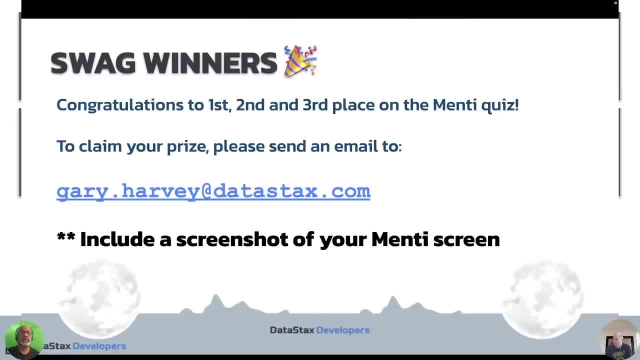 okay, so what do you do if you're the leaderboard? um, it says congratulations to the first, second and third, but we got some special permission today to give out more swag, so the top five are going to get swag. all that you're going to do is you send. 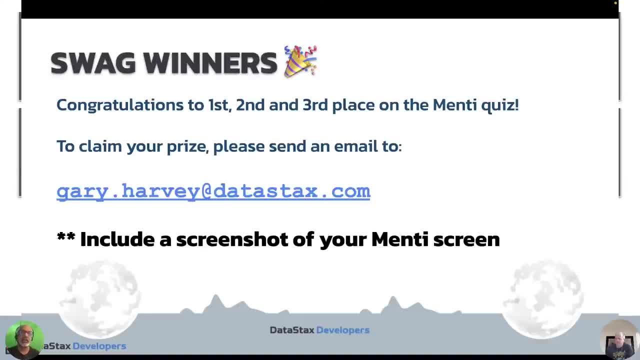 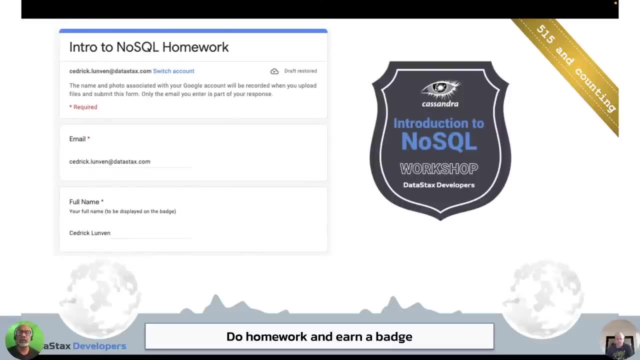 an email, take the screenshot and send it to gary harvey at datastaxcom and and you're good to go. okay, so again one through five, okay, um, please take a moment to review the homework. um, you know, if you hit uh exclamation homework, you should be able to see that um intro to no sql homework, you know. 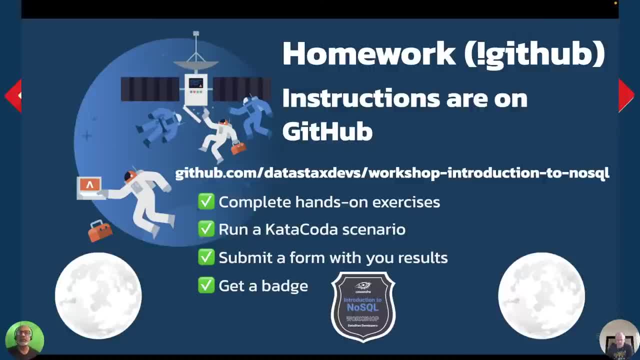 the exercises, uh, and there are some optional parts as well. okay, um, you run a catacord scenario: submit a form with your results and you're going to get a badge back. okay, nice looking badge, cool looking badge, which is the introduction to no sql. we also sponsored your education and certification. 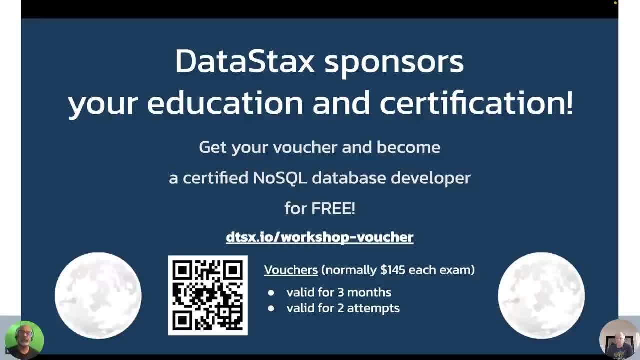 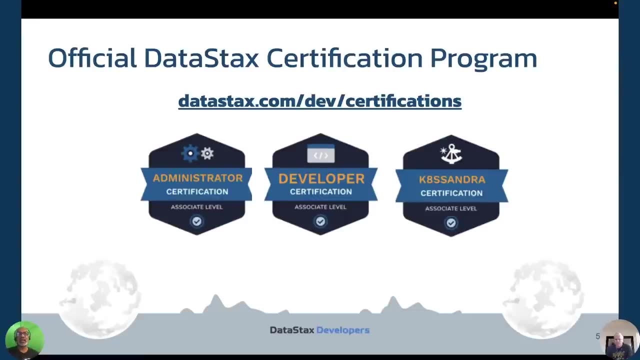 you know, if you want to scan this, i believe you can get a, a certification voucher that you can use. okay, it's valid for three months and valid for two attempts, and you can use it as in menus, please. okay, there are lots of other certifications as well. uh, you know, um, welcome to. 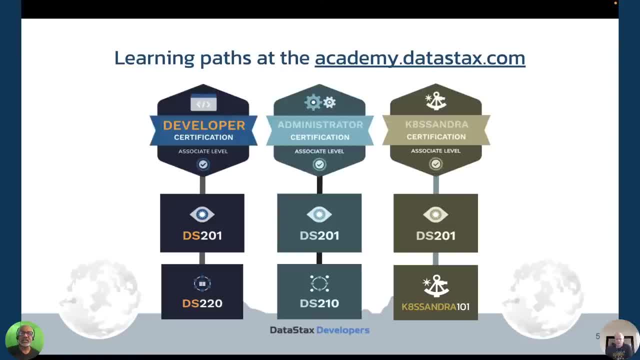 kind of check this out. if you go to datastaxcom, slash dev, slash certifications, you should be able to see all that and, like i said, plenty, plenty of resources you know for you to use. uh, you know i myself do a lot on the kubernetes side and kate sandra, so if you're interested in that side, you. 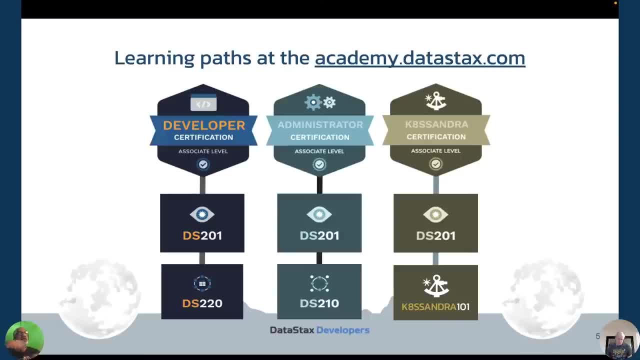 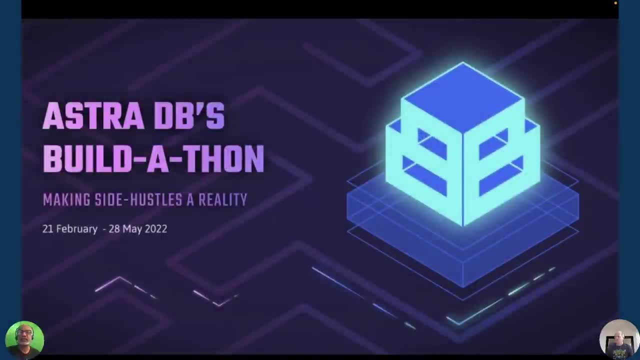 there are developer certifications, all kinds of cool things, uh. but more importantly, we have a build-a-thon that's going on right now, uh, and there are opportunities not just to win. i mean, i'm not gonna say that the t-shirt is not cool, t-shirt is cool, the swag is cool. 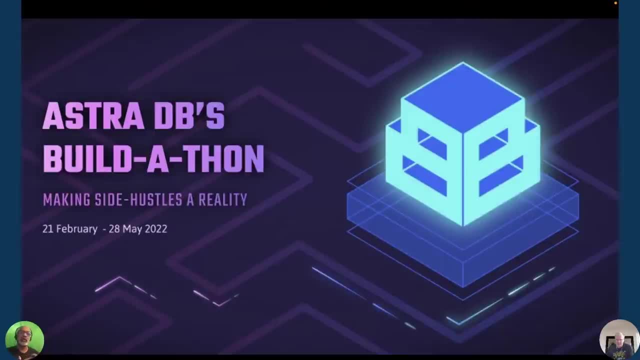 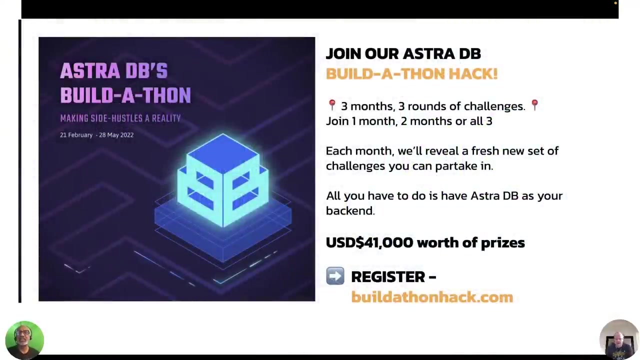 uh, but you can get money. actually, i believe there is something like a 45k us dollars, 45 000 us dollars, 41 000. okay, okay, correct me, yeah, and the largest price you can get is five thousand dollars, exactly, and it it actually we calling it the side hustles. we realize that all of you are. 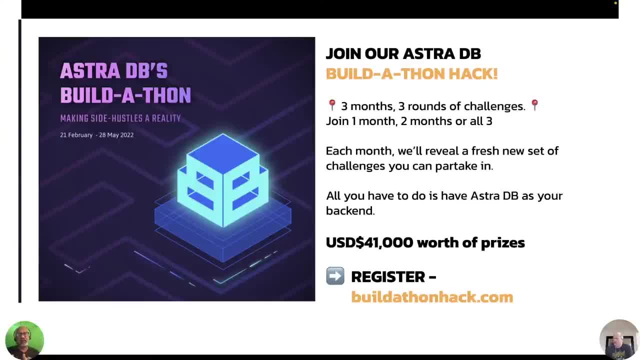 professionals, you know busy with your everyday life, but but take a moment to kind of try something with astra. maybe build an app for us and, and and put it in there. okay, um, and, and? you know, you can also win some money as a? uh in the process. okay, uh. all that the hackathon requires is you have to use astro db as your. 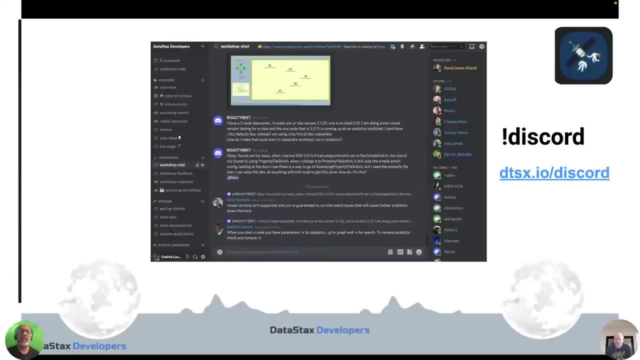 backend. okay, pretty straightforward. if you have some more detailed questions, you know, just join us at discard. discard is the place where you can get pretty much any questions you want answered. all of us are hanging out there. um, you know, we we really strive to answer your questions as soon as. 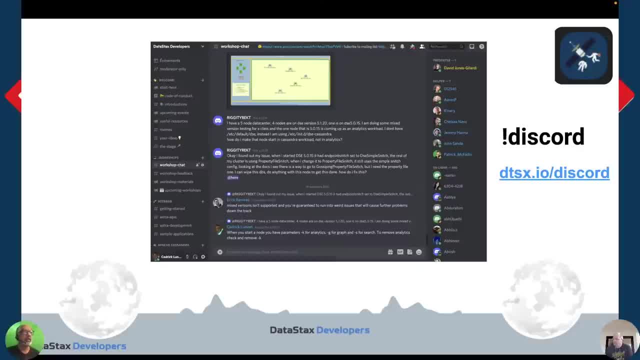 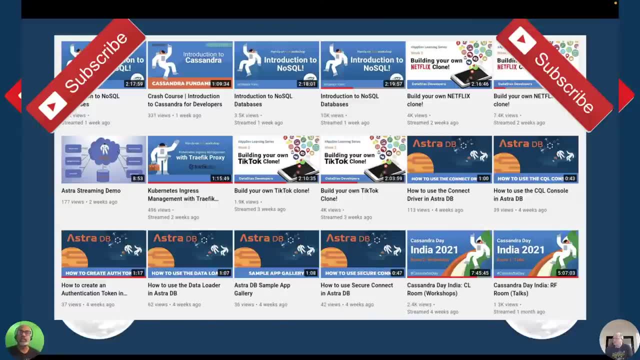 possible, um, but but again, um, you know you can help us by actually answering those questions as well, because you may have a little bit more information. um, do subscribe to our um. you know our uh channels, you know whatever. there are a bunch of channels that you can. you can subscribe to um. so take a.